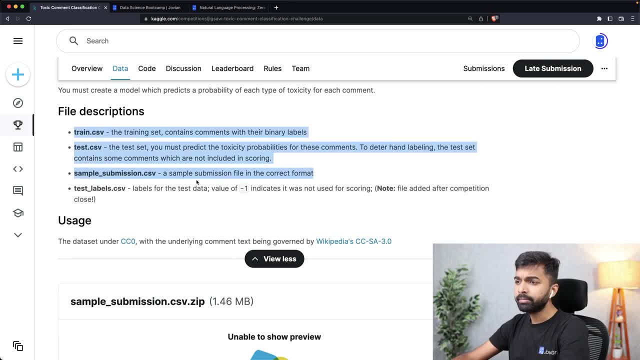 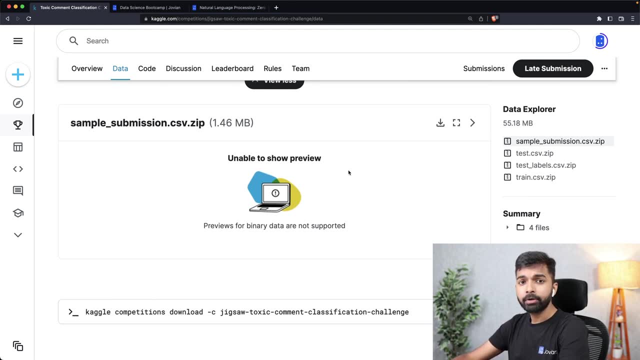 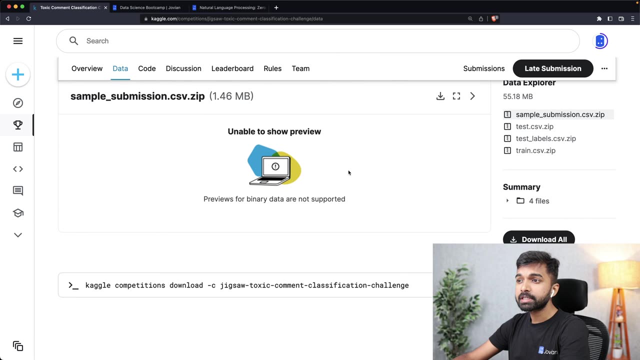 and testlabelscsv. So we will mainly be dealing with these three files, And one thing we can do is try to download this data set on our computer. But since we are going to use online, cloud-based Jupyter notebooks, we will download this data directly using the. 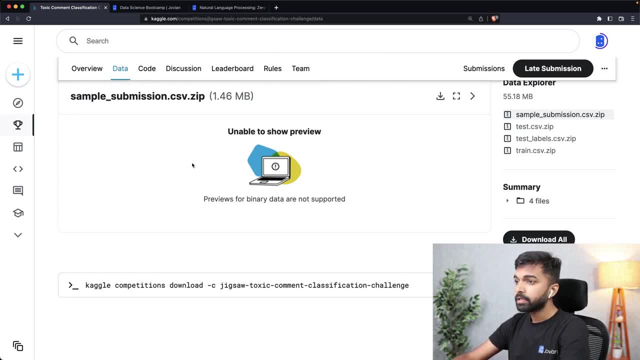 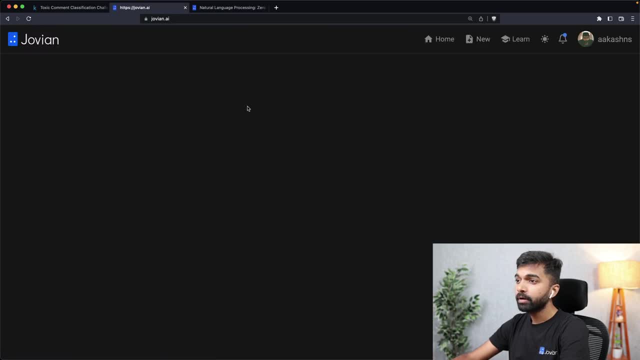 Kaggle command line tool, So let's get into it. I'm going to head over to jovianai and I am going to sign in here, And once signed in, I can create a new notebook. So I'm going to create a new. 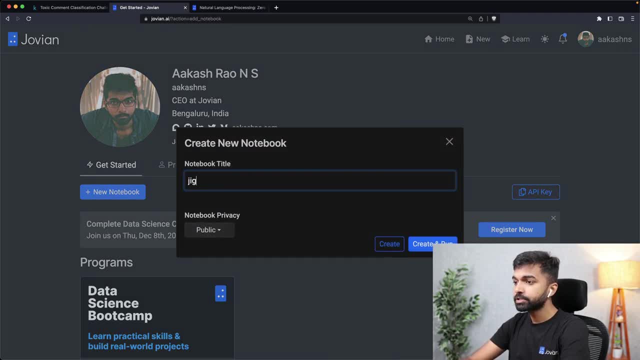 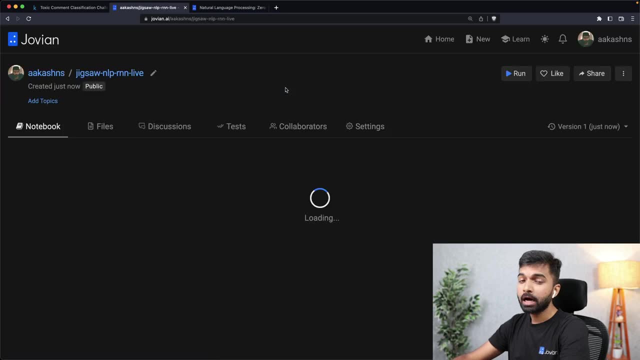 notebook. Let's call this jigsaw: NLP, RNN, live, And I'm going to create this notebook. So now I have created a Jupyter notebook that is saved on my Jovian profile. I can come back and check it out anytime I need. I can continue working on it Now I'm going to click run And I am going to 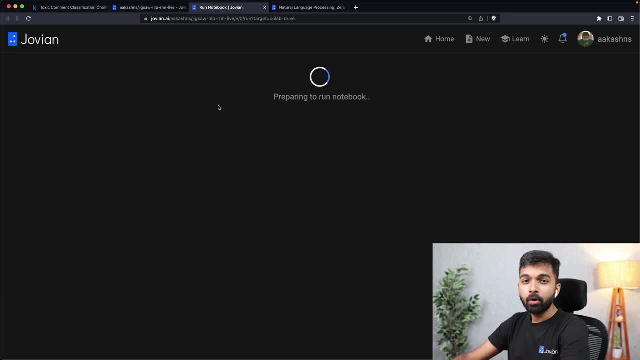 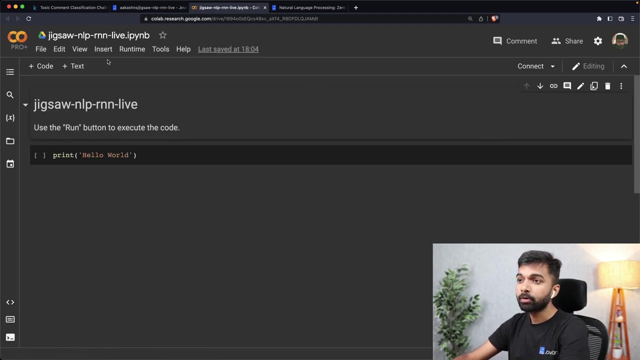 select run on Colab, Because this is a large data set containing hundreds of thousands of rows of data, And we will be training a fairly large model as well, So it's going to be useful for us to use a cloud online Jupyter notebook like Google Colab. So the notebook that we had created here on Jovian 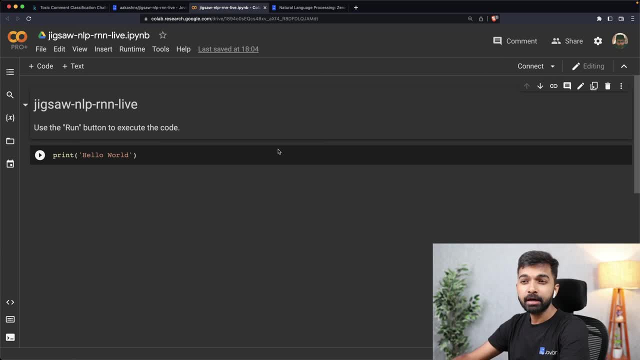 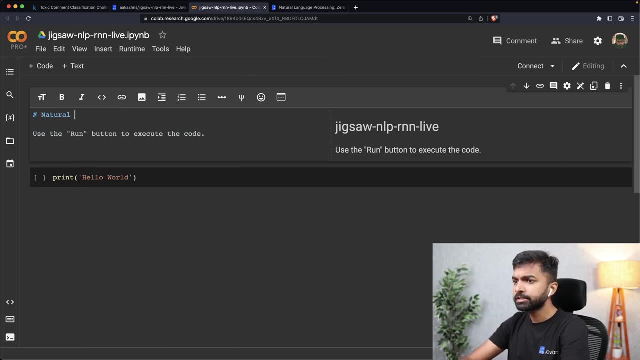 is now running on Google Colab And you might have to connect your Google Drive account in order to be able to run this notebook. And let's just give this a nice title, Let's say natural language processing, Toxic comment classification, And I'm just going to say with RNNs or recurrent neural networks. 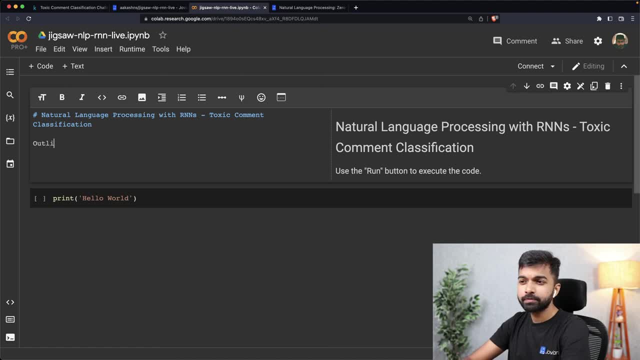 And I'm going to also create an outline here. It's always useful to create an outline for any project that you're working on. So the first thing we'll do is download and explore the data, And the second thing we're going to do is 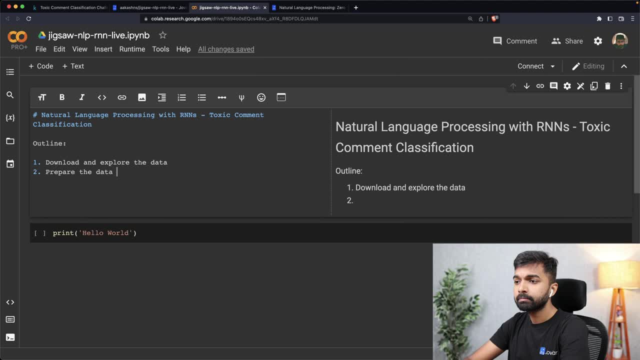 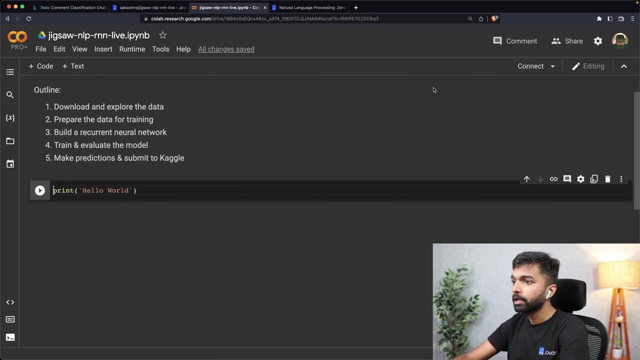 prepare the data for training. Next we will build a recurrent neural network, Then we will train and evaluate the model And finally we will make submissions. Or finally we will make predictions and submit to Kaggle. So that's the outline for what we're going to do today. 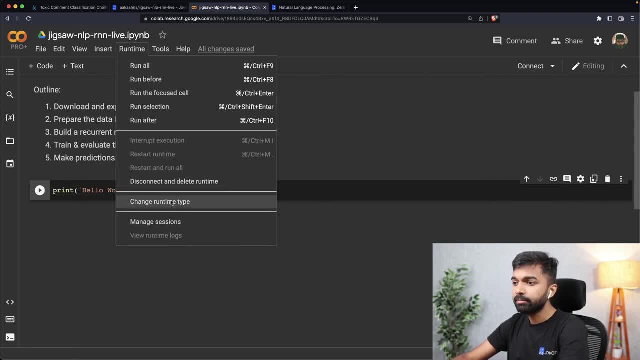 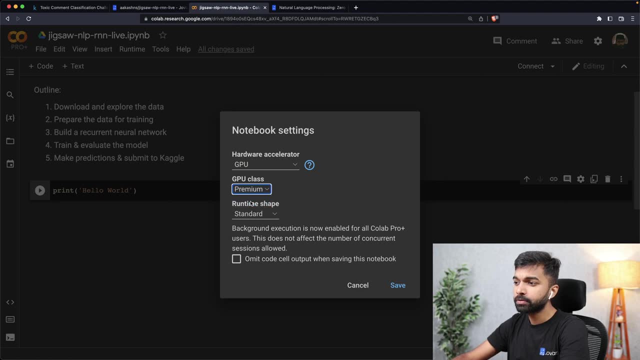 And one thing I'm going to do is just change the runtime here, So I'm going to click runtime- changed runtime type. Now, in my case, I have Colab Pro plus and that allows me to use a premium GPU and high RAM And that's justooooooooo nice. So it's that simple, So you don't have to. 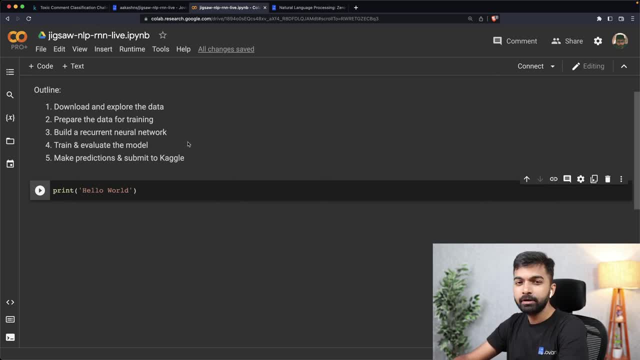 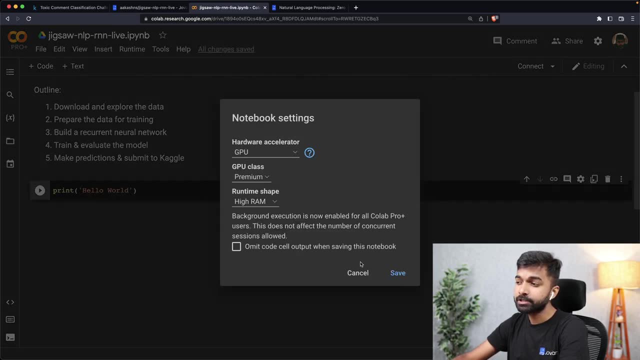 And that's just going to make things a little faster. But even even if you don't have these, you can always still work with Colab. but you still might want to change the runtime type and select the hardware accelerators GPU, because today we will be using a GPU for training. 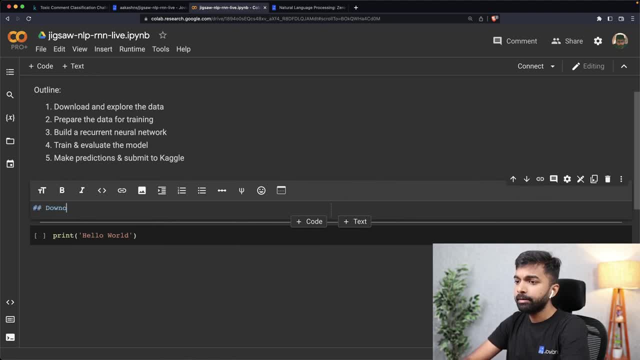 Okay, Now that we've created an outline, let me create a section called download and explore data And within this section, we will first download the data from Kaggle, Then we will load it using loaded into pandas data frame And finally we will explore the data set. 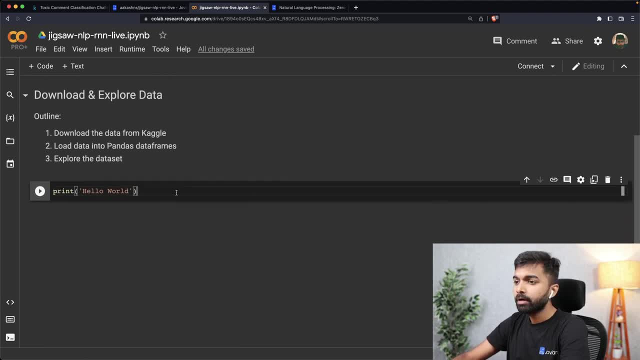 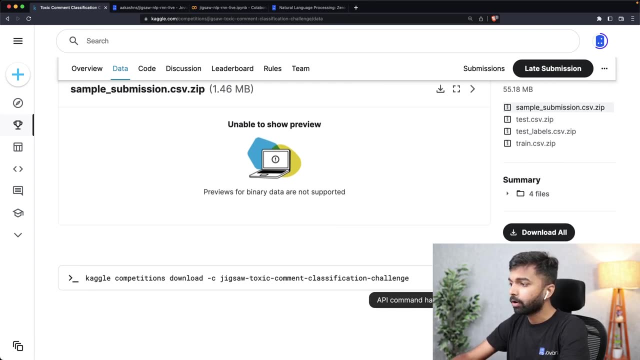 So just by doing a few visualizations now to download data from Kaggle, I can head back into the competition page and all the competition page. I can simply copy this API command. So I have this command and I'm going to come back here. 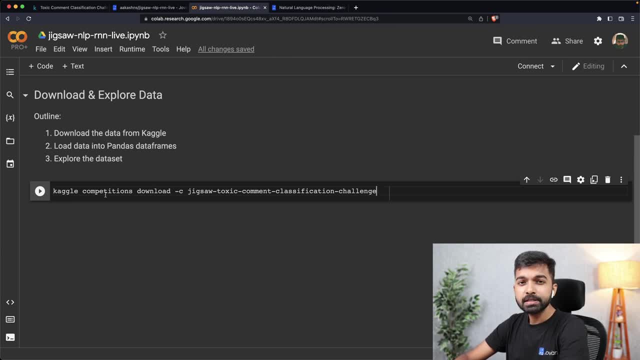 Back and run this command. but this is not Python code, This is a shell command. So that's why we have to insert this exclamation mark, this exclamation point, before the command, and now we can run it. but when we try to run it, 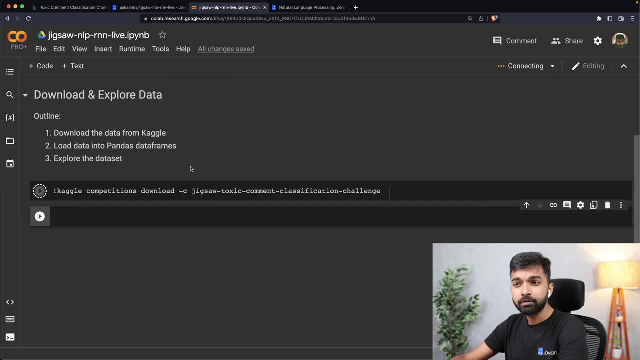 this is going to say that we don't have a Kagglejson file, so it needs credentials. It needs our credentials, our Kaggle credentials, to download this dataset from the Kaggle competition. So that's where let's. let's wait for this to run. 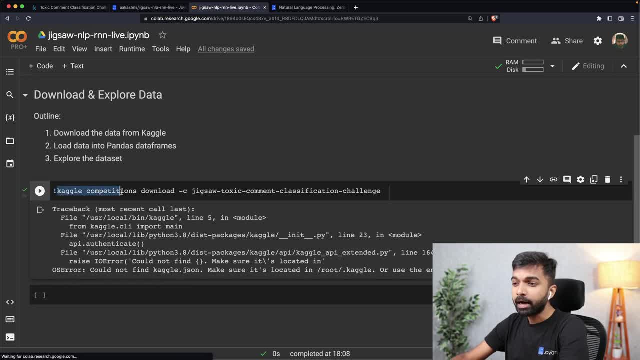 Yep. So you can see here that the comp, that the command, could not run successfully because it is looking for your Kagglejson file. It is looking for your Kaggle credentials, And the way you find your Kaggle credentials is by going to Kagglecom. slash me, slash account. 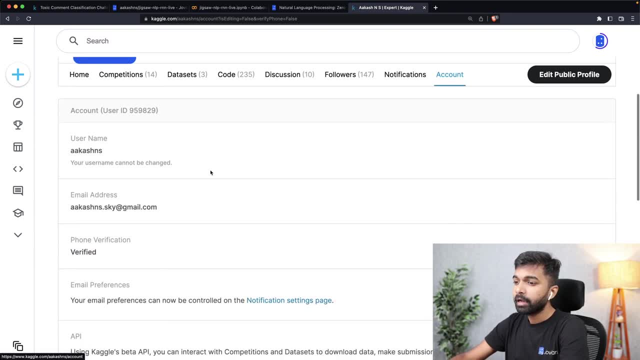 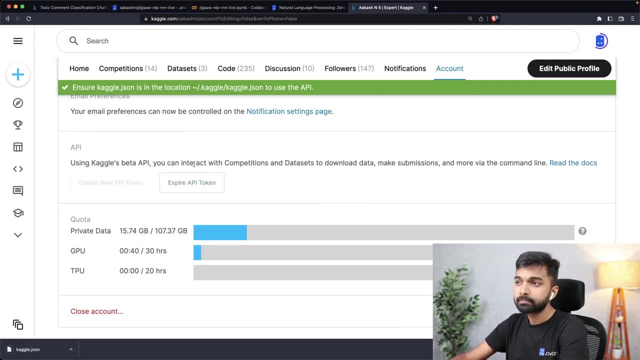 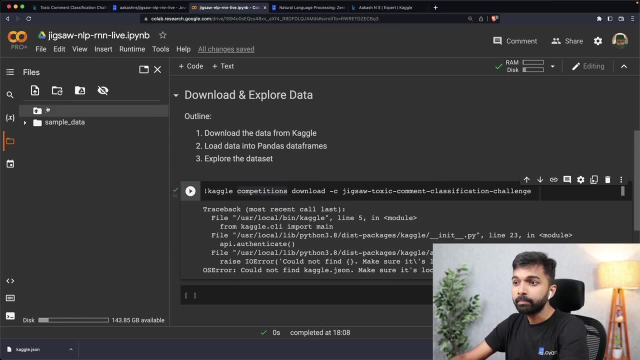 Or just go to Kaggle and open up the account settings, and under accounts you can click create new API token and just download this Kagglejson file that has been generated for you. Now you need to add it in Colab because we are running our notebook on the cloud. 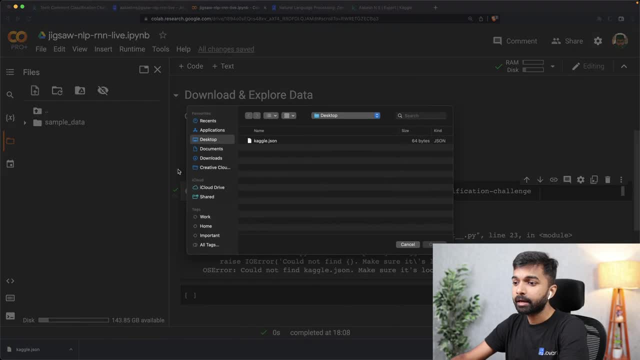 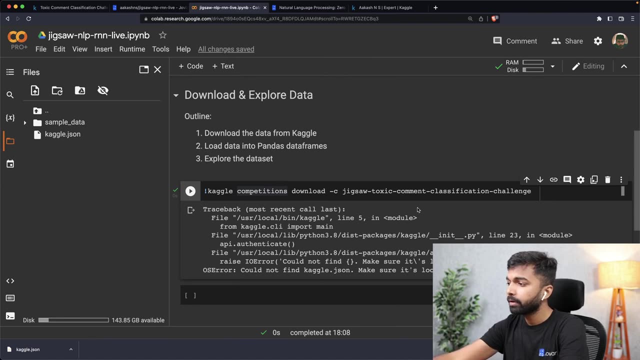 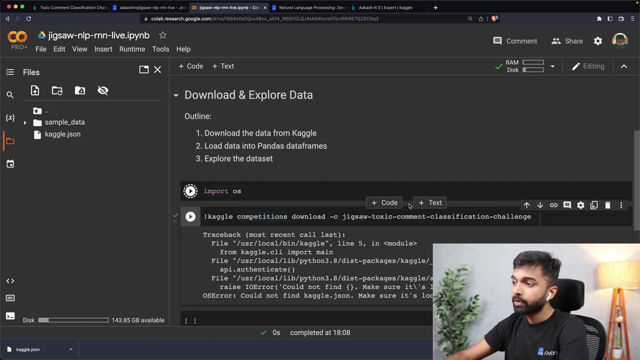 So we can open the files tab here from the sidebar and then click the upload button and select the Kagglejson file. And once the Kagglejson file is uploaded we can now use that Kagglejson file. But to use it we will have to inform the Kaggle CLI. 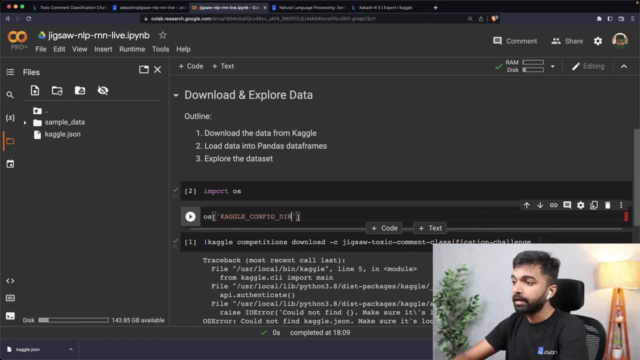 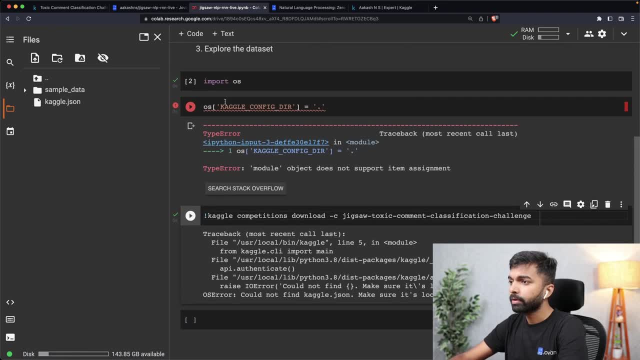 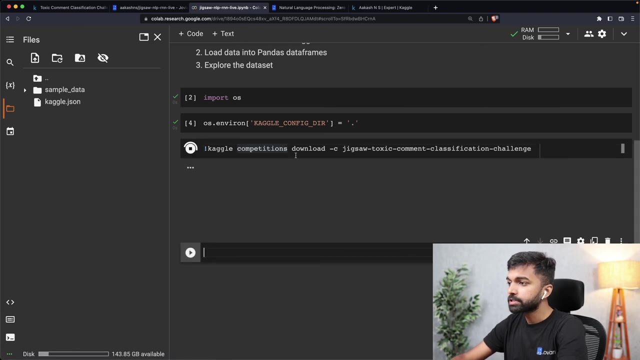 And I'm going to set it to the current directory. Okay, so we have to set an environment variable and we can set an environment variable using OS dot in we're on and here we set Kaggle config- DIR two dot. Now, when we run Kaggle competitions, download. this is going to download the data. 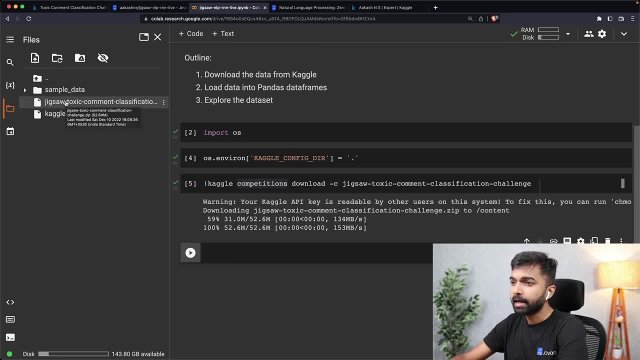 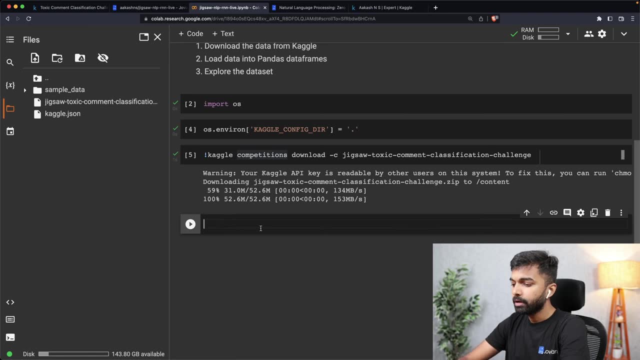 So now we have the zip file jigsaw-toxic-comment-classificationzip. This contains all the data for this competition. Now we can unzip the zip file using the unzip command. So I'm simply going to say: unzip jigsaw-toxic-comment-classification-challengezip and I'm going to unzip into a folder called data. 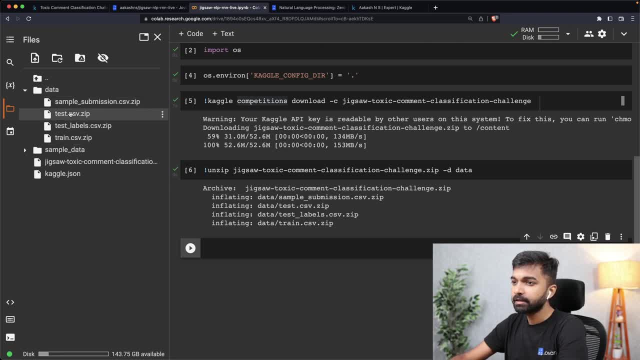 And now we have this folder called data. Inside it we have the test train and sample submission CSV files. So now let's load up this data using pandas. So I'm going to first import pandas as pd And then I'm going to create a data frame called rawdf, because the traincsv file contains: 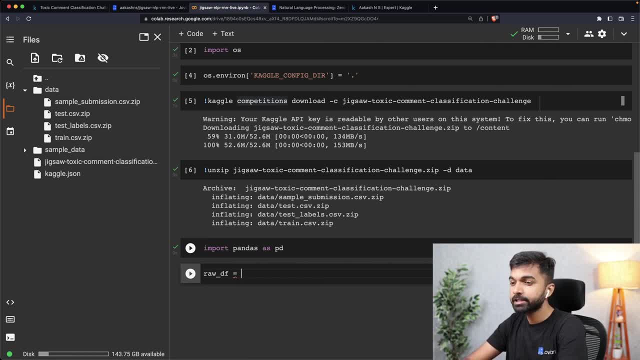 raw data which we'll have to process and then create a training and validation set out of it. So rawdf is pdreadcsv- data slash- traincsvzip, And similarly we have testdf is pdreadcsv- data slash- testcsvzip. 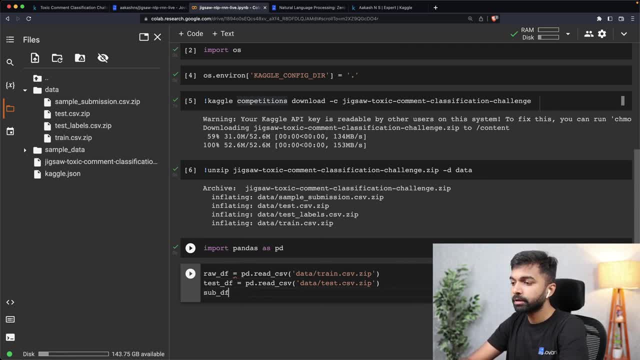 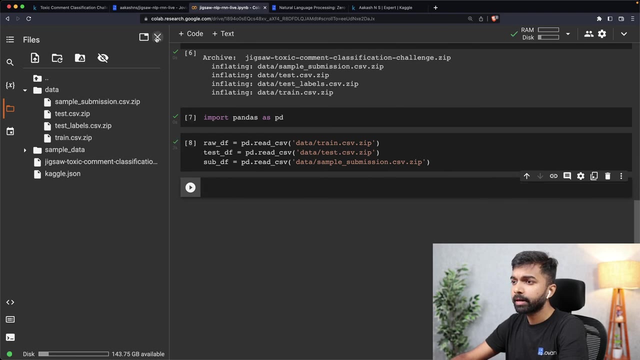 And then we have the sample submission file, which we will use later, So I'm just going to import that as well: pdreadcsv- data slash- sample submissioncsvzip. All right, So now we have read this data and now we can close this sidebar. 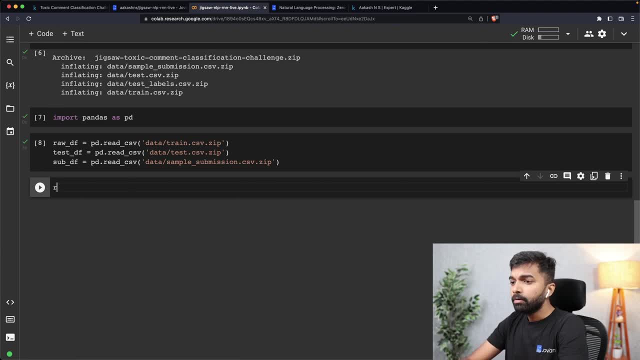 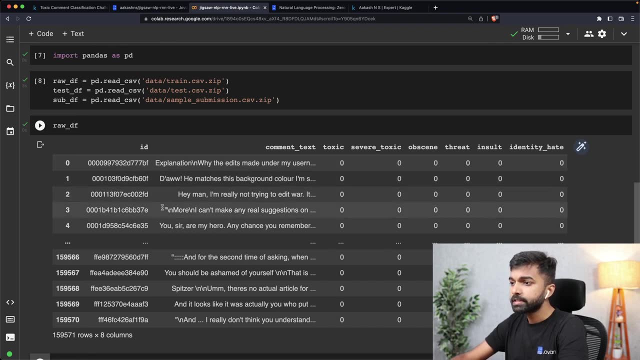 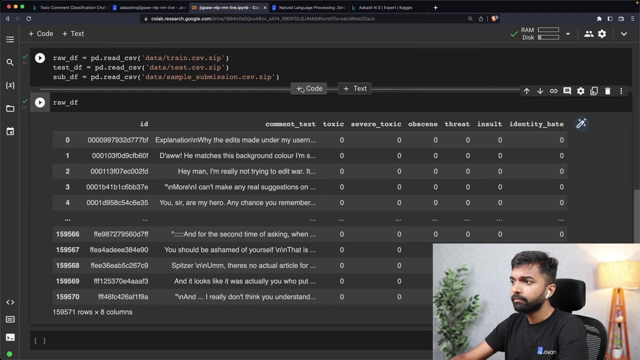 Okay, So we have the data already. Now let's take a look at what the actual data set looks like. Okay, So here you go. This is the raw data frame and looks like it has 159,571 rows. In fact, we can just do rawdfinfo to print this information. 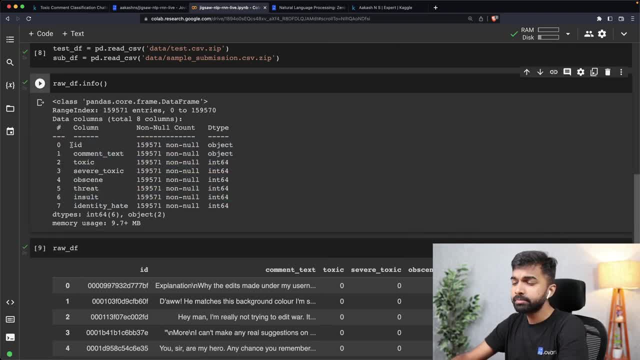 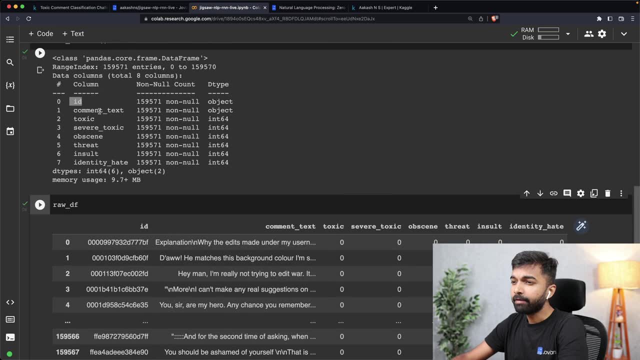 So it contains these seven or these eight columns. The first one is ID, which is simply a numeric Oh, which is: This is simply a unique ID for each row. Then we have the comment text. So this is an example of a common text. 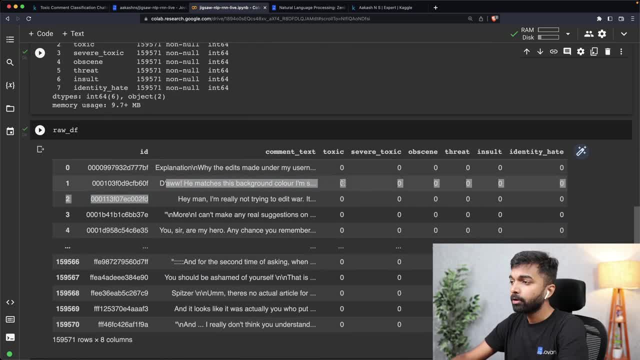 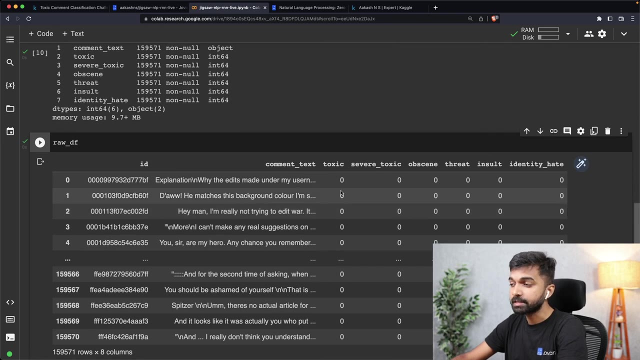 This is another common text and so on, And then we have information about whether the comment belongs to a certain class or not. So there are classes like toxic, severe toxic, obscene, threat, insult and identity hate. So there are a total of six classes and one comment can belong to any number of classes. 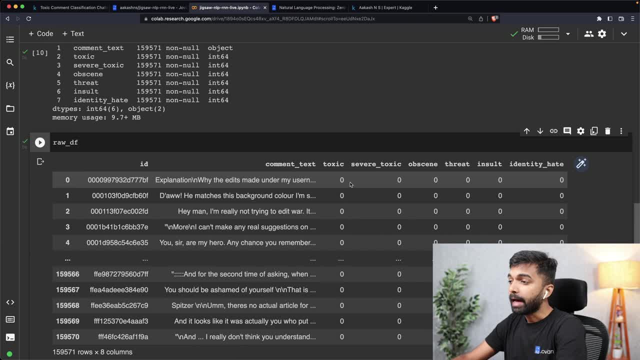 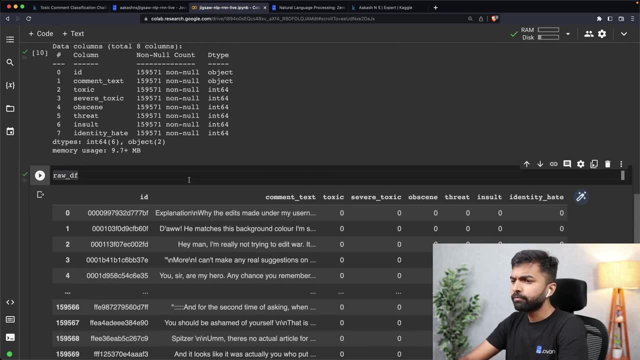 So that's why this is a multi-label classification problem And The zero One comment does not belong to the class One indicates that the column comment does belong to the class. Now let's look at a few samples. Let's maybe call rawdfsample20.. 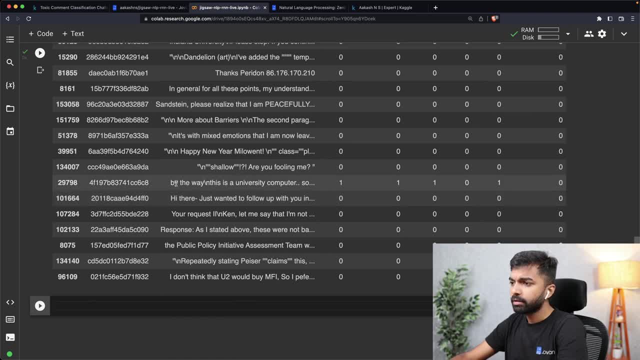 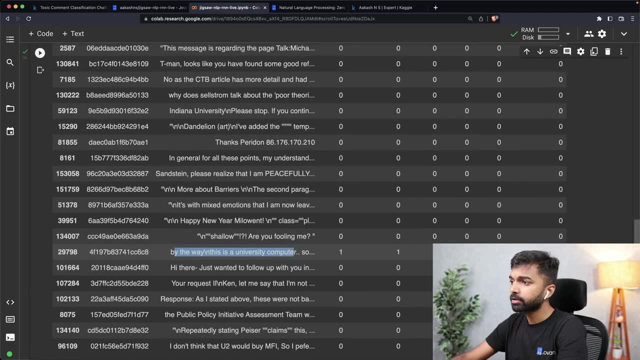 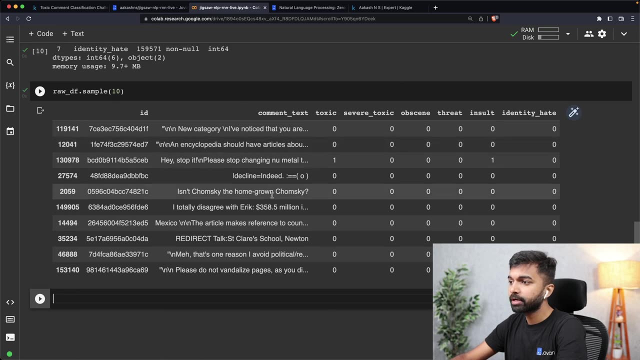 And we can see that it's okay. This one, this one definitely seems like there is probably some abuse or something going on here, because this is toxic, severely toxic, et cetera. Let's look at another sample. So this is always a good idea: looking at some sample data by picking samples from the dataset. 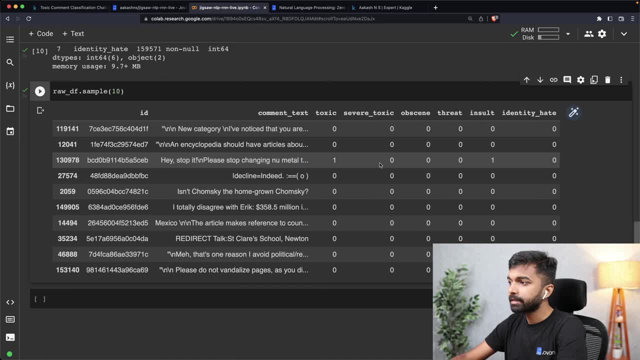 Okay, Once again here. Hey, stop it. Please stop changing new metal, et cetera. So here again there seems to be some toxicity, some insult. I'm not going to play the, I'm not going to show the entire comment, because this might. 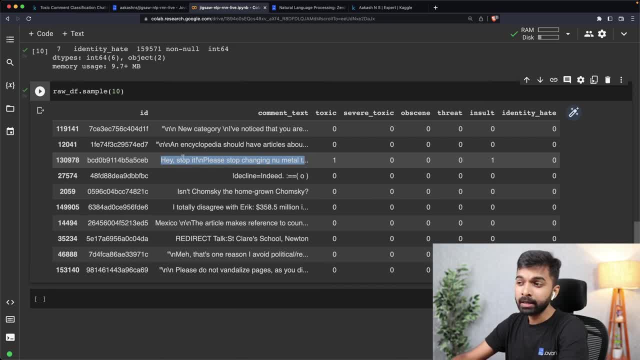 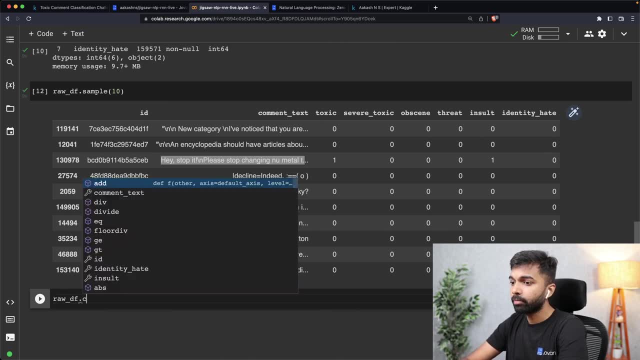 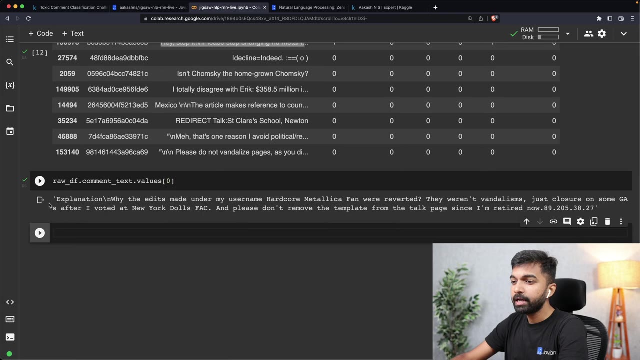 have some derogatory or vulgar language, but you can explore individual comments like this. So I'll show you just an example of a neutral comment. So say, rawdfcommenttextvalues zero. So this is the very first row In the Data frame. 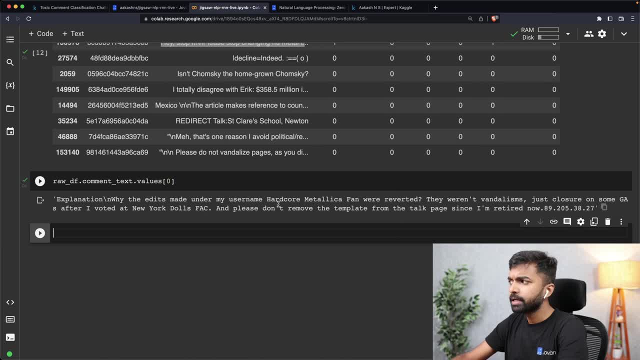 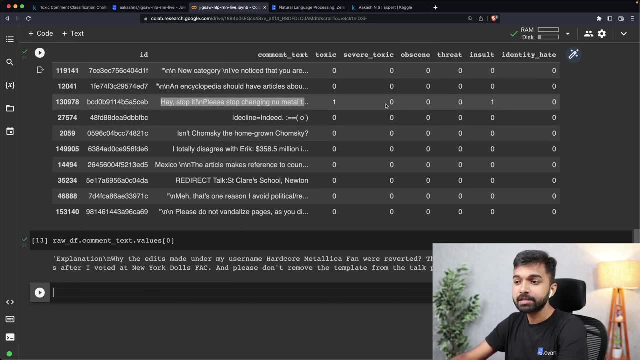 And this is a. this is not a toxic comment. This is a normal comment. This is perfectly fine. Okay, But I encourage you to also maybe check out a few toxic comments, just to understand what each of these classes means. Now, one other thing that we can do is try to understand what percentage of comments. 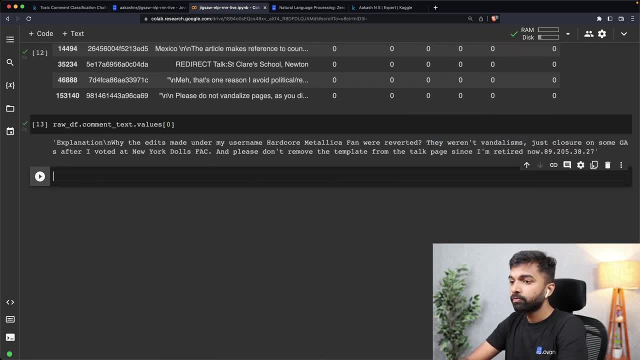 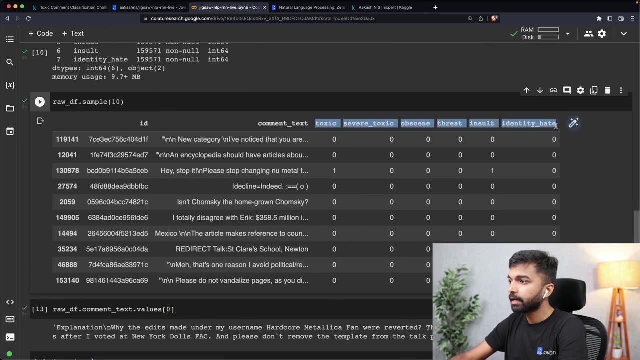 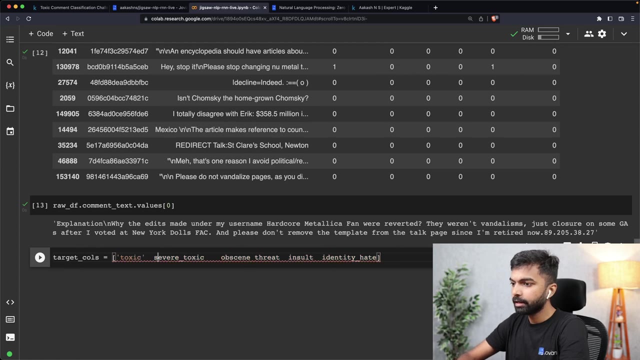 fall into each of these categories individually. So first I'm going to create a list of target columns. So these are the target columns: toxic, severe toxic, identity hate, et cetera. Okay, So let me just put these into ports and create this list here. 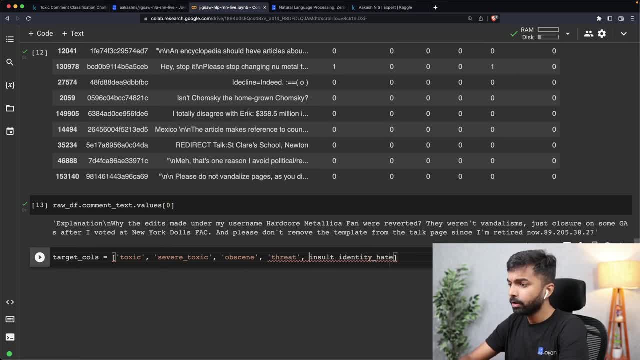 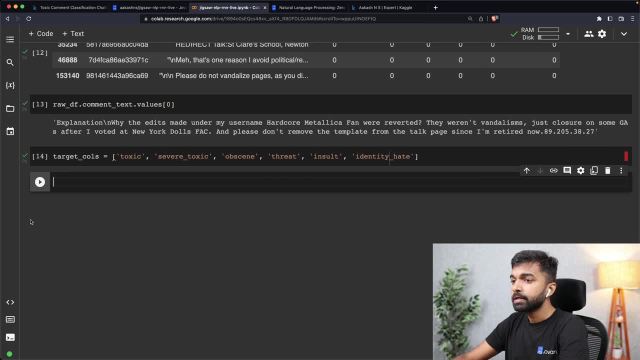 And, by the way, feel free to pause and follow along. It's always a good idea to type out all this code yourself. That's why I'm doing it as well. It's a great way to learn, great way to experiment, Okay. 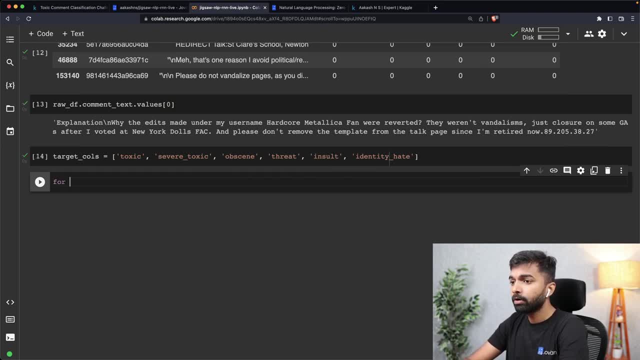 So these are all the target columns. And now let's do this for call in. Okay, Target calls. Let's print: First, let's get the from the raw DF, Let's get this particular column. So for each class let's get the data and then let's call: value counts on it. 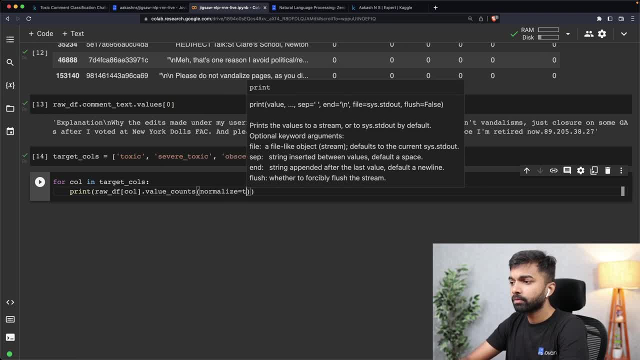 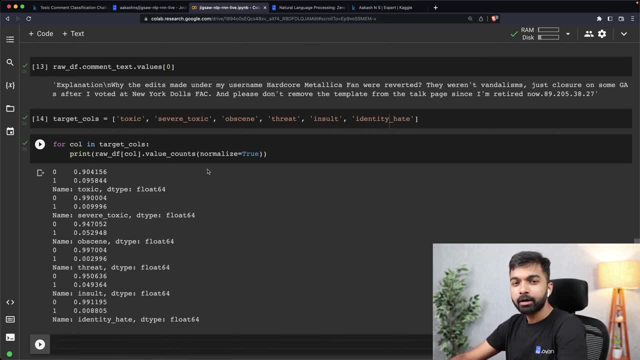 And then, after getting the value counts, let's just print it out. Okay, Now I'm using some pandas methods here which you can learn about, But in one of our free courses, a data analysis with Python, zero to pandas, or you can also. 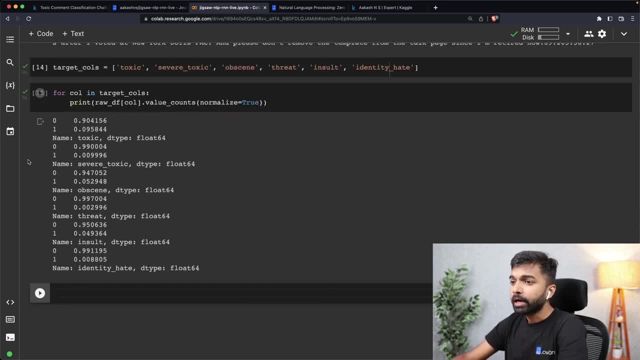 it's also something that we covered in our data science bootcamp. All right, So in the law in the case, toxic: about 90% of the comments are not toxic and about 9.5% are toxic, severely toxic. well, about 99% of comments are not severely toxic. 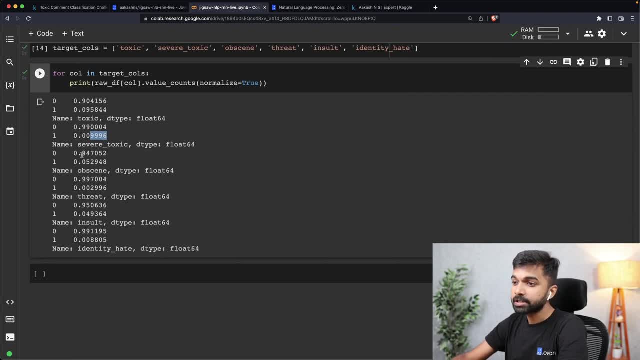 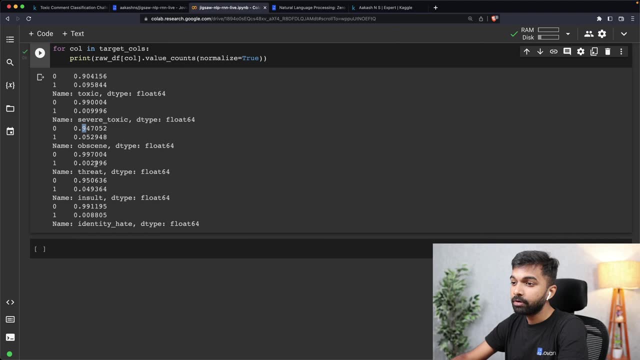 And only about 1% of comments are severely toxic. About 94% are not obscene. about 5.2% are obscene. Okay, So 99.7% are not threatful. only about zero point. only about 0.2% are threatful. 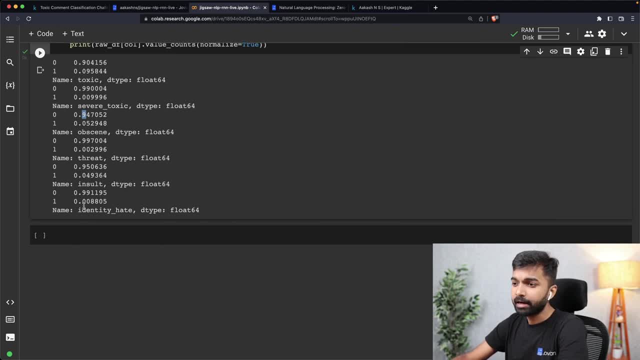 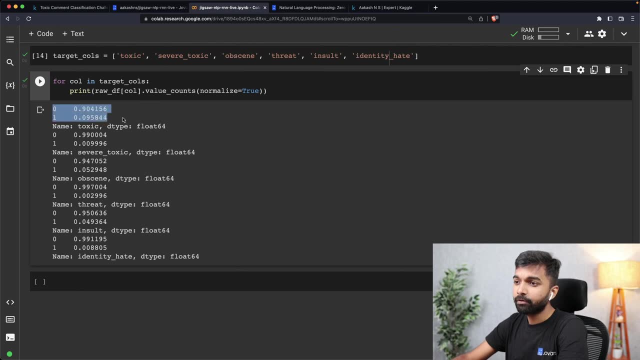 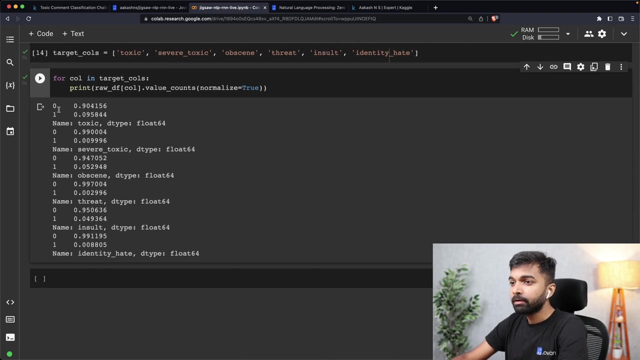 And then we have the insert. about 5% have an insert and there is about a 0.88% of identity hate. Okay, So this is the distribution for each of these and remember, each of these can be applied independently. Okay, So now we have a good understanding. 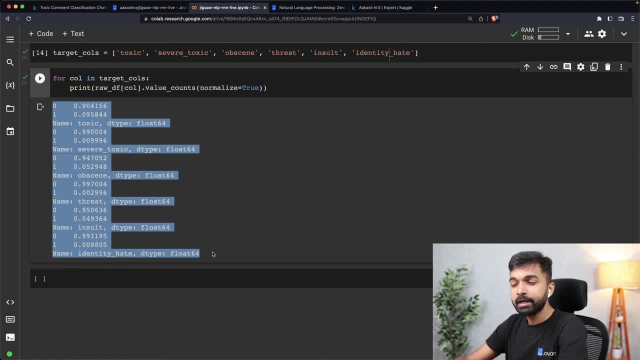 And one thing we know is that a very few, a very small percentage of ones are present Okay In the target columns, And that's why accuracy may not be the best metric in this case. In fact, if you go into the competition again and check the evaluation, they use something. 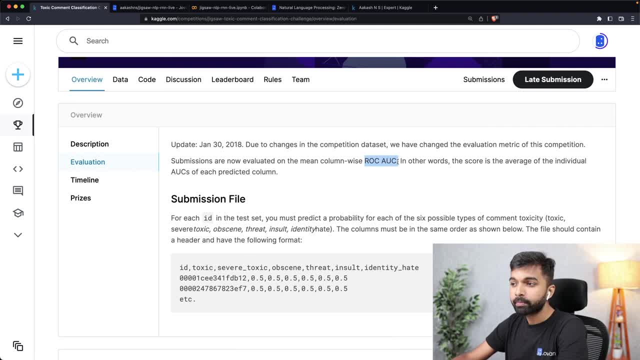 called an ROC AUC score. All right, And that is the score that you will see on the leaderboard, So I encourage you to read about the ROC AUC score. You can find a bunch of great tutorials, specifically videos, on YouTube. Okay, 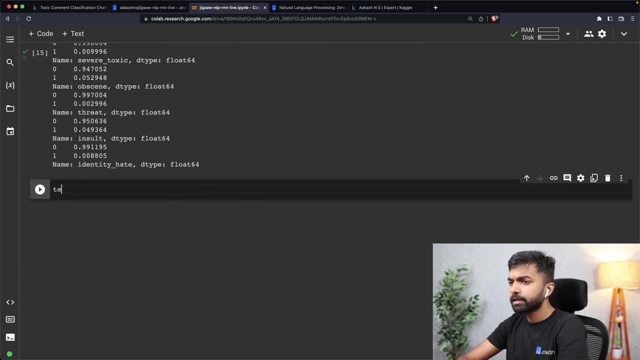 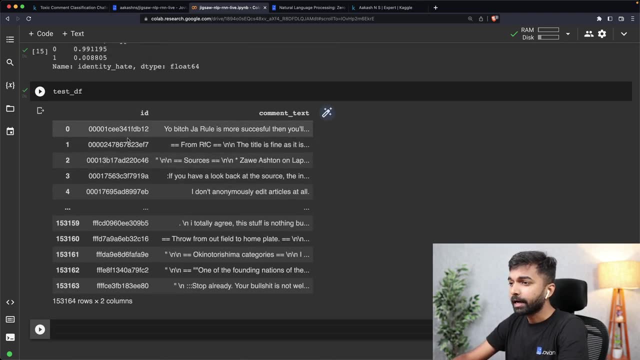 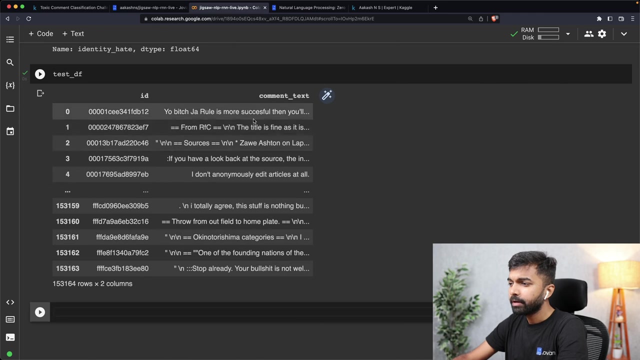 So that's the training data. It had about 159,000 records. Let's check the test data frame Now. the test data frame contains an ID, and then the test data frame also contains some common text, And you can see here that there's definitely some derogatory words being used here. 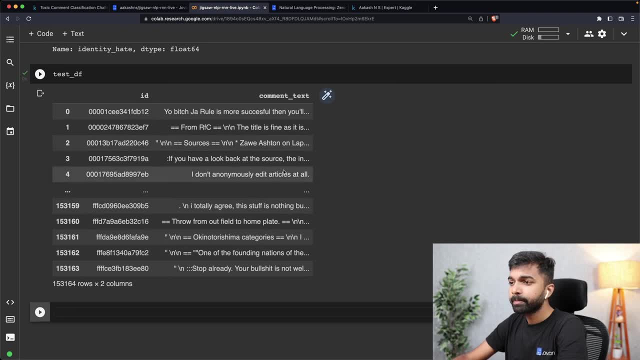 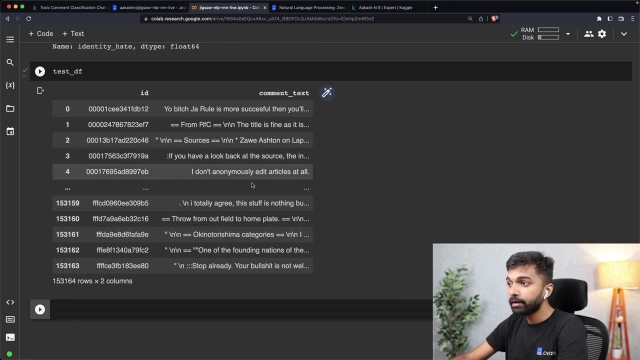 So there's definitely some level of toxicity in some of these at least. now, the text in the test data frame does not actually contain any labels, And what you have to do is you have to look at the, you have to train a model. 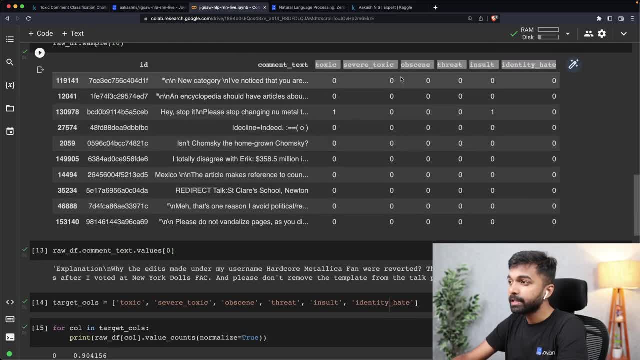 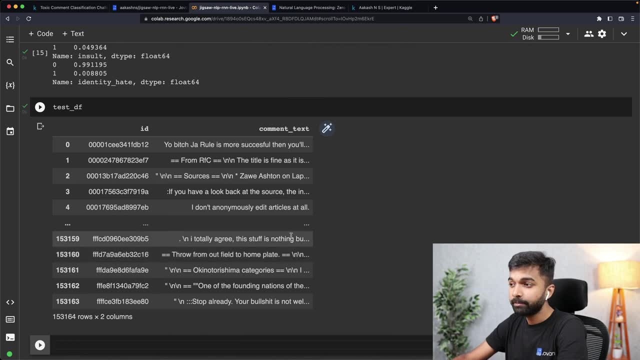 Using the training data set. So look at these comments, look at their labels, train a model and then make predictions for each of the rows in the test data frame. And what do you have to predict? You have to predict the probability that this common text belongs to each of the classes. 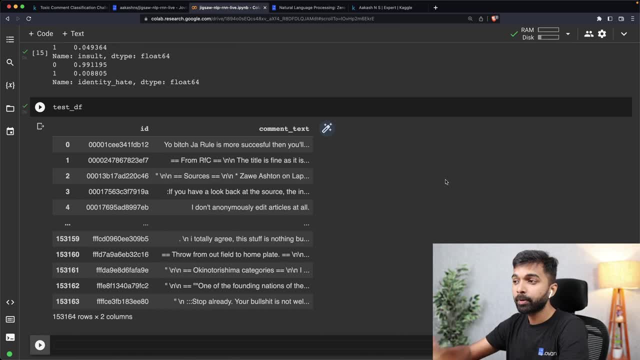 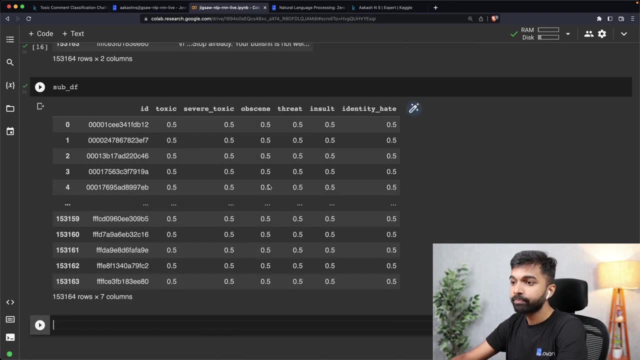 independently. All right. So for each class you have to predict a probability between zero to one for each common text, And then you have to put those into a submission file, And this is what your submission file should look like. It should contain the ID: 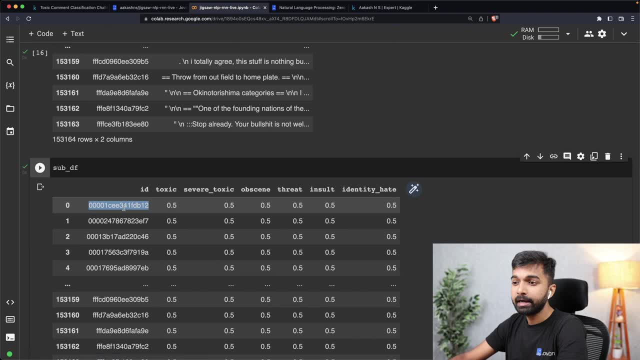 And you can see here that the ID here matches the ID here, So the IDs correspond to the IDs of rows in the test data frame in the exact same order. And then you have to make predictions here, for example: toxic, severe, toxic, obscene. 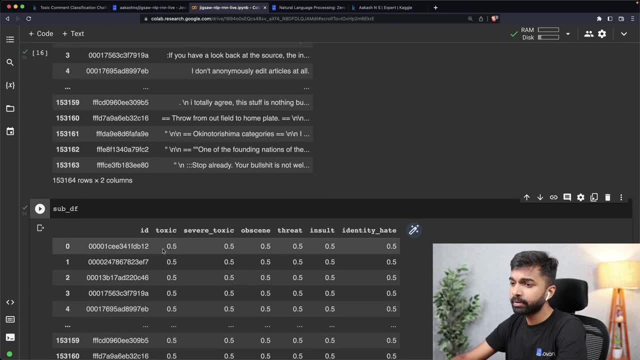 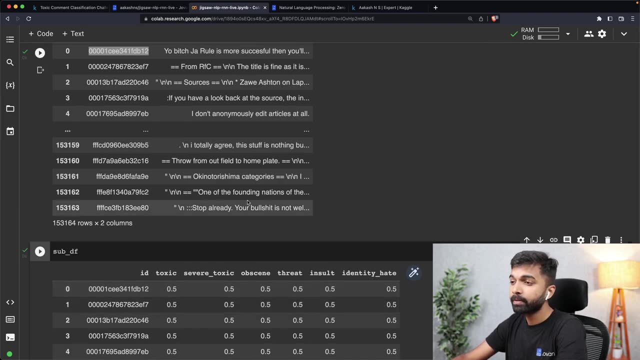 threat, insult, identity, hate, et cetera. Now here, the sample submission file just contains 0.5 everywhere, but you have to make a probability prediction, something between zero and one for each of these, And then you can submit that file. 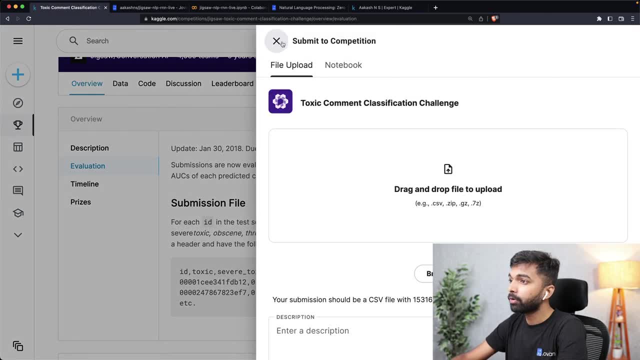 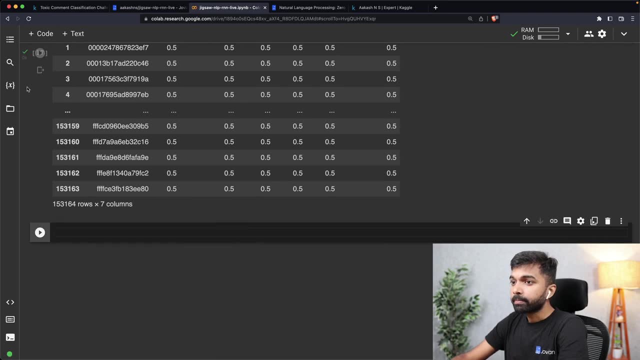 So you can go in here and you can click late submission And you can actually upload it. You can upload your submission file and see your score on the leaderboard. So that is what we are going to do. Okay, So with that, we have completed the first step, which is to download and explore the. 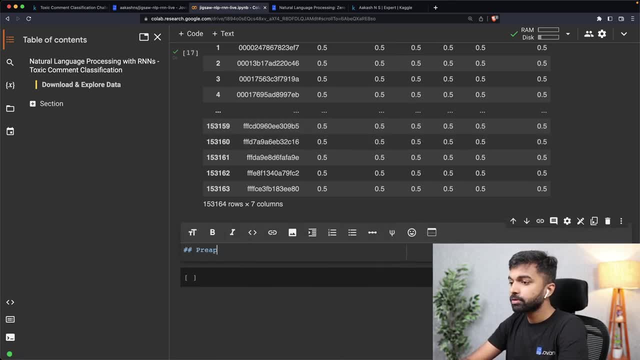 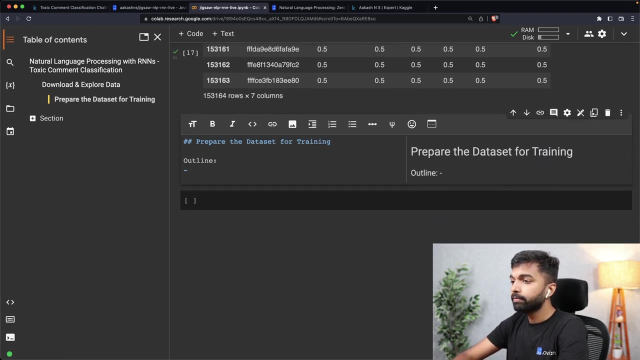 data. The second step is to prepare the data for training. So what are we going to do here? Well, let's write out an outline. Once again. the first thing we will do is Create a vocabulary using torch text, then create training and validation sets. 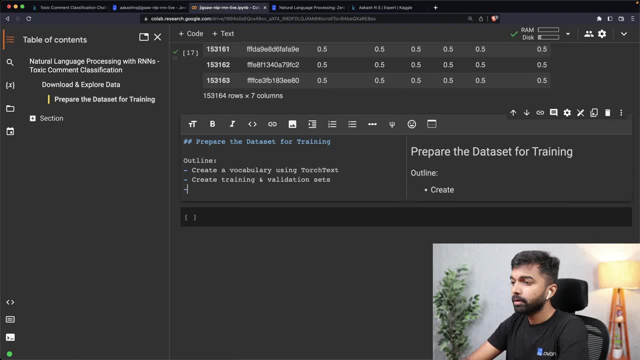 And then finally create PyTorch data loaders. Okay, So so far we have. if you've, if you've attended some of the previous sessions, you can see that we have a lot of training and validation sets. Okay, So so far we have. 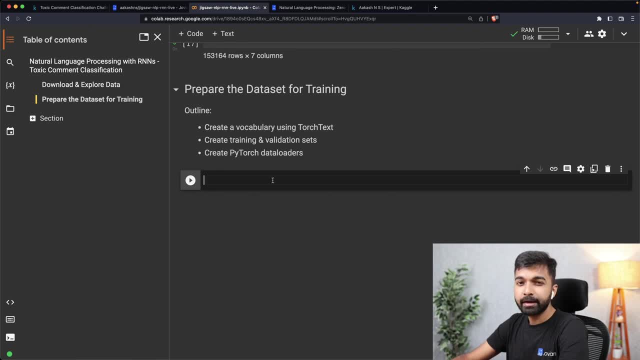 If you've, If you've attended some of the previous lessons here, we've used libraries like NLTK and scikit-learn to create our vocabulary and our vectors, But now we're going to use torch text, which is a library, a companion library for PyTorch. 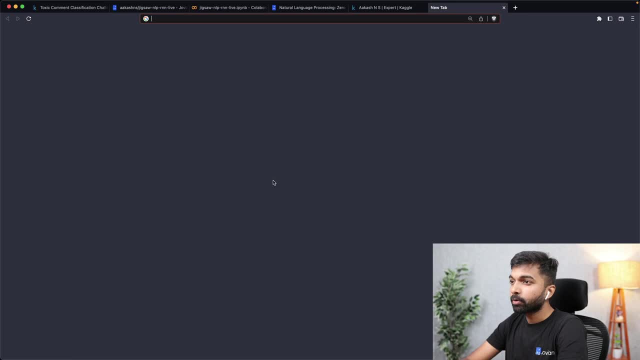 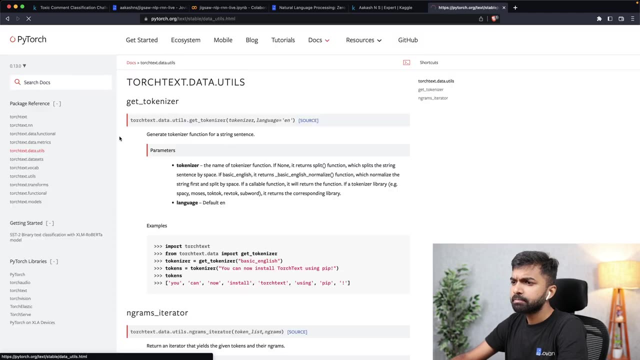 So let's see. So the first thing we look for in torch text is a tokenizer. So I'm going to search torch text tokenizer And it looks like there is this module called torch text or datautils, And from here you have this function: get tokenizer. 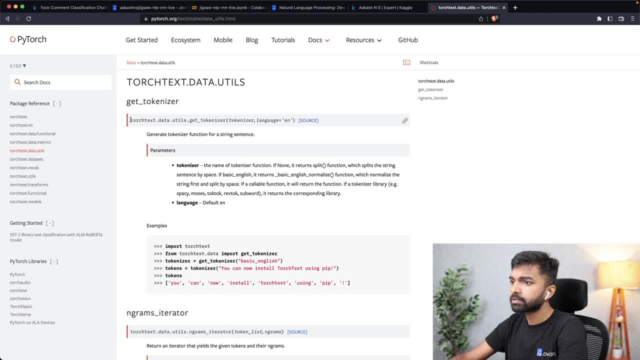 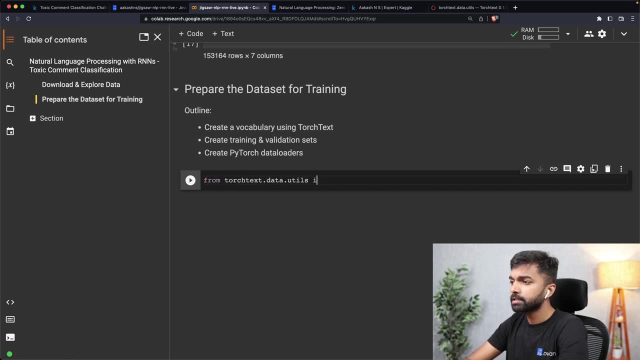 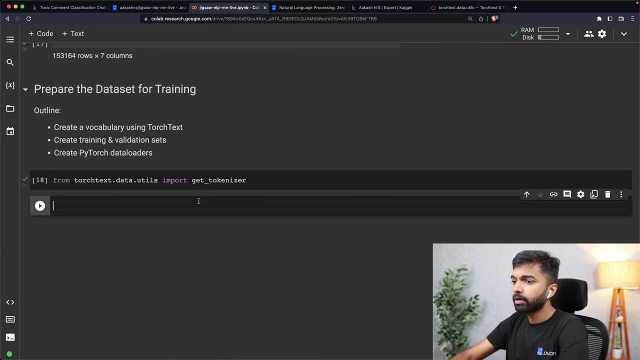 Okay, So I'm going to first just import this torch text or datautils. Let's see from torch text or datautils, import get tokenizer And I encourage you to check out the documentation of get tokenizer. But the way this works is you can create a tokenizer, which tokenizer is simply something. 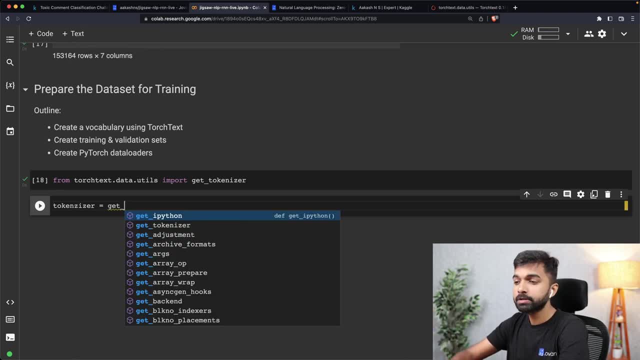 that splits a given text into its individual tokens or individual words. So let's call it get tokenizer here, And we need to give it a language. I'm just going to give it the language- Basic English. And now let's look at an example comment. 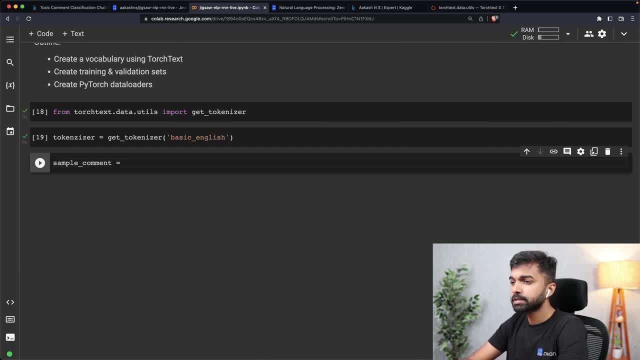 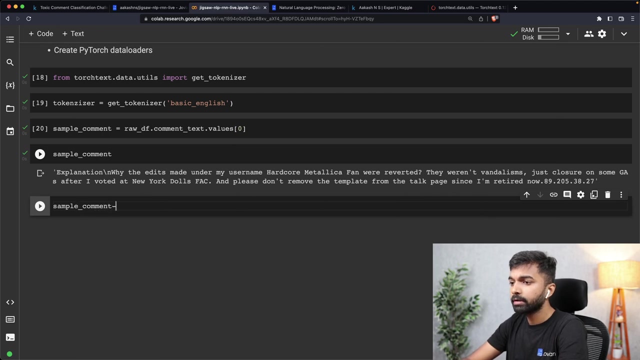 So let's call this sample comment, which is plodifcommenttextvalue. So this is a sample comment. and now let's convert this comment into token. So sample comment: Tokens equals tokenizer, Right tokenizer. Oops, this should be called tokenizer. Yeah, The tokenizer is simply a function. 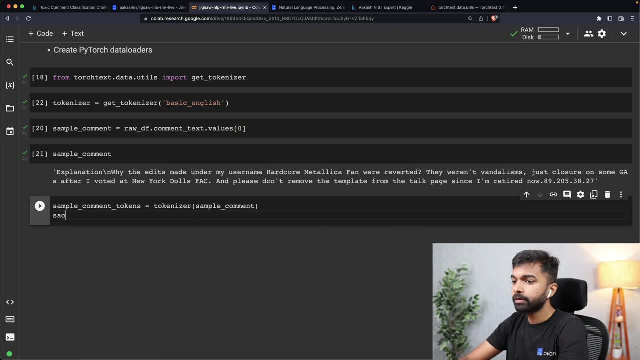 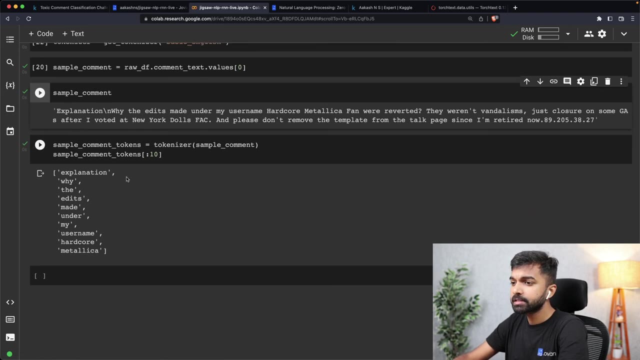 And let's pass into it a sample comment And let's look at maybe just the first 10 tokens. So there you go. So all our tokenizer is doing is taking this single comment and it is splitting it into its individual word components. One thing it's also doing is lower casing everything. 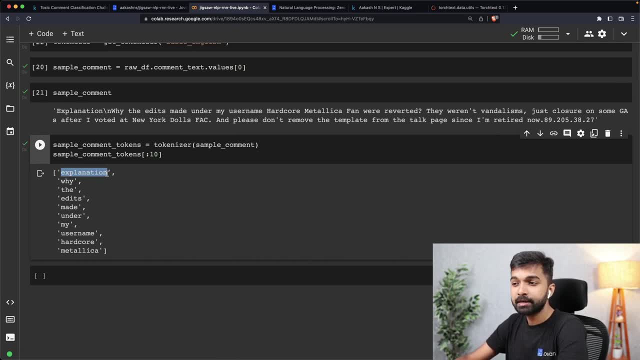 because we are over here at least, we're not interested in the case, Although some models, some more advanced models, even look at case. but you can see that explanation why the edits made under my name, etc. We're just looking at the first 10 tokens, So we simply take. 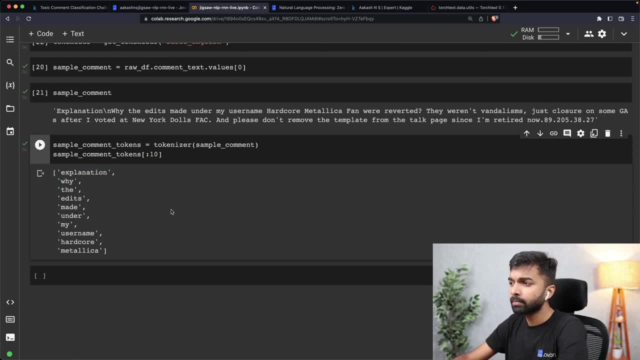 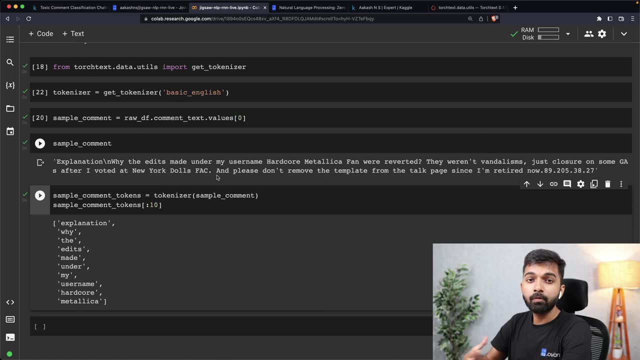 the text and convert it into a list of tokens. All right, great. So now we have been able to create a tokenizer. Now the next thing we will do is we're going to create a tokenizer. So the next thing we will do is we'll actually learn a vocabulary. we will understand what is the full vocabulary. 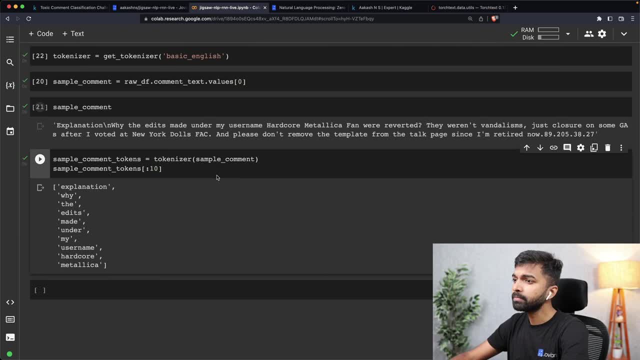 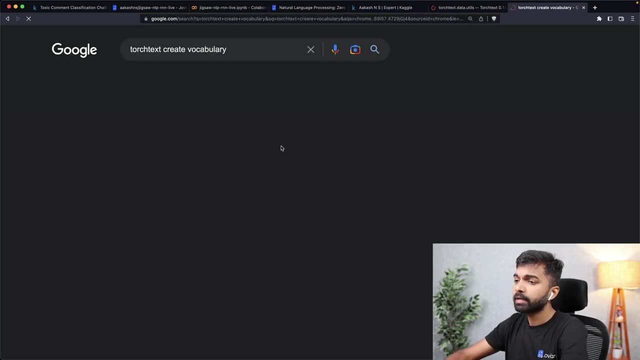 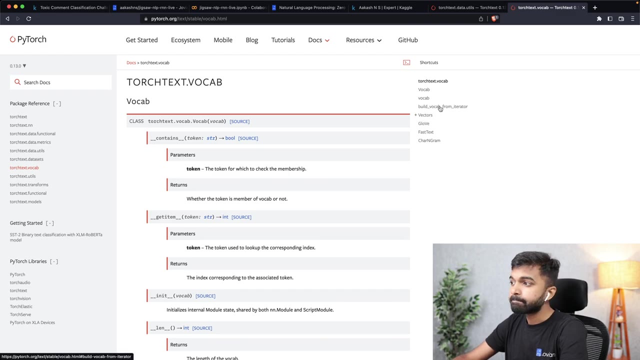 of words that are present within the data set. And let's see how to do that using torch text. The torch text create vocabulary. let's just search that. And this is literally how I do my coding: I look things up And I follow the documentation and experiment around with. 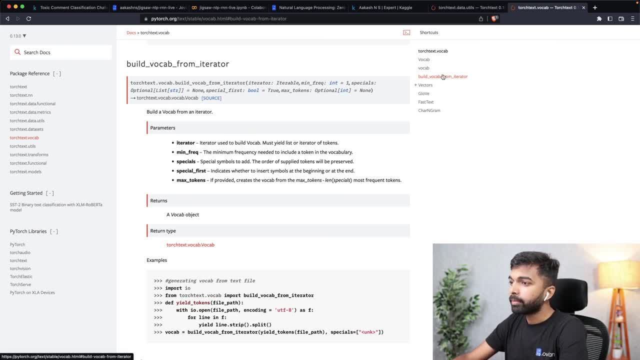 it. So it looks like there is something called build vocab from iterator And I'm going to create a tokenizer, And I'm going to create a tokenizer And I'm going to create a tokenizer. And iterator is simply a list or something that can return items one by one. 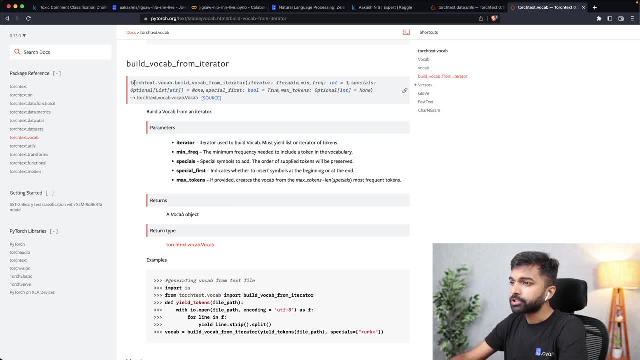 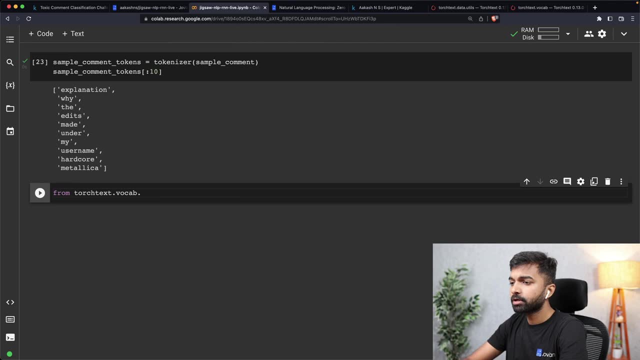 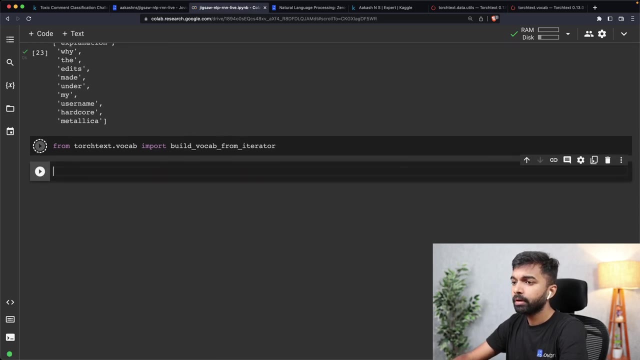 So build vocab from iterator is a function present in torch text or vocab. So I'm just going to import this, I'm just going to say from torched text or vocab: import build vocab from iterator. And now, if you read the documentation carefully here, what this needs is that there's 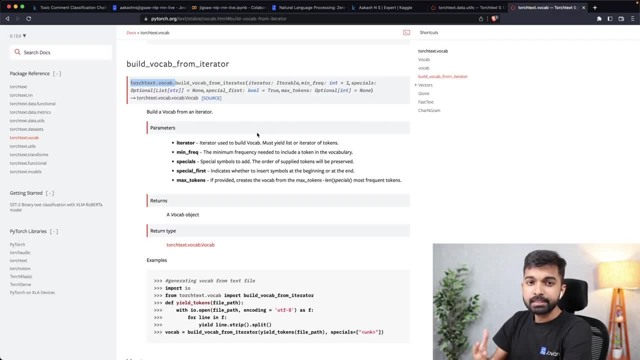 a function called build vocab And I can export it into a work package. So let's create a tokenizer. Okay, let's just create a tokenizer, And once you create a tokenizer, I'm going to import needs. is it needs an iterator? or, conceptually speaking, just a list, and in the list you should. 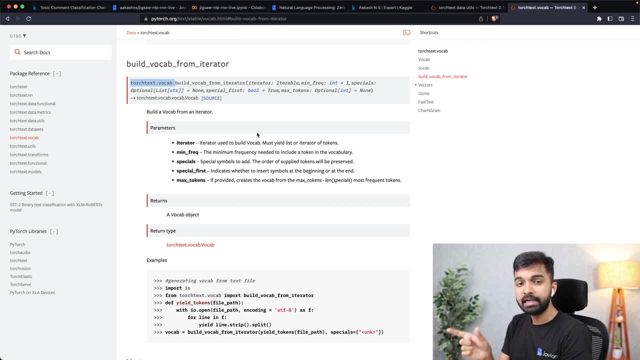 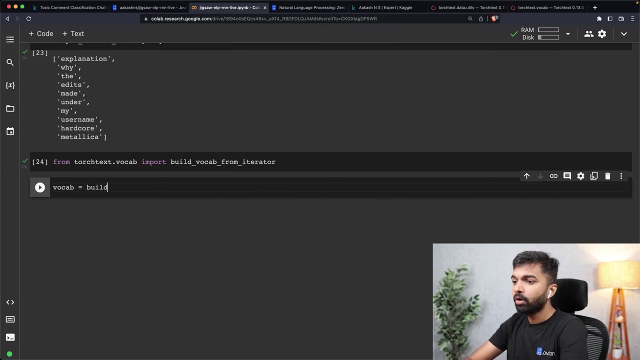 contain. the list should contain sentences in a tokenized form, so you can see here the list the iterator must yield and a list or iterator of tokens, which means that if you want to create a vocab- we call build vocab from iterator, and the first thing it needs is the iterator, which is 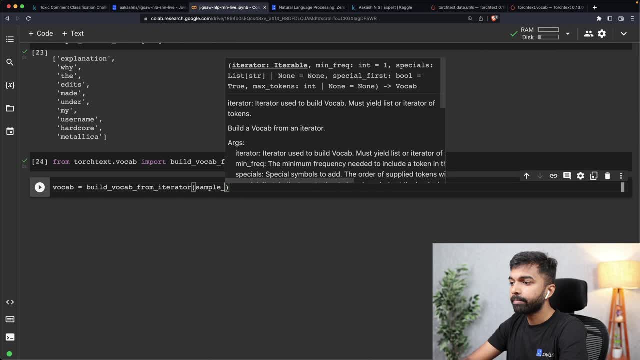 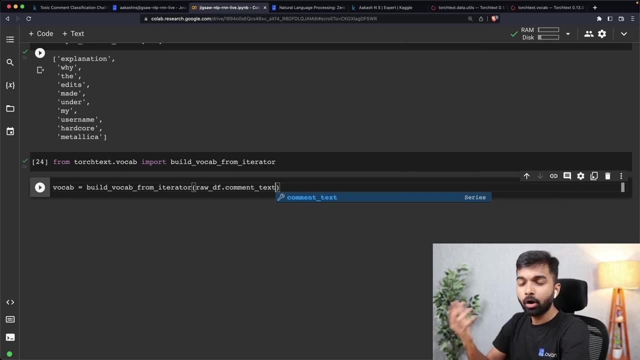 basically the list of comments, so we could do something like this rawdf dot comment text. but the trouble here is comment text and now comment. rawdfcomment text is a list, a series, and it's going to return the comments one by one, but it requires not comments one by one, but it requires 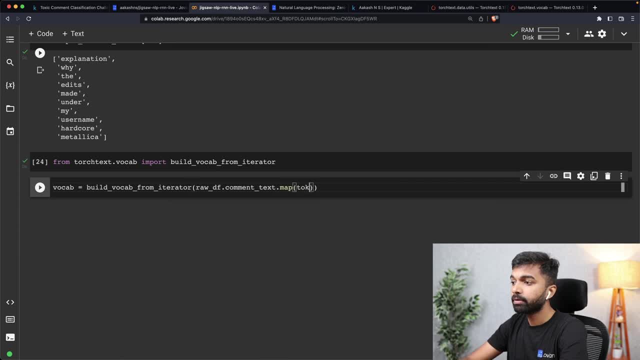 a sets of tokens, one by one, so we can just call dot, map, tokenize or tokenizer. so now what we're saying is for each common text we are applying tokenizer and then we are going to pass that into the vocab iterator. and apart from this, build vocab from iterator takes a few more things. so one thing: it. 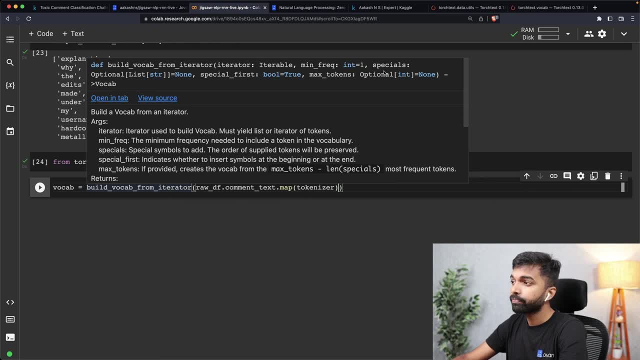 looks for is the minimum frequency, frequency that you want to set, and you can also specify a bunch of special characters. so I'll talk about special characters in a bit. you can also specify a number of maximum tokens, the maximum vocabulary size, and it's only going to pick, let's say, set the 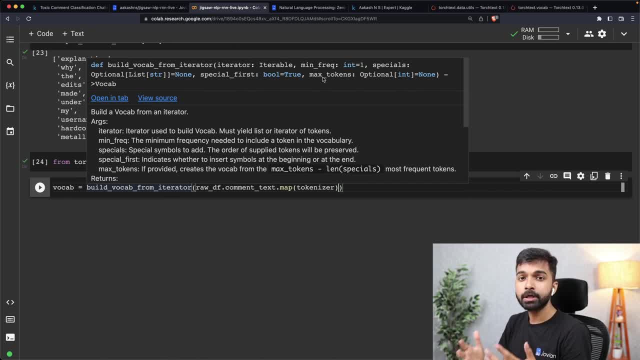 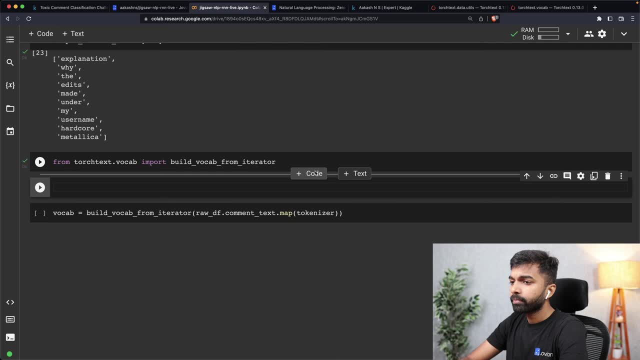 vocabulary size to a minimum character. you can specify to say specar jogar ords. you can also user a thousand. it's only going to pick the thousand most common words, So I'm going to use max tokens. Let's just create a variable called vocab size and let's maybe 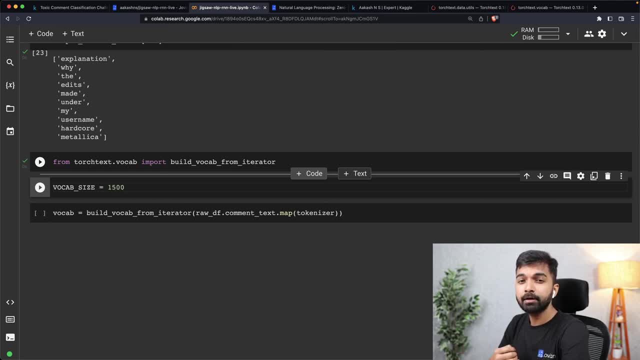 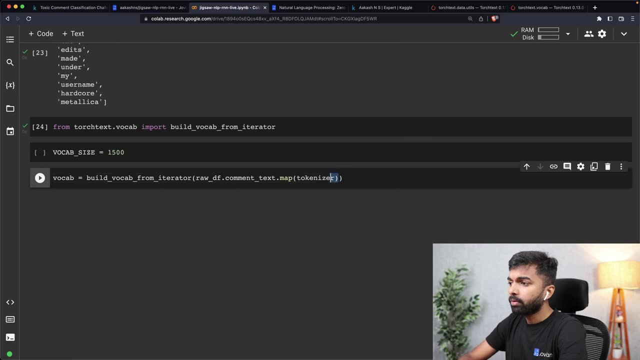 pick a vocabulary size of 1500. So we will only consider the 1500 most common words. Okay, So now we have- let's put this on a separate line as well. So common tokens is simply rawdfcommenttxtmap- tokenizer, which. 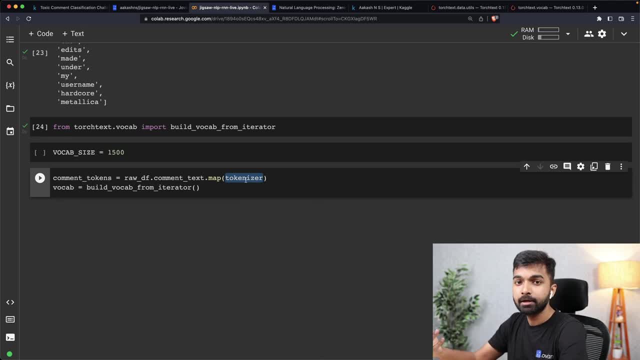 means we have taken each common text and converted it, converted it into a list of tokens. So now we have common tokens and maybe we can just run it above here as well. And apart from this, I am going to also include a couple of special items in the. 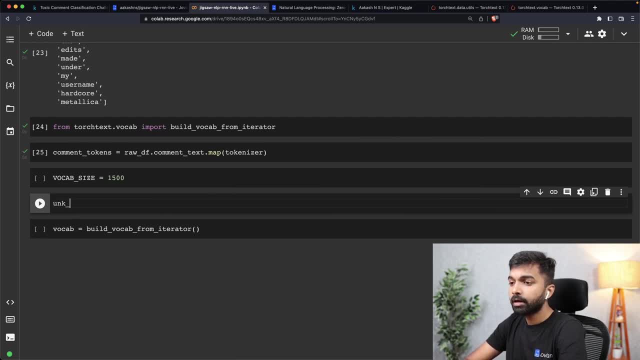 vocabulary, a couple of special tokens. So one is going to be the UNK token- UNC token, Which is going to simply be UNK. this token will be used to represent words that are not present in the vocabulary. And then one is going to be something called a pad token. 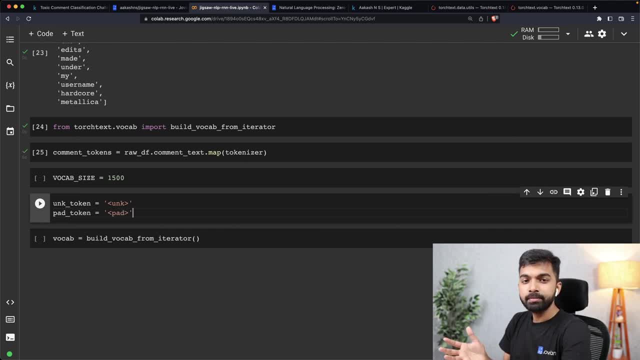 And we'll see how these are used in some time. Now, sometimes some sentences might be too short, Some sentences might be too long for recurrent neural networks. We require all of our input sequences or input sentences to be the same length. So we are going to pad the shorter sentences and we are going to clip the longer. 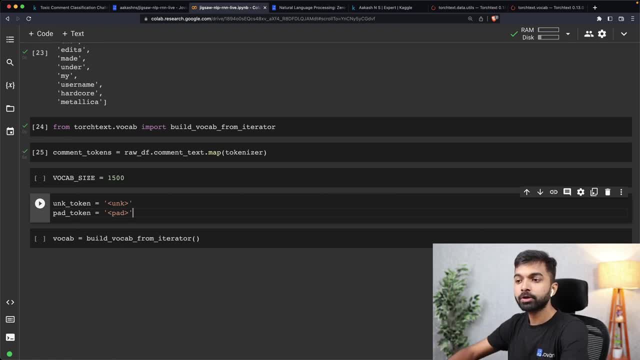 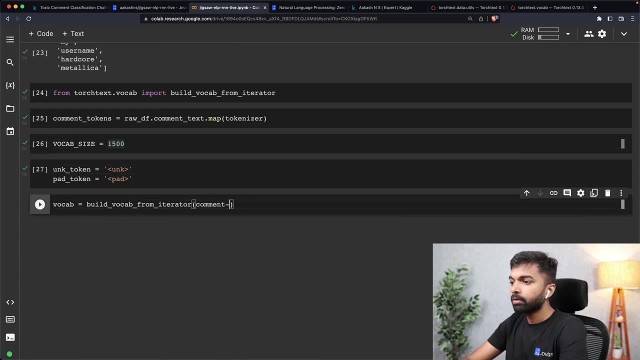 sentences, And that's what this pad token is for. Whenever we have shorter sentences, we're going to add this pad token. Okay, So now we have common tokens. This is the iterator, This is what the vocabulary will be learned from, but then we also have specials. 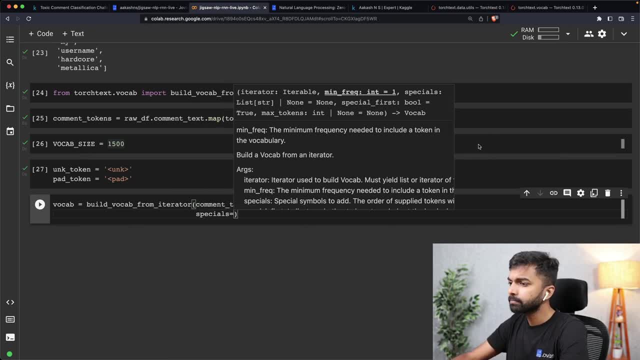 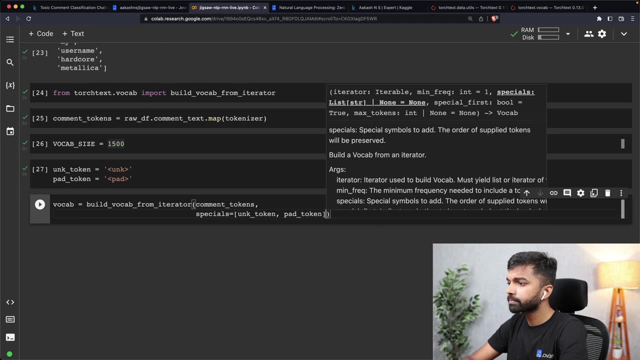 So I'm going to pass these specials. So we have the special UNK token and pad token. These are the two Special tokens that we're going to use. Then we are also going to pass max tokens, and the max tokens is simply going to be the vocabulary size. 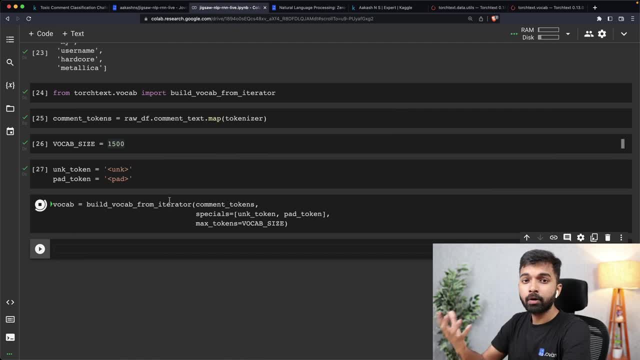 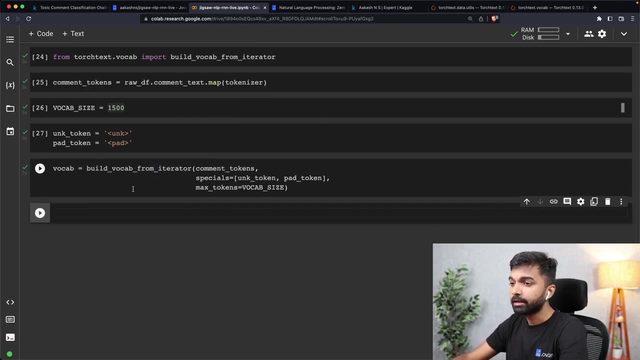 Okay, So one thing you should experiment with is a larger or a smaller vocabulary size, and that will help you learn more or less respectively. Okay, So now the vocabulary has been created, So build vocab from. iterator has looked at all the comments and of course we've. 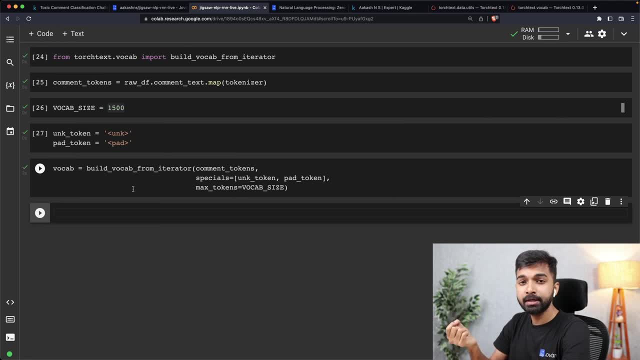 given them in tokenized format. It Has identified all the words that are present in all these comments. It has identified the thousand 1500 most common words, and then it has just kept those, and now we have a vocabulary. Okay, So here's how we can use a vocab. 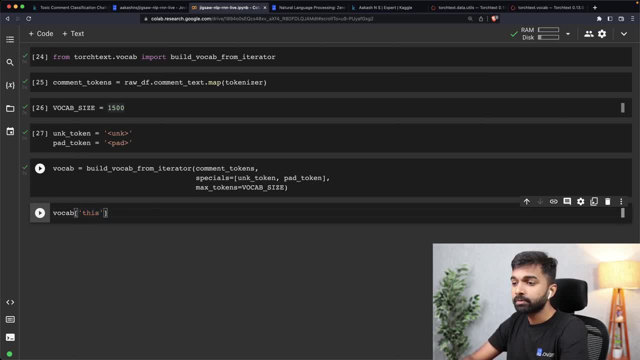 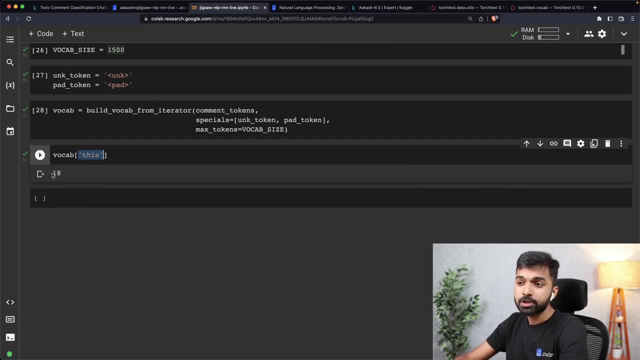 So let's just- we can use it like a dictionary and let's just pass the word This and vocab is going to tell you that this has the position 18. so all the vocabulary does is it assigns a number To every word, And this is how we convert our tokenized comments into numbers. 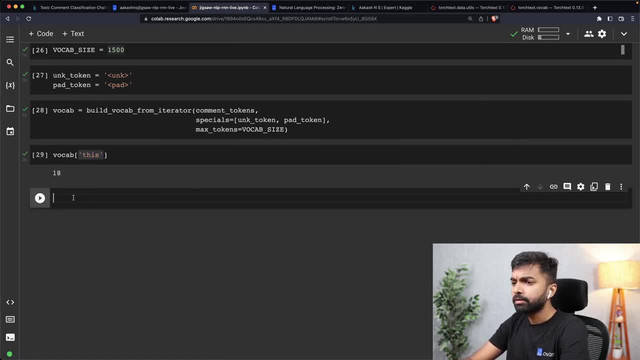 Okay, And similarly one, or you can also do the other thing you can get. you can say something like this: will gap dot get tokens and you can just give it a list of tokens. So, for example, we have these sample comment tokens: 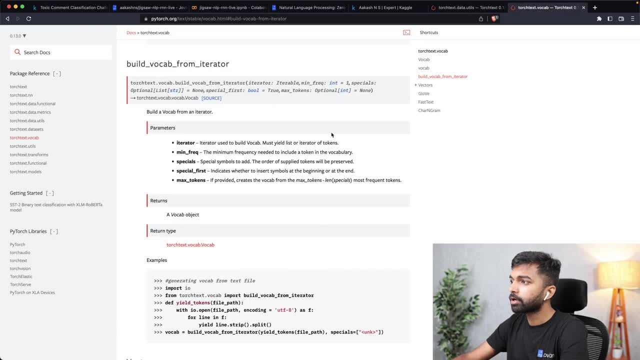 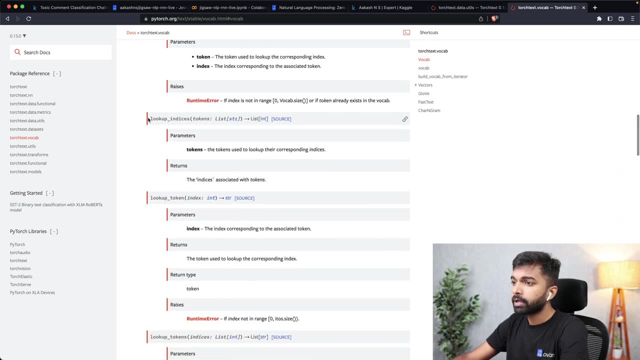 Oh, actually, let's see, let's just go in here into touch text, start vocab, and let's see what are the differences, What are the different examples or what are the different things you can do with it. So you can do this, you can go look up indices and you can give it a list of tokens and get. 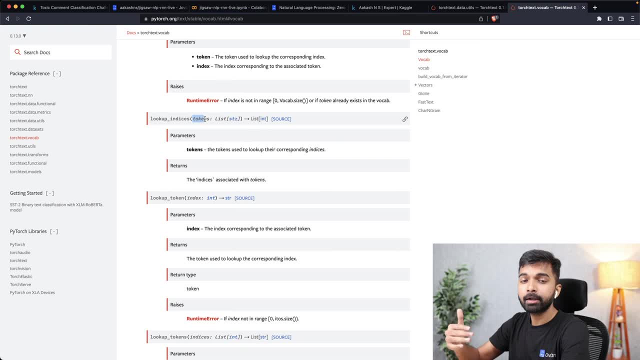 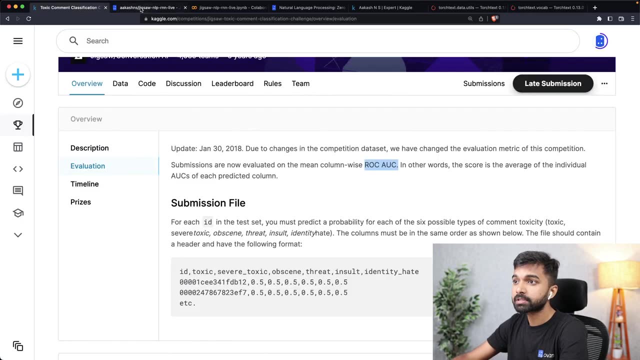 back a list of indexes. So each word that you provide will get converted into a number, and you can also do look up tokens and this. you can give it a list of indices and you can get back a list of tokens. So let's try to do that. 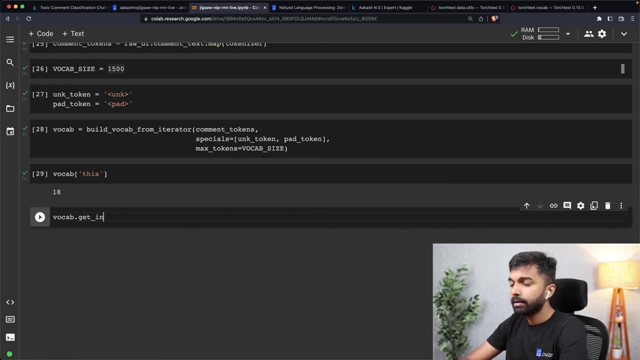 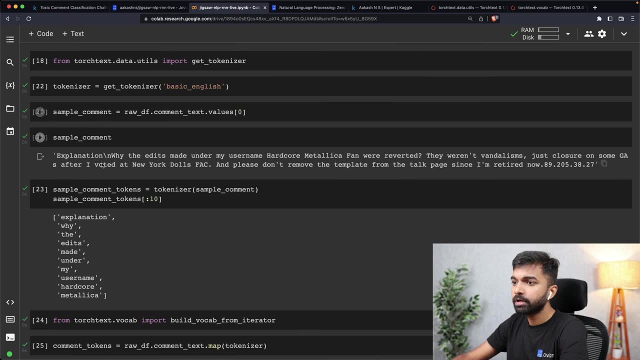 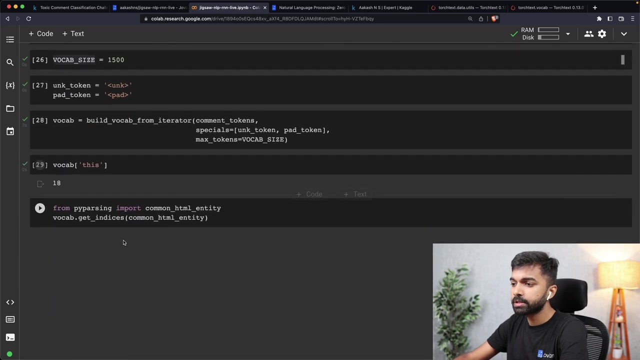 Let's first try get indices and let's give it The sample comment tokens. So here we see, we have the sample comment and we've converted that into sample comment tokens and that's- and these are some, the first 10 tokens. 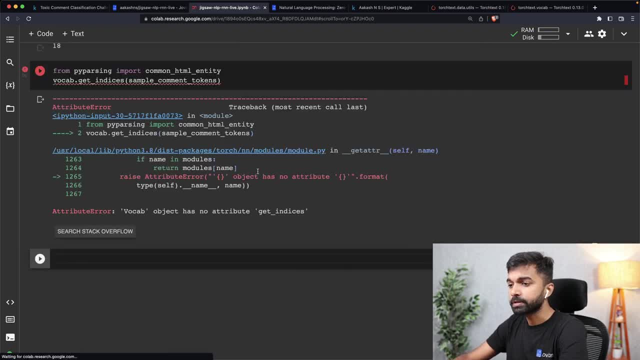 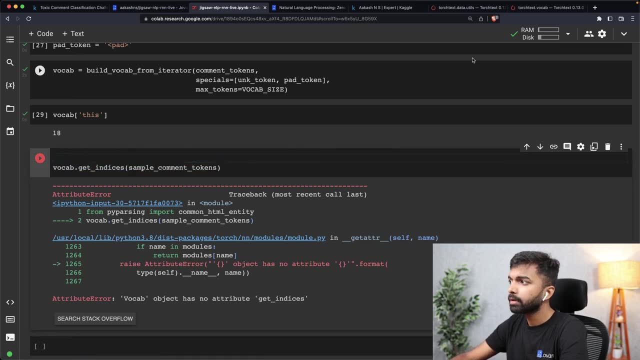 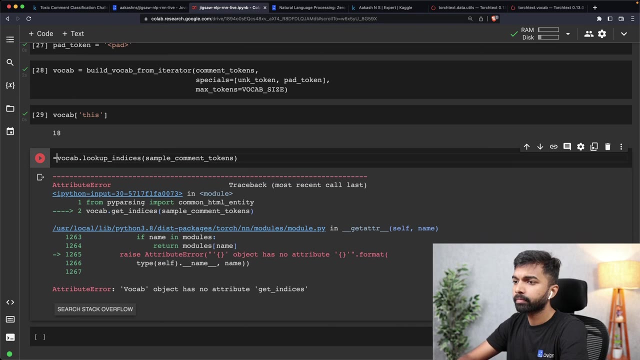 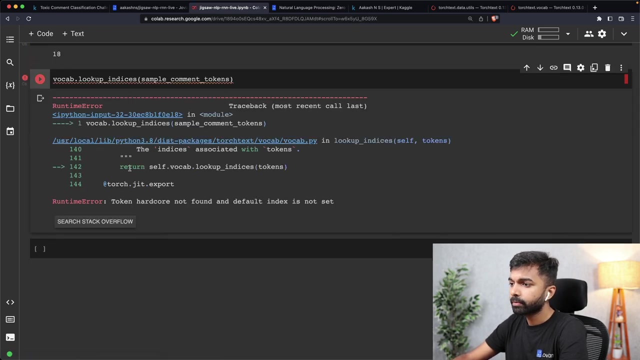 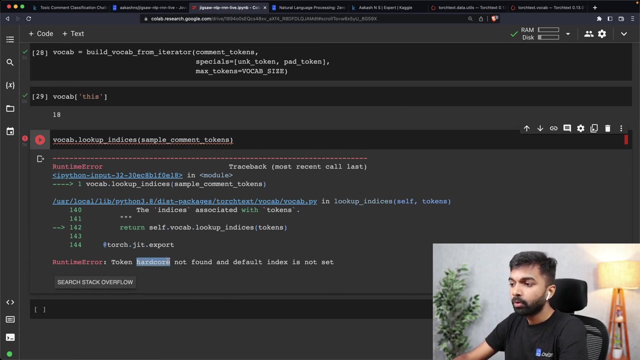 So let's give vocab dot- get indices, sample comment tokens. Let's try that again. Oh, it's called lookup indices. Yeah, So vocab dot- lookup indices, sample comment token. Okay, So now it tells us that there is a particular word called hardcore which is not present. 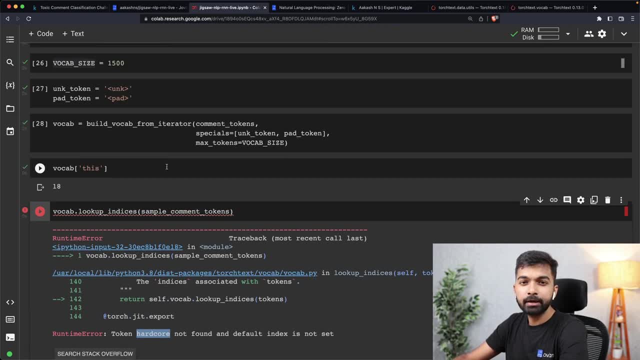 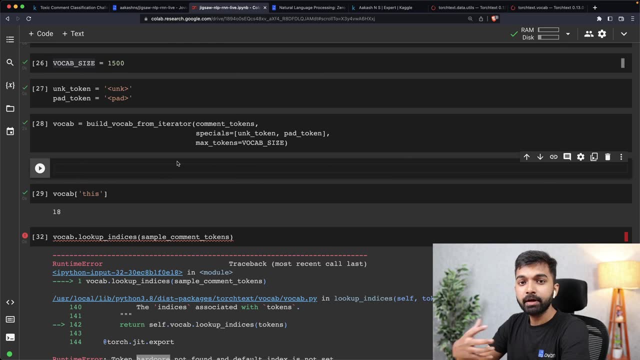 which is not present in the vocabulary, because we've only created a vocabulary with the 1500 most common words. So this is where we need to configure a default token Whenever, whenever a particular word is not found in the vocabulary we want to configure. 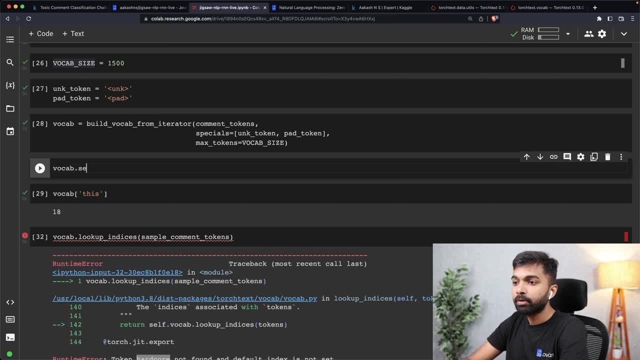 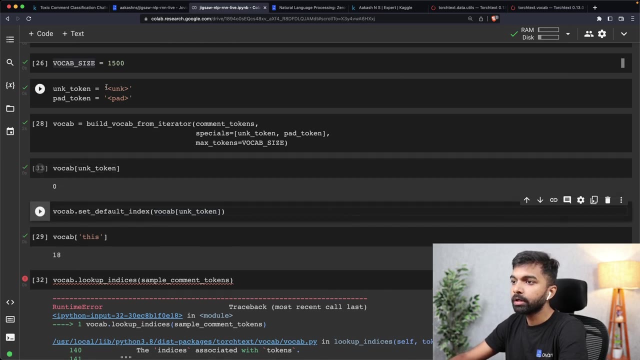 a default index. So I'm going to say, Let's say vocab dot set default index to vocab unk token. Okay, So what are we doing here? We are basically saying that the token unknown as the index zero. that is the first special. 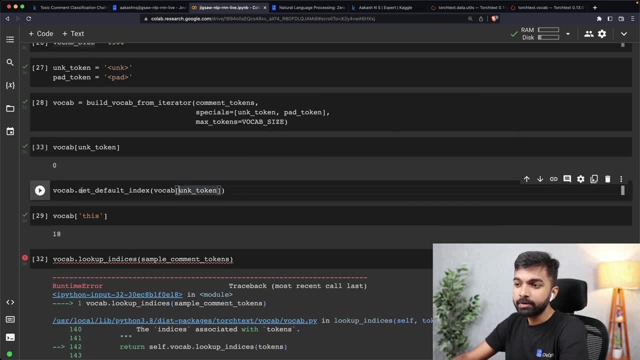 token. So it has a, it has the index zero. And now what we're saying by calling dot set default index is that whenever a particular word in a particular text is not found in the vocabulary, Then is replace it with the token at this index which we are picking here. 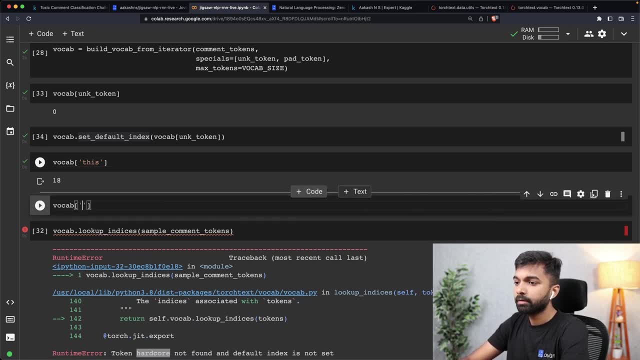 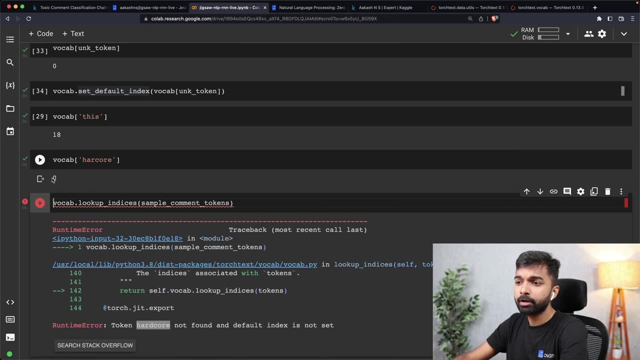 Okay, So now if I say vocab hardcore or hardcore or anything that is not in the vocabulary, it's simply going to return the index zero. All right, So this is how we replace all the out of vocabulary words with the unknown token. 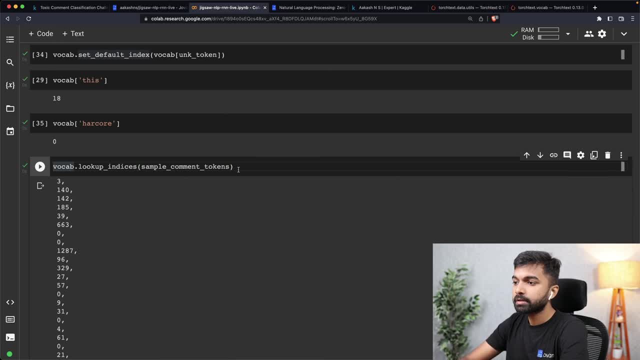 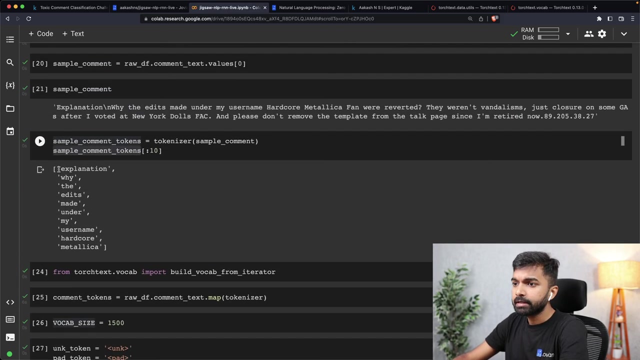 Okay, So now, if we say vocab dot lookup indices, sample comment tokens, And let's just save the sample indices and let's just print the first 10.. So now you see that all we have done is these tokens have been converted into these numbers. 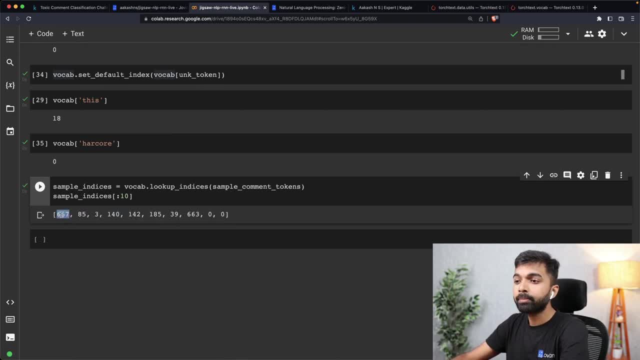 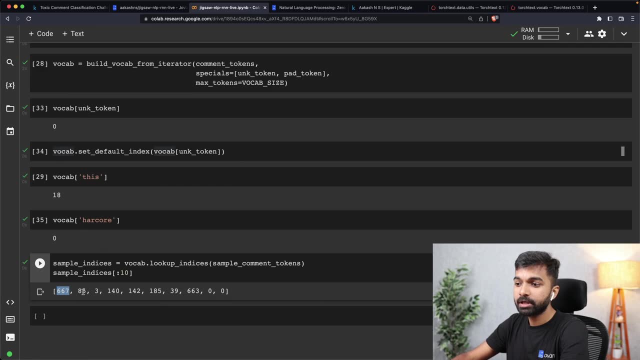 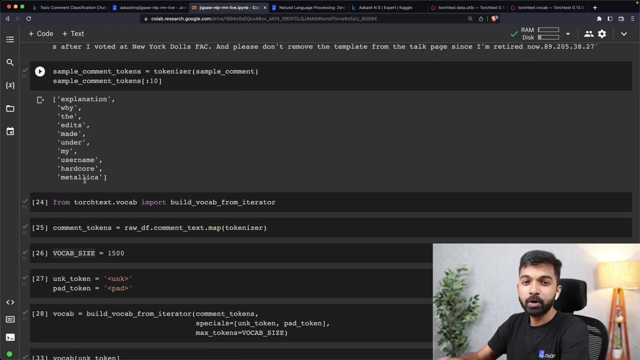 and each number here represents the index of that particular token. So in our vocabulary, the word explanation is at position 667.. The word why Is At position 85, the word though is at position three, and so on. Now notice that the words hardcore and met Metallica, because they're not very common. 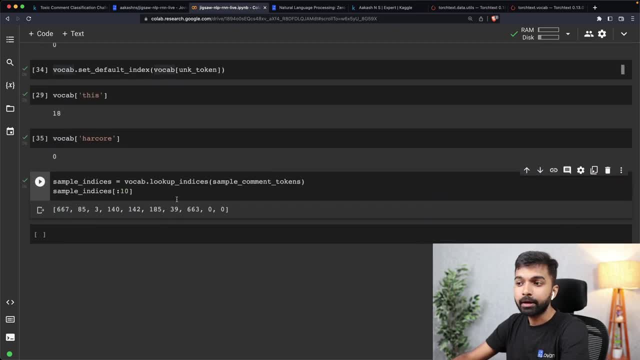 don't show up in the vocabulary, and they have been replaced with zero, which is simply the unknown token. Well, you can do this the other way around as well. So, sample comment recovered. uh, I'm going to call it, which is simply sample indices. 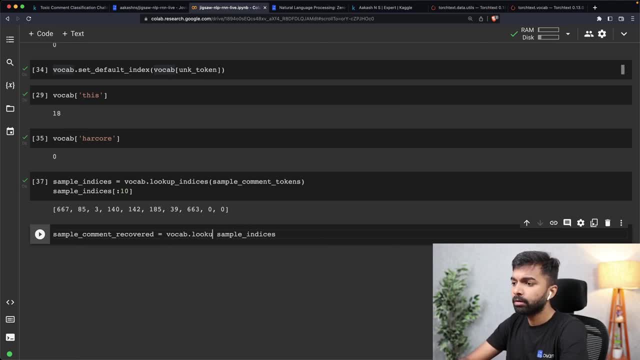 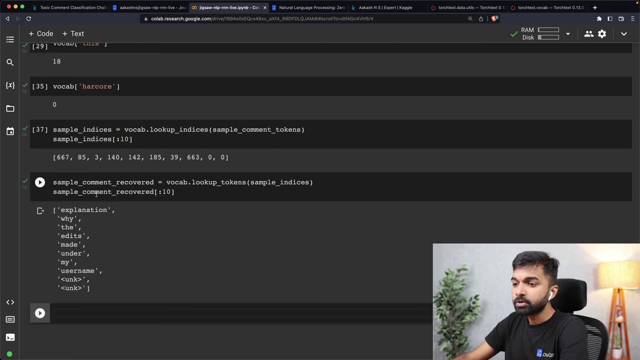 And I'm going to pass sample indices into vocab dot. Look up tokens sample indices and let's print sample comment recovered first, 10.. Okay, So what do we get back? We get back explanation why the edits made under my. so each word corresponds to a number, which is the index here. 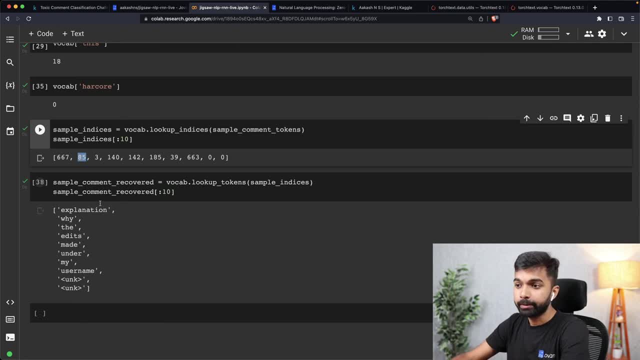 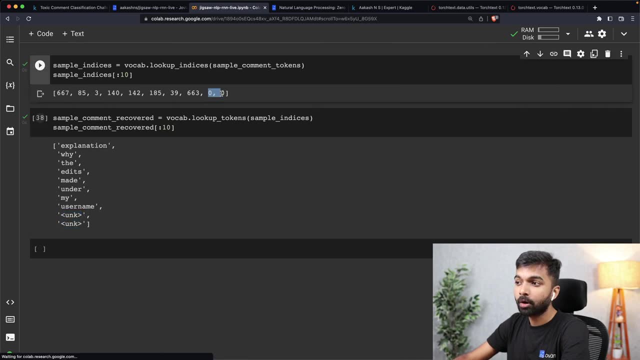 And then each index corresponds back to a word. Now notice that when we try to convert it back, These last two words did not get converted. because these last two words were lost in the encoding, because hardcore and Metallica are not part of the data set or not part of the vocabulary. 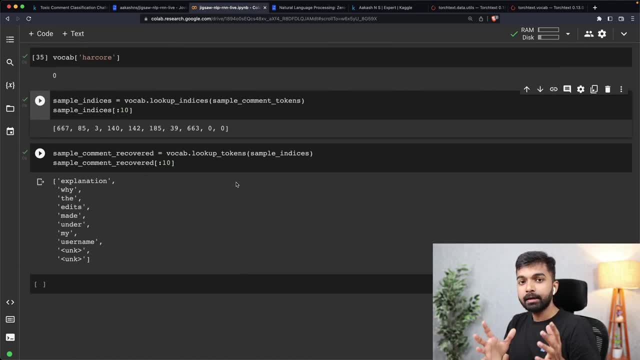 Okay, But the whole idea here is this is how we take our text and convert it into: first a list of tokens and then convert those tokens into numbers, which is a list of indices, or those tokens in the vocabulary. Okay, So now we have learned the vocabulary. 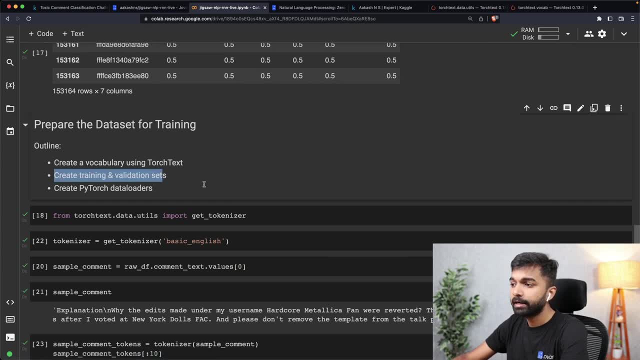 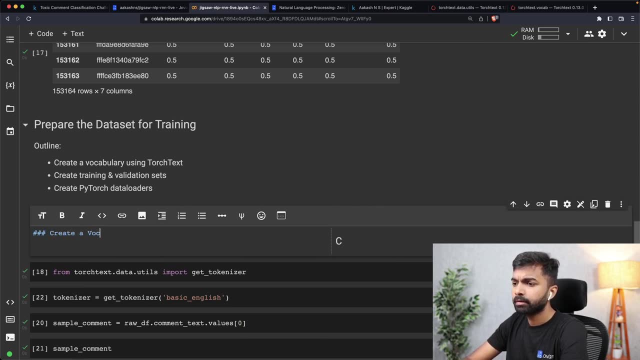 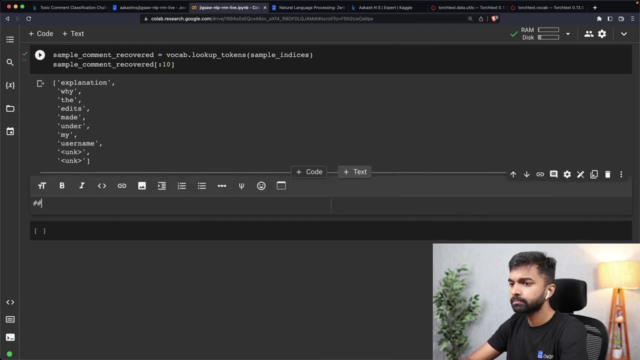 That was the first step. The second step is to create training and validation sets. Let's give these section names. So I'm just going to create top sections here. So create training and validation sets. Let's get into that, All right. 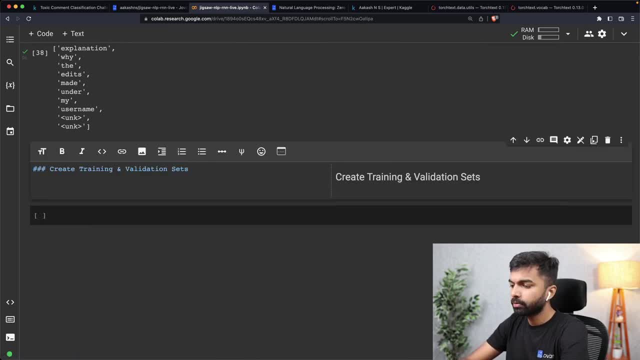 So how do we do this? How do we do this? Well, we are first going to define a custom I touch Data set, then we are going to create, create or pass the raw data into the data set And finally, we are going to let the PyTorch data set. 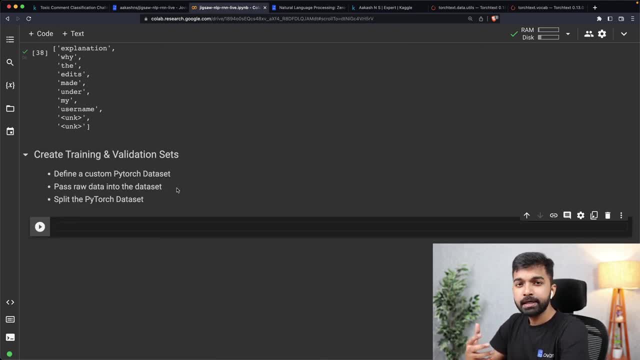 Okay, So so far we have created data sets for scikit-learn, but because we're using PyTorch, We are then going to create a. we're now going to create a PyTorch data set. So here's how you create a PyTorch data set. 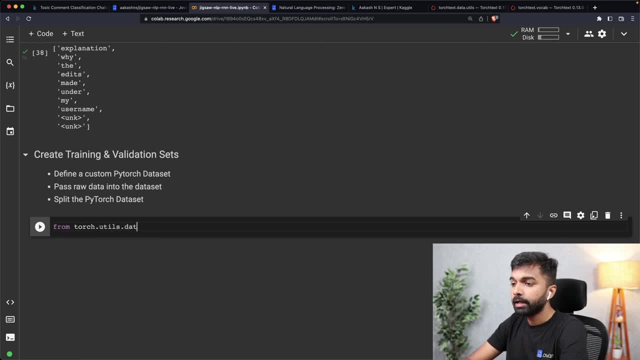 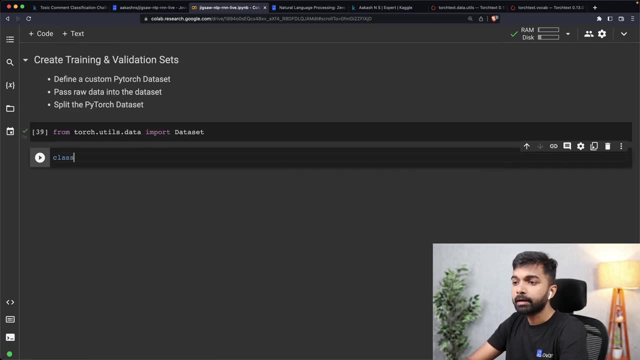 You say, from torchutilsdata import data set And now we can create a custom data set class. So I'm going to call this jigsaw data set and this is going to extend the data set class. And in any PyTorch data set we have to implement three things. 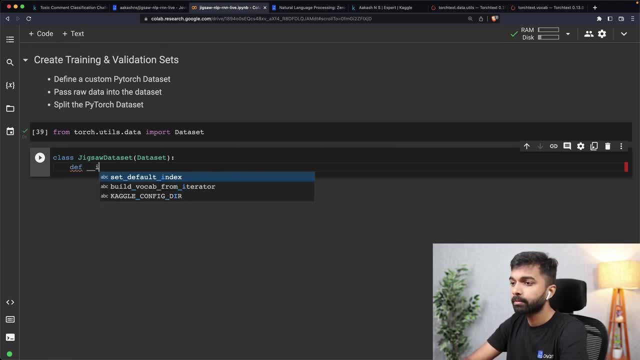 The first, we have to implement an init function. This is how you define functions within a class or methods within a class. Then we have to implement the get item function. The get item function is going to be called with an index and we have to return the element at that index. 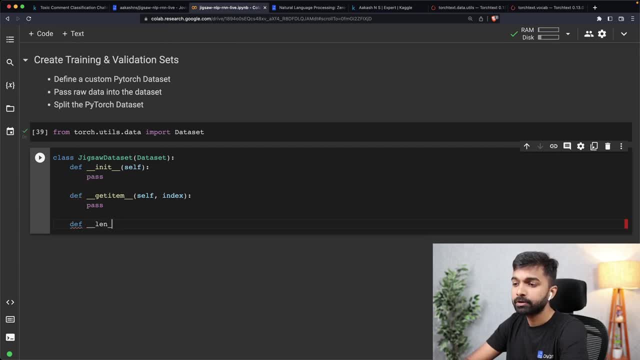 And finally, we have to implement a len function- Underscore, underscore. len, underscore, Underscore. This is supposed to return the size of the data set. Okay, So what exactly do we want to do here? So what exactly do we want to do here? 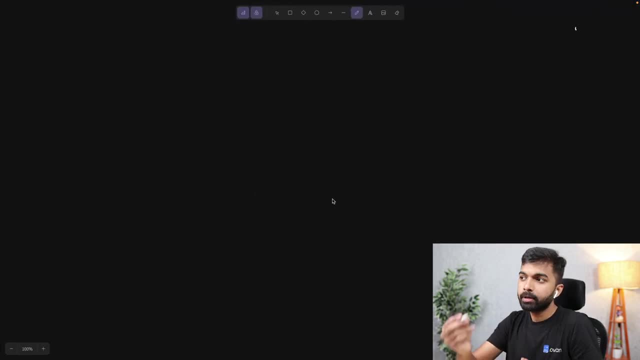 Let's take an example. So let's say: we have a comment. This article is great, All right. So now we have a comment. The first thing we want to do is Split it into tokens for which we already have a tokenizer. 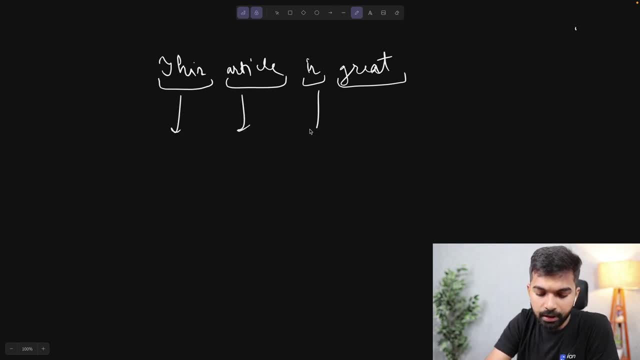 The next thing we want to do is convert these tokens into indices. So let's say this article is gate. So let's say this has the index, index 18.. Let's say article is not present in the vocabulary, So this will get the index zero of the unknown token. 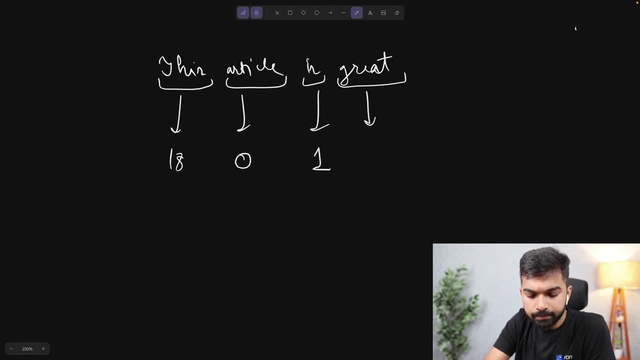 And then this is: is is going to get the index one, maybe, or let's say 12, or let's undo that- Is is going to get the token index 17,. maybe and great is going to get the token index 23, or something like that. 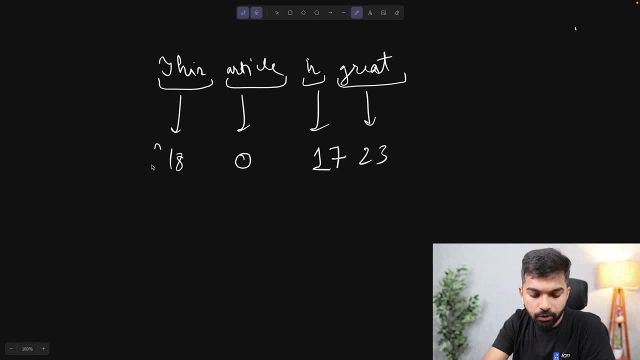 Okay, And then we? this is going to be the input that will be passed into the model, but there's one thing we want to do. Suppose there's another comment called I love this. So this comment is only three words long. 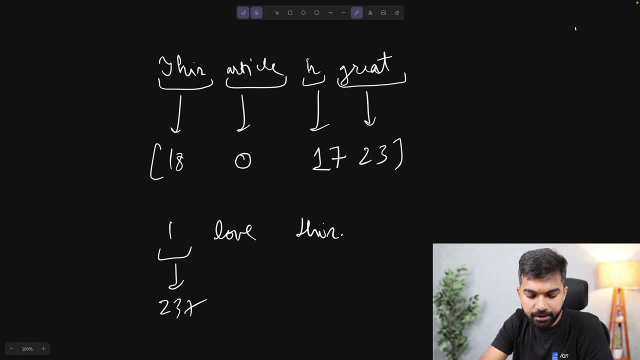 So again, we're going to convert, Okay, These. so let's say, this is 237 and this gets converted to 73, and then this and this, the word this here- gets converted to 18.. Now, these two inputs are of different lengths. 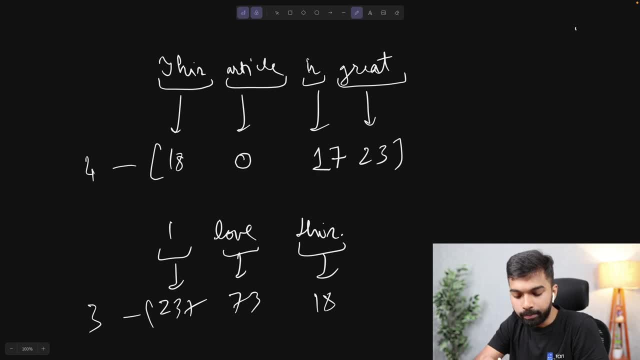 This is of length four and this is of length three. That is a problem, because recurrent neural networks, or neural networks in general, expect data to be properly formed, have a nice shape. So what we're going to do is we are going to insert the padding token here, the pad token here. 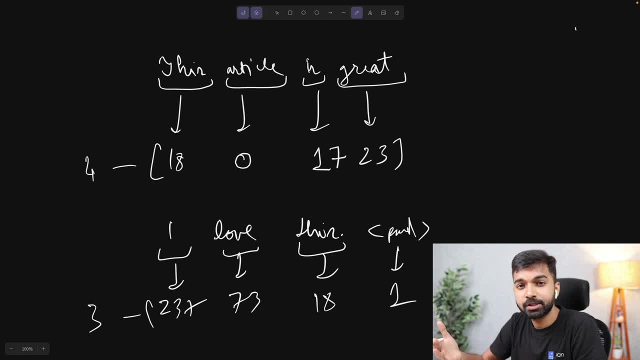 And then the pad token- because we pass it as special symbol- has the index one and the unknown token has the index zero. So this becomes two, two, 37,, 73,, 18, one. So what we need to do is add the short sequences or the short sentences. 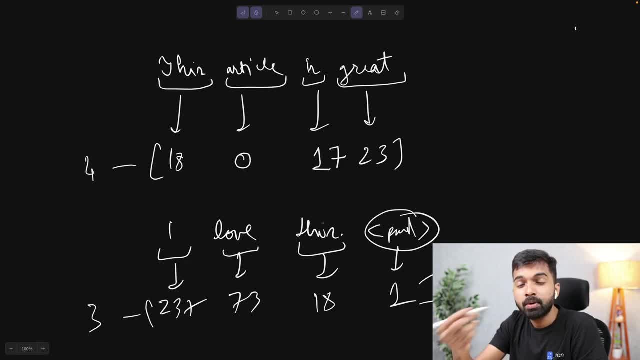 And again, we also want to fix a maximum length. So let's say we have fixed a maximum length as four, and then this article is great. I suppose this one also has an, isn't it at the end? So that's two more tokens, isn't an eight? 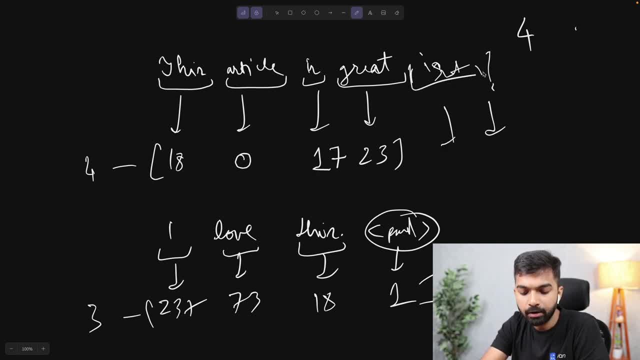 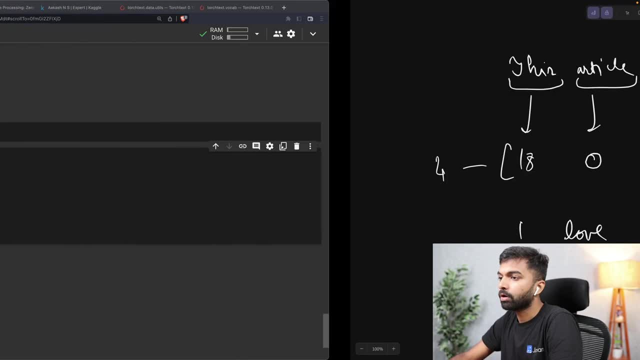 Now, because our maximum length has been fixed to four, we may need to get rid of the last two tokens. All right, So let's write a helper function called pad, which is going to help us do all of these. So I'm going to first create a function. 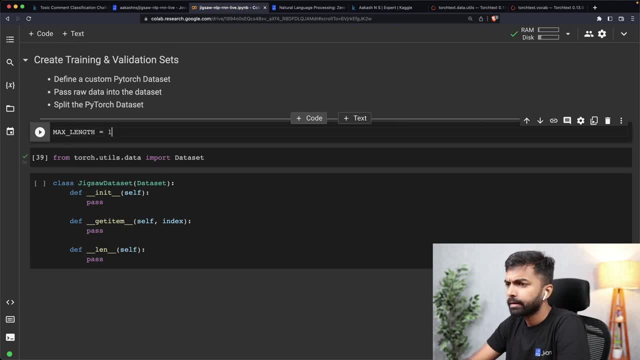 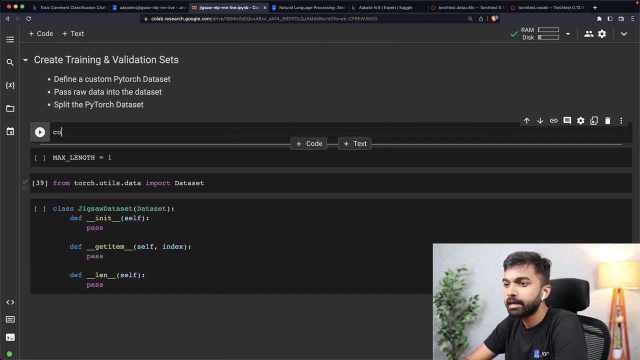 I'm going to first define a variable called max length and we are going to set the max length. How do we decide what to set the max length? as let's see, I'll do a quick analysis. So let's take. let's take Roddy F. 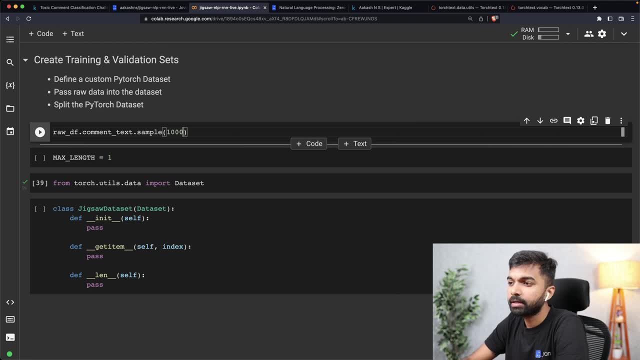 Dot comment text and let's take a sample of maybe a thousand comments And then let's map these to, let's add tokenizer. Let's map these to tokenizer, which means we let's converted, which means let's convert these comments into tokens. 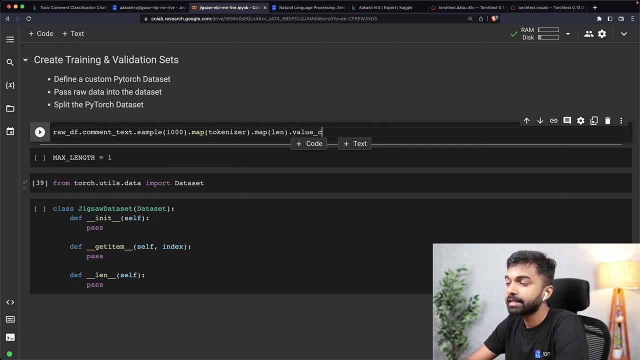 And then let's get the lengths of these tokens, and let's then get the value counts And finally let's plot it As a histogram. Okay, So now that's a lot of pandas logic going on here, but I'll just tell you quickly what is happening here. 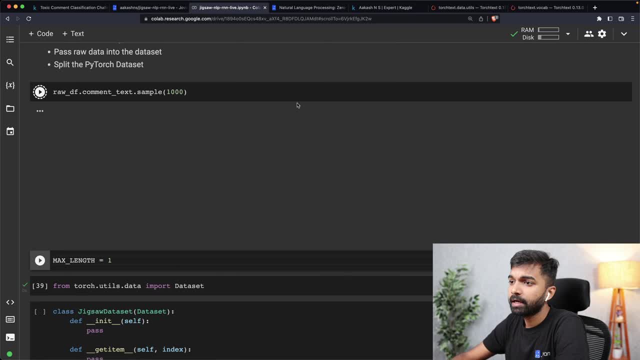 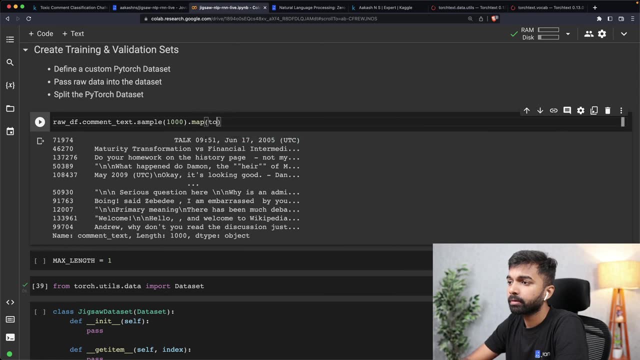 And we can actually just see it step by step. So here we have taken a sample of thousand and if we add dot map tokenizer, that is going to give us A list. So each of these, each of these comments is going to get converted into a list. 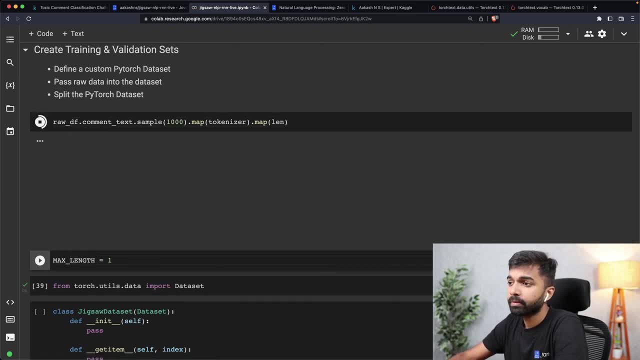 And again here, if we map dot, Len now for each token or not for each comment, here we have the length in terms of the number of tokens. And then now, if we call dot, P, dot, plot, kind equals hist. that is going to now create a histogram which is going to tell us how the lengths of the tokens are distributed. 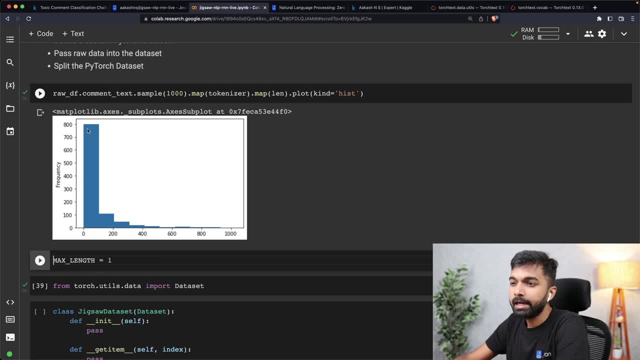 So you can see here that, Okay, Out of the out of the thousand, 800 tokens are under 800 tokens are under a hundred characters, under a hundred. Out of the thousand comments, 800 comments have less than a hundred tokens. 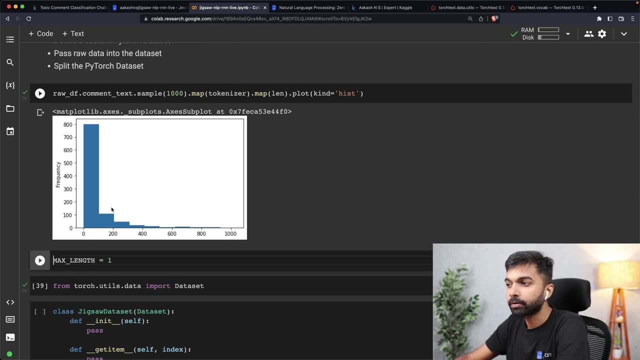 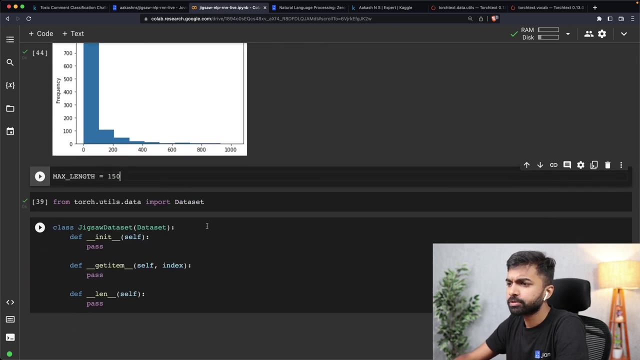 And then about another hundred or so have less than 200 tokens. So what I'm going to do then, is I am going to just pick a certain max length, which is the number of tokens that any particular comment is allowed to have. let me pick 150, just to just to cover 90% of the comments in their full length. 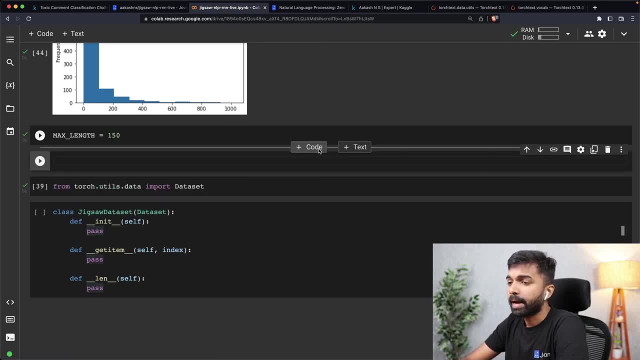 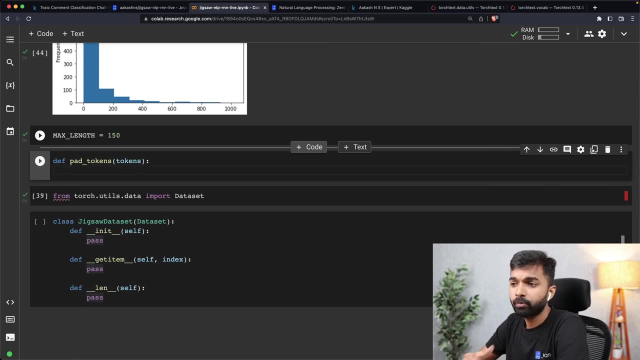 Okay, And now let's create another function called Pat tokens, And this is going to take a set of tokens which is a tokenized comment, and this is going to pad it. So the way we're going to do this is if there are less than max length tokens, or if there. 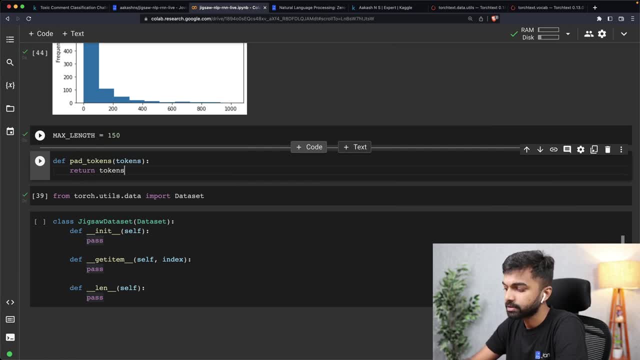 are more than max length tokens, then we need to pick only the first max length tokens. Okay, So if the tokens has more than 150 tokens, then we are going to just pick the first 150 tokens. On the other hand, if token has tokens as less than 150 tokens, then it's simply going. 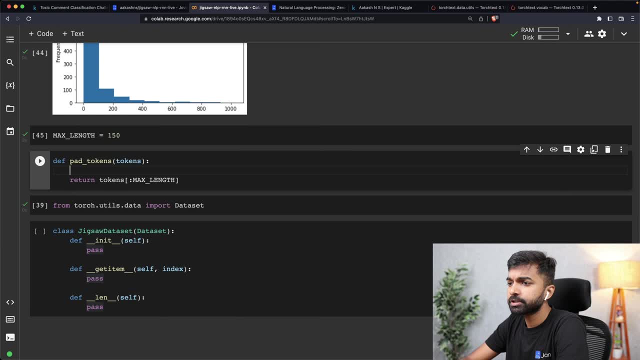 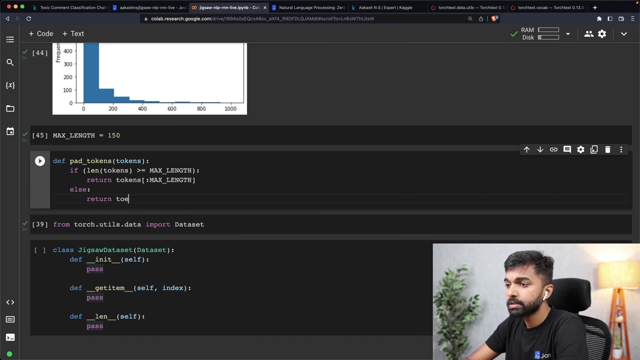 to return. Well, actually, let's just put an if condition here. So if Len tokens is less than max length or is greater than max length, greater than or equal to max length, then this is what we want to return. If it is shorter, then we want to return tokens, and then we want to add a few more. 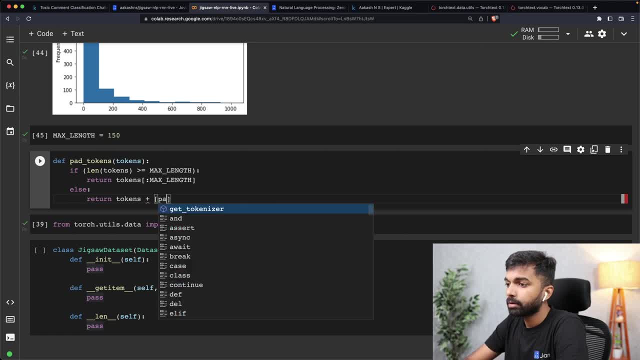 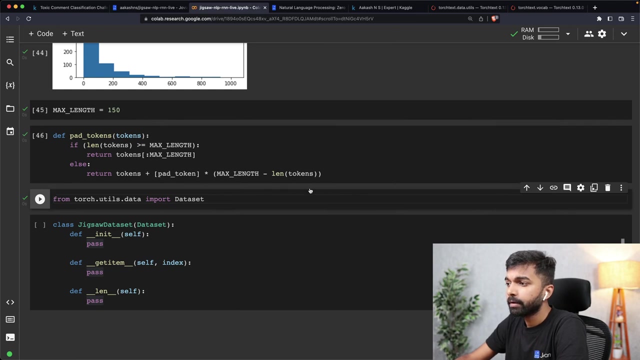 So we want to add the pad token, But we want to add it a number of times that we don't want to just add the pad token once. we want to add it: max length minus length, tokens, number of times. okay, Now you can see this in action here. 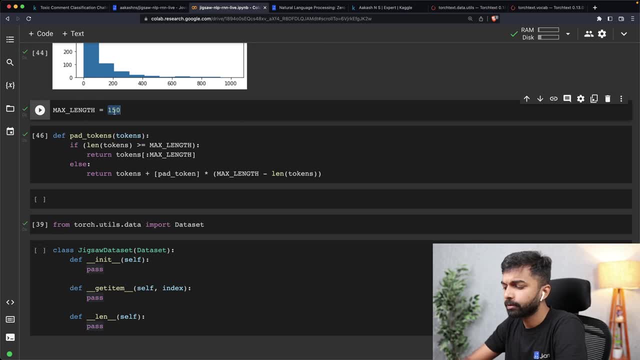 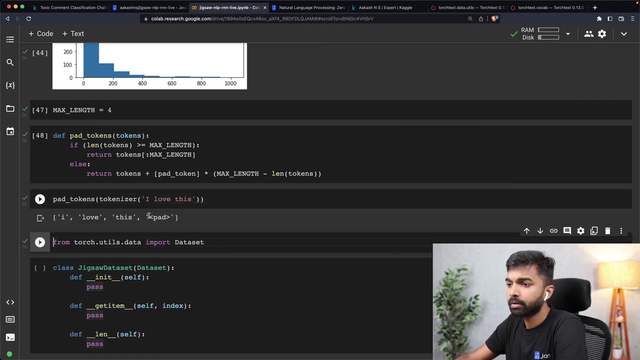 Let's say we have for a second, I'm just going to change max length to four. And let's say we call pad tokens on tokenizer. Okay, I love this. So it's going to convert that to I love this, And then it's also going to pad it at the end. 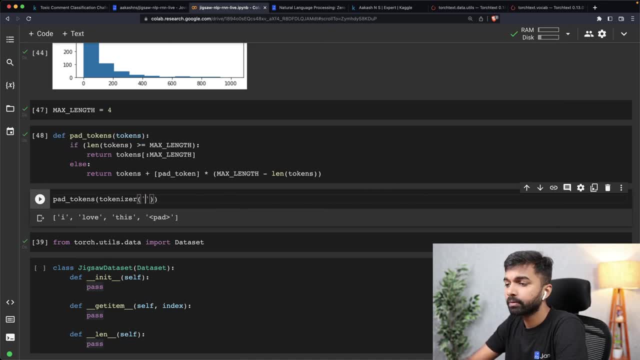 On the other hand, let's say, I call it with. this is great, Is it not? Now, in this case, it is gonna tokenize it, but it's only going to pick the first four tokens. Okay, So that is more than max length, and it's going to just pick the max length first, max. 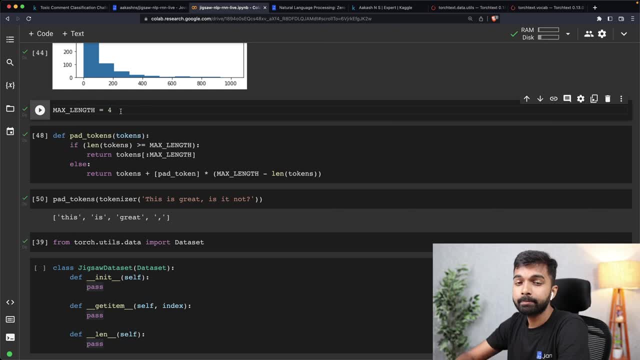 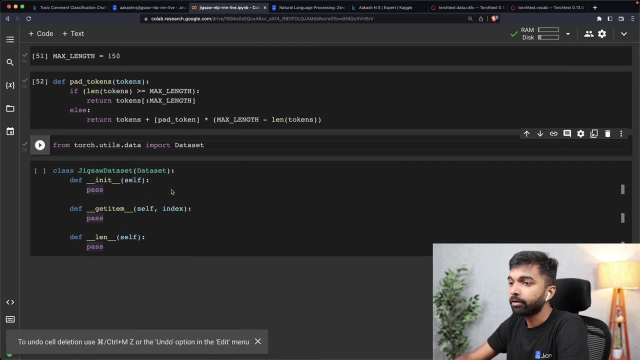 length tokens. If you have a comment that is shorter than max length in terms of the number of tokens, then it is going to add the pad token. all right. So with that out of the way, we now have a way to pad tokens. 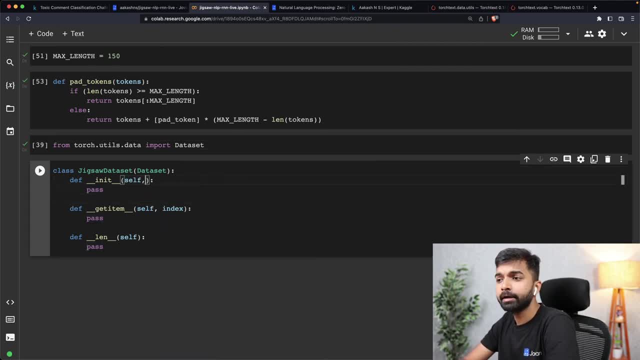 And now we can actually create our data set. So, while creating the data set, we're going to pass a data frame into it And we are also going to pass this information. whether this is a training data set or a test data set, It does not have any labels. 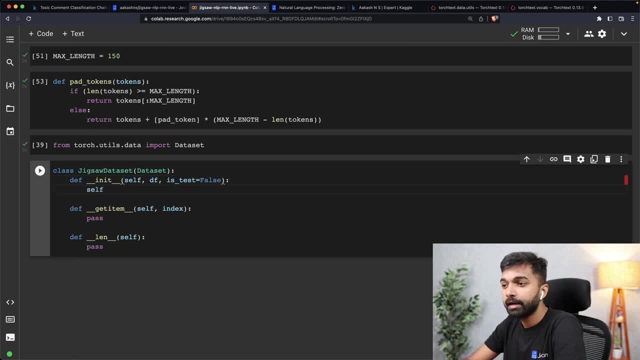 So, by default, is test is going to be false And in the init I am simply going to save the data frame information and I'm going to save: is test equals is test. Okay, This is simply how we create classes in Python. 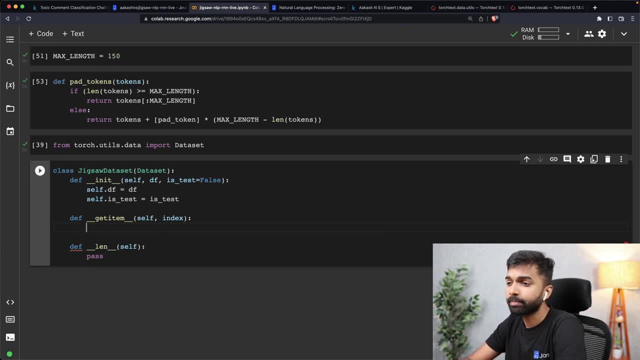 So, in case you're not familiar with this, check out a tutorial on how to create classes in Python. Okay, Next, Len should be easy, So this should simply be return Len selfdf. So whatever data frame They're storing within the data set, that itself is going to be the length of that data frame. 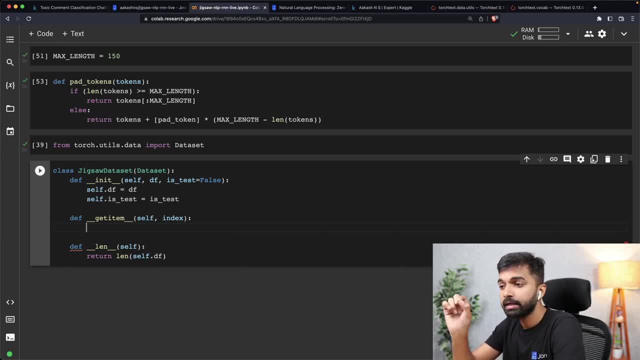 is going to be the length of the data set. num. get item- you're supposed to get the item at a particular position And in get item you're supposed to return two things. you're supposed to return the input, the input value and the target value as well. 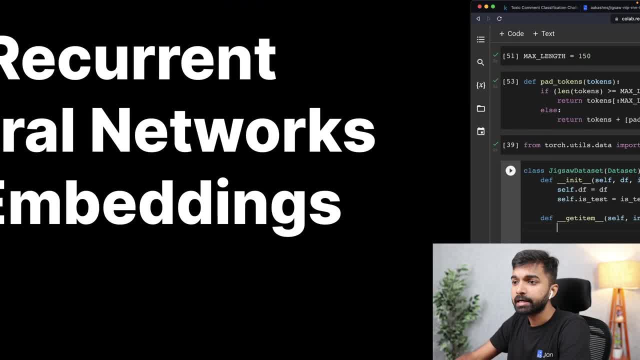 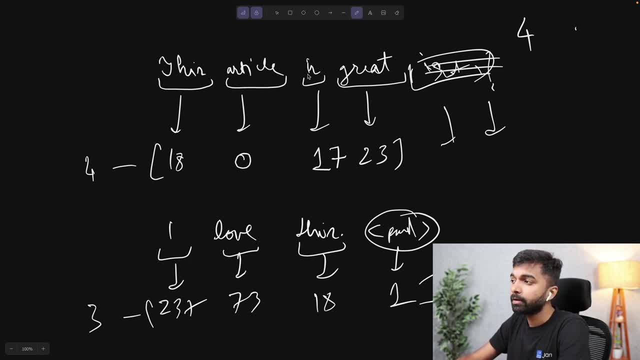 So the input in our case is the, as you can see. as you can see here, the input in our case is going to be: first we take the text, then we tokenize the text, then we pad the text and then we convert it into numbers using the vocabulary right? 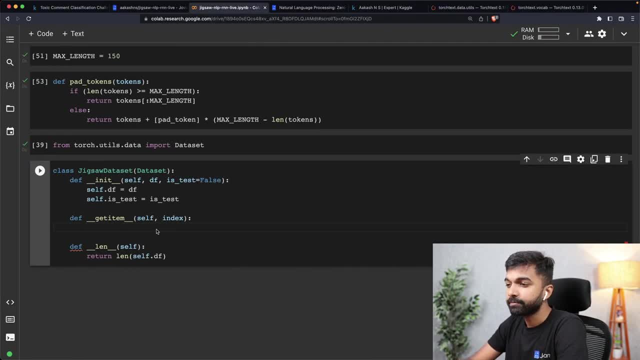 So all of that has to be done to get the input. So let's see, let's first get the comment text at the given, at the given index. So comment text is simply self dot, df, dot. comment text, dot values index. all right, 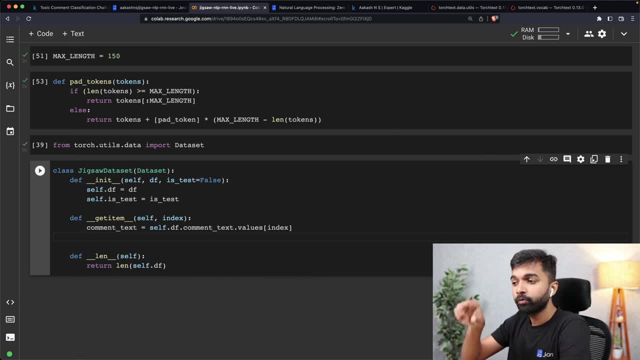 So from the data frame that we are going to create the data set with, we're going to get the comment text column. from that we will get the values, the list of values, from the comment text column and we just pick the value at the given index. 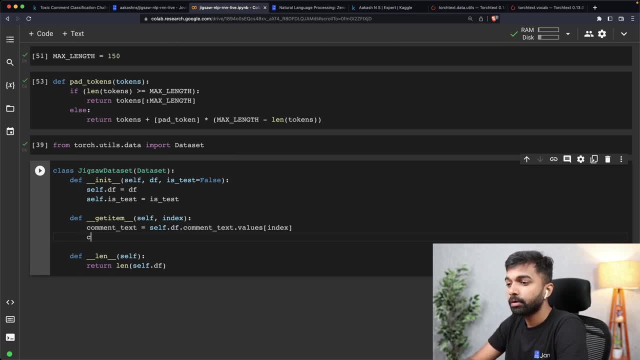 Then we can convert it into the input. And the way we convert it into the input is first we say pad tokens, comment text, and that is going to ensure that it has the proper max length, And then we are going to have before pad tokens, we have to tokenize it. 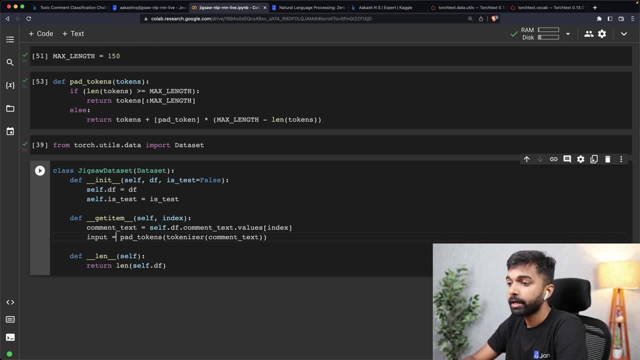 So, tokenizer, we're going to pass it to the tokenizer, All right. And then one last thing we're going to do is we're going to convert into pytorch tensors. So I'm going to- I'm going to also import torch here. 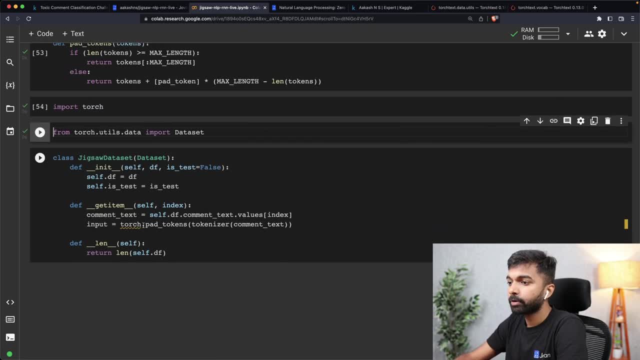 And I'm going to write torch dot answer that. okay, then we also have to create the target value. So how do we get the target value? Well, first, if it is the test data set. so if self dot is test, then there are no target. 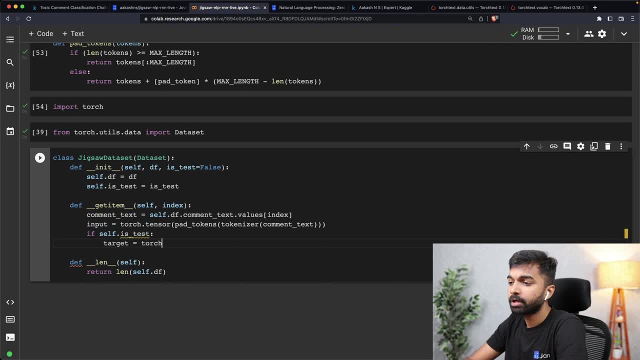 value. So this should be easy. So target equals: remember that there are six classes of target, though there are six classes we need to make predictions on. So, torch dot tensor, I'm just going to return zero, zero, zero, zero, zero, zero. all right, 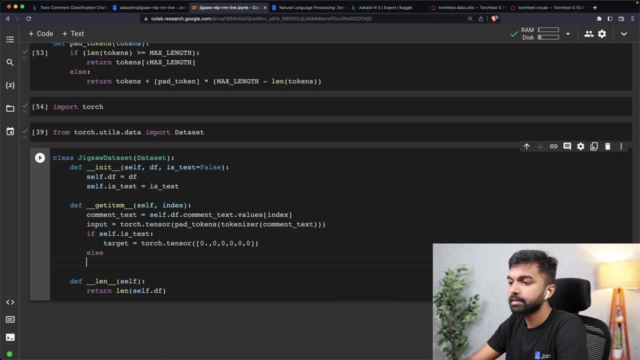 so six zeros, else the target is. let's see comment text: no self dot df. so from self dot df we get the target columns, And from the target columns we just get the values, And from the values we get the given index. 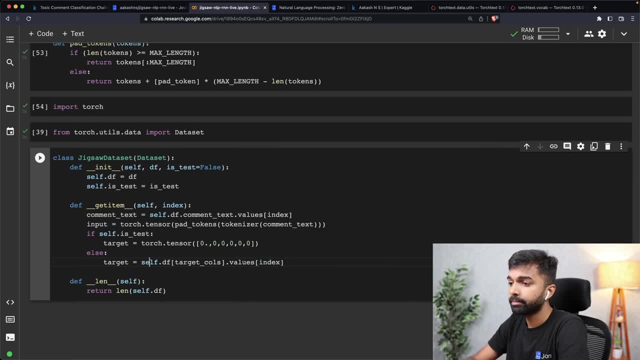 All right, and that is going to be the target, And I'm just going to convert it into torch dot tensor. Yeah, I think we don't need. Yeah, I think we may need to convert these into float. So I'm just going to convert these into float. 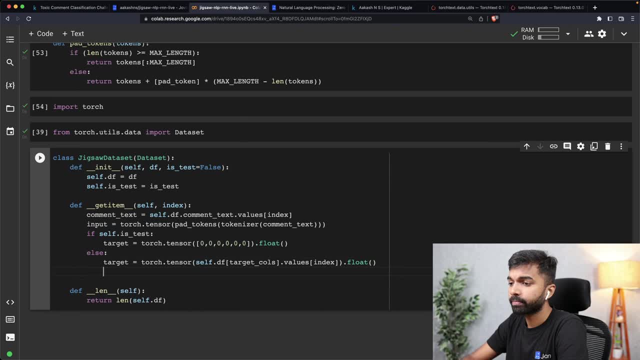 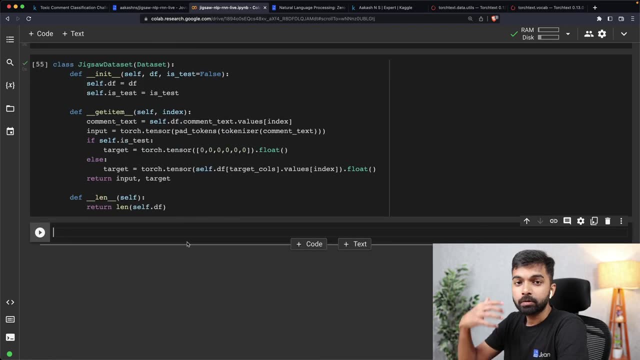 Because otherwise some of our loss functions etc. might complain. Okay, And then, once we have picked the input in the target, we simply have to return it. Okay. So this is how we can. This is how we create a custom data set in PyTorch. 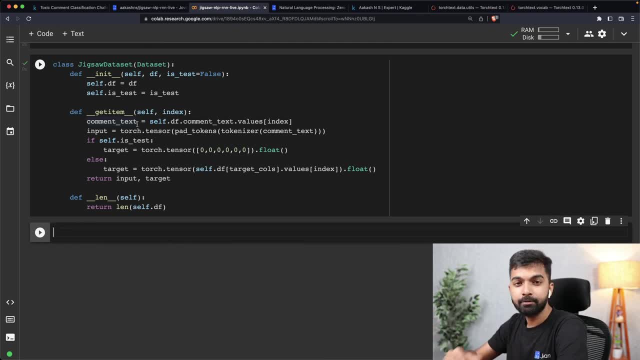 It looks a bit complicated. I encourage you to work it out line by line And we look at its users in a second. But basically what we're doing is we are initializing it. So let's create the raw data set. I'm going to call it raw DS or for raw data set. 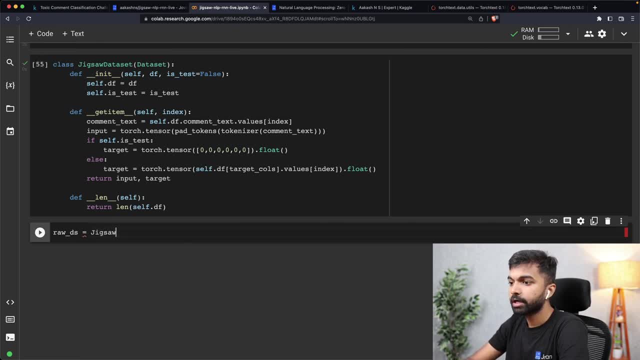 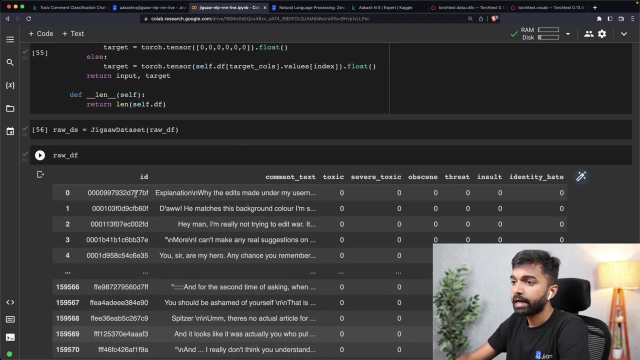 And raw data set is simply jigsaw data set called with the data frame, which is raw df And is test- is false, So that we don't need to pass That. Okay, So if you check raw df- or actually I'm just going to check the first couple of first few- 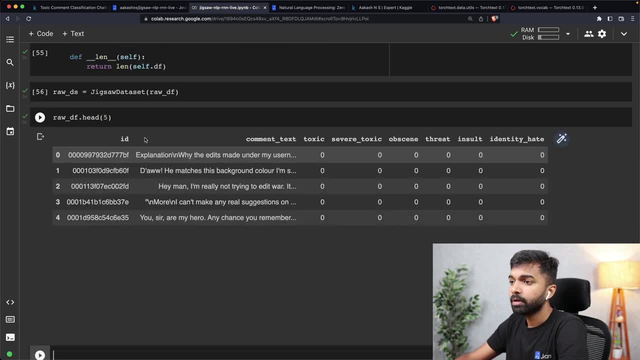 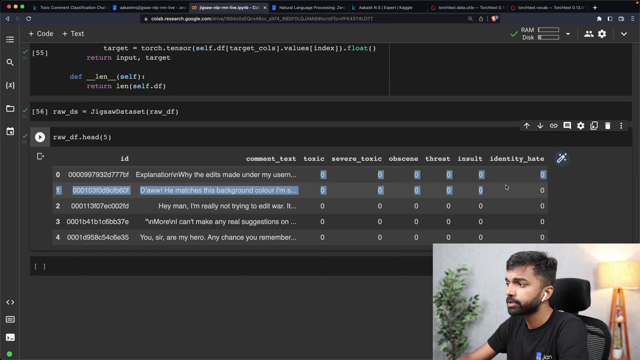 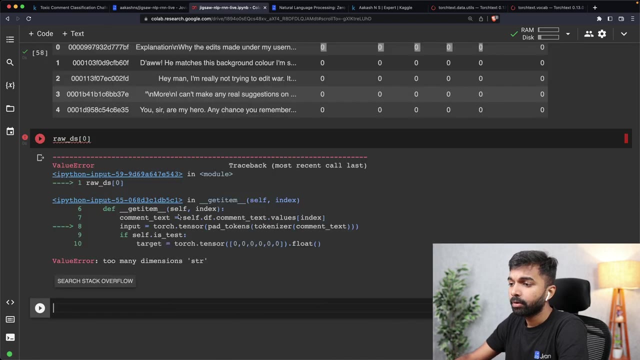 rows. So raw df, head five. So this is what the data frame looks like, the pandas data frame, Okay, and this contains this comment text and it contains this information about this, the labels. But if I check raw DS and I give it the index zero, okay, what's happening? here we are. 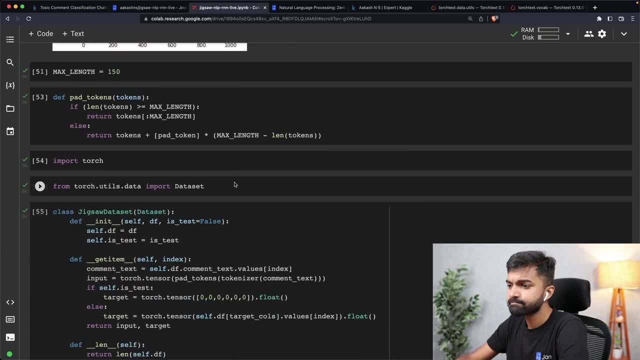 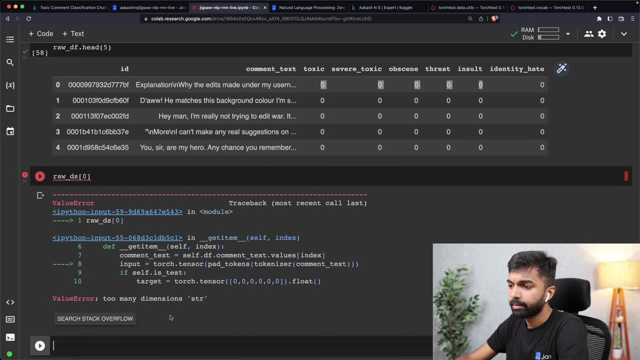 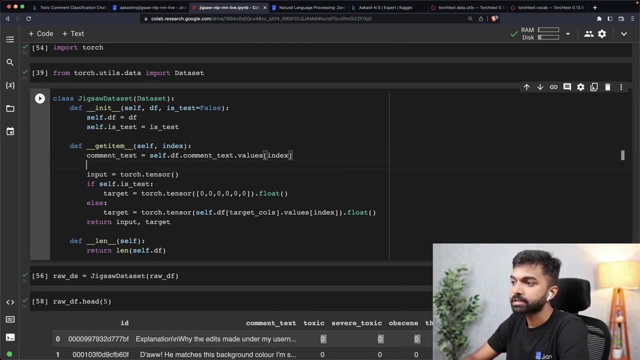 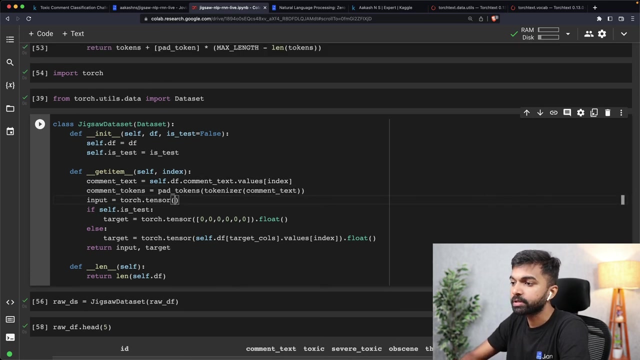 saying pack tokens tokenized: Okay, These are common text, Too many dimensions, STR. we forgot to actually convert the tokens into numbers. So common tokens. and now we want to convert these tokens into numbers. So we also have to say vocab dot. 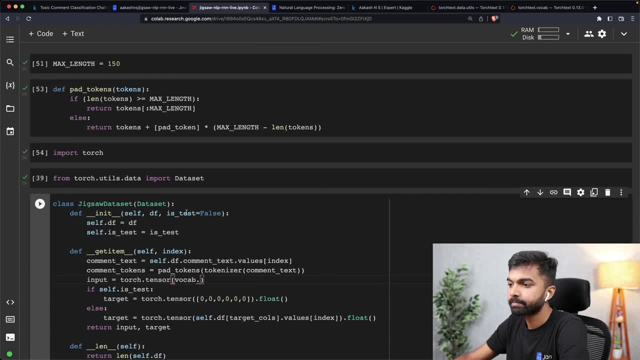 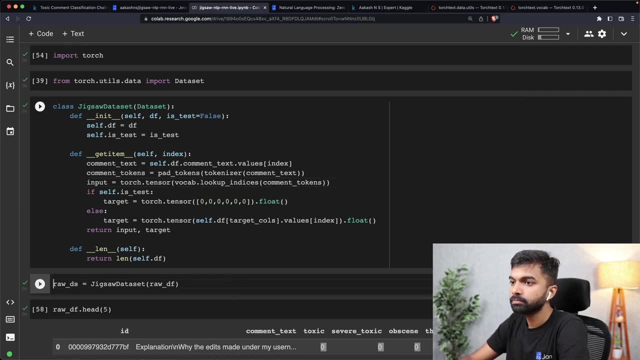 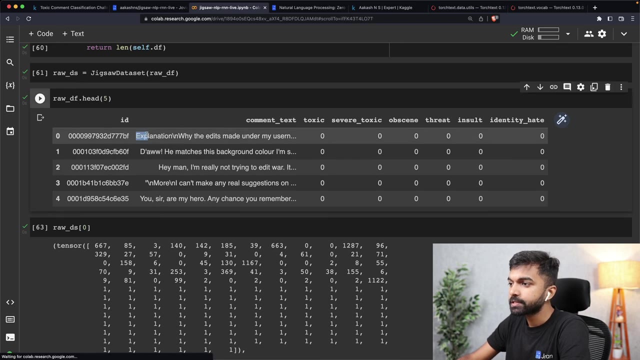 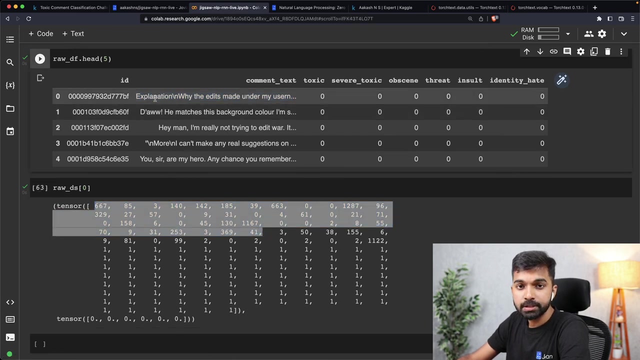 What was it called? vocab dot- look up indices. Yeah, Common tokens. Alright. so now you can see what has happened. There was this common text And we took this common text And we then converted the common text into tokens. 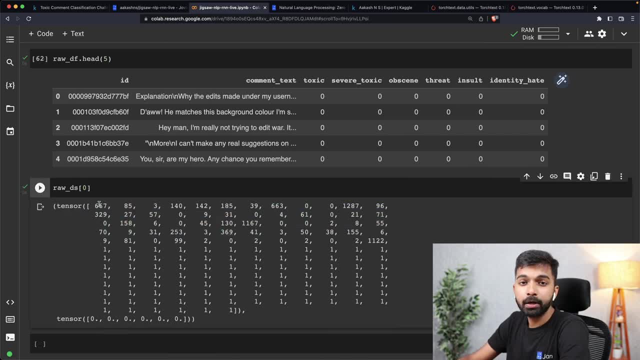 Then we also padded it with a bunch of pad characters And then we converted it into indices using the vocab, And this is what we get finally out of it, And of course, the target for this case is all zeros. So the target here is going to be all zeros. 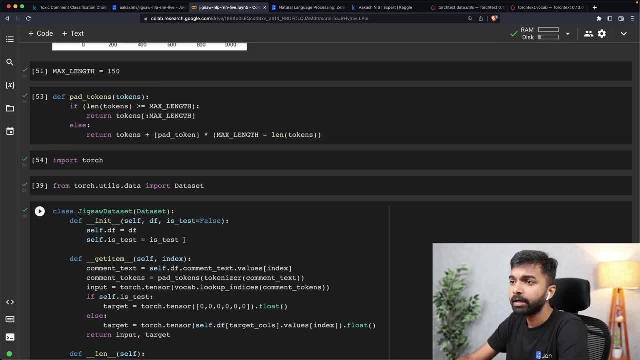 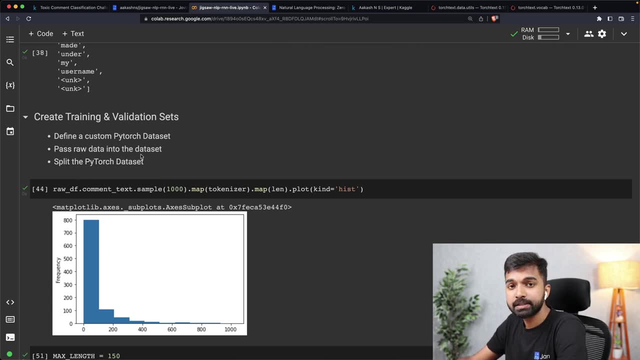 So that's how you create a pytorch data set. Pretty straightforward, All right. Now, once we've created the pytorch data set, we have and we've passed the raw data set data into the data set And we can look at example values. we have to then split this pytorch data set into training. 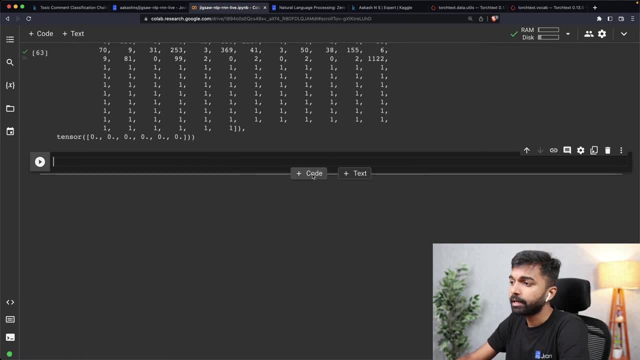 and validation. Okay, so for this I am going to use from torchcom, Okay, Okay, So I'm going to import utils dot data. import random split- Again something you can look up easily, not something that you have to remember. 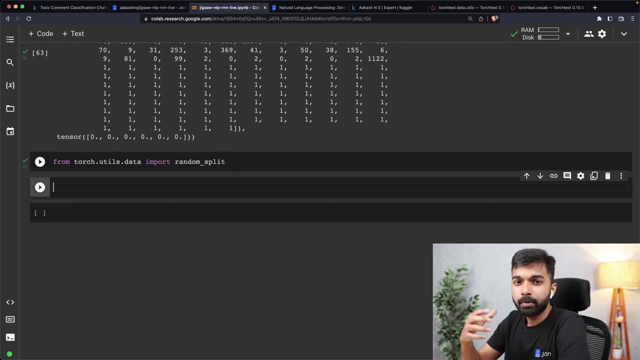 And random split simply takes a certain data set and then the sizes that you want to split it at and it gives you multiple data sets. So I'm going to set the validation set size or the validation set fraction to be point 25.. I'm going to use 25% of the data as a validation set. 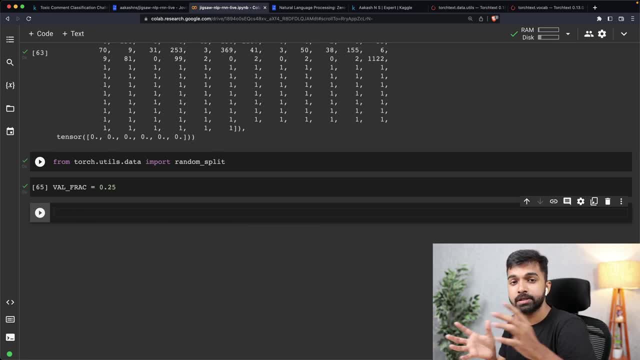 What is the purpose of a validation set? You train your model, Then a certain portion of the data- about 70, 75%- And then you evaluate the model on the remaining 25%. And it's important to do that because your model is going to be used in the real world. 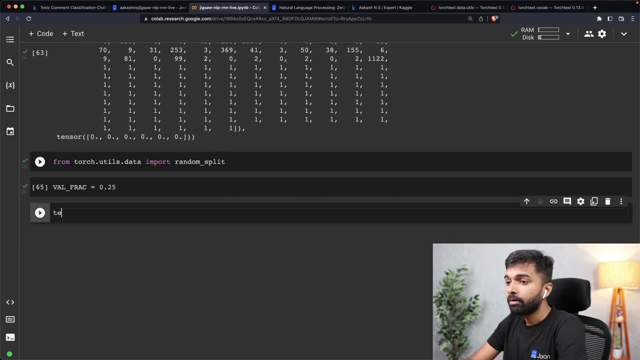 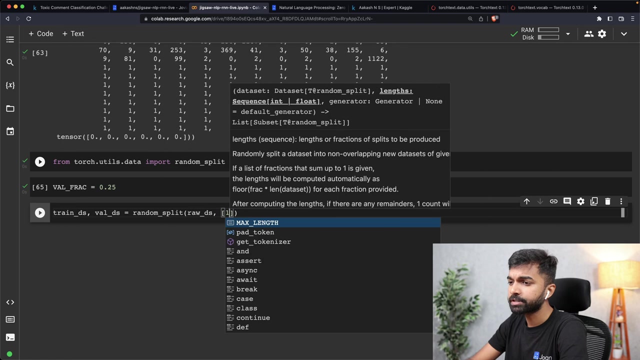 on data that it is not already seen. All right. So now we can create a train DS comma, while DS equals random split, And let's pass it the raw DS, raw data set, And we need to pass it the fractions. So the fraction for the train DF is going to be one minus val frac. 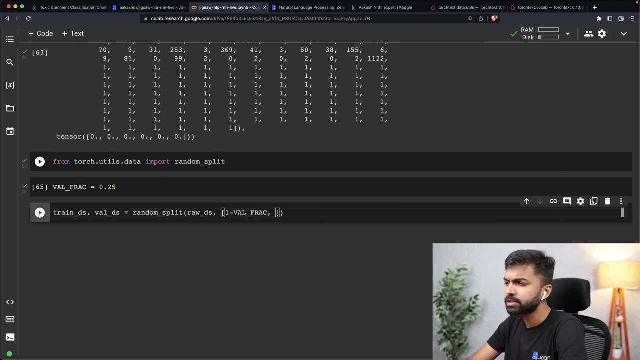 So we can either pass exact sizes or we can pass fractions, And I think we can just go ahead with fractions here, And the fraction for the validation set is simply going to be val frac. Okay, so 0.75 is going to go to the training data set. 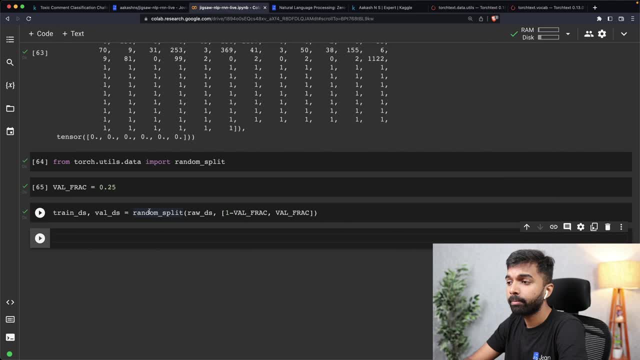 And the validation data set is going to contain about 0.25.. And now we can actually check the length of the raw data set, the length of the training data set and the length of the validation data set, And you can check here. 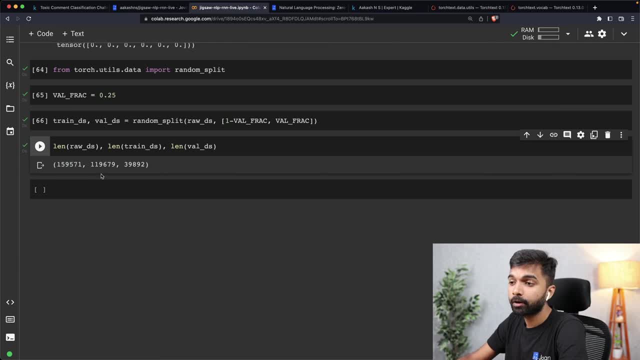 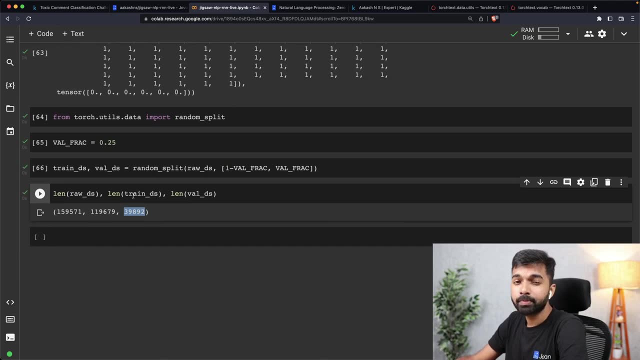 That 159,000 data points were present in the raw data set, out of which 119,000 have gone into the training set and about 40,000 have gone into the validation set, And that's how you split a training and validation set in PyTorch. 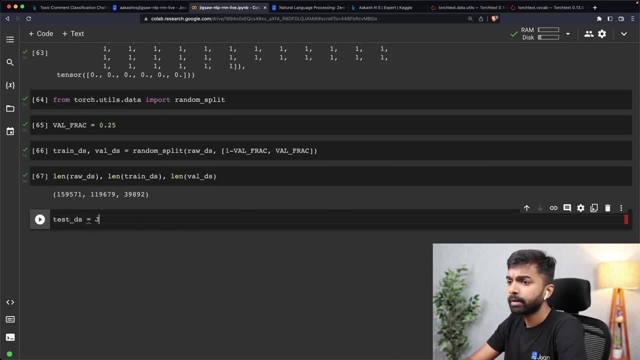 It's also created test data set. So I'm going to call it- and this is why we defined a class, because you're going to use it more than once. So jigsaw data set and let's pass it in. Let's pass in test DF. 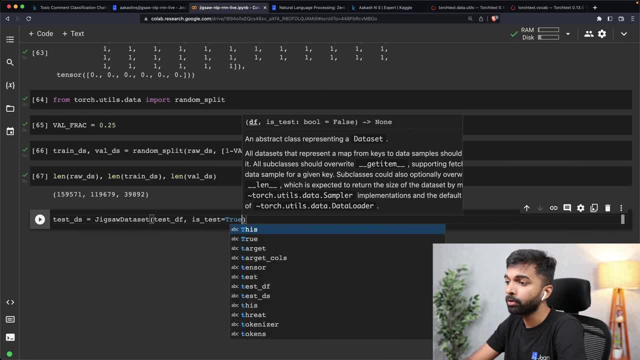 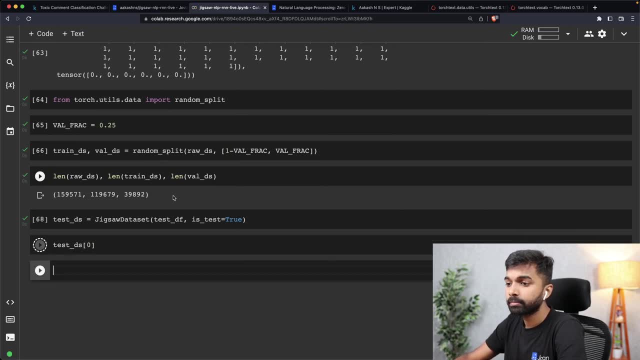 Of course let's set is test equal to, Because in the test data frame we don't have any targets. So when we say test DS zero, you can see that we get this data, and then this is going to just be all zeros. 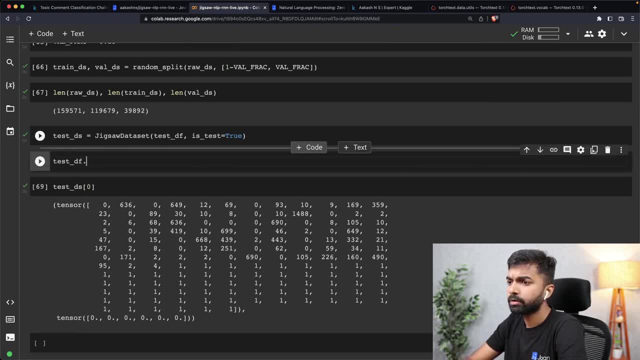 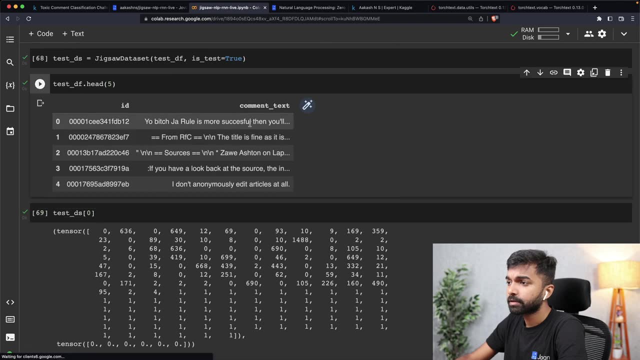 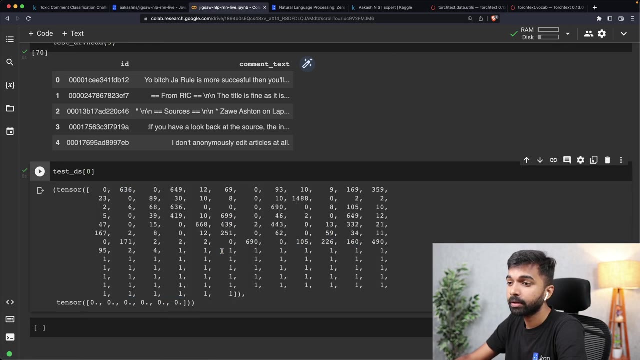 And, of course, this is simply the first row of the test data set. So this comment has been has been tokenized, then padded and then converted into indices Like this: All right, So now we have created a test data set as well. 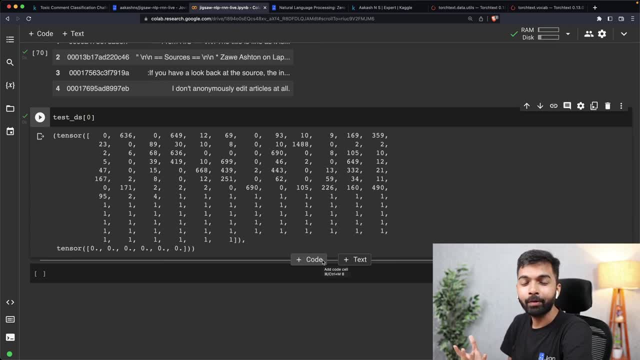 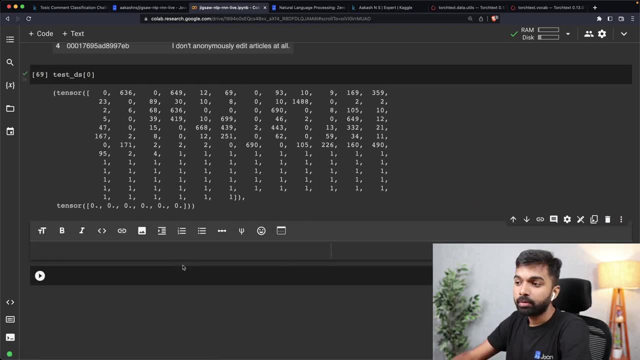 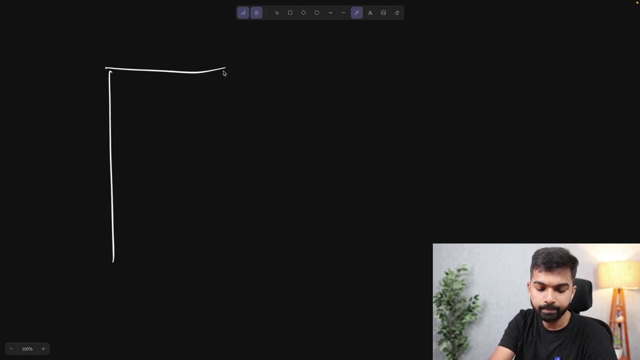 Final step, before we can actually start talking about recurrent neural networks- we're already one hour into the tutorial- is to convert these, is to create PyTorch data loaders. Now remember how deep learning books. So typically what we do is we have this data set. 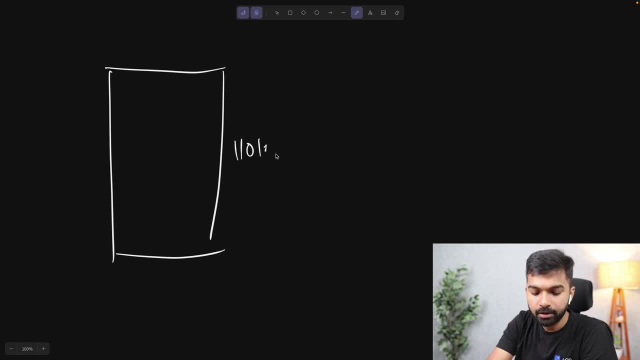 So in our case, the training data set contains, Okay, About 110,000 rules, but we can't pass all 110,000 rows of data into a model for training, So we have to split the data into batches And what we do is we pass one batch of data into the model for training. 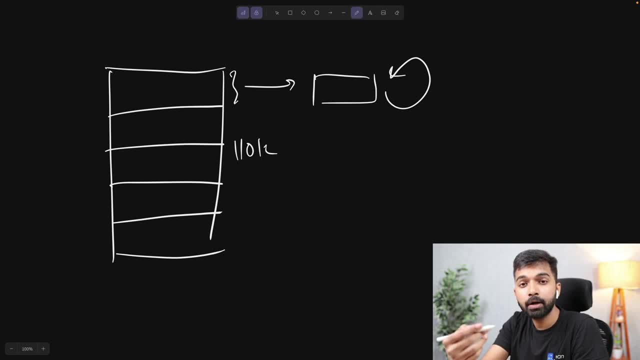 And using that we train the model a little bit, So the parameters of the weights of the model get a little better. Then you pass the second batch of data into the model And as we go through all the batches of the data, we complete one. 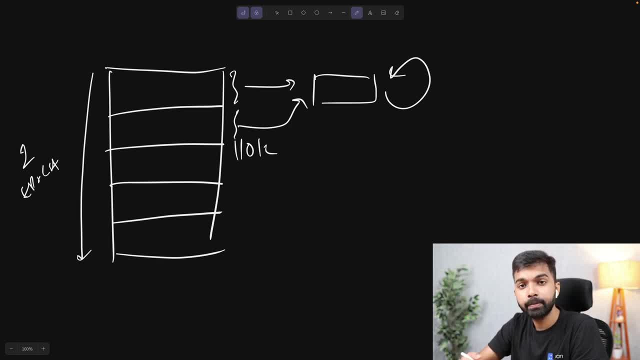 Epoch or one pass through the entire training set, And then we evaluate the model on the validation set And then we repeat for multiple epochs. All right, So that's how deep learning works. We split the data into batches, and the way you split data into batches in PyTorch is: 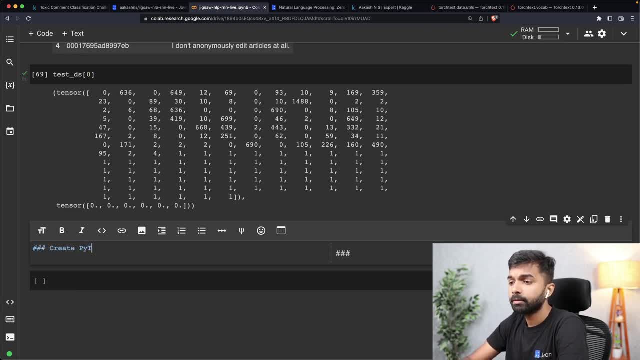 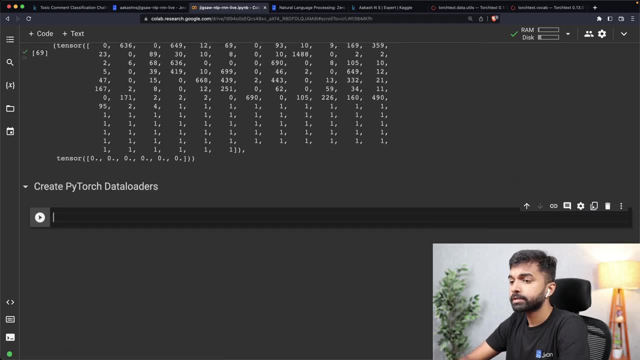 using PyTorch data loaders. So I'm going to create PyTorch data loaders here, All right. So from torchutilsdata Input: All right, So I'm going to import data loader and let's create a train data loader first. that is simply. 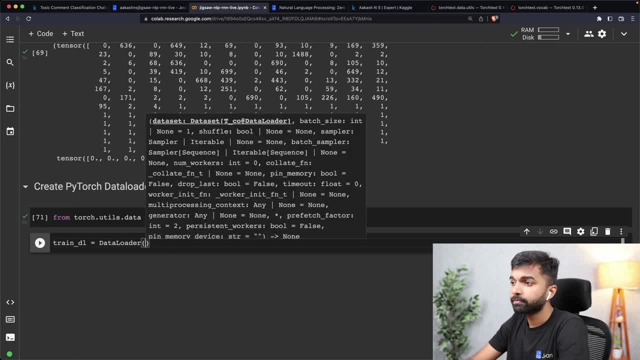 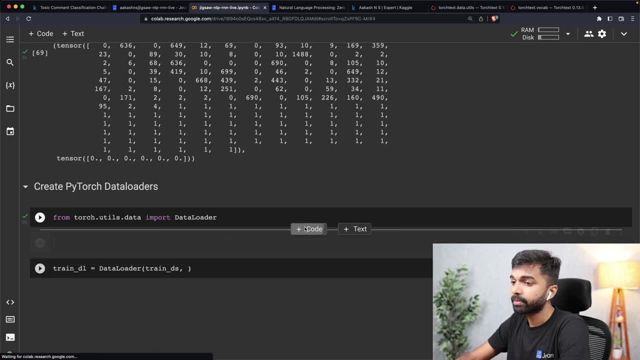 data loader, And what do we need to give it? So first thing we need to give it is a data set that is going to work with. So the data set is going to be trained DS. Then we need to give it a batch size. 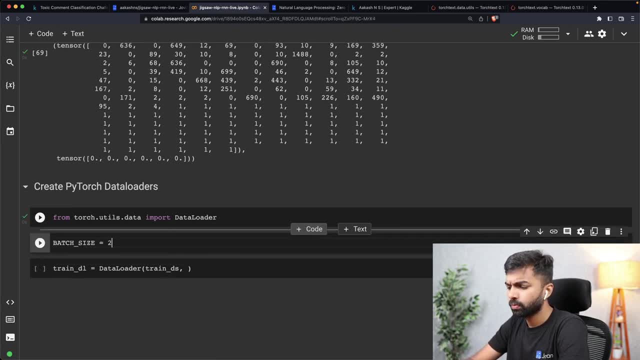 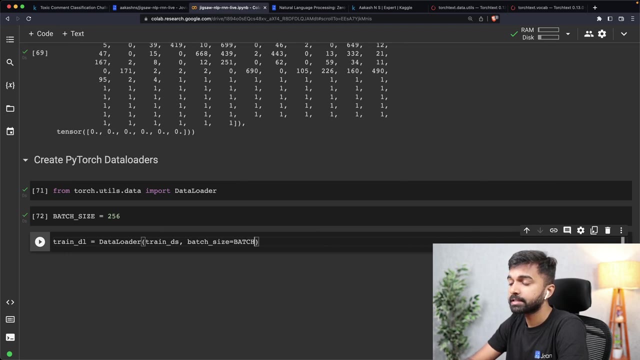 I'm going to set the batch size to 256, and I'm using 256 because I have a lot of RAM on this particular machine. but you can use a smaller batch size if this runs out of RAM on your computer. So let's pass. the batch size equals batch size. 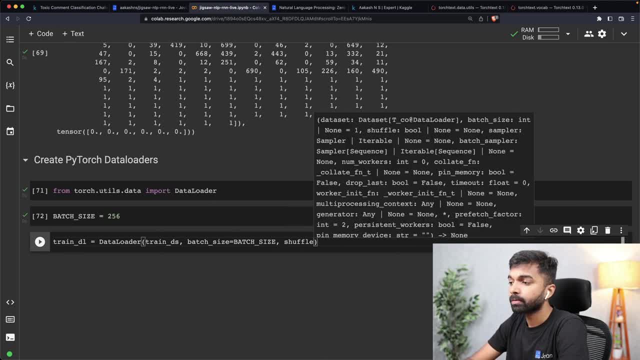 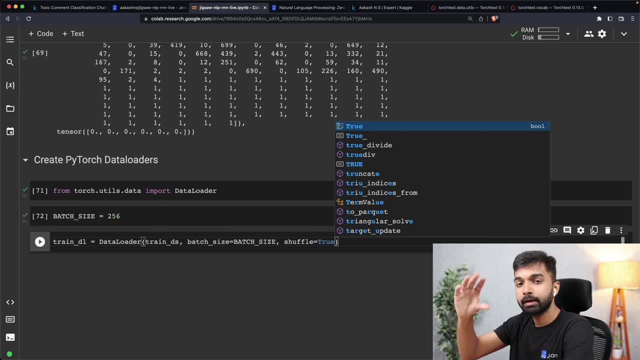 What else I'm also going to pass. shuffle equal to true. So when you're working with the training data set, it's a good idea to shuffle the data in each epoch And then that creates different batches of data or different sets of rows going into. 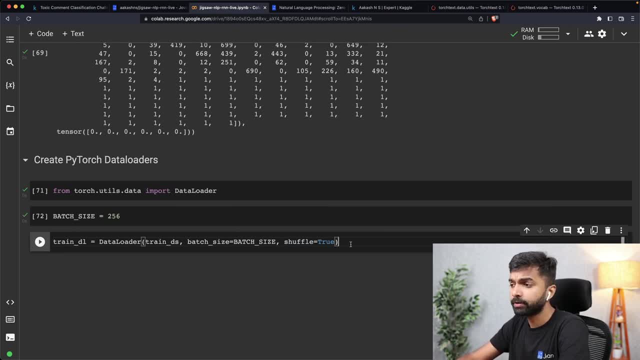 the training data set each time. I'm going into the model, each time for training. I'm going into the model each time for training. I'm going into the model each time for training. So it's always a good idea to add: shuffle equals true. 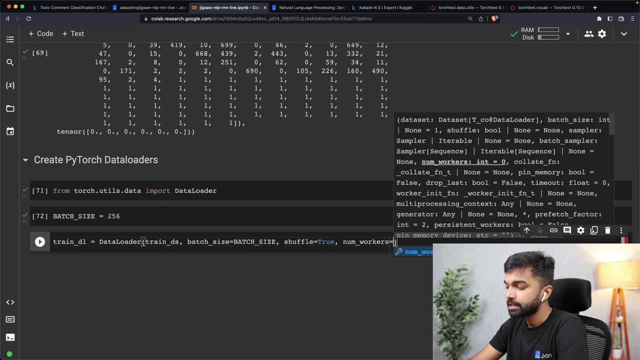 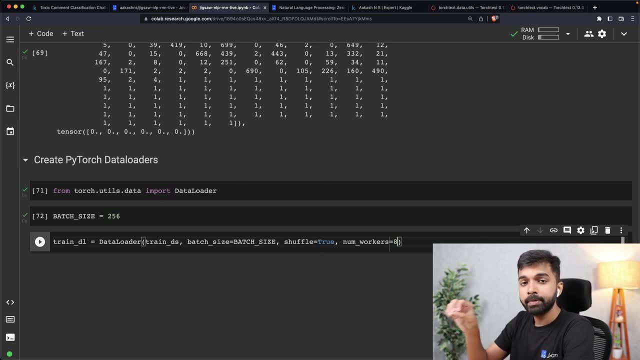 Then I'm also going to set up some parallel processing. So I'm going to pass num workers equals eight, depending on how many cores that you have on your machine. What you can do is, when a batch is being constructed, data can be fetched from the data set in parallel. 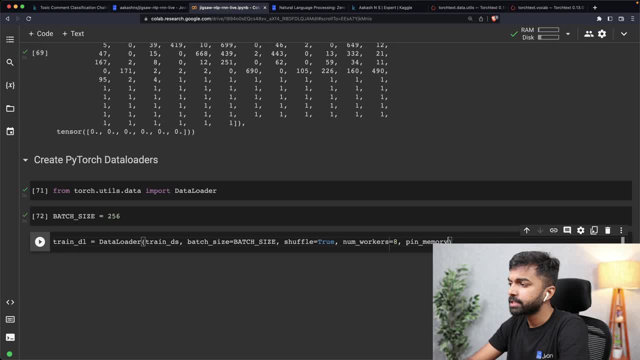 using many threads And a small memory. optimization is by setting pin. memory equals true, Okay, So that's the training data loader. Similarly, let's create a validation data loader. So that's again a data loader and I'm going to pass it: the Val DS, or validation data set. 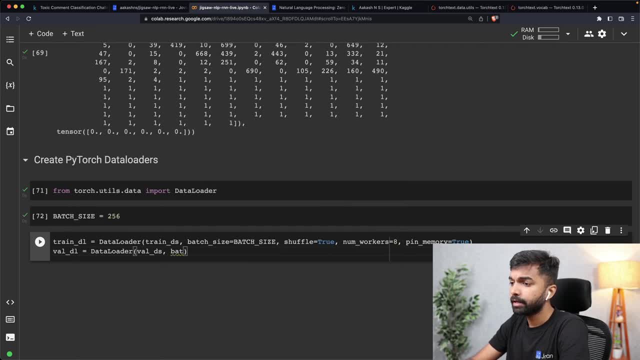 Batch size is going to be. now here's another trick for the validation and test sets: You can actually use twice the batch size, because when you're doing validation, you are not calculating gradients, And this is part of gradient descent is part of PyTorch. 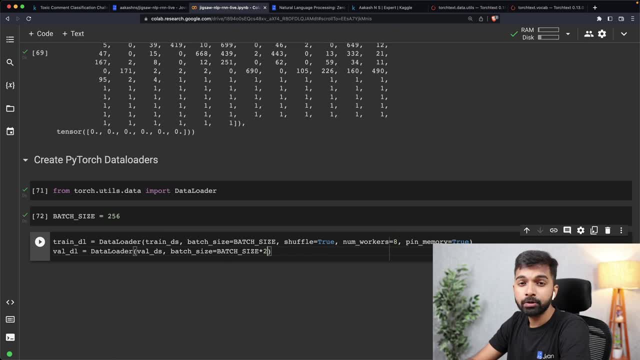 Check out our GAN score, Check out our course on deep learning, because you're not calculating gradients, You have more memory And you can use that to just double the batch size and you don't need to shuffle it, because we just want to evaluate the model. on the validation set, 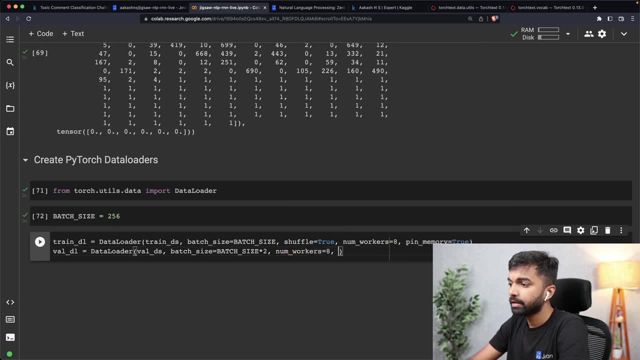 Shuffling is not going to change anything, but num workers equals eight and pin memory equals true are still going to be useful. Finally, let's create a test data loader as well. So data loader test: DS: batch size equals batch size into two. 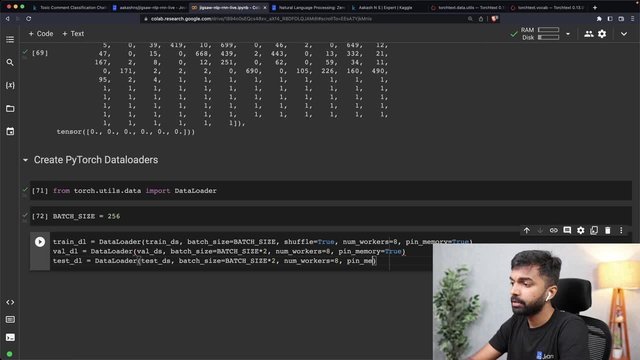 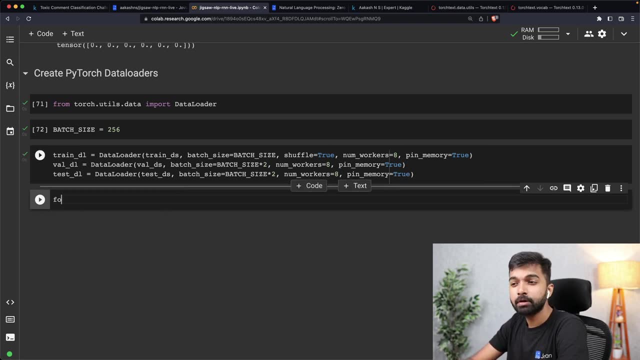 Now we have a data loader and this data loader is typically used in a for loop. So I could say something like for batch in train DL. and now it could say: like batch inputs, batch targets equals batch, So the batch is a tuple containing inputs and targets. 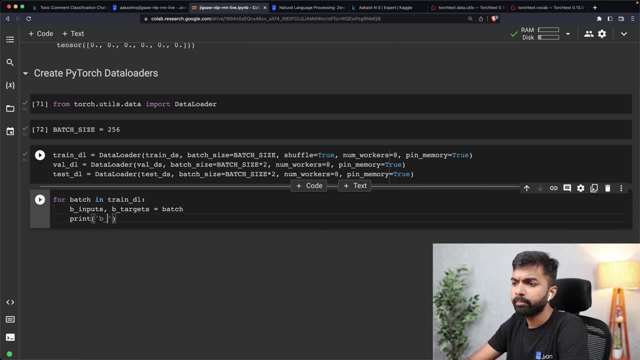 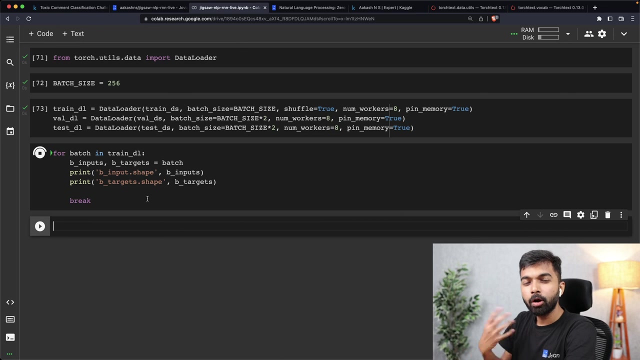 And then I can simply print Print out B- inputs- dot shape and print B in targets- dot shape. And I'm just going to print this information for one batch just to see whether data is going to be generated properly or not. It's always a good idea to just test out what you've done to check the shapes and things. 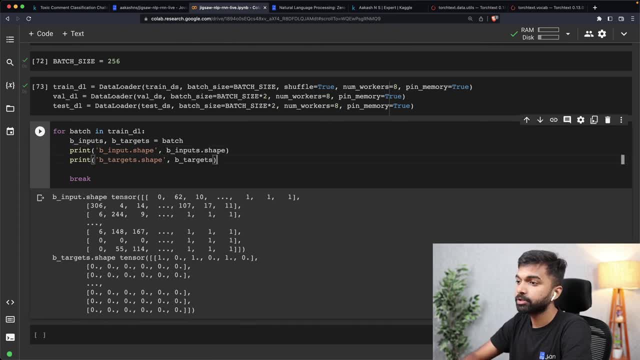 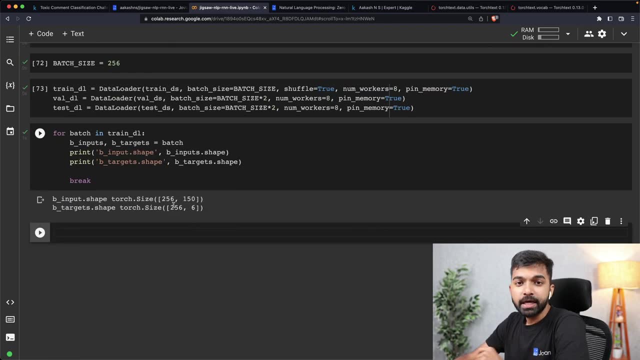 like that. Okay, So I've printed the shape. So let's call it dot shape here. Let's call it dot shape here as well. So there you go. We have set the batch size to 256.. And remember, we have set the max length to 150.. 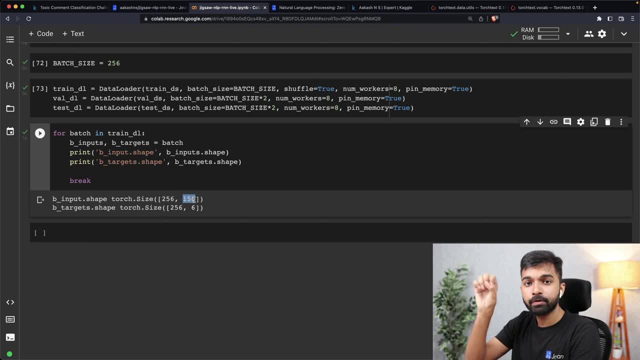 So what's happening is 256 rows of data, which means 200 quarter, and 56 comments are picked randomly from the training data loader after a random shuffle. So the first batch, which is the first 256 comments, are picked from the training data. 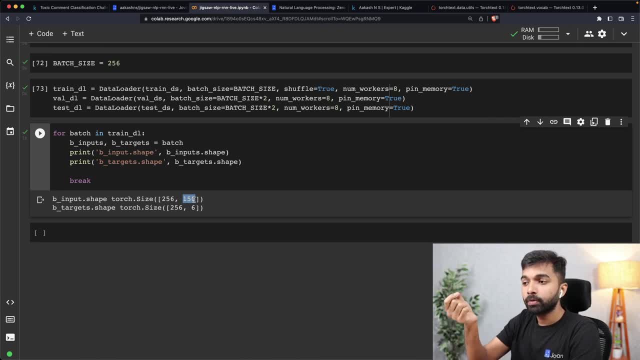 Then those 256 comments are converted into tokens and then into indices, And of course we have set the max length to 150.. So that's why, for each comment, we get a vector of length 150 containing the indices of every word in the vocabulary, every word present in the token. 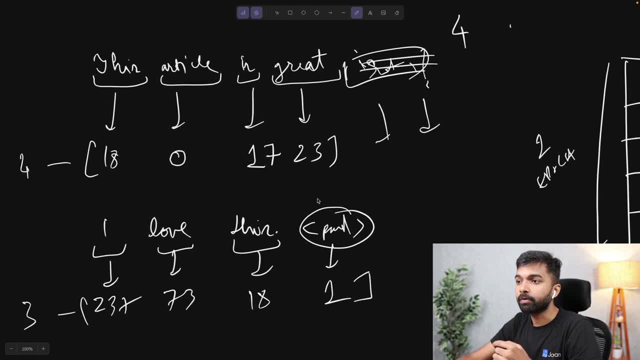 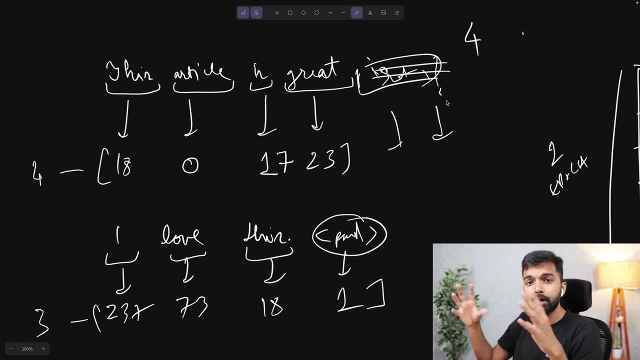 So one thing you should keep in mind here is, unlike things like bag of words, here we are actually maintaining the order of the Tokens. We have not converted or summarized the sentence into a single vector. We are actually maintaining the order of the tokens. 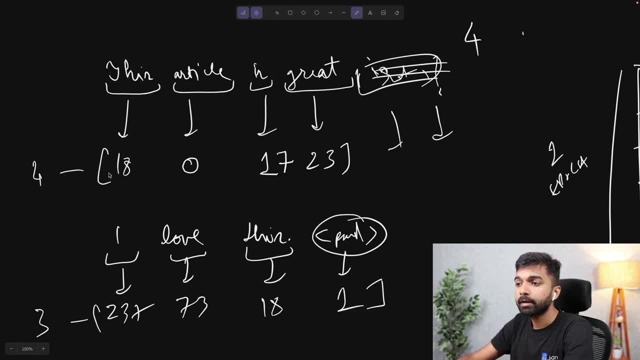 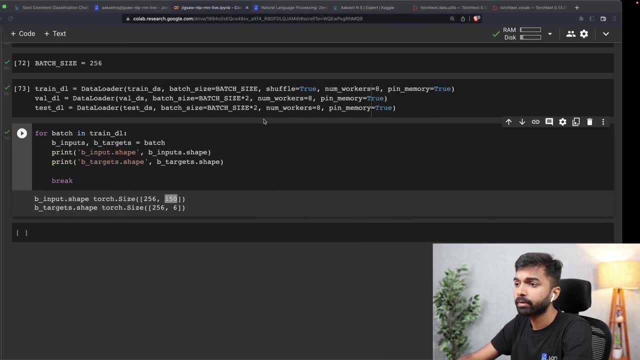 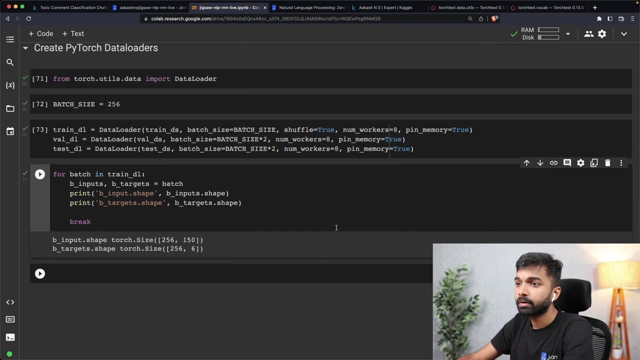 All right, So each comment gets turned into a list of tokens and we can actually recover the sentence largely from this list. All right, And of course for each of those comments in the batch we also have six target values. So now we've created pytorch data loaders. 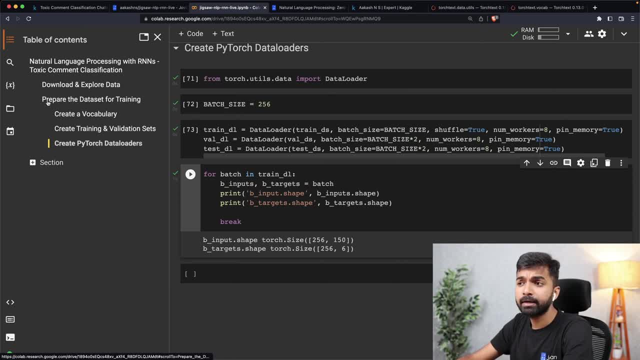 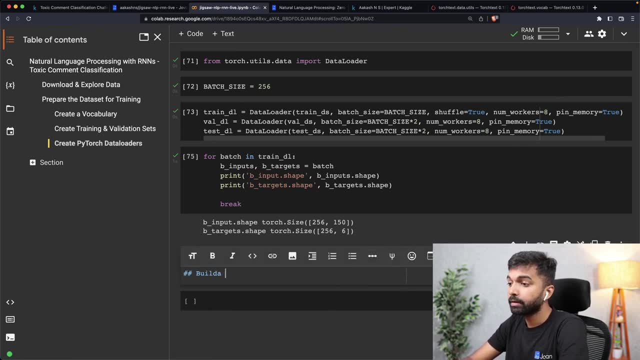 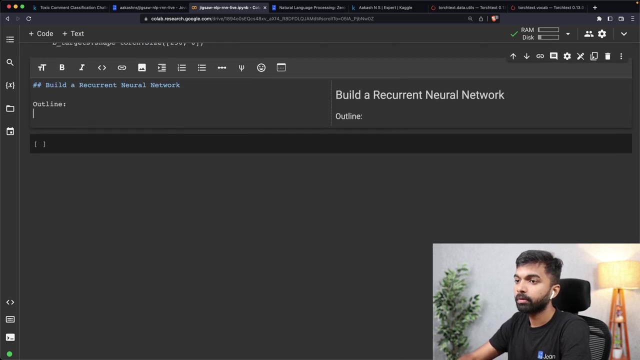 Okay, And with that we have prepared the data set for training Next up. next section is to build a recurrent neural network. So how are we going to do this? Let's write an outline. first step is to understand how recurrent neural networks work. 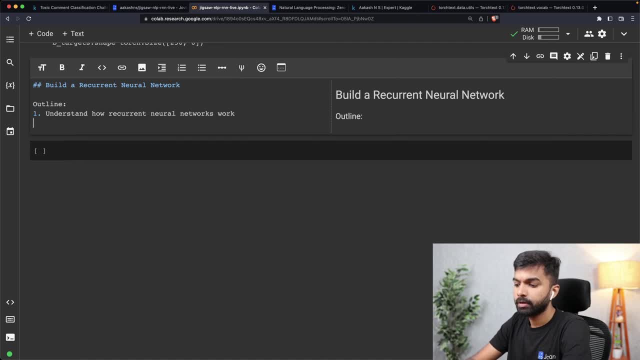 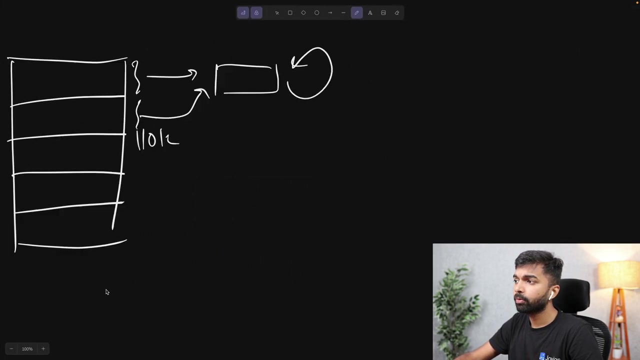 Second is to create a recurrent neural network, And then the third step is to pass some data through the network. All right, so let's do that. Let us switch back into the whiteboard. Okay, Now, if you're familiar with some, 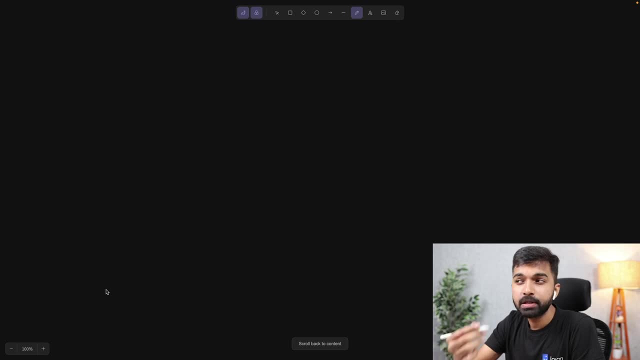 Classical NLP techniques like bag of words. This is how they work. First let's say I have a comment, I like this movie. What we first do is tokenize it And then we convert these token indexes. So three, seven, 2319.. 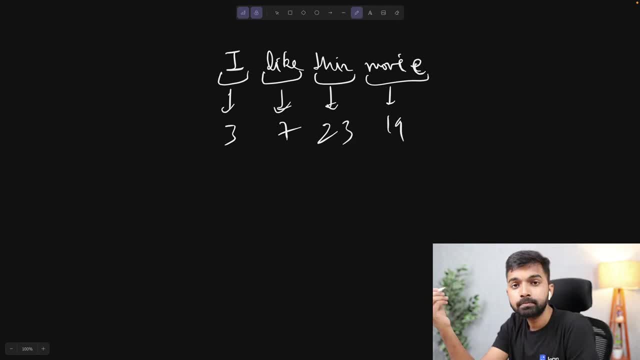 And now- and this is where the difference comes in- from bag of words versus recurrent neural networks. So on the left, we are going to study the bag of words approach. On the right, we are going to study the recurrent neural networks approach. 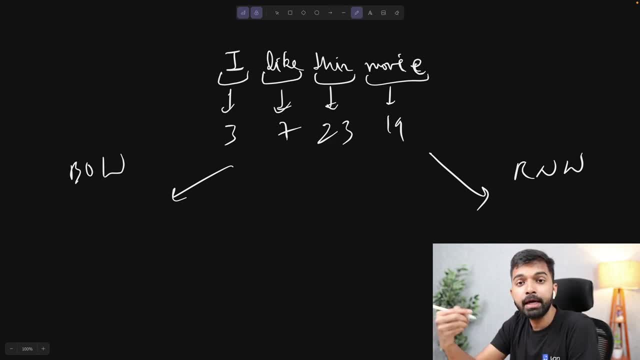 Now, in the bag of words, what we do is we already have a vocabulary right. We have a vocabulary like a and the, et cetera, et cetera. So there are a bunch of tokens in the vocabulary that have been learned by looking at the data. 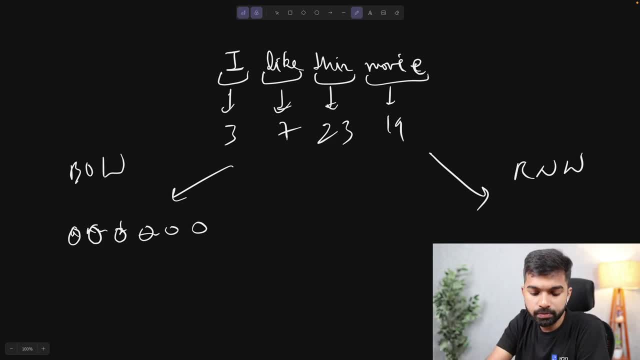 Okay, We have a data set And what we do is we convert this sentence, the sentence that we have- I like this movie- into a frequency table, essentially right. So our sentence I like this movie, let's say this- is that sentence gets converted. 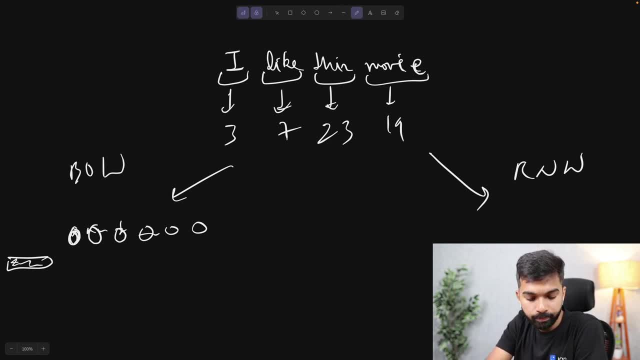 So we count, Okay. Or vocabulary item Number one: What? how many times does it occur? It occurs zero times. vocabulary item Number two: how many times it occurs One time? vocabulary item Number three: it occurs four times. 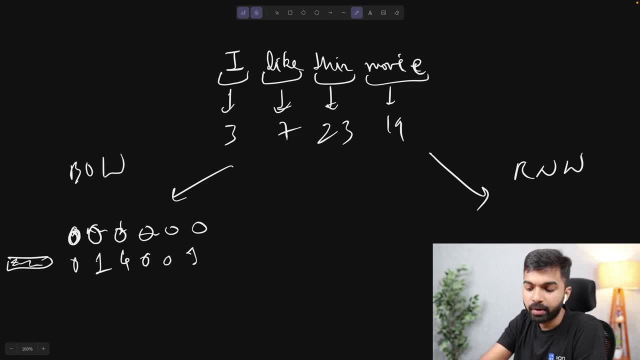 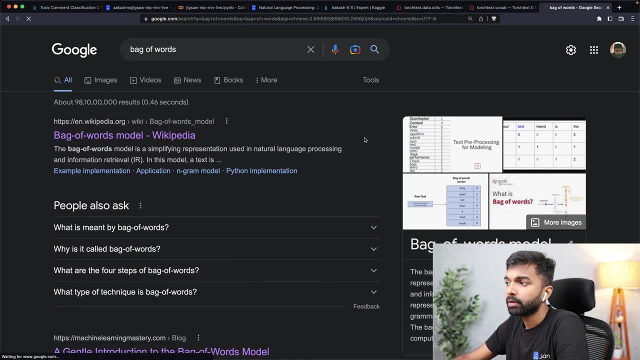 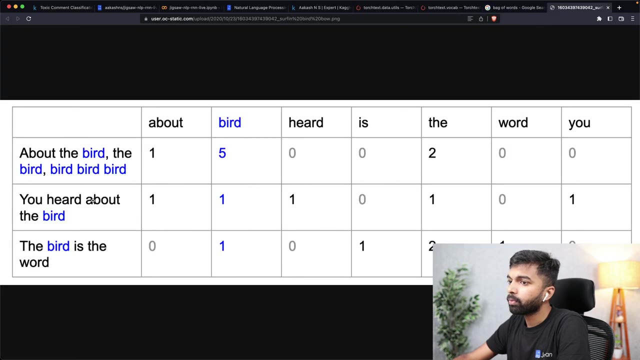 It occurs zero times, Zero times, Right? So I encourage you to check out the bag of words model, and you can always, of course, Google it. So what we do in the bag of words model is we turn each sentence into a vector, and this: 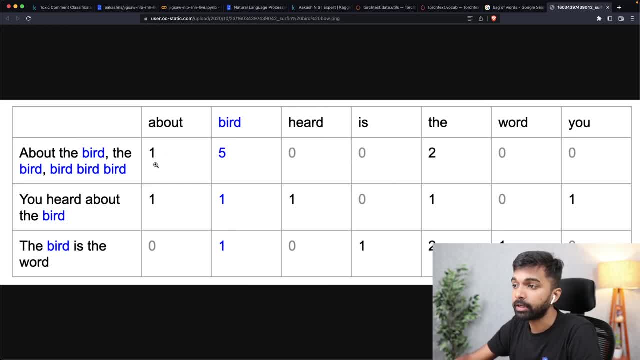 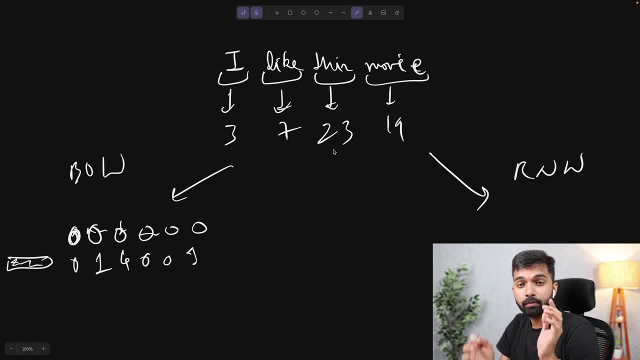 vector contains the frequencies of each word in the vocabulary: one, five, zero, two, zero and so on. Okay, So each. Okay, We turn into a vector containing frequencies of vocabularies. Okay, So this is what we use in the bag of words. model. 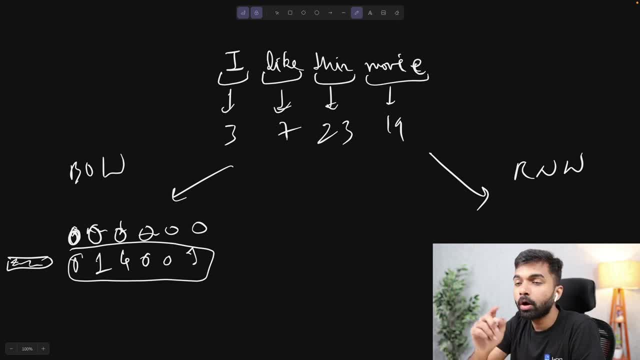 On the other hand, when we are using RNNs, we do not convert the entire sentence into a single vector. rather, in RNNs We have in order, the tokens, the indices of the tokens that are present. Each of these tokens is converted into a vector. 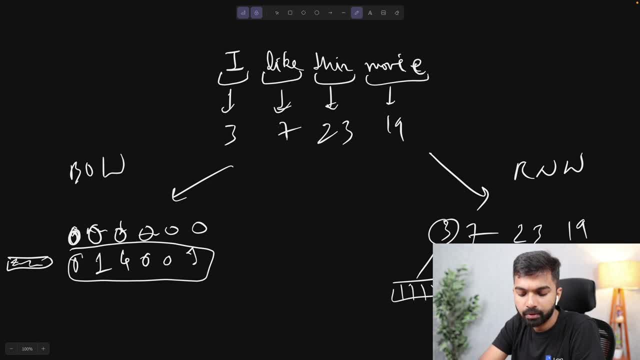 Okay, Okay. So in the bag of words the entire text is converted into a single vector by looking at the counts of the words or counts of the different items of the vocabulary in that text. But in RNN the text is converted into a list of token indices and then each of those tokens 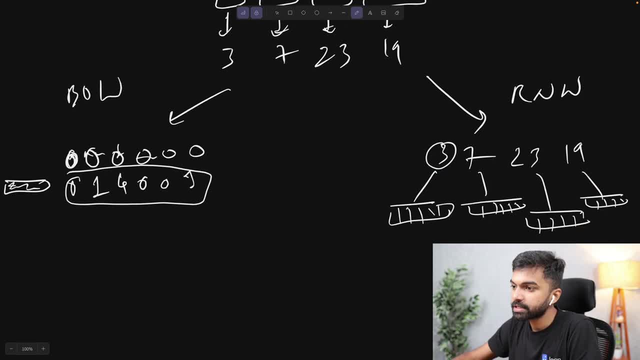 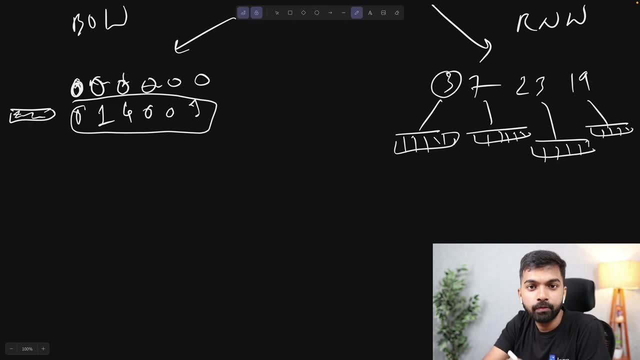 is converted into a vector. Now This is where things start to get interesting. So we have bag of words and we have RNN. how we process a bag of words Input is: we use these neural networks. So we have a NN, dot linear and we pass it in. 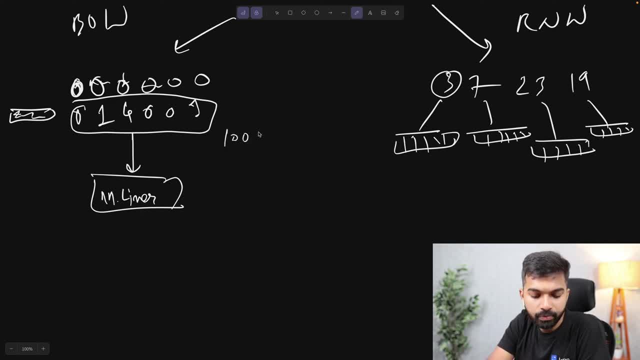 And let's say you start with a vocabulary- size of thousand. So each input variable is going to be of size thousand, or each input row is going to be a size thousand, a vector of size thousand That is going to then get converted into maybe let's say you're going to reduce it. 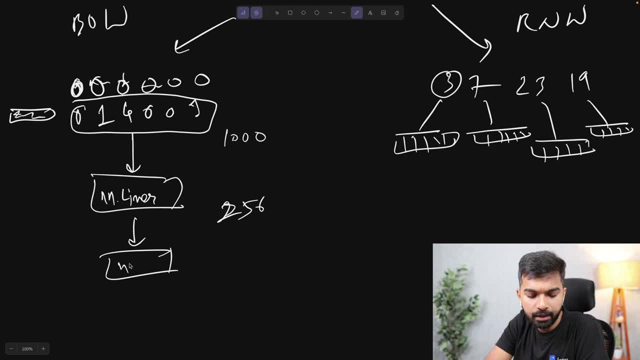 down to 256.. And then you're going to pass it into another NN, dot, linear, And then maybe, let's say, we're going to reduce it down to 64.. So you, you start with tokens or vectors of length thousand, you reduce them to a length. 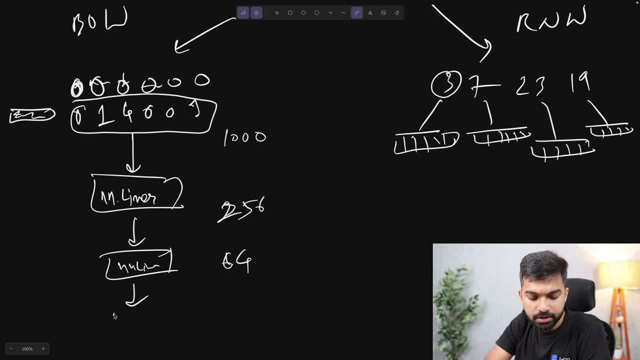 256, reduce them to length 64.. And finally, because the final output is six, you want to predict six classes. you reduce that to six. Okay, So you just sequentially Pass This Entire vector at once through the model. 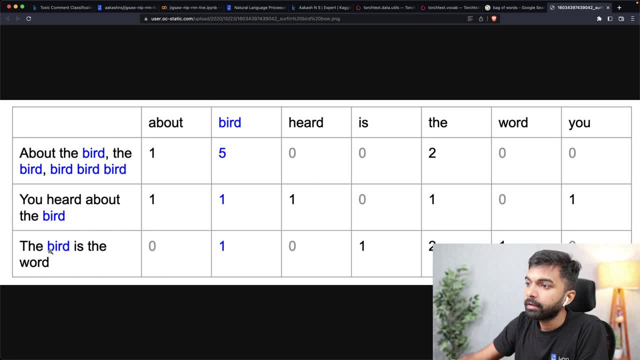 Now the problem in bag of words is that information about order is lost, about the bird, the bird, bird, bird, or you heard the bird gets converted into this vector And in this vector we simply have counts of the different items of the vocabulary. 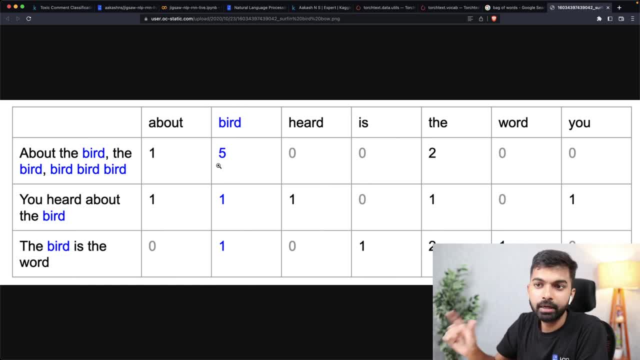 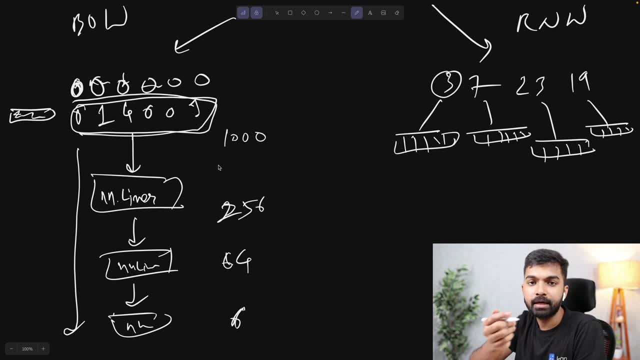 We don't have information about which word comes after which one right. The order of the words is lost. On the other hand, in a recurrent neural network, the order of the words is maintained. but how do you actually train the model? 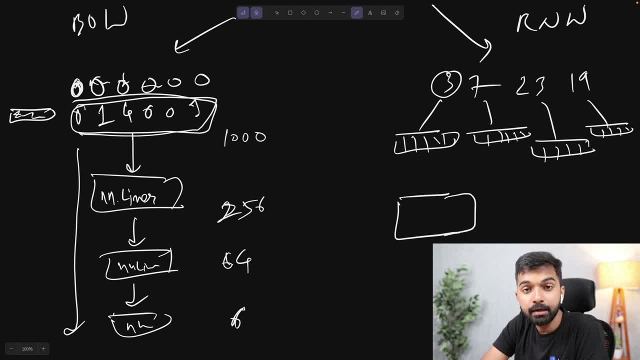 So here is how you train the model. You have this recurrent layer, So this recurrent layer is called NN dot RNN recurrent layer, And the way this recurrent layer works is you pass the first word into it. So you pass the first word and the first word itself. each word has been encoded, or each. 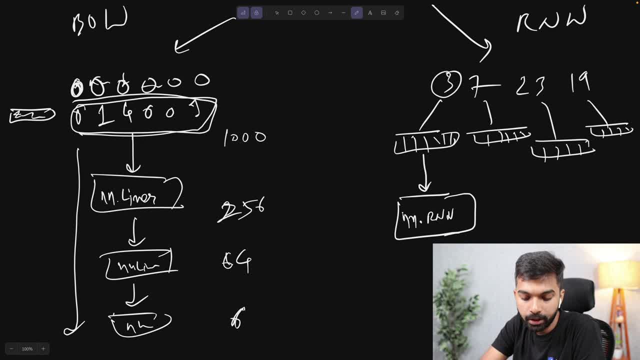 token has been converted into a vector, So you pass the first word into it and you pass a hidden state called H zero, some hidden state, initial hidden state- And the neural network or the recurrent layer returns two things: It returns an output or zero and it returns a new hidden value, H one. 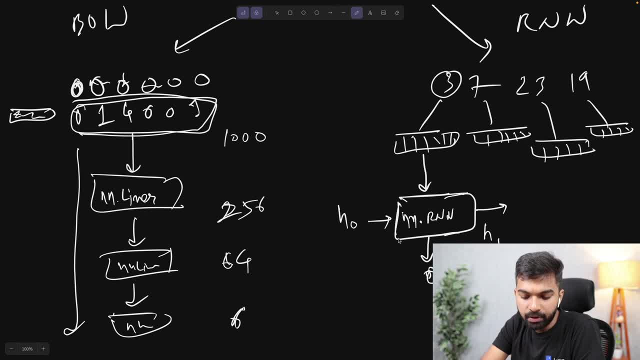 Then you take the same, you take this exact same layer and you take H one and you pass H one into that layer, right? So we're still? we're not using a new layer, We're using the same layer. So it's like a four loop essentially. 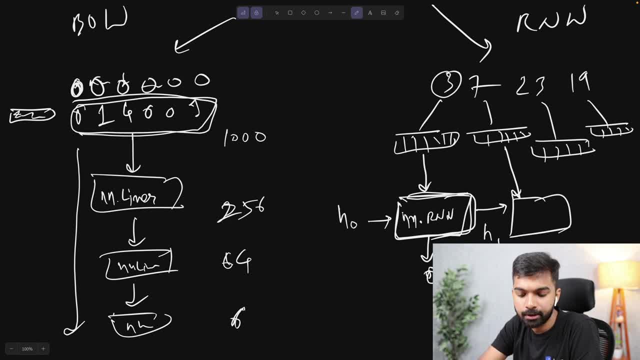 So you take H one and pass it into the layer, And then you take the second word. You can pass it into the layer NN, dot, RNN, and it returns the second output- O one, Okay. And then you do this for the third one and it returns a third output- O three. and then 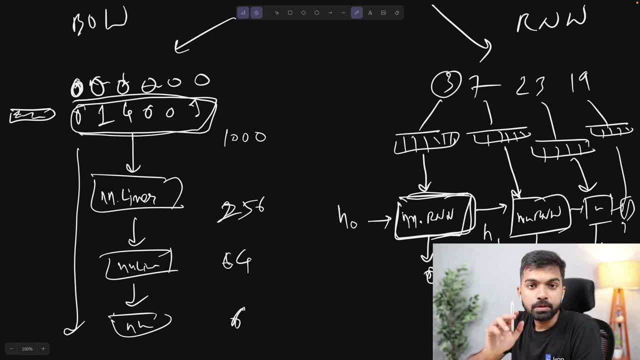 do this for the fourth one, and so on. So what's the difference here? First thing: instead of converting the entire, converting the entire text into a single vector, you convert each word into a single vector. Okay, So you have 150 vectors. or you have 150 vectors because each text, each comment has been converted. 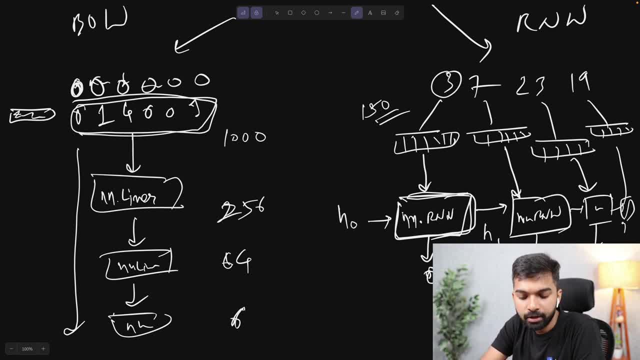 into length one, 50, because that is a max length. we have picked now 150 vectors. The first vector is passed into the recurrent neural network. that returns an output, returns a hidden layer. Then the second vector, the second word vector is passed, and so on. 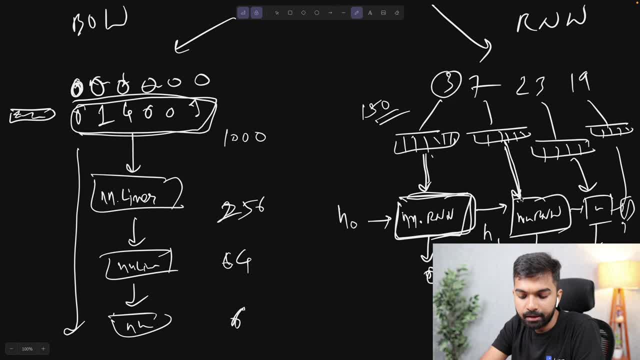 This maintains order. When you are passing the second word vector into the recurrent neural network, it has information about the hidden state. So about the first vector and everything that has come before it because of the hidden state. All right, And finally, what you can do is at the end of your training, you can either use all the 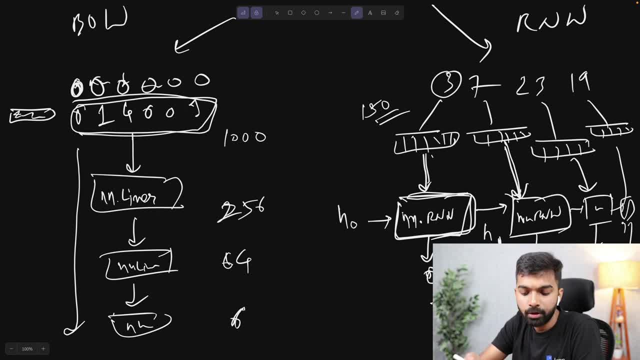 outputs, or you can only use the final output. that's up to you. But now you have more information about the order in which things were passed. Okay, So couple of nuances here. I just want to point out is that we take this word: embedding. 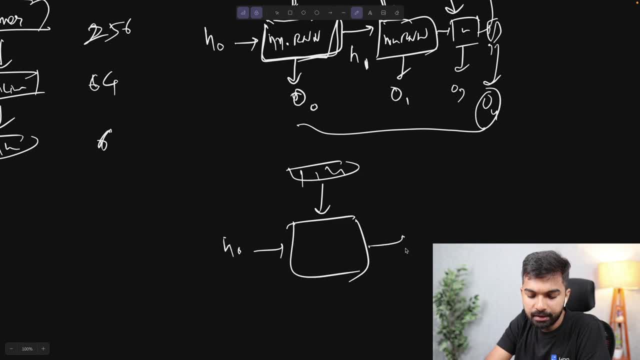 and then we pass it into the model And it takes a hidden state and then it gets an H one and then it returns a output zero. What we do is we take the second word and pass it into the exact same layer And now, instead of H zero, we pass S one and that gives out. that gives out one out one. 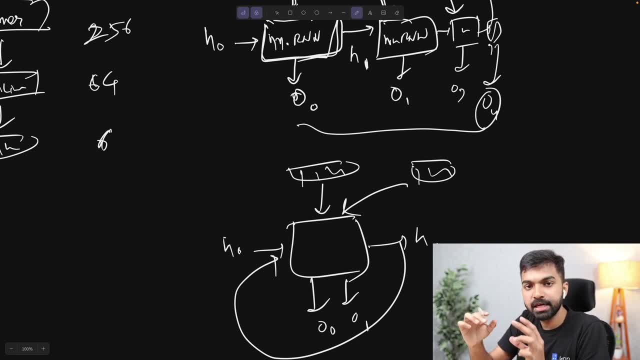 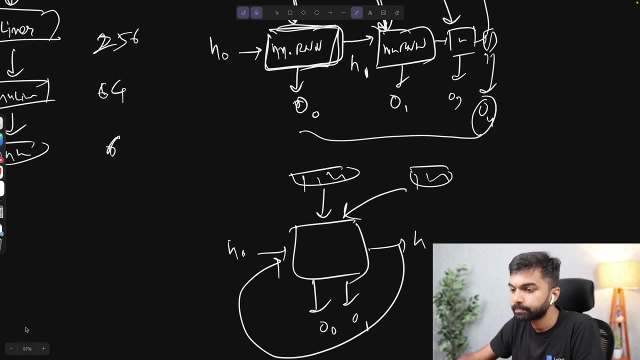 All right, So it's the same, is the same node, It's the same layer into which we are passing it one by one: H one or one, H two or two, and so on. Then the second thing I want to point out here is we have something called an embedding. 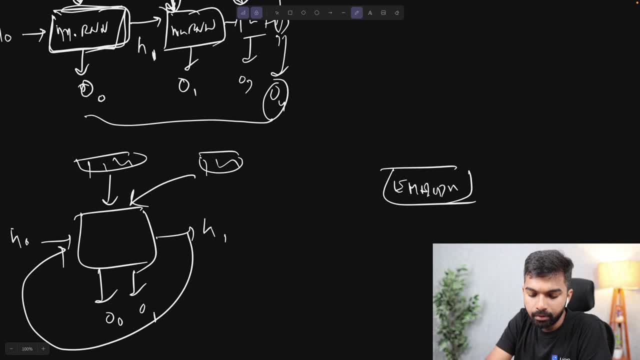 layer which is actually going to take the words. So let's say: you have, I love this movie. excuse the bad handwriting. We convert that into tokens three, seven, 10,, 11, then the embedding layer three is going to get passed into the embedding layer. 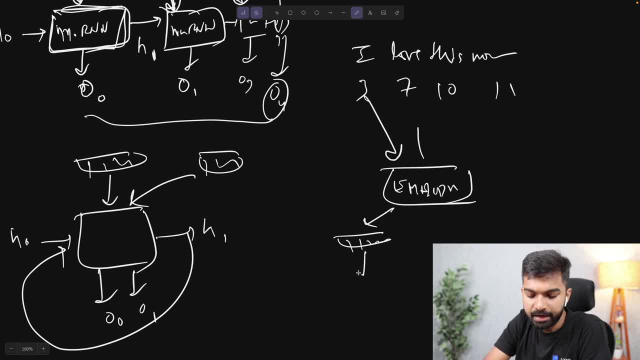 It is going to emit the vector and that is going to get passed into the model. That's going to return a hidden output and an output in a hidden layer. Then seven is going to get passed into the embedding layer And that's going to return a vector and that is going to then get past into recurring network. 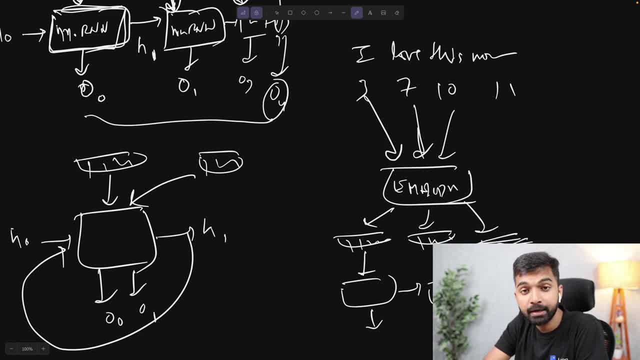 and then 10 is going to get past, that is going to get the embedding layer, is going to return the vector for it, and that is going to pass. And then 11 is going to get past as remove to return the vector, and so on. 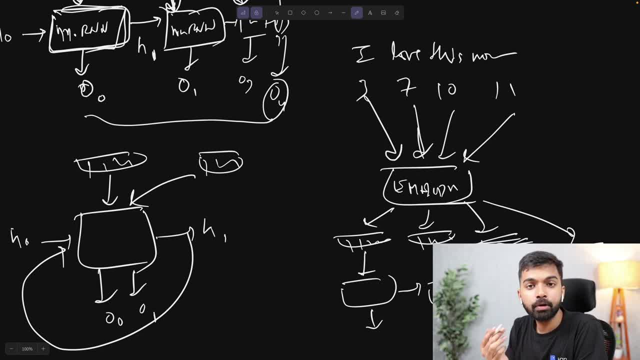 Alright, So we have, before any recurrent neural network layer, we always have an embedding layer, and how are the Well values for the different vectors decided? So how do the word vectors get decided? Well, that's the interesting part, that the word vectors are also. 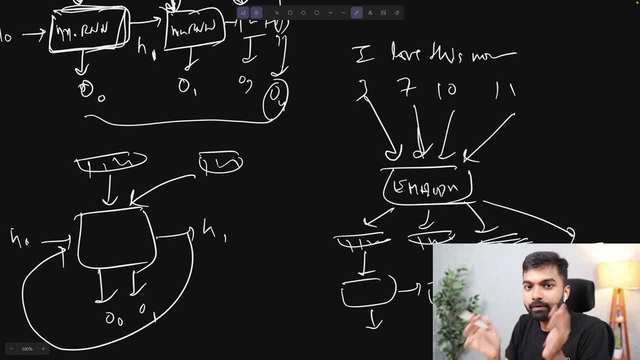 learned by training the model. So instead of us defining that we have to create the vectors in a certain way, we just create a matrix internally And we make that a part of the model and we pass it through the recurrent neural network. we get a loss of course. after all this, we're going to use a linear 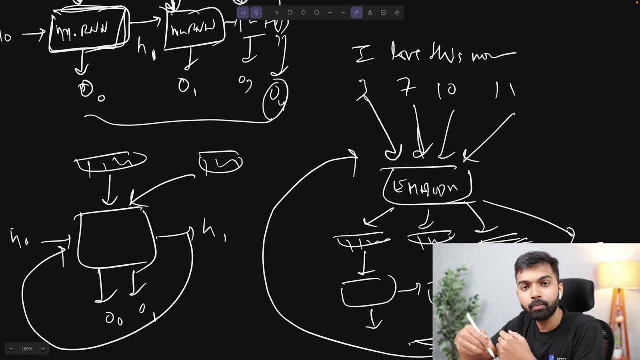 layer and we are going to get a loss, and then use that to change the weights of the model, and then your embedding is going to get better, Your recurrent neural network is going to get better and your entire result is going to get better. Okay, 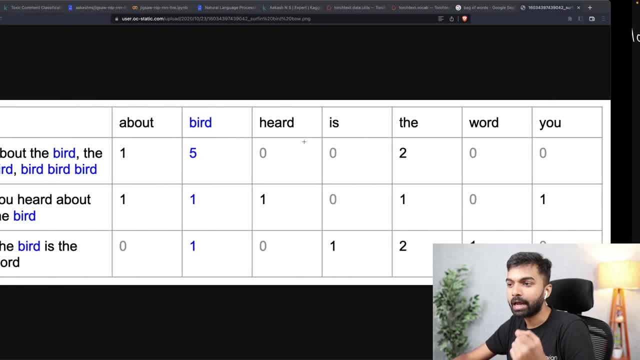 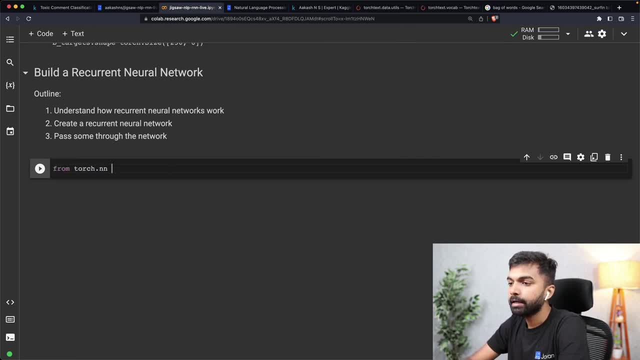 So that was a quick introduction to how recurrent neural networks work And as we see it in action, as we see the code, things will become a lot more clear. So let's do this from torchnn, Let's import torchnn as nn. 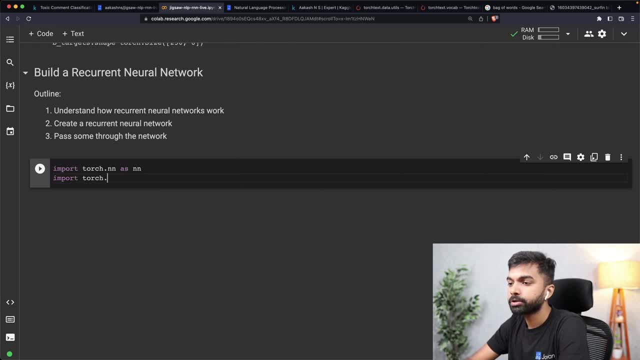 And let us also import torchoncline, All right, Okay, So now we are going to. well, let's see if we have any questions at this point. Okay, I don't see any questions, so that's fine. Yeah, I think we're doing fine here. 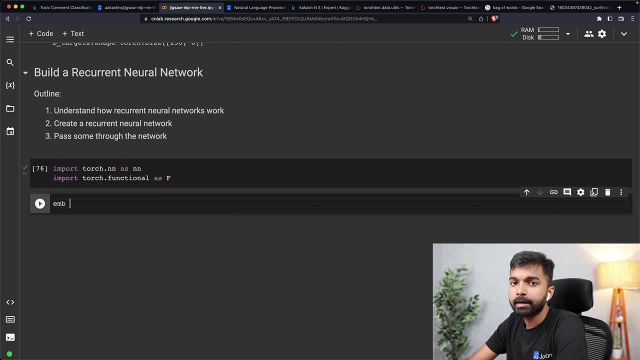 All right, So now, let's first create an embedding layer. So let's create a layer called EMB, and EMB is simply going to be nnembedding. Now, nnembedding requires the number of embeddings, which is basically the vocabulary size, and let's just call it emb layer, just to be clear that this 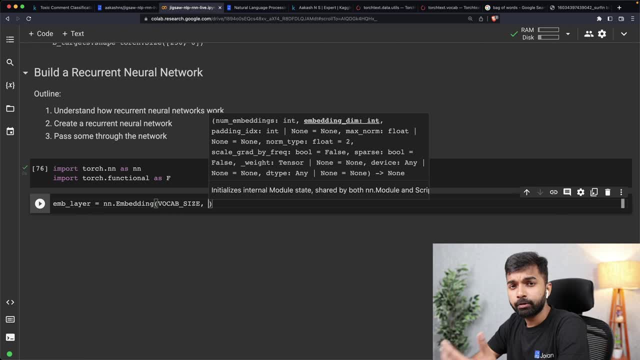 is a layer in a neural network. We're not creating the neural network yet, We're just looking at individual layers. and then it also requires the dimension or the size of the vector for each one. So let's create vectors of size 256.. 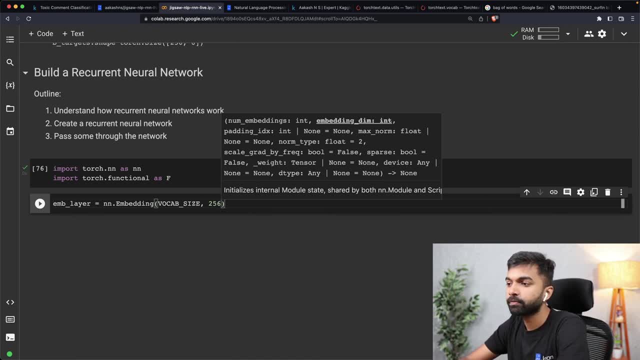 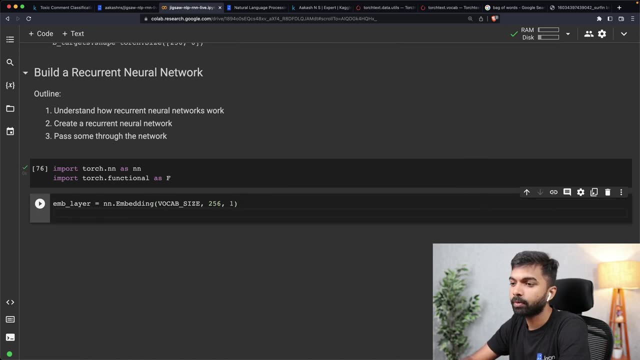 So each word is going to be converted into vector of size 256.. Okay, That's fine, And it also requires the index of the padding token. So the padding token is at index one. We can actually verify that. So we can say vocab pad token and it has the index one. 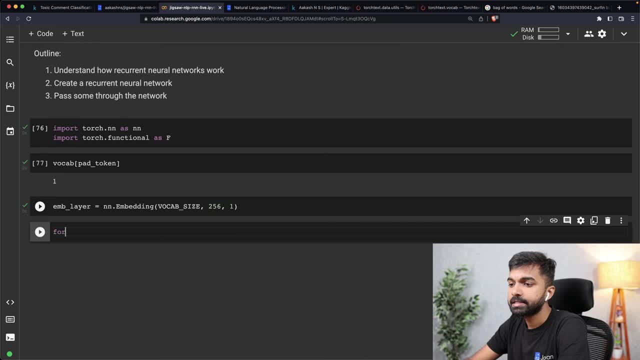 Okay, So that's the embedding layer and let's say: or let's get a batch from the training data loader for batch in train DL. I'm going to just look at one batch- the B inputs and B targets equals batch, And I'm going to- I'm just going to print information about these. 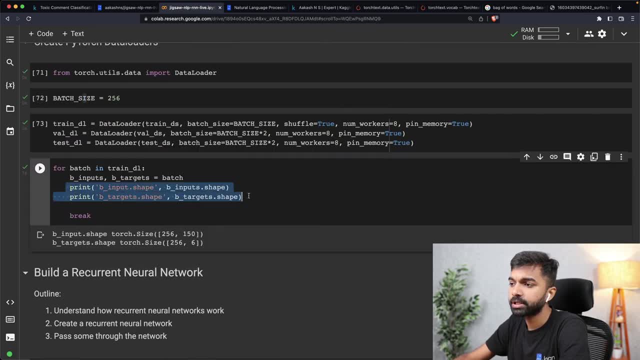 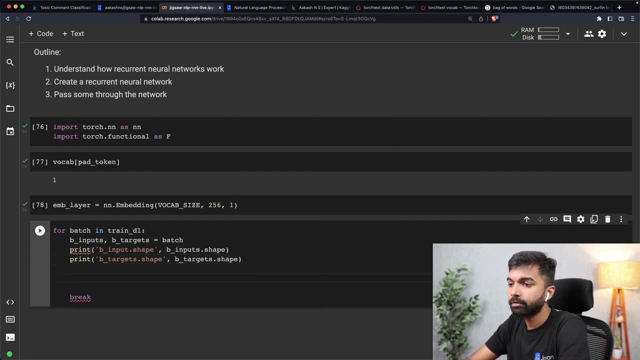 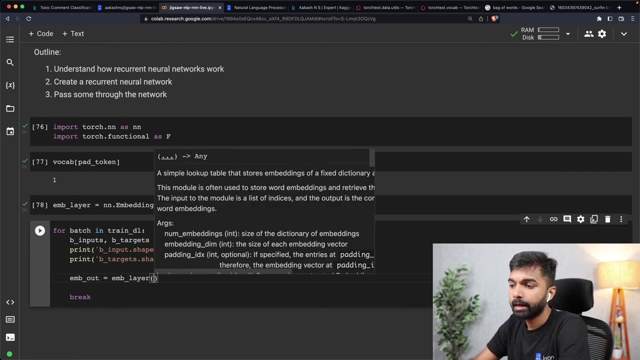 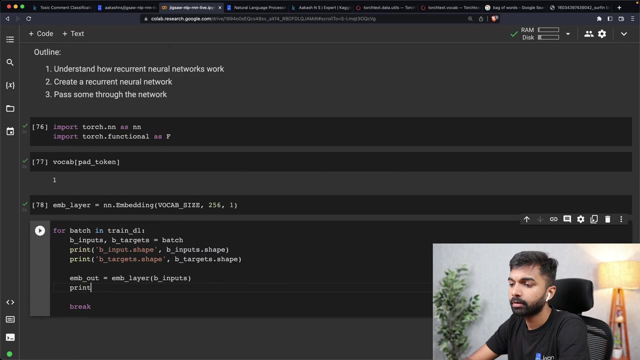 So I'm just going to copy that information from here. So yeah, B inputs or shape, B targets or shape, And now I am going to pass this into the embedding layer. So EMB out equals embedding layer. And let's pass the B inputs and let's just print out: EMB out- dot shape. 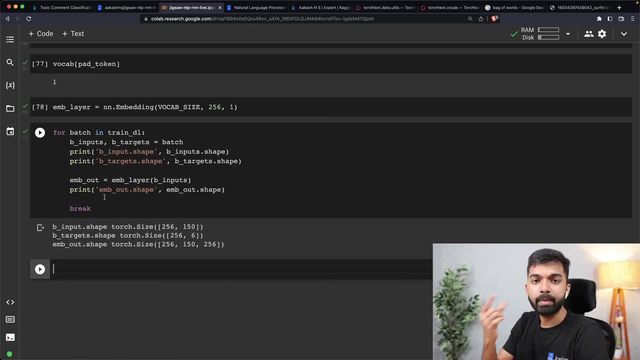 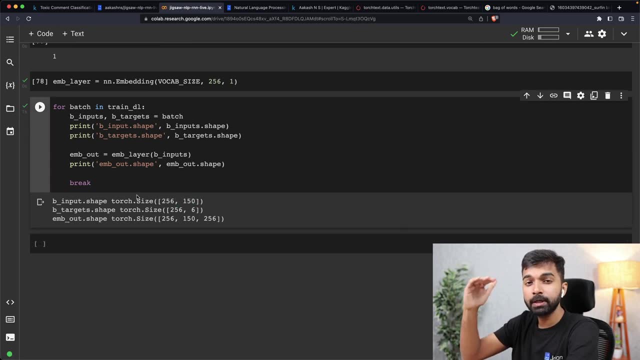 Okay, So let's see what happens here. What happens when we actually pass a batch of input into the embedding layer. So the input has the shape Two. We've 156 comma one 50, which means there are two, 56 rows in the batch. 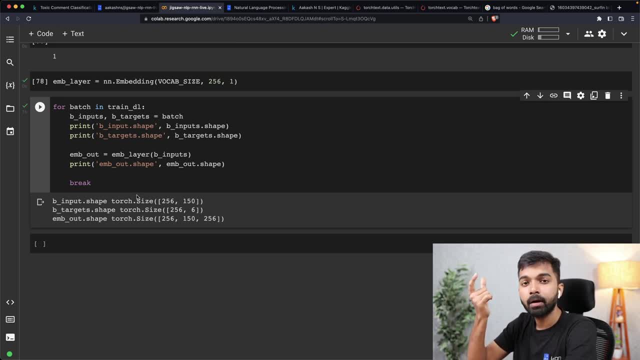 Each row in the batch contains a vector of size one 50. This vector is simply the indices of the tokens present in that comment. Then we pass the batch into the embedding layer and we get back again to 56 outputs. But now this vector of size one 50 has been converted into a. 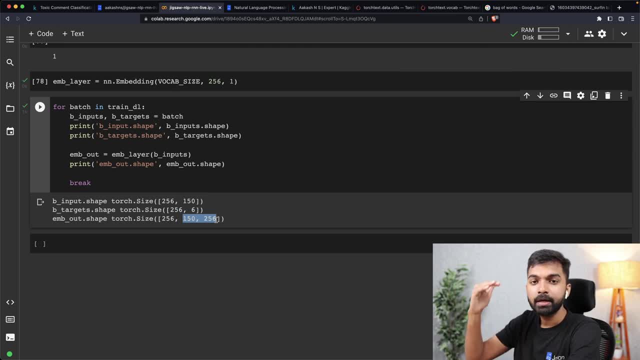 matrix of size one, 50, by two- 56.. So what has happened Is that the embedding layer has taken each of the indices of the tokens present in the common text and it has converted those indices into word vectors. right On we have said that each word is going to become a vector of size two- 56, and that is. 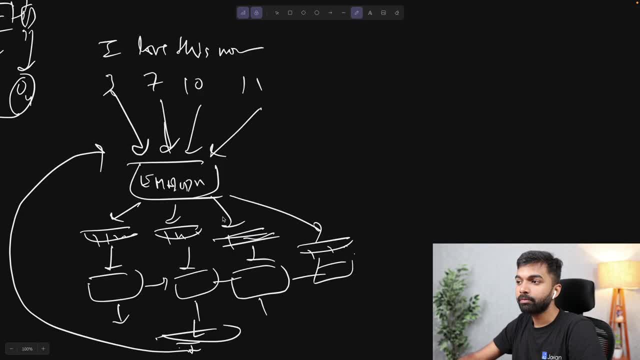 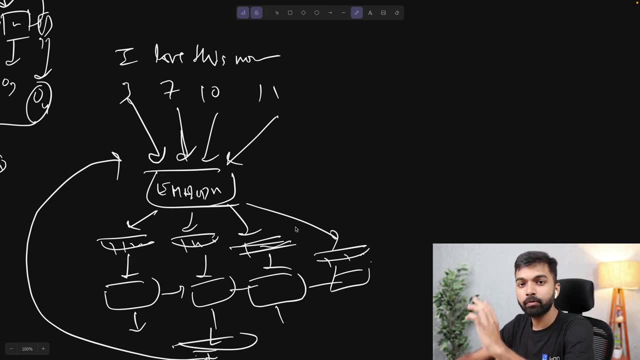 what we are going to get here, Okay, So this is the part that you really want to understand carefully: that three, seven, 10, one becomes a set of four vectors, And then we are basically stacking those four vectors on top of each other. 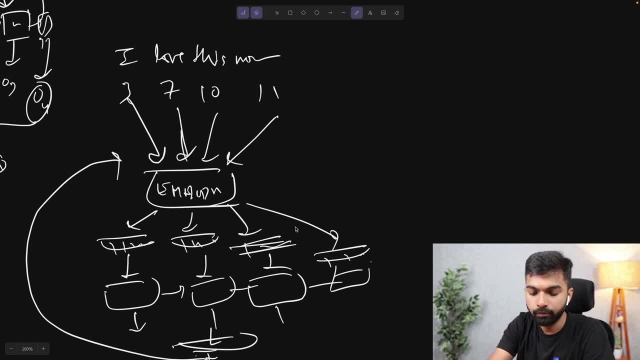 So here, if you were working in a batch, uh, one input. So let's say we had a batch size of two, 56. So we one batch would have two, 56 comma four if four was a max length. And now these four have been converted into four vectors of size, let's say 10.. 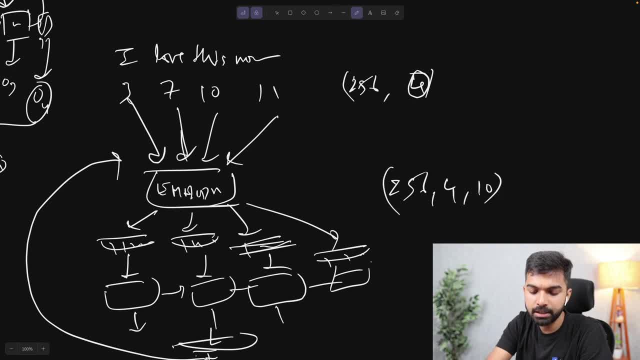 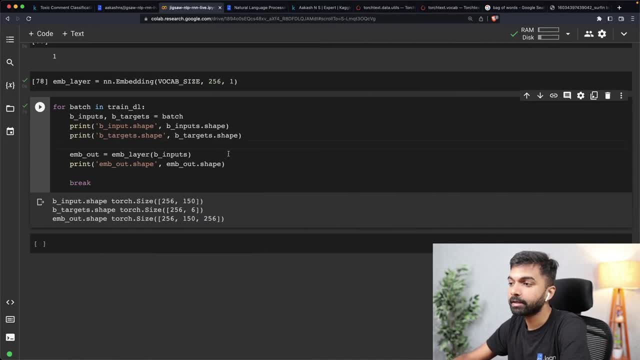 So then you would get two 56 comma, four comma 10, because each of these four numbers has been converted into a vector of size 10.. Okay, So make sure you understand what these specific dimensions mean. Now let's introduce our recurrent layer. 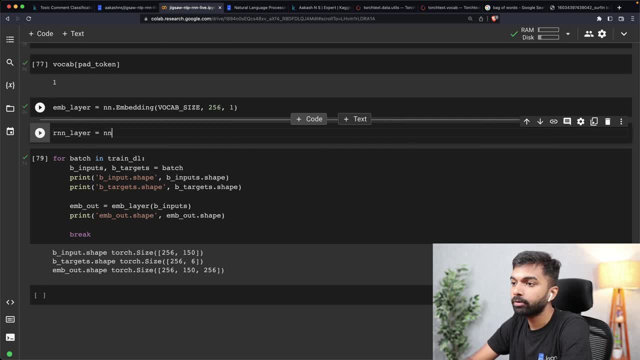 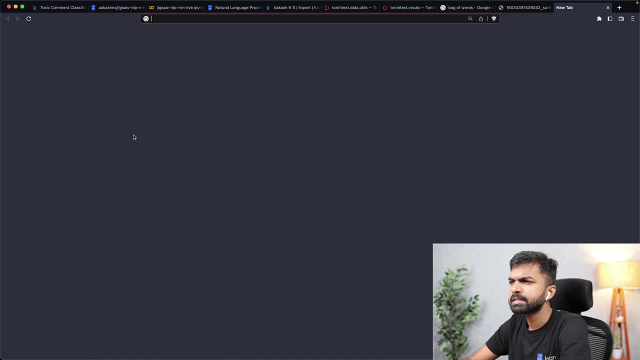 So let's also get an RNN layer And here, and the way you create an RNN layer is simply by saying NN, dot, RNN. Okay, And let's see how do we create an RNN. let's search: torch RNN. 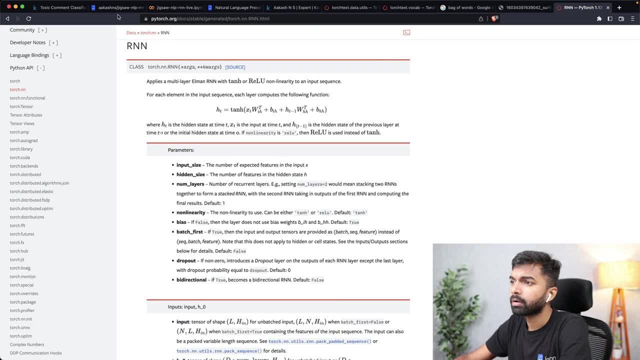 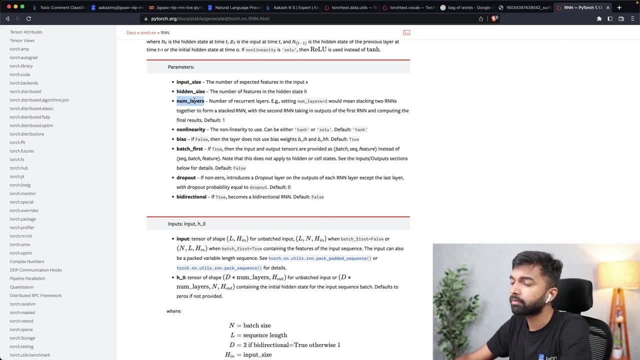 How do we create an RNN Yep? So this is what we need to give it: We need to give it the input size, We need to give it the hidden size and then we need to give it the number of layers. So we're going to give it the number of layers. 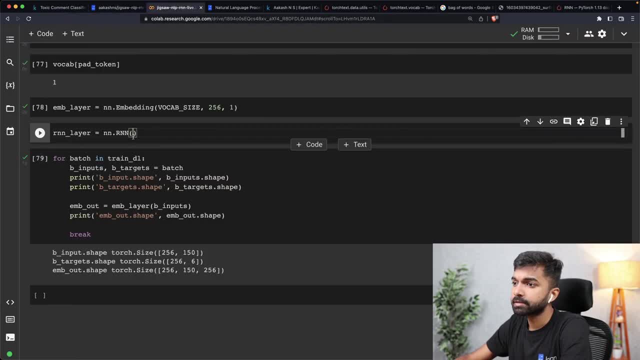 Okay, So I'm going to pass in the input size of two- 56,, because each of the word vectors is of size two, 56. And let's get an output of one, 28.. All right, And let's put just one layer for now. 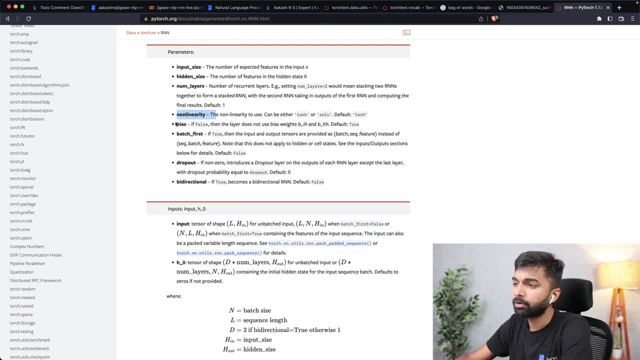 Now one other thing we will have to pass here. Okay, We don't need a non-linearity, We don't need a bias, et cetera, although we'll handle one other thing We need to pass as a batch first. 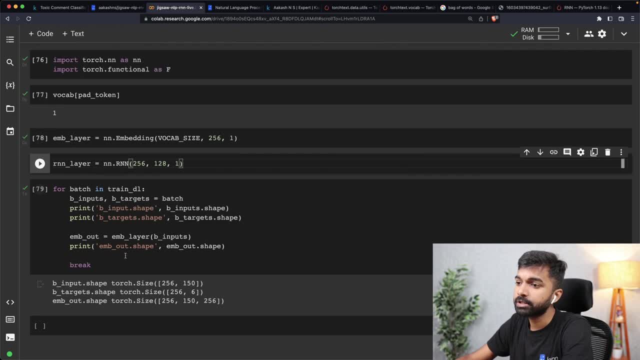 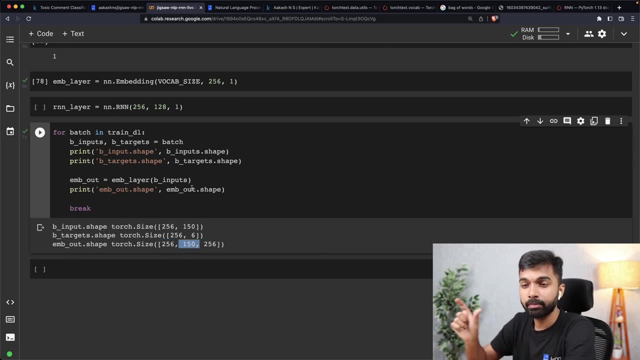 So what we have From our embedding layer is that the first dimension is the batch. You can see here, the first dimension is simply the number of batches, And then the second dimension is the number of elements in the sequence, That's the number of tokens. 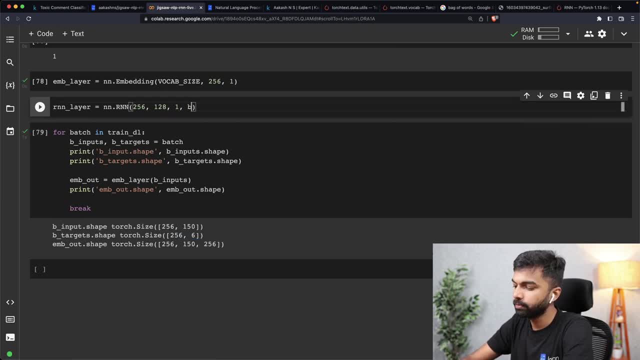 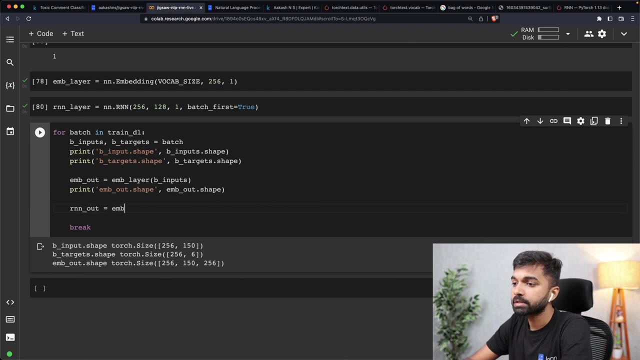 So that, so in this case we need to pass batch first- equals true, because the default behavior of by torch RNN is to expect the batch to be the second dimension. Okay, And now what we can do is we can say: RNN out equals. 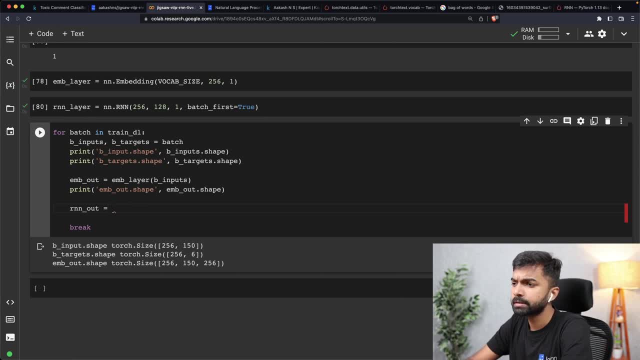 M Blair, RNN out equals um RNN layer and we can give it the embedding output, and the RNN layer returns two things. So it returns the out, doubt the output, but it also returns the final hidden layer output. Okay. 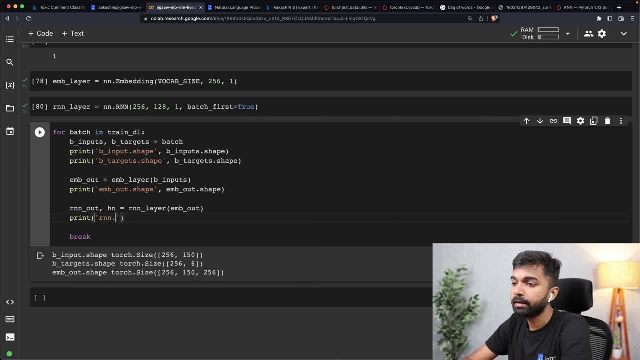 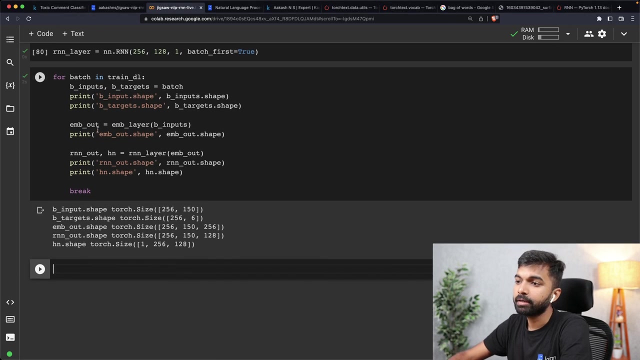 The final hidden state and let's just print both. So RNN out dot shape and let's print That's in dot shape. Okay, And let's print that, All right. So what's happening here? So now, from the embedding layer we got a 150 tokens, or 150 vectors, each of size 256.. 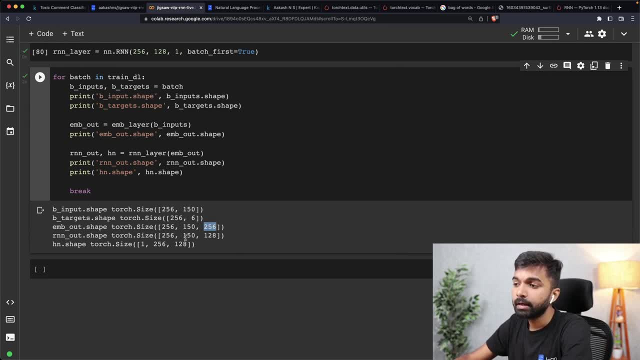 When we pass those 256 vectors, We, when we pass those, when we pass those vectors into the RNN one by one, each of them resulted in an output of size 128. okay, and the final hidden layer, the final, the output from the final RNN. the hidden state is also provided to us here, which we need not concern ourselves with. 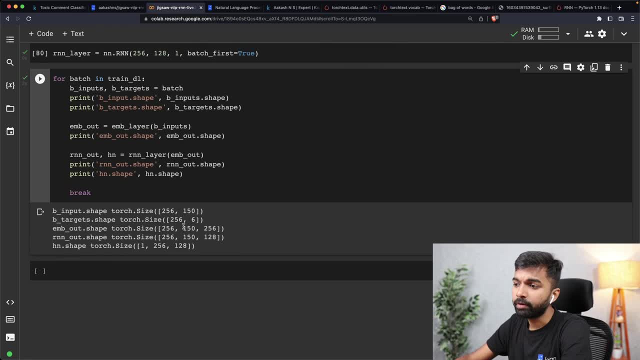 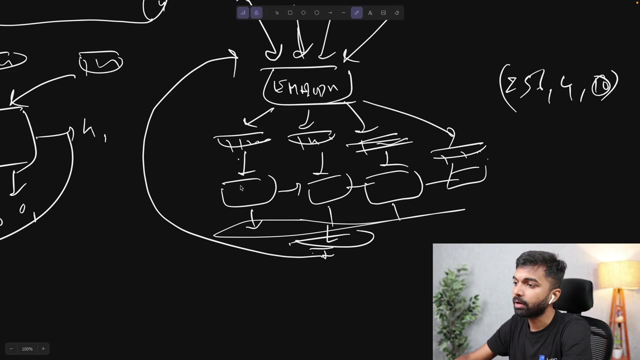 necessarily. so. this is how it works. so what we get back is we get back all the 150 outputs. so what so this? what we're looking at here, RNN out, is basically all of these outputs combined together, right? so the output of the first step, the output of second step, third step, 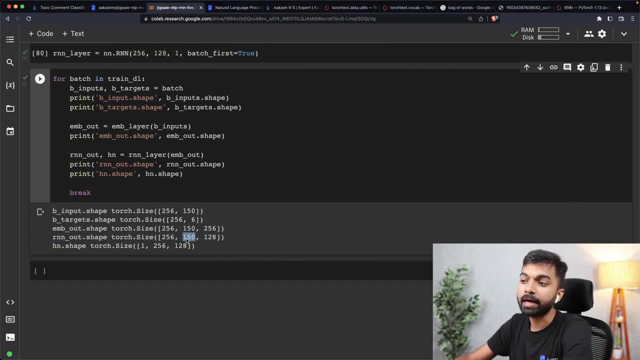 fourth step and so on, and in our case we are only going to use the final output from the model. so we're just going to use the final output, the output of the final step, and pass that into a linear layer to finally make a prediction. okay, so let's now define our dataset. 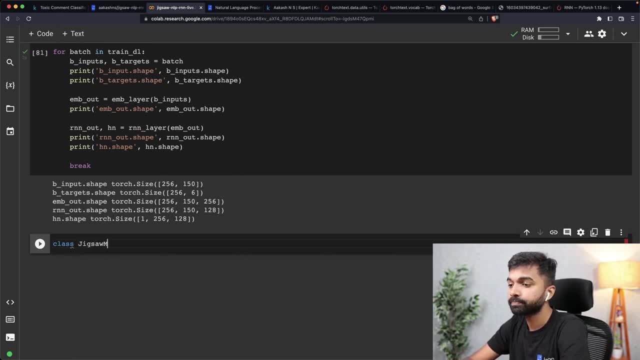 let's now define our model. so I'm going to call this jigsaw model and for this model I'm going to use pytorch lightning, because it's going to make the training of the model a little bit easier. so you might have to install pytorch lightning. so the way you install it is just say pip install. 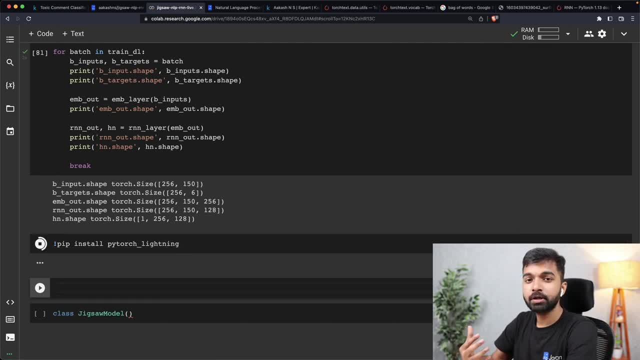 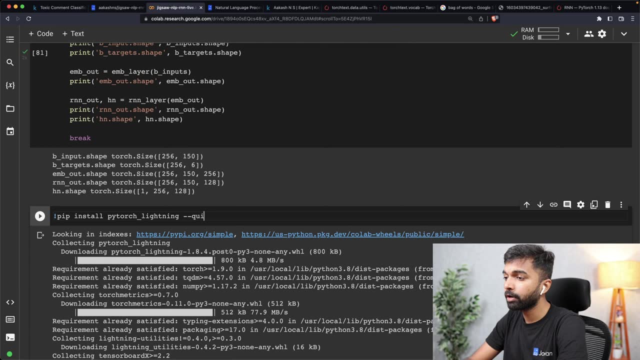 pytorch lightning. it is simply an extension of the pytorch module and it can be used to just simplify the training loop a little bit. we don't have to use a. we don't have to implement our entire training loop from scratch. okay, so now we're going to call this model and we're going to 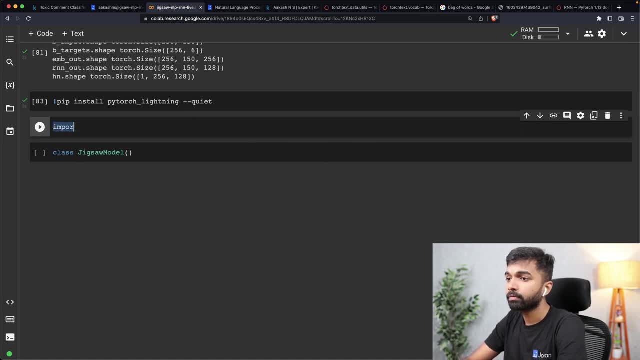 now we have pip, install pytorch lightning and I'm going to import pytorch lightning as pl and I'm going to use pllightning module and we need to define in any pytorch model. we need to define self or we need to define an init. 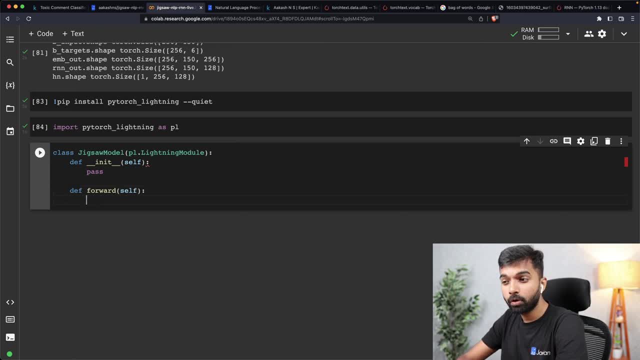 and we need to define a forward function. okay now, if you don't know how to use pytorch, then you should check out our course. keep learning with pytorch: zero to gans. so these are the two things that we need to define in any pytorch module, which is what pytorch lighting module is an extension of. so let's do that so. 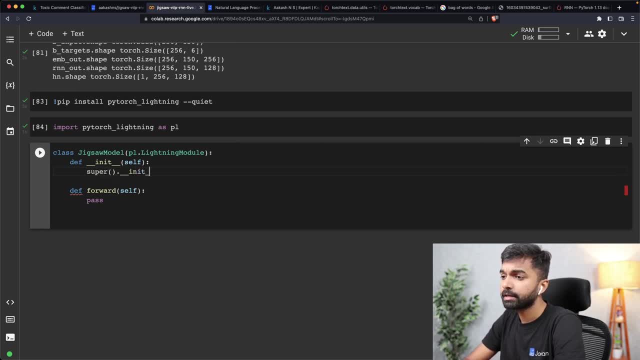 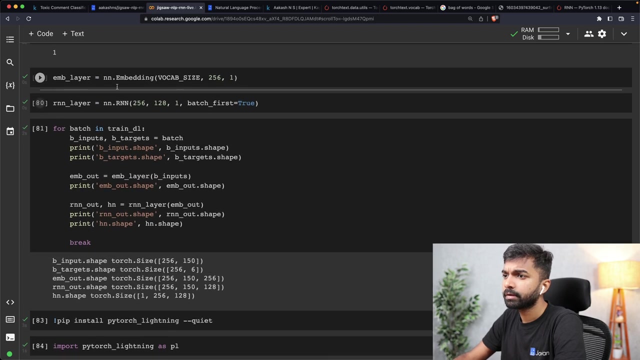 I'm going to first say super dot, underscore, underscore init. this is something that we have to do in pretty much any uh class in python, really. when we're extending, then let us first define an embedding layer. so self dot emb is: let's see, yep, let me use that. 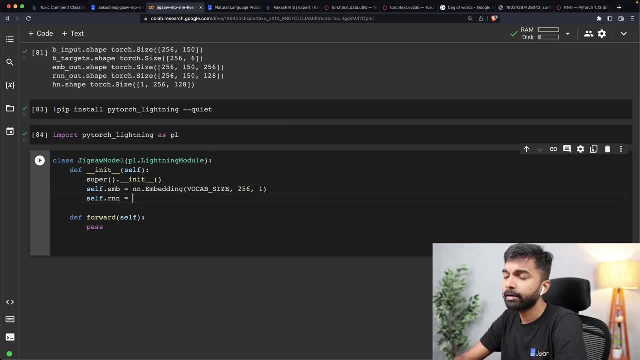 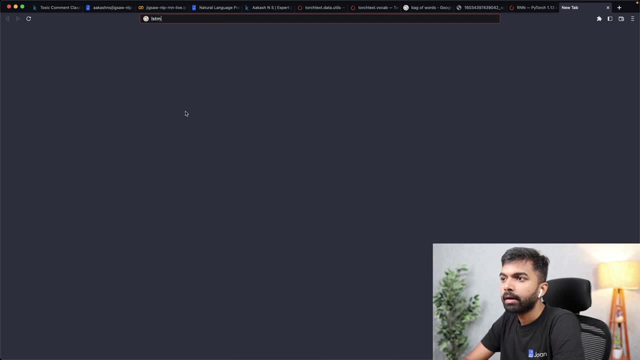 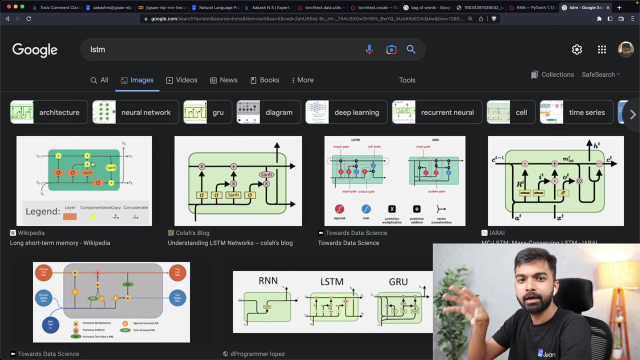 and then let me create an RNN layer, so self dot RNN. now I'm going to use an advanced form of RNN called lstm. so the lstm layer is a slightly more complex version of RNN. so it contains this inner structure inside it of a bunch of nodes and it has some special activations. so this is what an RNN a. 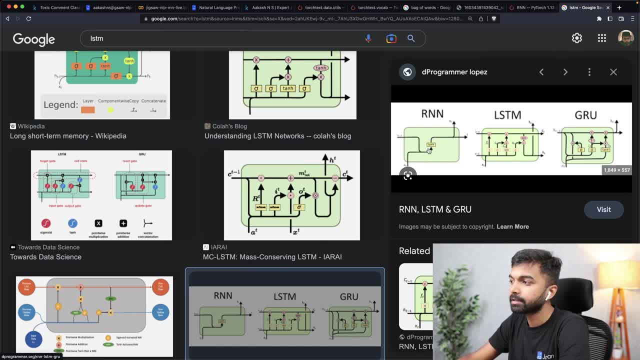 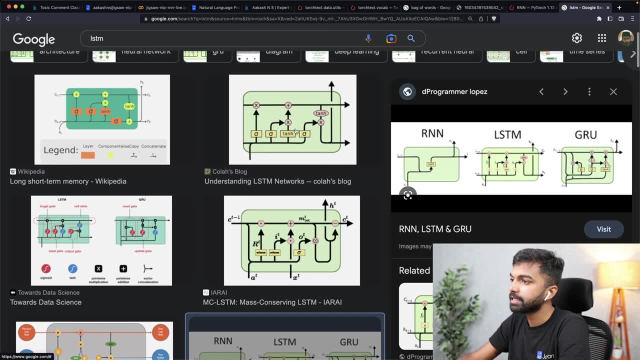 normal RNN looks like. it takes the hidden out input. it takes the uh the input and it combines them in some fashion through a simple computation. we have a more advanced version called lstm. so here is what an lstm looks like. it has a bunch of things inside it, but conceptually it's similar to 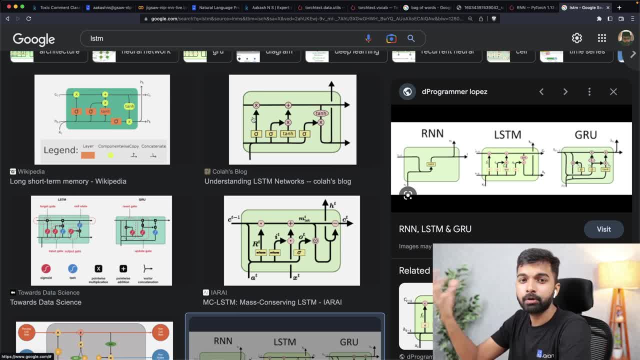 an RNN, you give it an input, you give it a hidden state, it's going to give it you an out, give you an output and it's going to give you a new hidden state. another one people use is something called gru, but I'm I'm just going to use lstm, so self, I'm just going to call it selfrn. 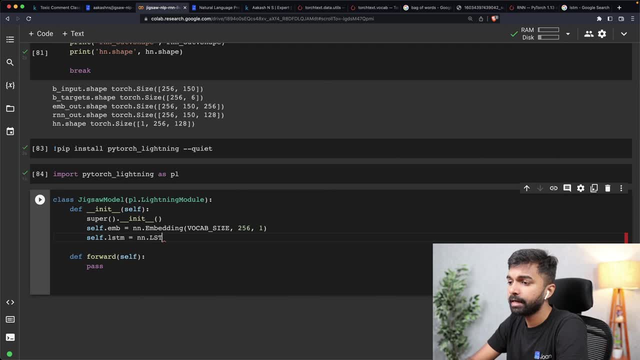 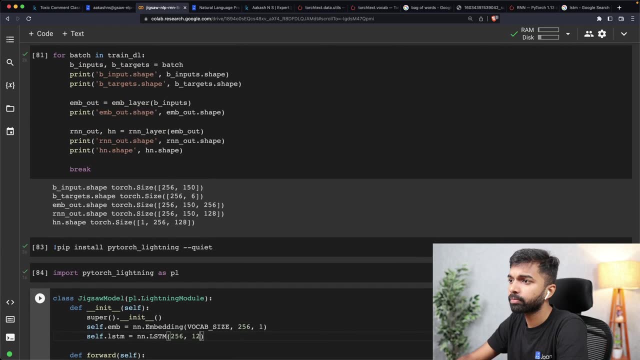 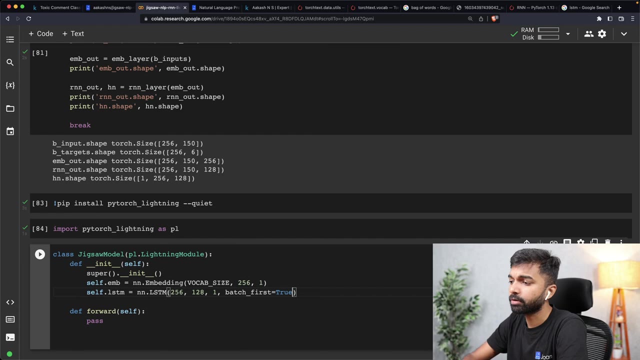 dot lstm equals nn dot lstm and it accepts the same input, so it accepts the input size. then it accepts the output, so the output is going to be 128. it accepts one and it accepts whether it is the batch, is the first position or not. okay, then, finally, I'm also going to have a linear layer, so 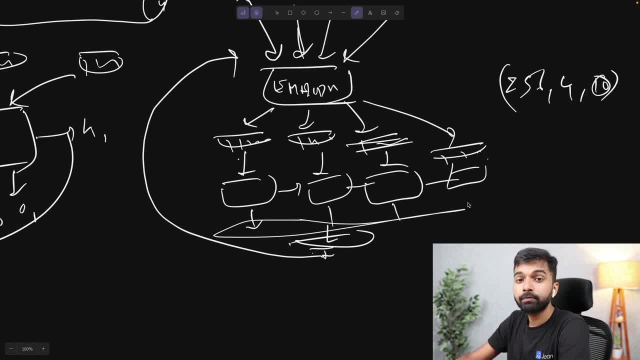 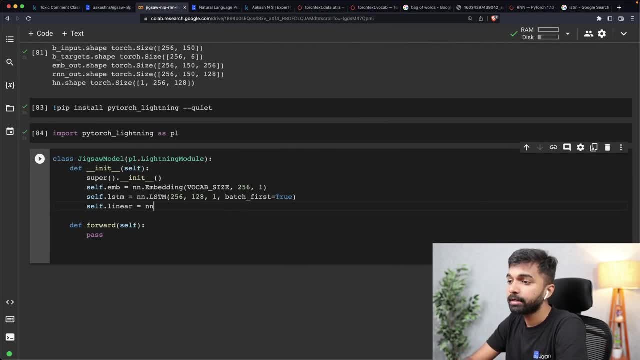 what I'm going to do is take the output of the final step and pass that through a linear layer of the model. so selflinear is simply nnlinear, which takes 128 inputs and it returns six outputs. okay, and that's our model. we have an embedding layer, we have an lstm layer, we have a linear layer. 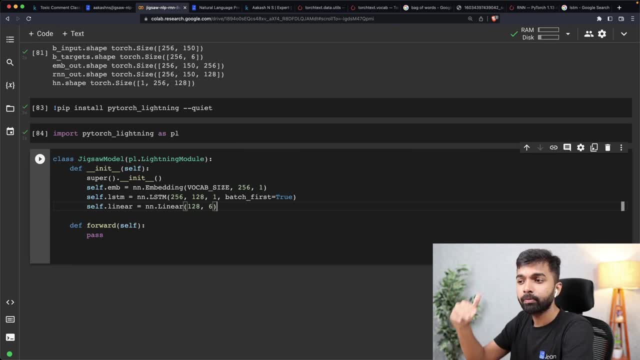 this is a very basic model. we can have multiple lstm layers, we can also then have multiple linear layers, and then we can do all sorts of regularization, batch normalization, so there's no limit to what you can do here. so let's implement the forward pass. so in the forward pass we get an. 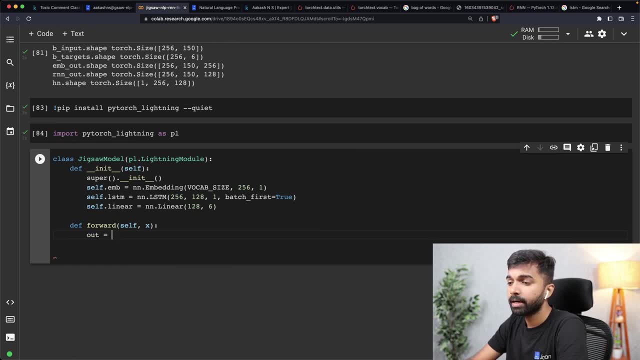 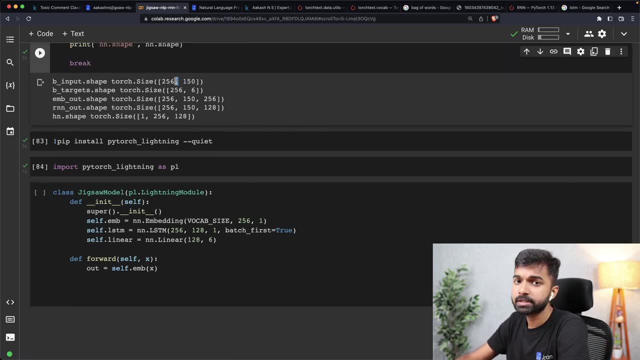 input x and first we pass it through the embedding so we say selfembx. okay. so the x is going to be of this shape: 256, so batch size of 256, and then vectors of size 150 containing the token information, information about each token that is present in that. so it's a padded comment and 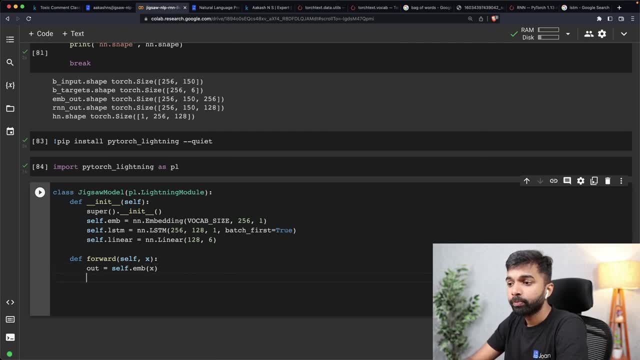 information about the tokens present in the comment. then we have to pass it through the rnn. so that's where the sequential loop occurs. so first the first token gets passed after the first tokens embedding vector gets passed, and then we get a hidden state. and then the second token's embedding vector gets passed, and then we get the hidden state, and so on. 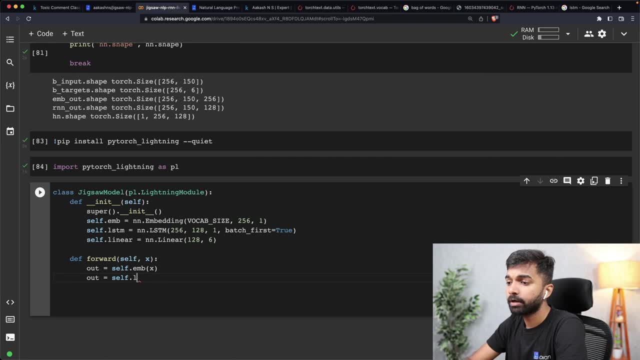 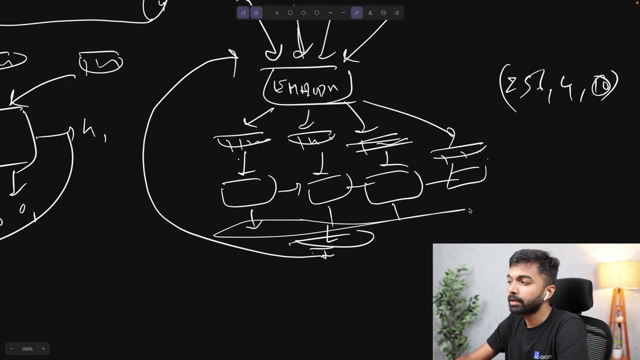 so then we can say selfrnn or selflstm out, but of course we get, apart from the out, we also get that final hidden state now from our rnn output, which contains 150 outputs. right, so it contains the output of every step. we just want the last step output. so what we're going to? 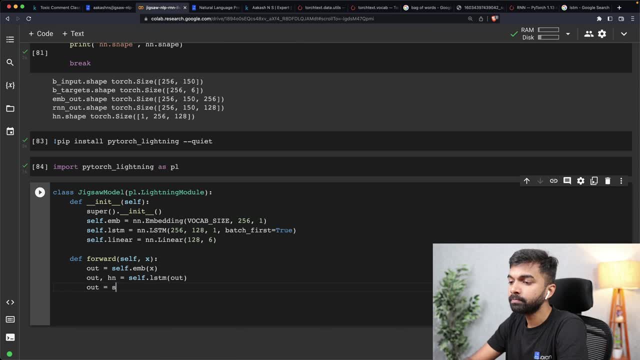 do isvp. we're going to do is supply. we're going to ServiceWise, so we're going to do service, do service, deviceserviceservice, And we're going to choose the service vo Windpoints for that in is. we're going to say out equals self dot or F dot value. 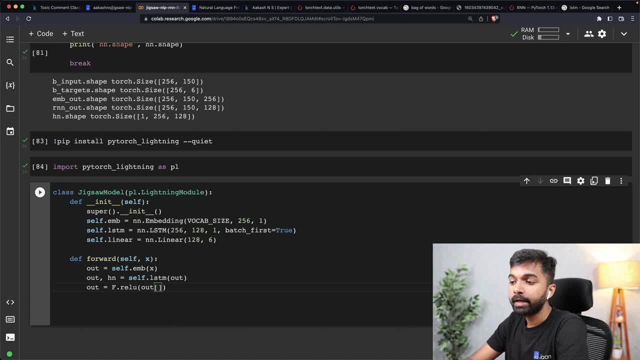 We are going to apply an activation function, but now we're going to apply it not to everything, but simply to the output, simply to the final output. All right, So what we're saying is: we want all the, we want every element in the batch. 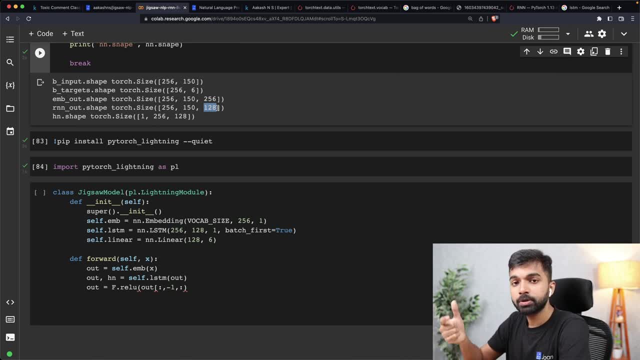 and we want all the outputs that we have obtained, the outputs of size one, 28,. but we only want the output from the final step. Remember the one 50 steps. one 50 times. we are passing tokens one by one. Now the final output should contain the summarize information for all the one. 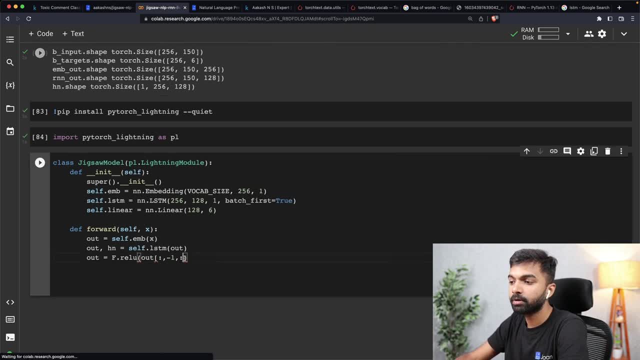 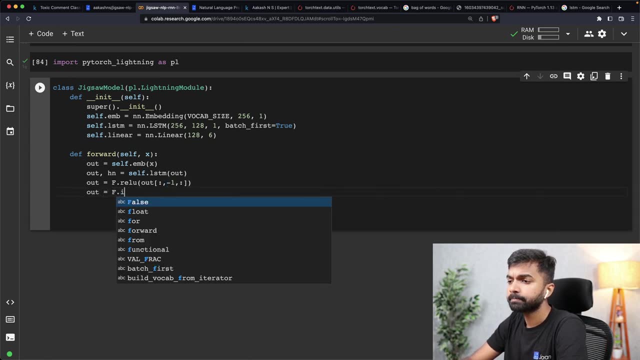 50 steps, because the hidden outputs are passed into it. And that is what we're doing here: We're simply taking the final output out of the one 50, and then we can finally pass that into our linear layer out And I can simply return out. 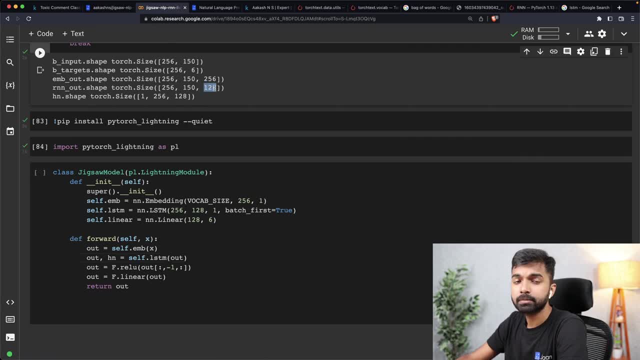 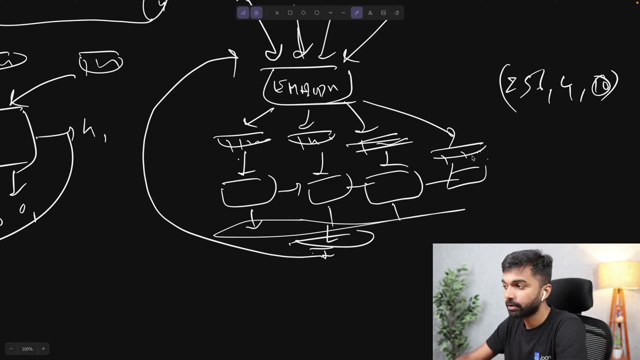 The linear layer is going to then take those one 28, the output of size one 28 that has been received from- Yeah, Each of these from the final layer, from the sorry, from the final step, and convert that into a bunch of six numbers, basically by just doing a matrix. 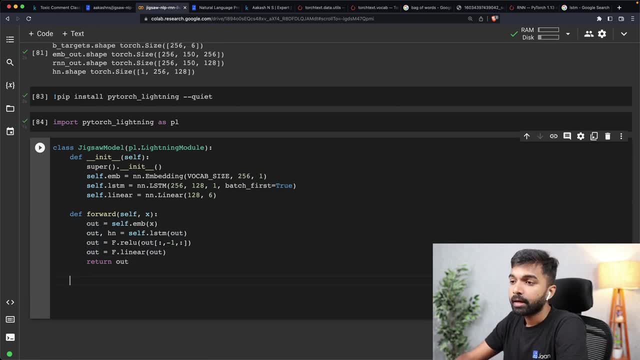 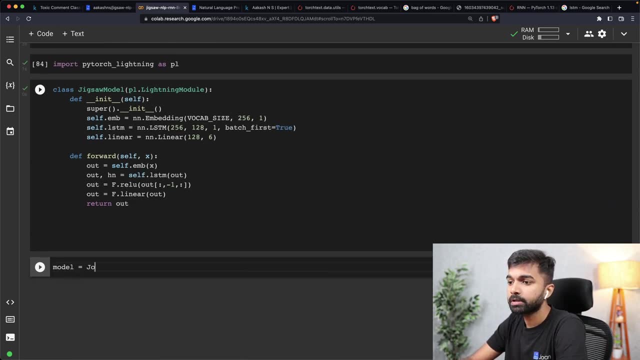 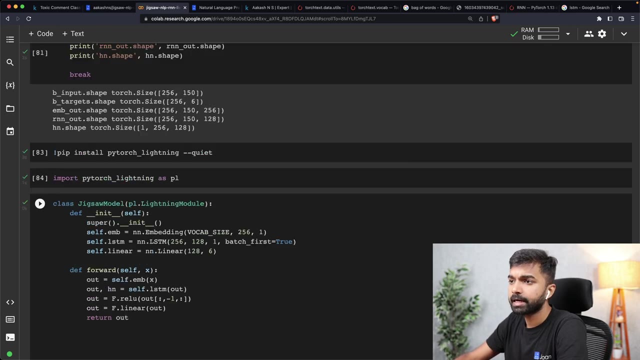 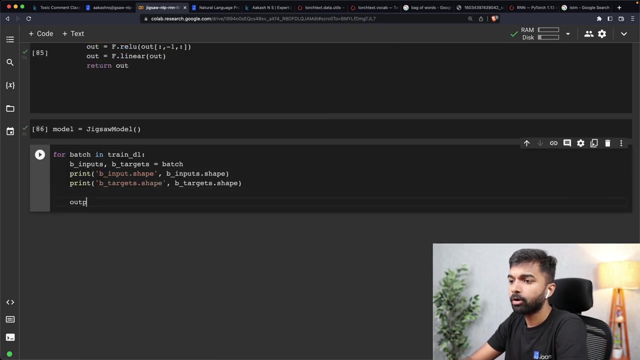 multiplication. So that's our forward step And that is how you would define a normal by torch module And now you can actually see: her model equals jigsaw model And we can now say: let's get all that information back here Now. we can now say: outputs equals model batch inputs and we can 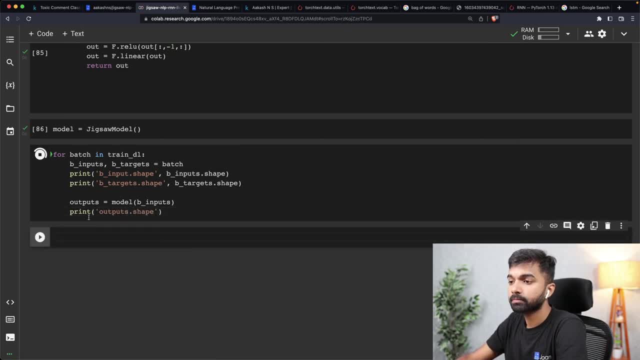 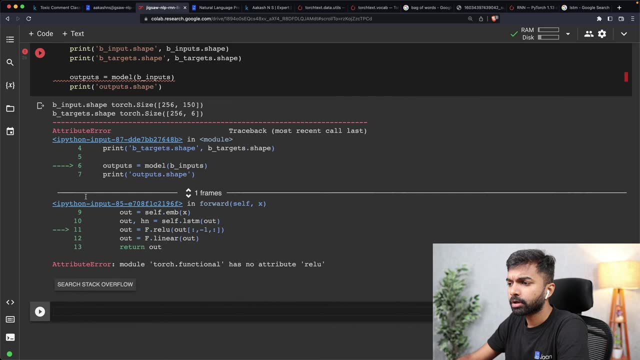 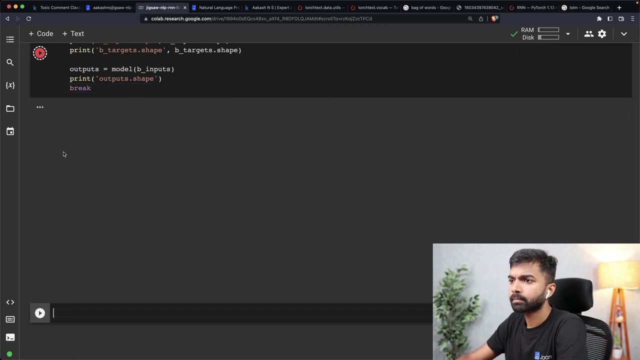 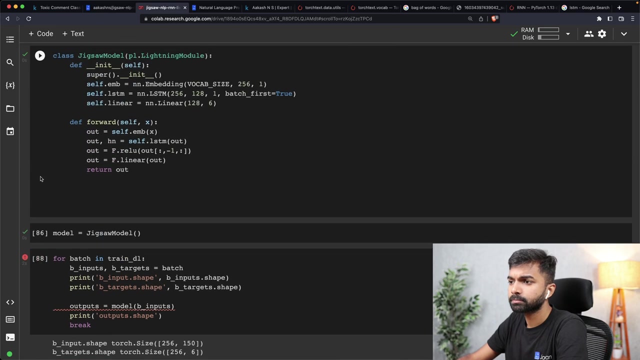 simply print or put start shape. Okay, Well, Torch NN Function has no attribute value. Oh, I Just need to put in a break here as well. Yeah, We just want to look at the first batch. Okay, I'm just going to check why a PyTorch doesn't work. 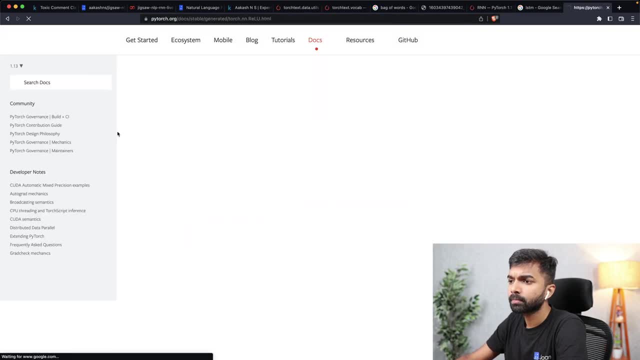 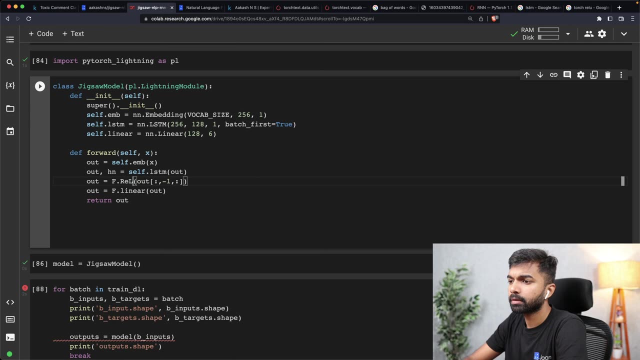 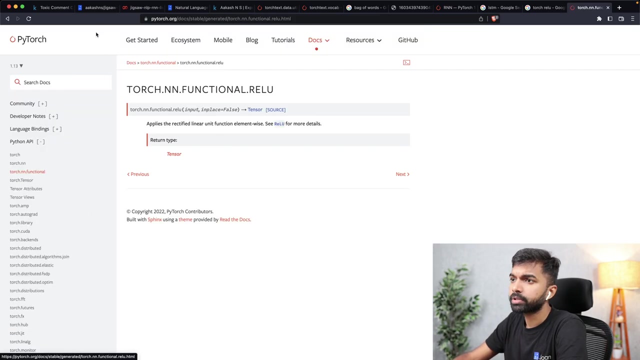 So Okay, I believe it's just. If you are watching this video, you might have gotten that wrong. This is my first time doing this, So here we are And I'm going to make a search for this. It's called search. 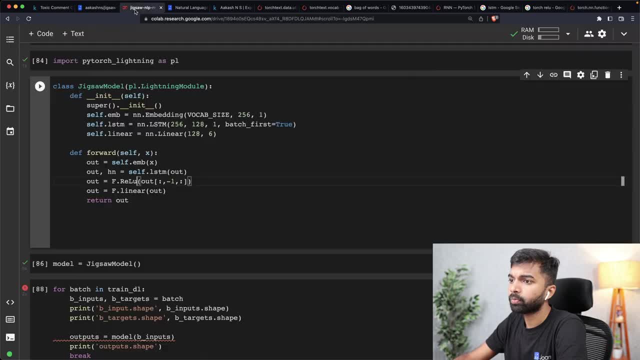 And you can go to search. So I'm going to say the Service. So it's all: Torch NN, functional dot value. So I can't even figure out what my data is going to be. So I'm going to say this: Okay, So I'm going to say this. Okay, So let me just do that, So let's do the search So I can see the URL. That's the value of, That's the value of my data, The value of the data. 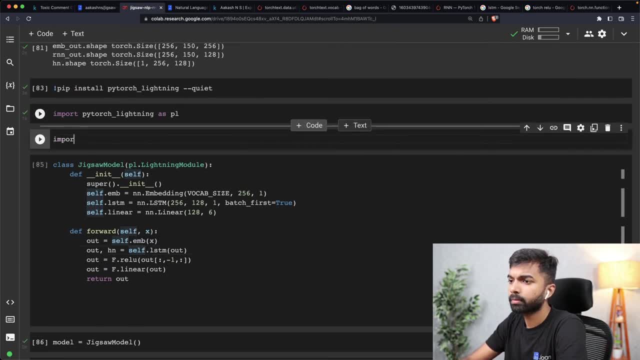 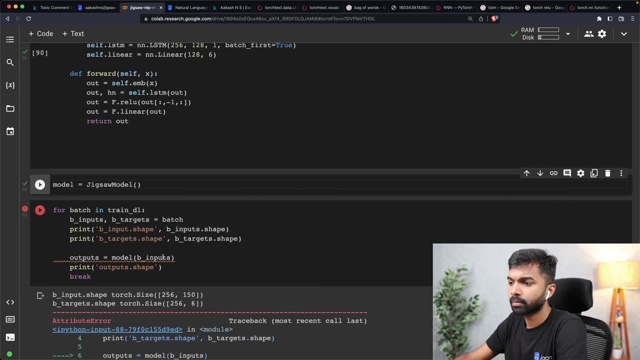 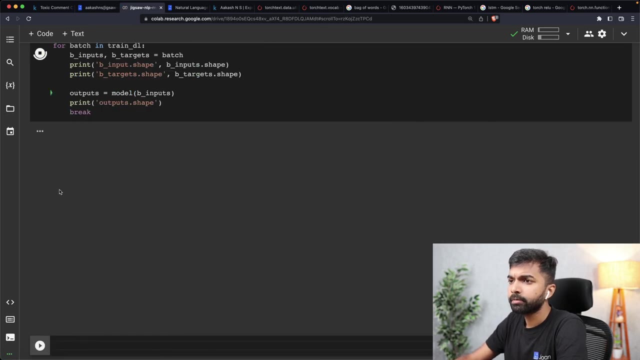 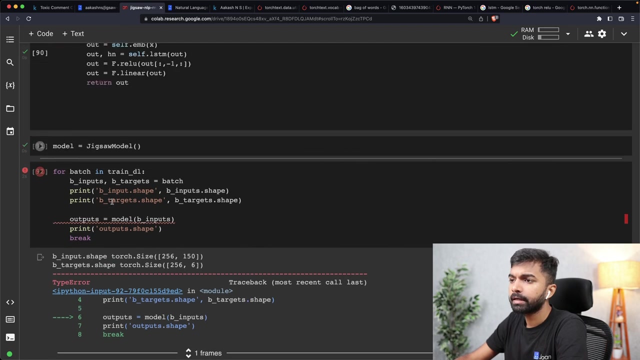 So I'm going to say So, I'm going to say: Okay, let's create a model once again, let's just print this information out. Okay, and linear is missing. it's not F dot linear, it is self dot linear. 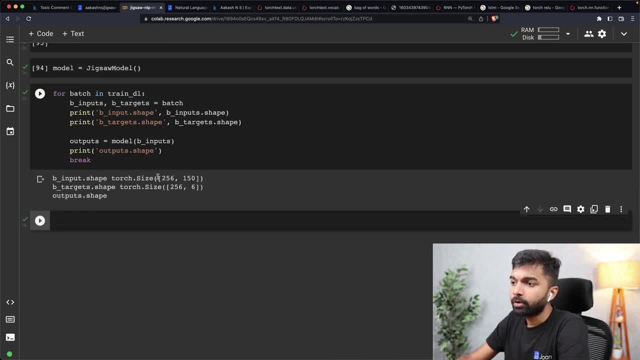 Yeah, So now we are passing in 256 vectors. those are going to get passed through the embedding, those are going to get passed then through the RNN. then we're going to pick the output of the last step And then we're going to pass it through the linear layer. 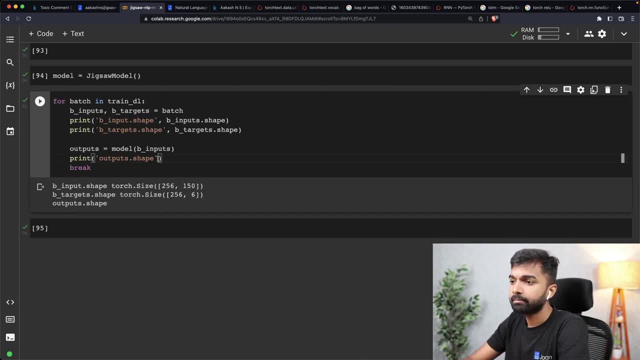 And that is going to give us six outputs and outputs dot shape. Let's just print that out And we should see that we get back six outputs. So now we get back six outputs from the model. we get back six targets. we get, we have six. 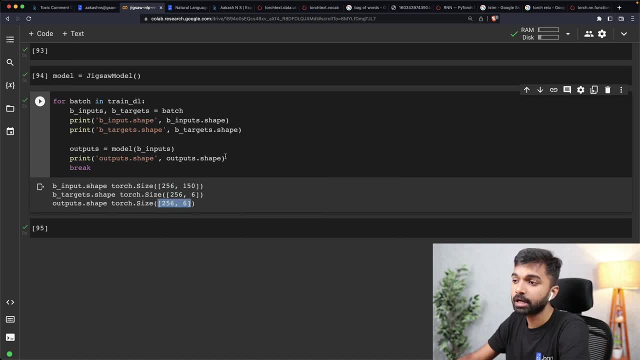 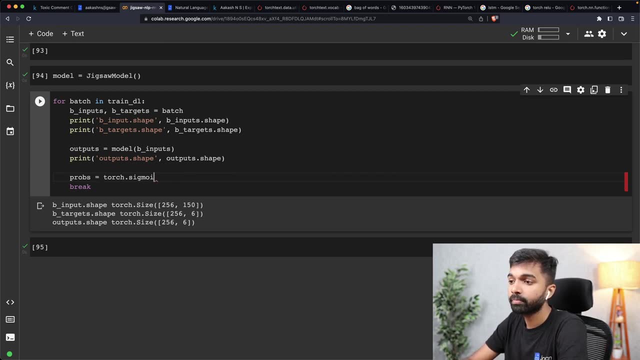 targets for each. For each row, we get back six outputs And now we can compare these. the way we can compare these is first convert these outputs into probabilities using torch dot sigmoid. we can call torch dot sigmoid on the outputs and get back probabilities. 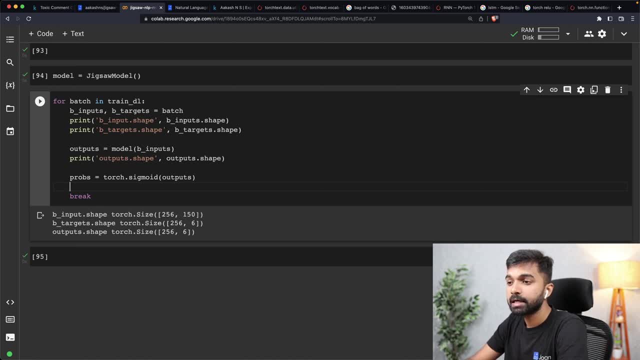 And then we can use the binary cross entropy loss. So we can say: loss equals F dot binary cross entropy and give it the probabilities and give it the targets And that is going to be our loss. So we can now print our loss. 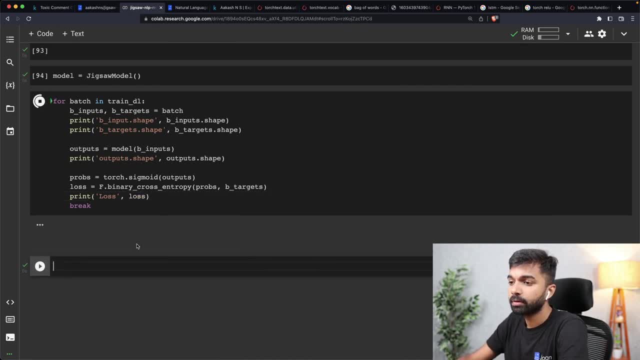 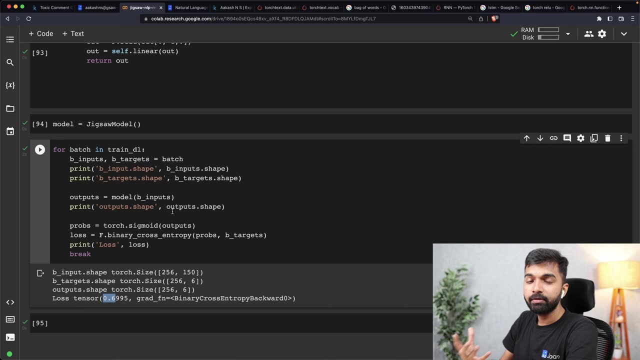 So the loss of our model is 0.69.. All right, and that is the model that we have trained, And now we have to set up the training loop so that we can reduce the loss by performing the gradient descent optimization and improve the performance of the model. 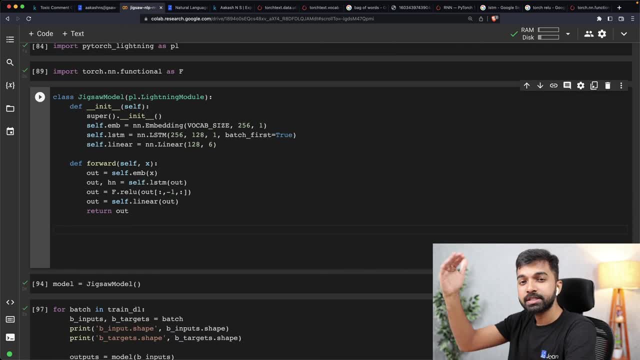 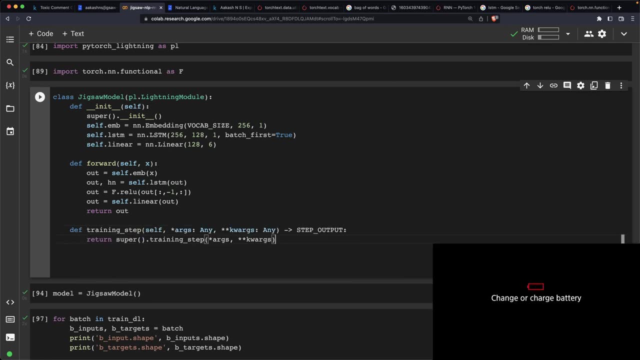 Okay, Now here's one thing we can do in pytorch lightning. we can specify a bunch of steps from the training process within the model itself. The first thing is a training step, And in the training step we get a batch of data and we simply have to specify what. 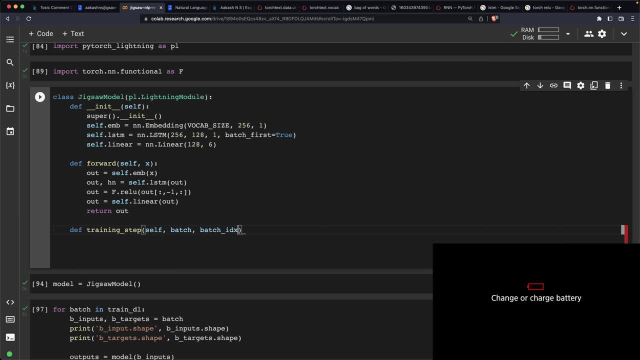 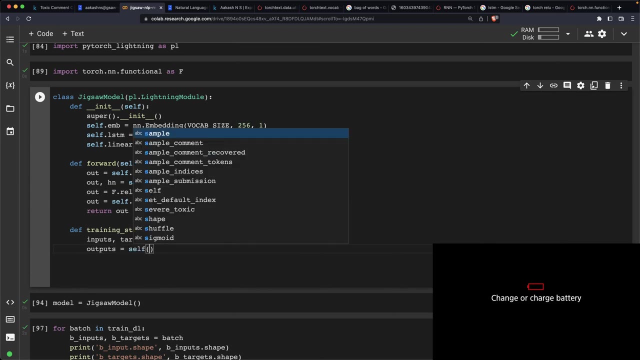 to do with that batch And we also get a batch index. not that we need it, And now we can. we can do this so we can get the inputs and targets from the batch And now we can pass the, we can pass the other inputs through the model. 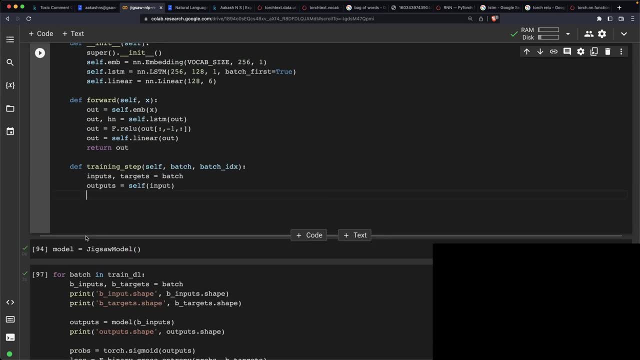 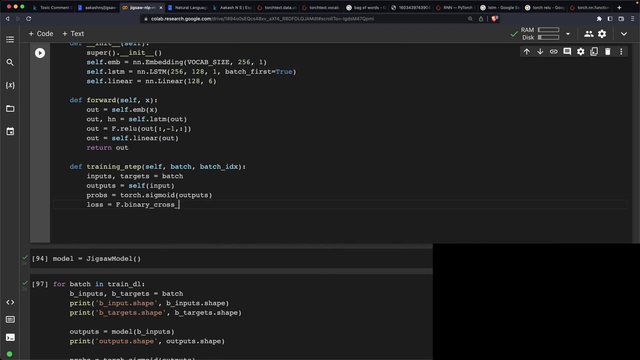 So self inputs, and that is going to give us the outputs, And then we can get the loss. So first we can get the probability, So probs is simply torch dot sigmoid outputs. And then we can get the loss, So loss is simply f dot binary cross entropy probs, and then we can return the loss. 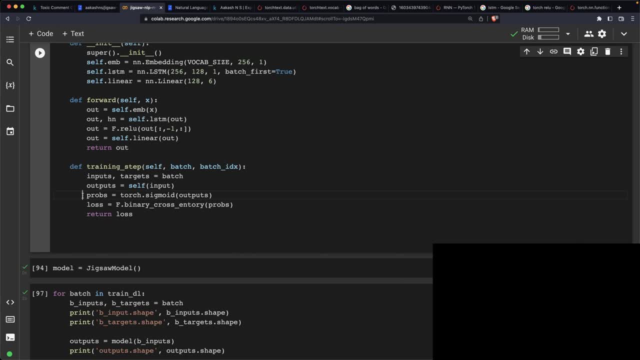 Okay, so this is all we have to do, And pytorch lightning will give us a trainer which can use this function to automatically train the model. Okay, And we also can define a validation. Okay, So validation step, the validation step. again, it's going to receive the self, the batch, and 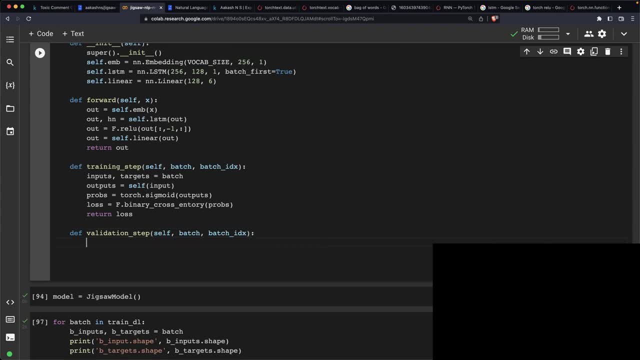 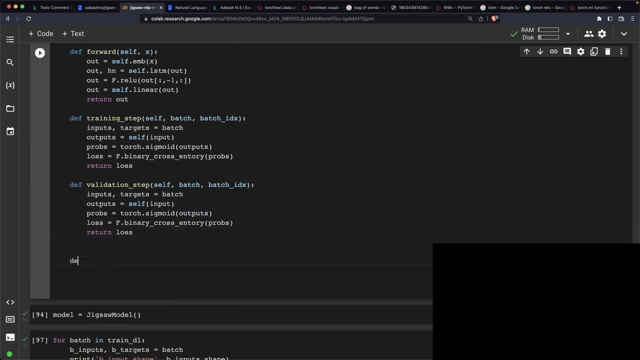 the batch IDX And the validation set is, the step is going to look very similar. So it's going to get a batch of data and we are simply going to return the loss. Then we have we can define something called a validation step end or validation epoch. 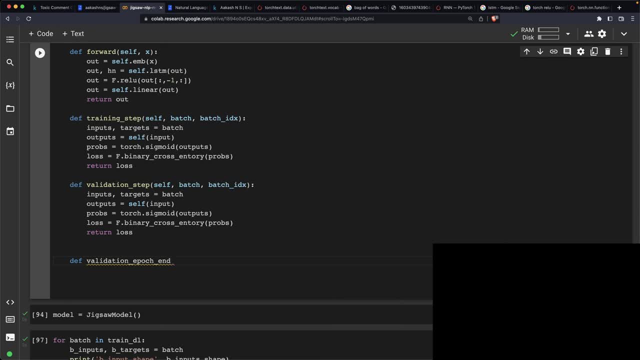 end, which is after all the batches from the validation data have been passed through the model. what do we want to finally do? So that's where it gets All the validation step outputs And we can just give return the overall total loss. 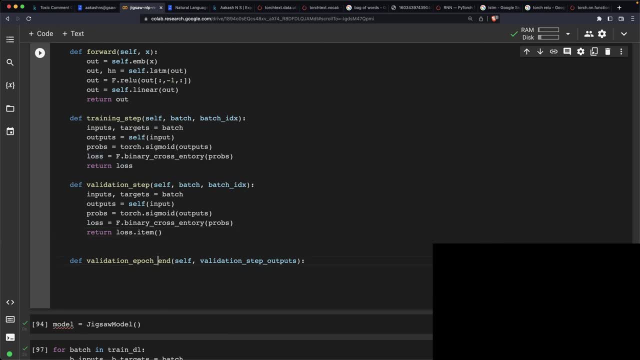 So I guess one thing we can do is we can simply return here loss dot item, which is just the value of that loss, And in the validation epoch end we can simply print the epoch number Okay, And we can print the loss. 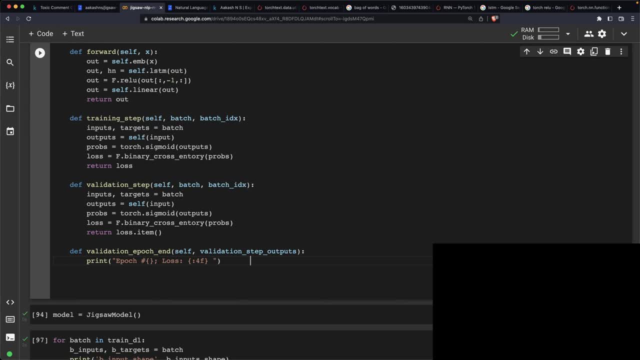 And I'll show you in just a second how all of this fits together. But I'm just going to format this with self dot, current epoch, And I'm going to add in the loss here, And the loss is going to be the average loss across all the validation steps. 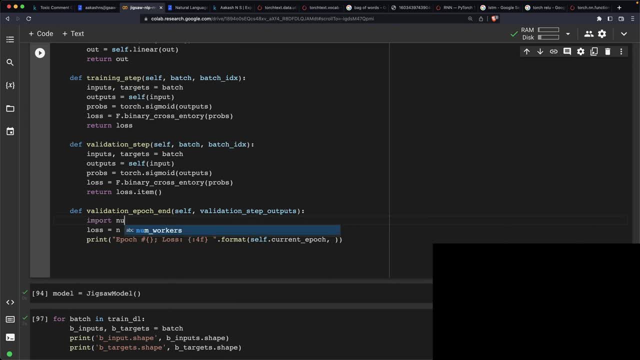 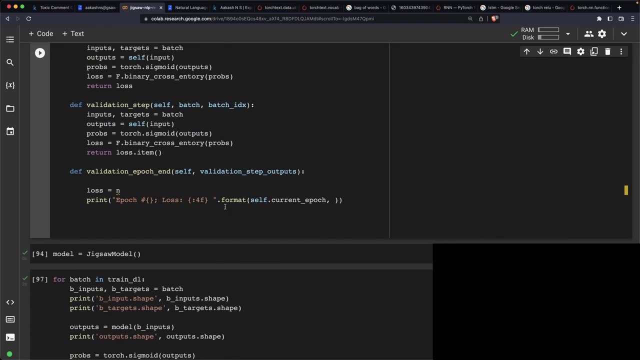 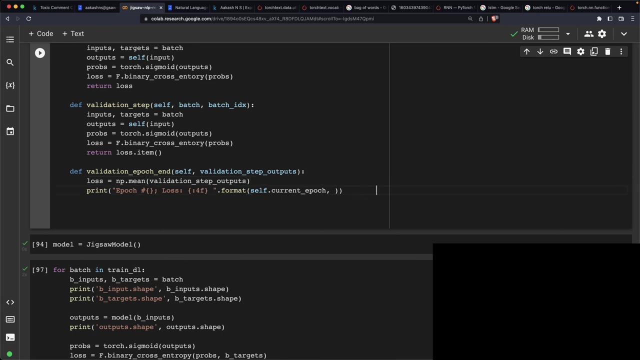 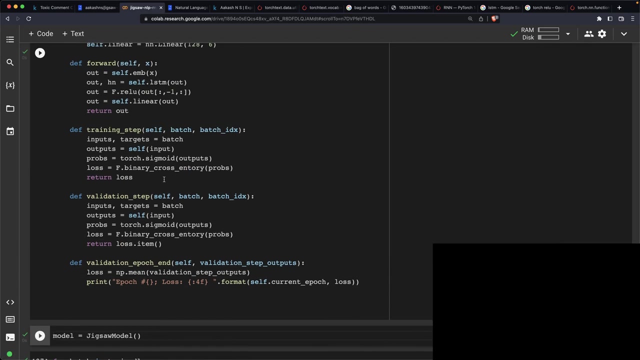 The loss will simply be: I'm going to import numpy here, Let's import it here itself. I'm simply going to say in p dot mean validation step Okay, And let's pass in the loss here. So what are we doing here? We're simply defining: given a batch of training data. 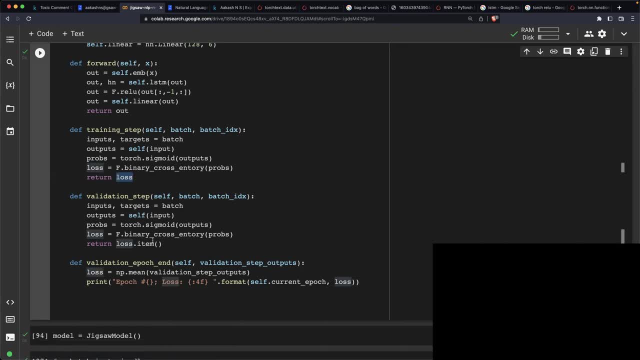 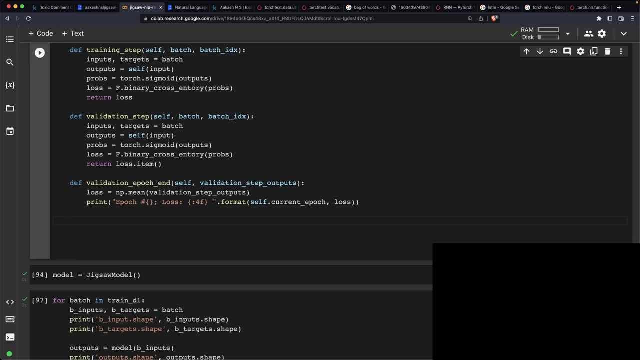 Okay, The loss, given a batch of validation data, how to compute the loss And, once we have all the losses from the validation data, how to compute the overall loss for and what and what we want to print out. Finally, there's also something called a predict step. 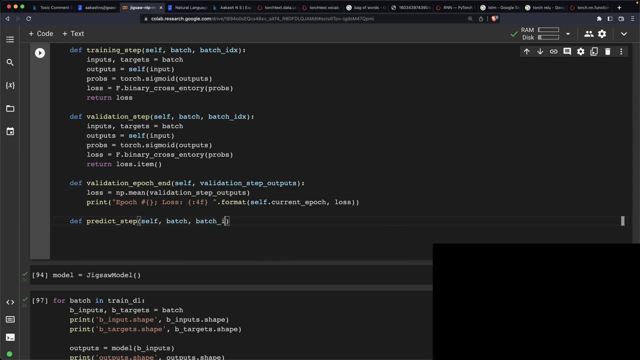 This is something that we will use with the test data set, And here what we will do is we want to actually generate predictions from the model. So I'm going to again get the inputs, outputs and probabilities and because in our submission file We're going to return the probabilities, we're simply going to return the probabilities. 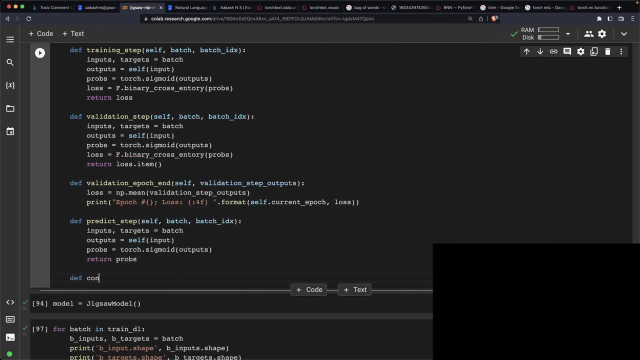 here, All right. Last thing, we also have to configure optimizers. to configure optimizer, or configure optimizers, is what this is called in my torch lightning, And all we're going to do here is we're going to use torch dot of them. Let's see. 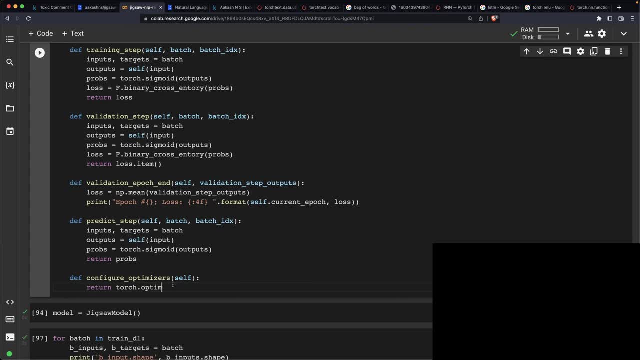 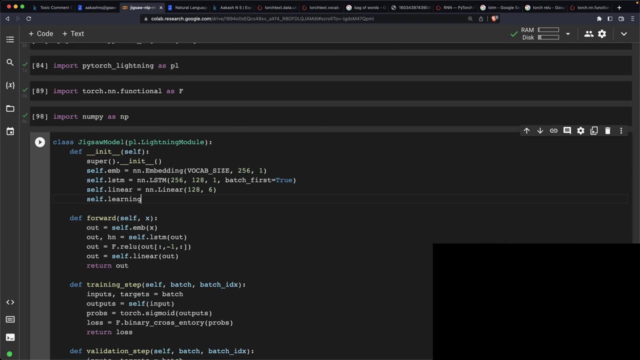 We can use the item optimizer, So torch dot optimizer, Okay, And I'm going to set a learning rate. Let's see It's a learning rate is something that we might want to allow ourselves to modify, So I'm going to put a learning rate here in the top learning underscore rate equals 0.001. 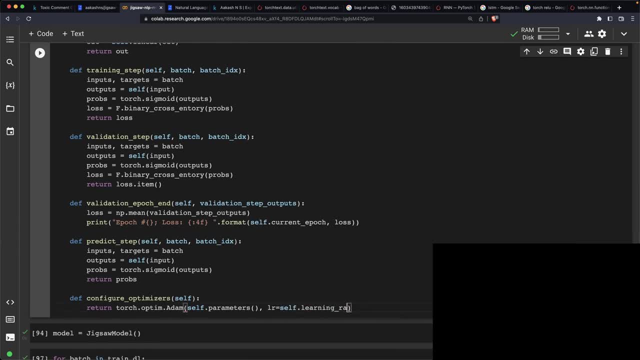 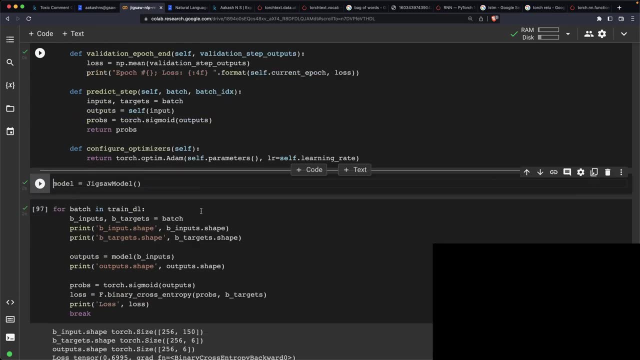 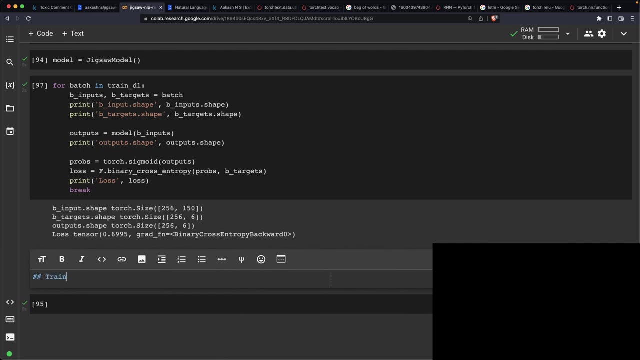 I'm going to just pass in the learning rate as self taught learning rate. All right, So that's our model, That's our pie torch lightning module, And now we can actually train the model. So let's train and evaluate the model. 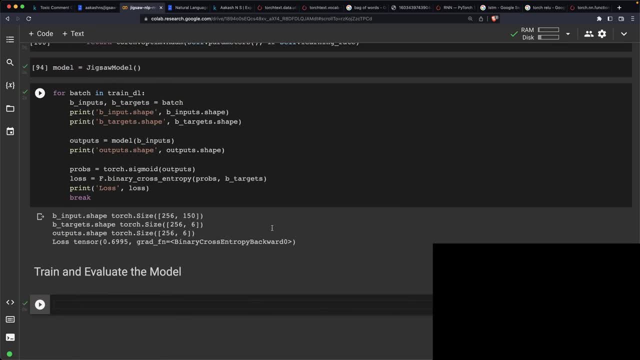 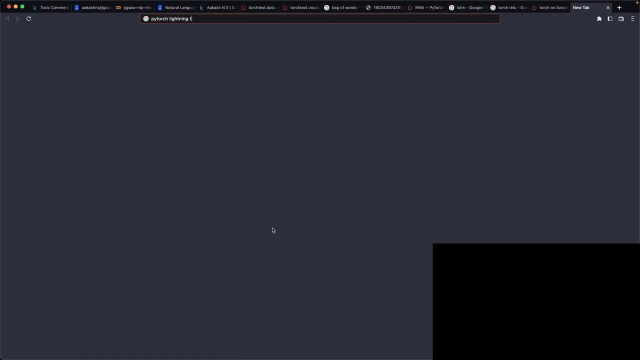 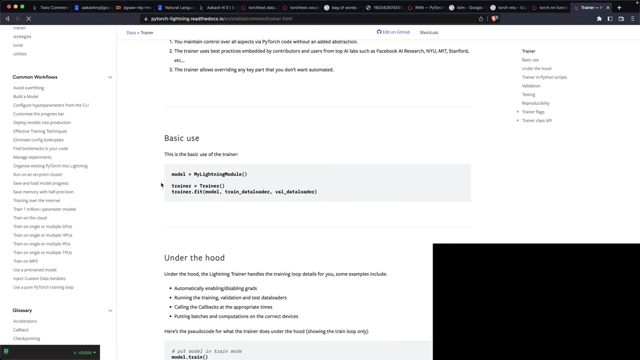 Okay. So what's going to happen is we're now going to create a trainer. Let's search by torch lightning rainer. So the lightning trainer Automates A lot of the Processes of training. the model for us, Okay. 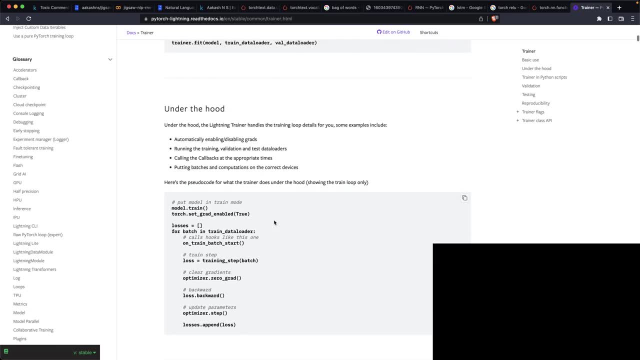 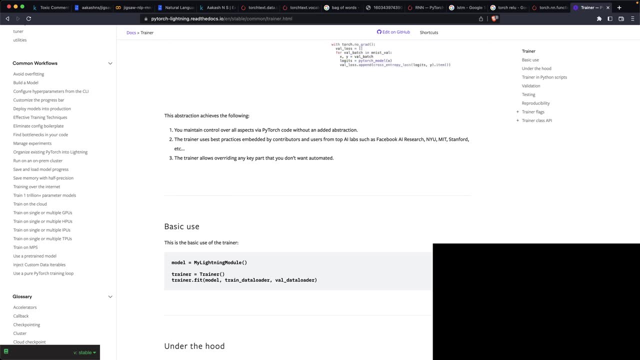 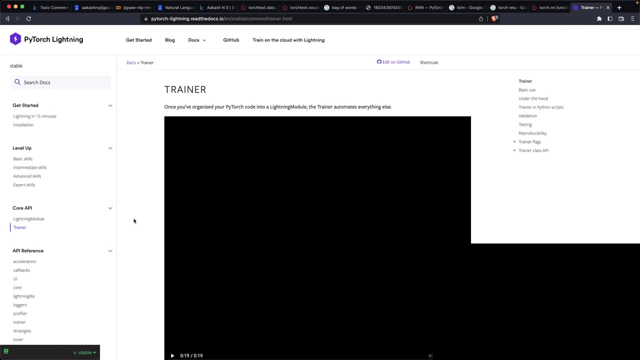 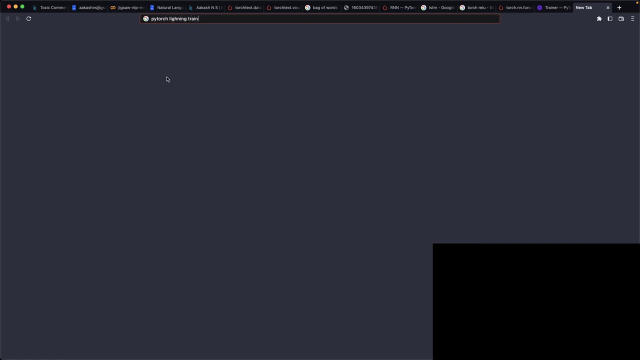 So we are going to create a trainer, and the way we create a trainer is we just say we just import from by torch lightning, We just import the trainer class. So let's see here How do we import the trainer. Okay, I see. 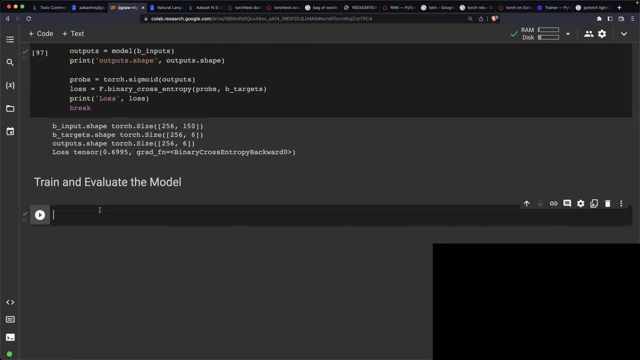 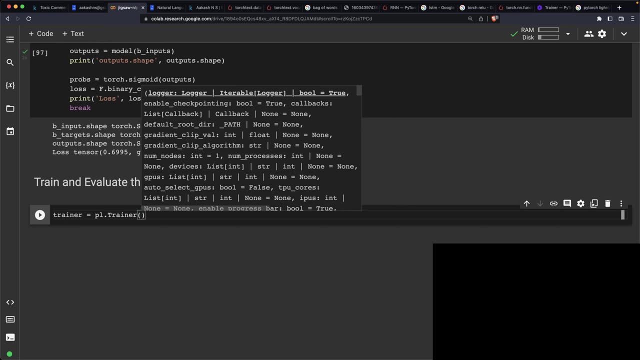 Okay, It's just PL dot trainer. I see, All right, So we create a trainer equals PL by torch lighting dot trainer and we can give it a bunch of information. The first thing we can give it is the number of epochs, maximum epochs that you want to. 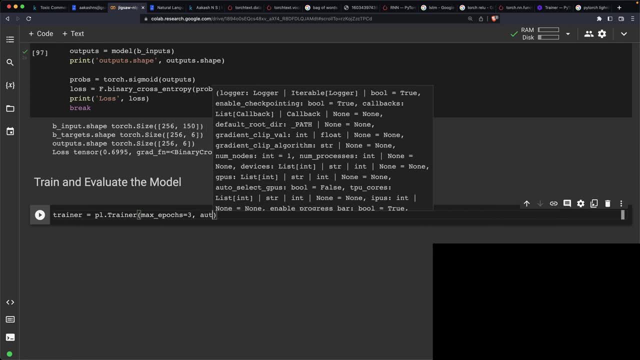 train for. So let's see, Let's train for three epochs at a time. Then we can also configure it to use an accelerator- In this case, I'm going to use the GPU accelerator, Okay, And we can also set it up to use and and to find the learning rate automatically. 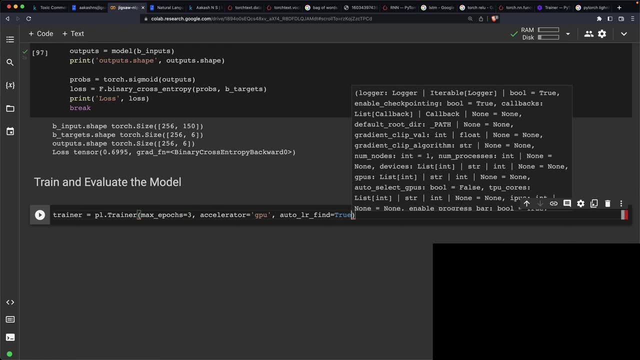 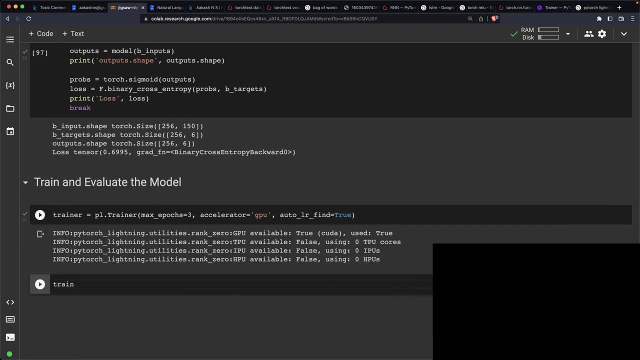 And that's why we have passed that learning rate as self dot learning rate. I'm going to say auto LR find equals, true. And then there is a yeah. so I think that's pretty much enough And now we can just create, now that we have created the trainer, now we can say trainer. 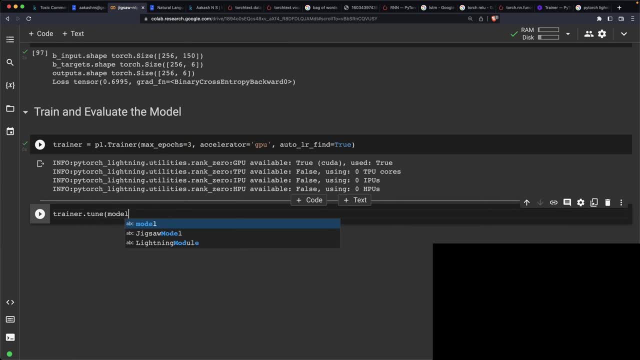 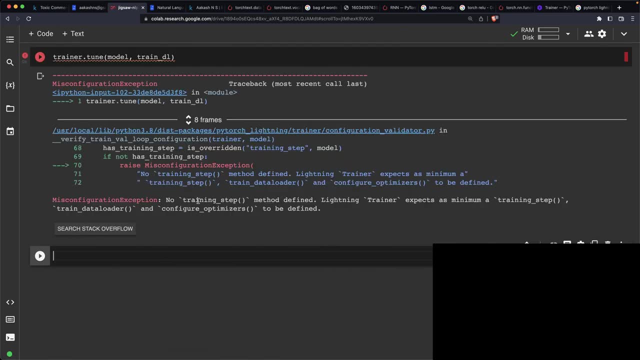 dot human, and that is going to figure out the learning rate for the model, the trainer dot tune model. And now let's give it a training data loader And what this is going to do is this is going to get Okay, No training step is defined. 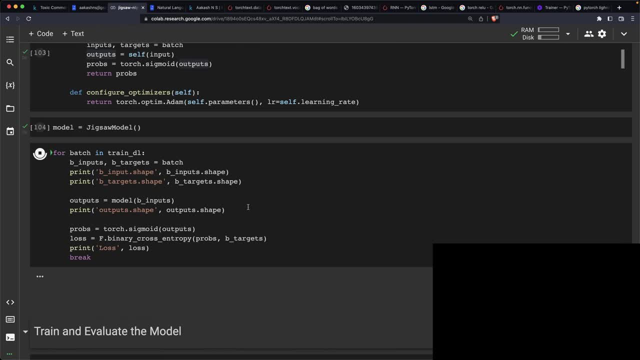 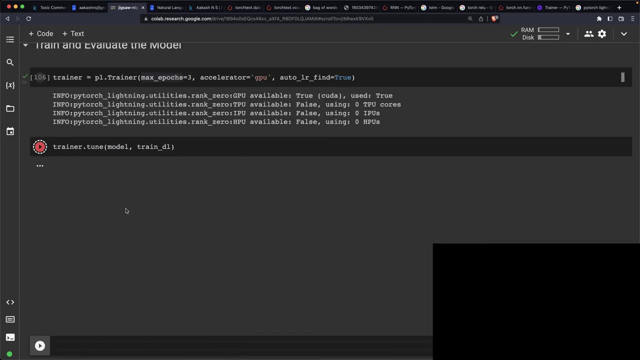 Let's run this model again. Yeah, So we've just defined, we decided to use new, these new methods, So you just have to create the model again. Yeah, Now we're going to tune the model. So now it is tuning the model. 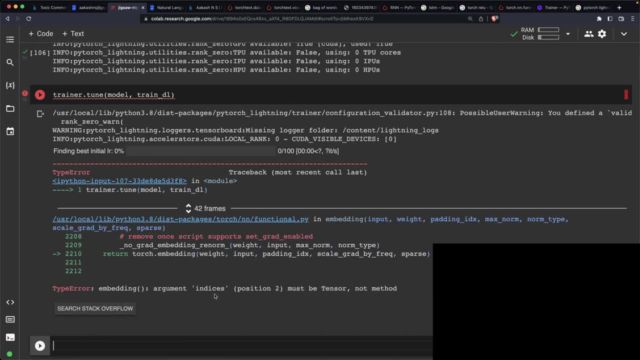 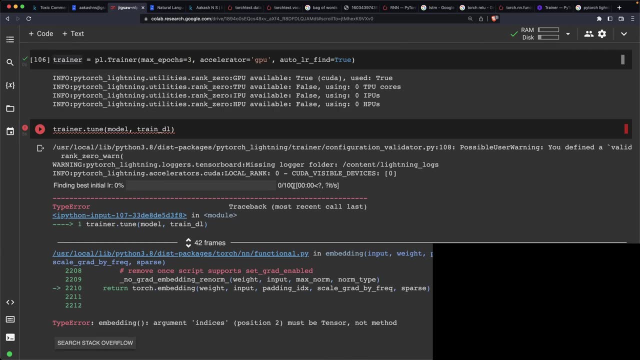 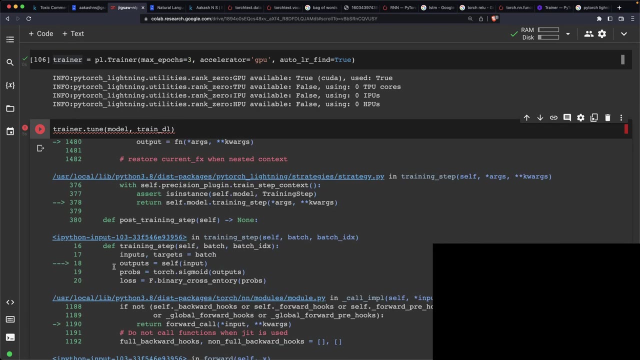 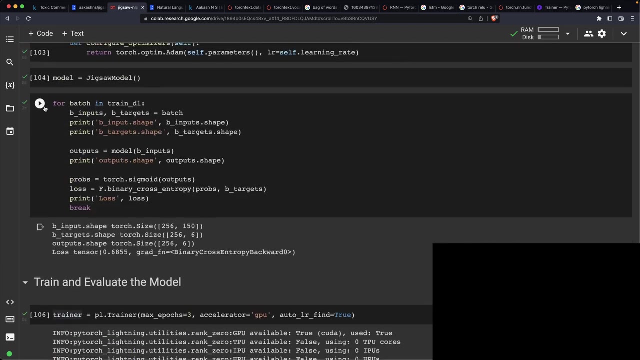 So what it's doing basically is trying embedding argument. indices must be a tensor, not a method. Okay, So we're going to go ahead and create the model here, or should embedding? Let's just check this out. Yeah, Let's just make sure that the data is getting passed properly. 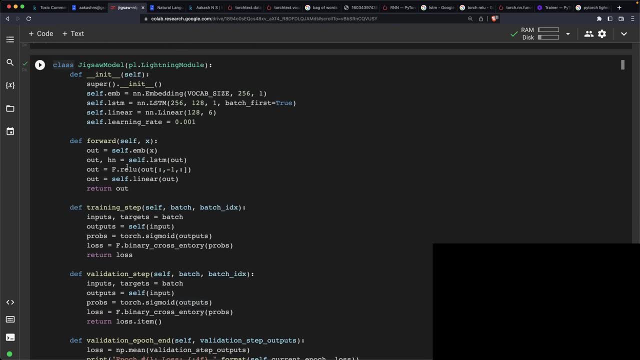 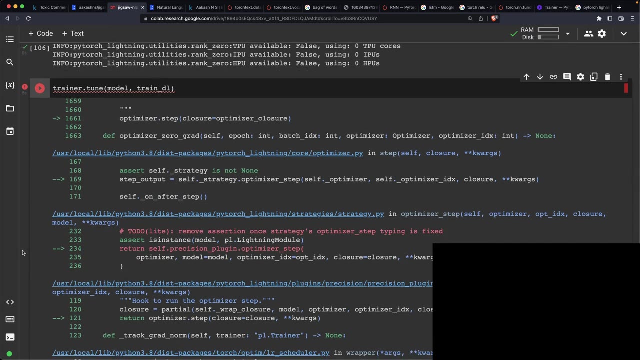 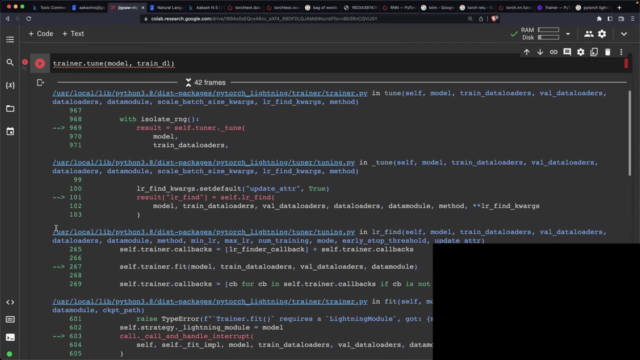 So we have- oh, we have- our LSTM to self dot LSTM. We have our embedding layer. That is fine. We have a relu, We have a self dot linear. All of this seems to be fine. This is what happens when you train live, but I think we should be able to figure out. 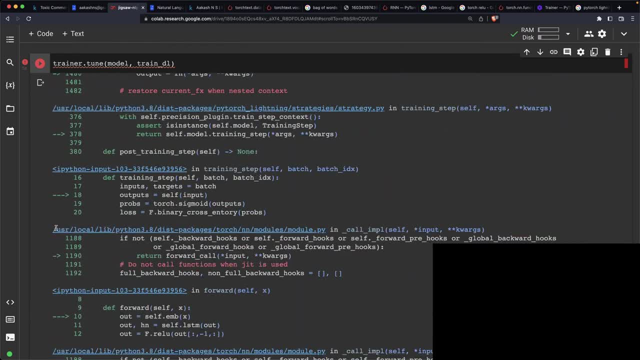 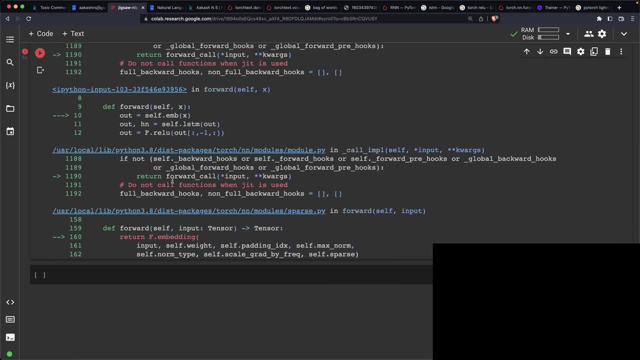 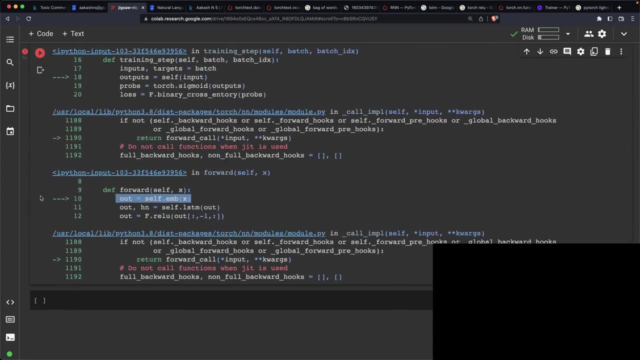 the issue. Let's see Where did we exactly run into the issue. So torture embedding is in F dot embedding, which is in the forward call, which is in self EMB And in self dot EMB. the error that we're running into is argument index indices. 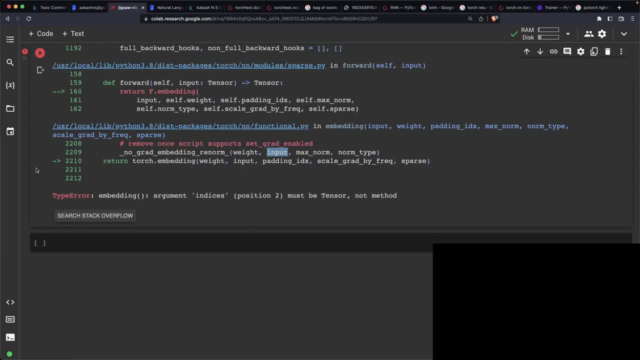 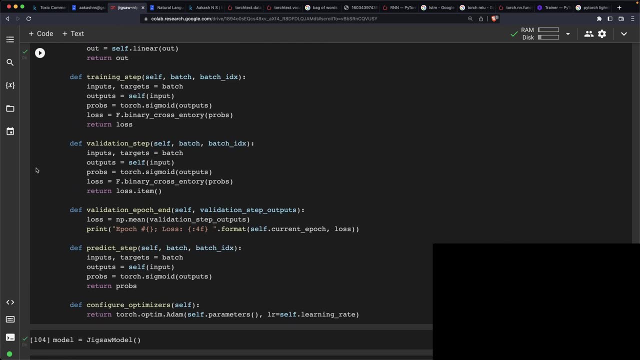 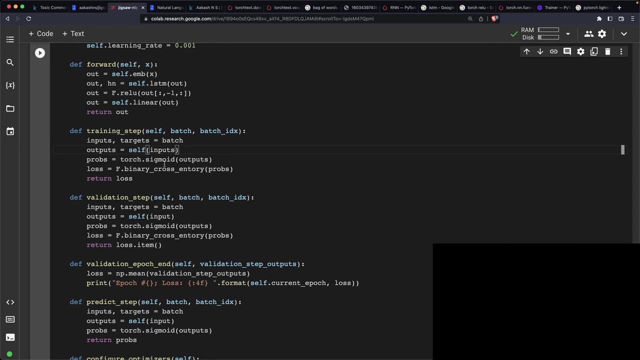 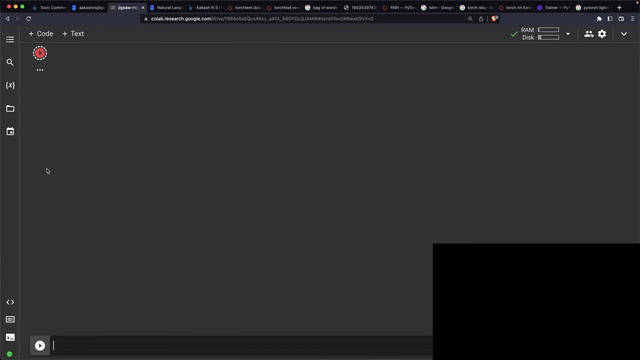 Position two must be a tensor, not a method for it. Okay, This should be called inputs, Not input. Yeah, So input is a method in Python and not an inputs is wrong. I mean input is a method in button. We should be passing inputs which we got from the batch. 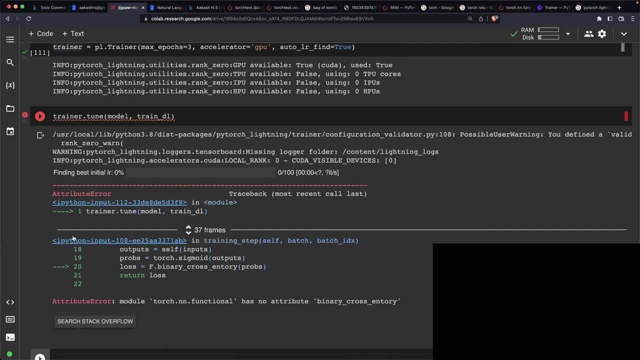 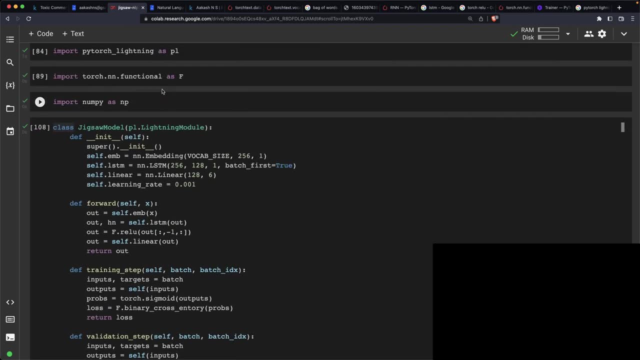 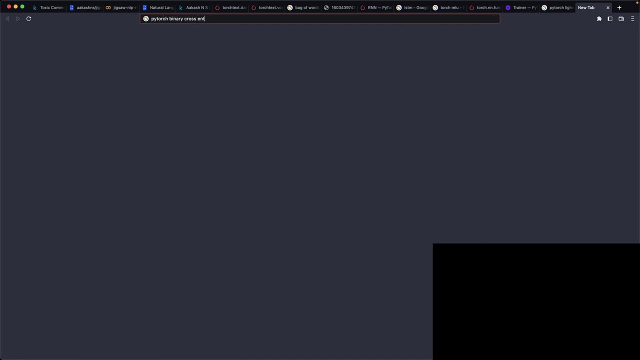 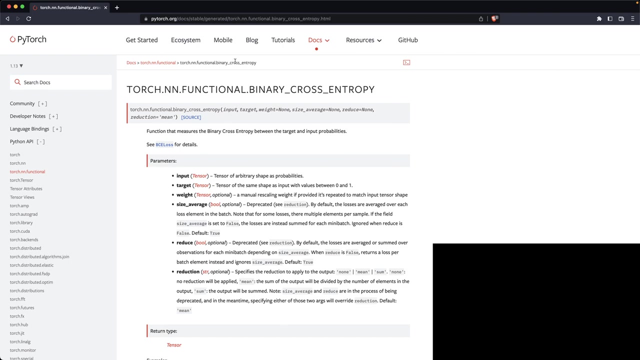 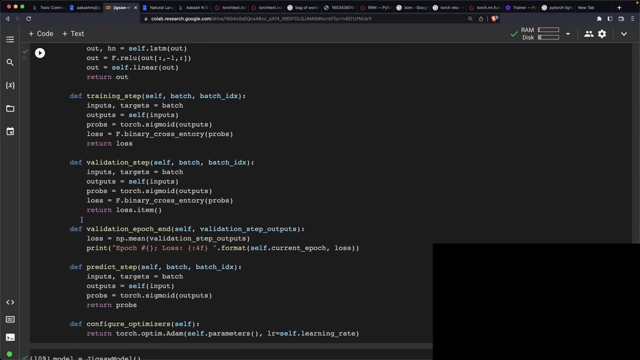 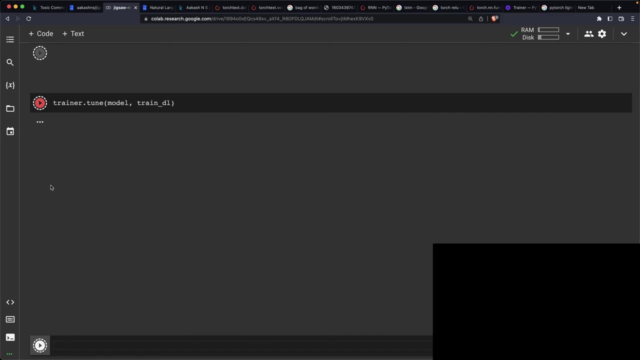 All right. So now we're trying to figure out a new attribute: binary cross entropy. What's happening? I torch binary cross entropy. it's called binary underscore, cross underscore entropy, Let's? ah, there is a spelling error, but now we are. we've created a trainer and now. 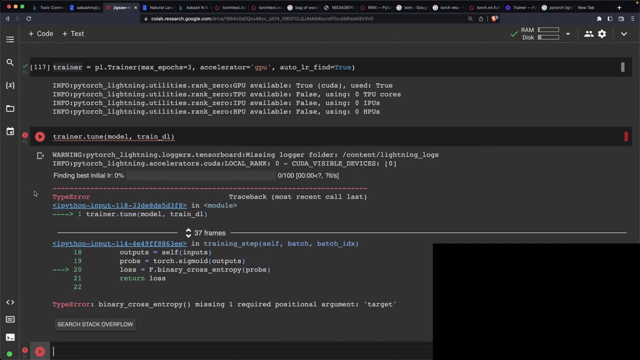 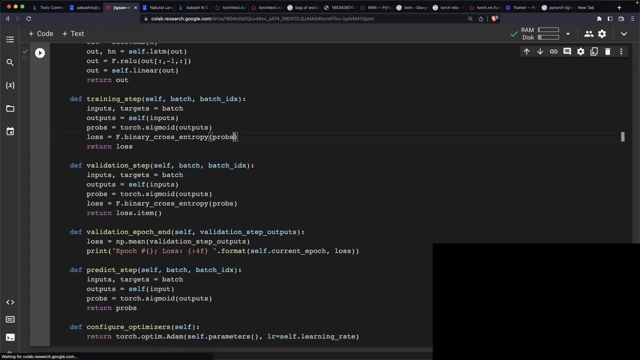 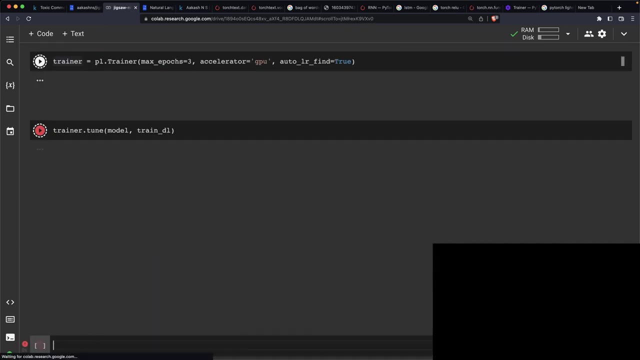 we are tuning the model, So now call. let's call train or tune. what else? binary cross entropy is missing. the one position argument, target. Of course we need to give it the set of targets as well, So it should contain not just the probabilities but also the targets. 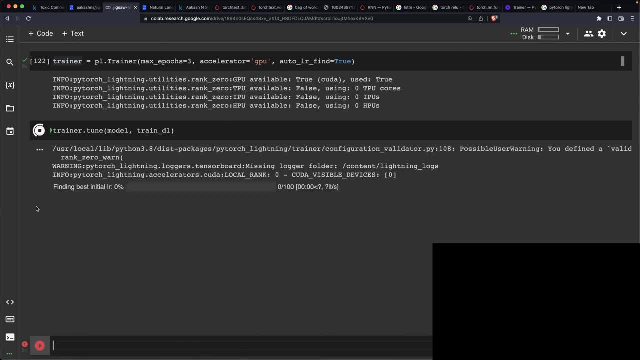 And this is generally how you create, how you write code in PyTorch. You try something and then it doesn't work, and then you fix it and then you move forward. Okay, So now it is finding a learning rate for us. So now PyTorch lighting has a way to figure out the best learning rate. 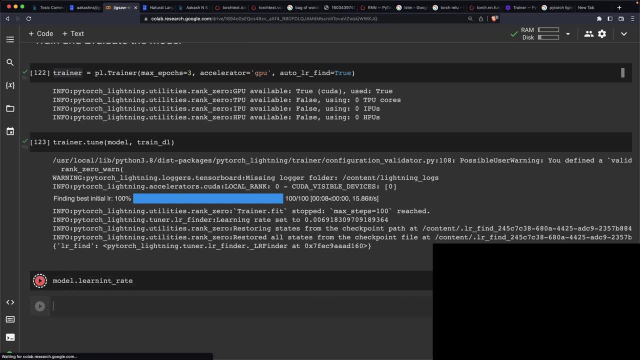 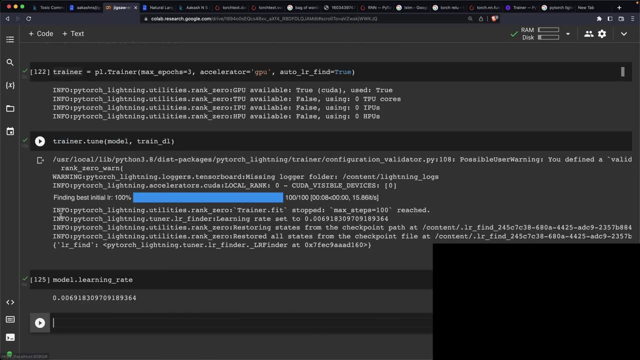 And now if we check model dot learning rate, Okay, It would have modified the learning rate If it could find a better one. if it could not find a better one, it would have left it as it is. So clearly it has found a better learning rate: 0.0069.. 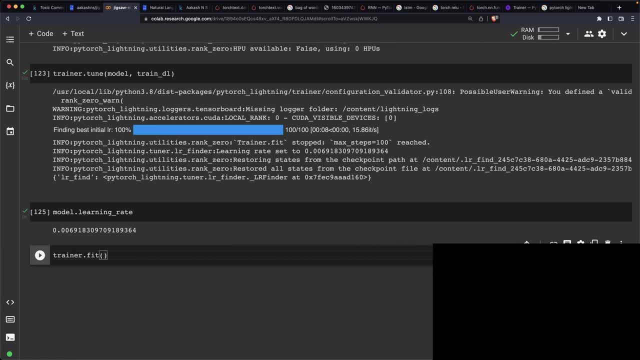 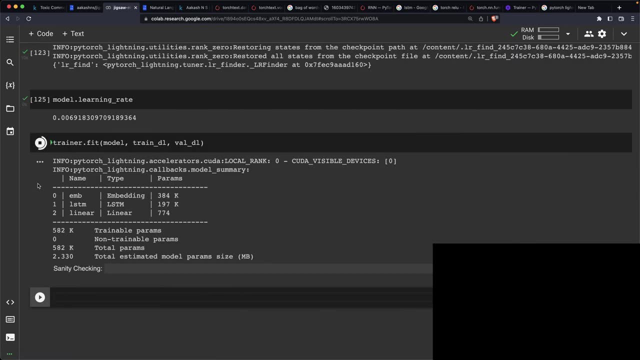 And now, like now, we can use the trainer to actually fit the model. So let's give it the model, Let's give it the training data loader, Let's give it the validation data loader, And now the model is going to get fitted for some time. 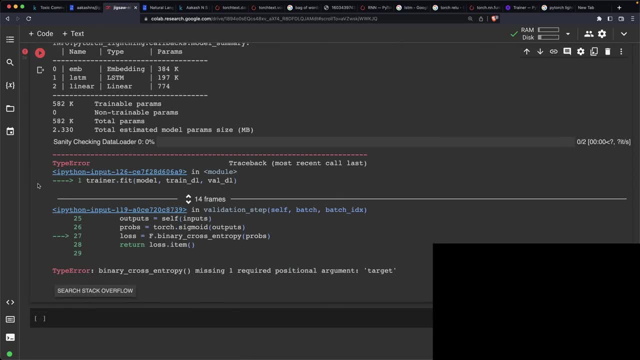 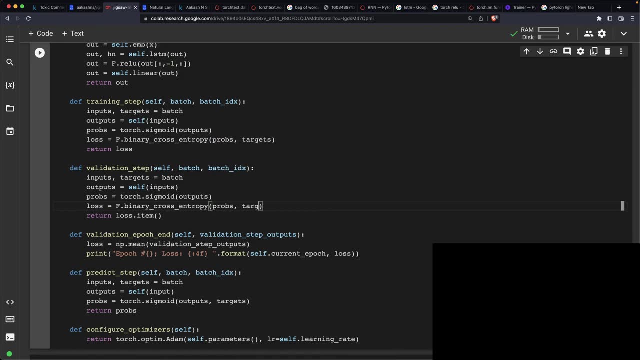 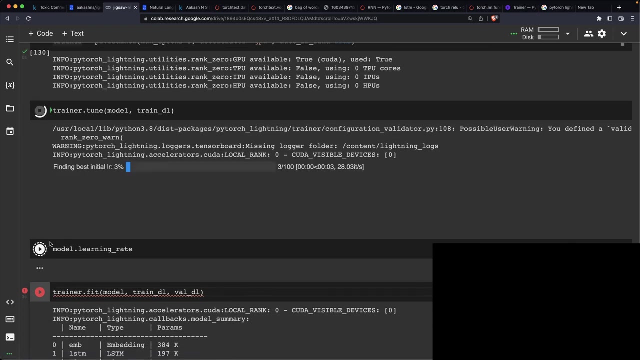 So it's going to put. so here's what is okay. Let's see, There is still one place where we are Missing. Yeah, Targets, All right. So we'll, we'll, we'll, let it find the learning rate once again, and then we are going to. 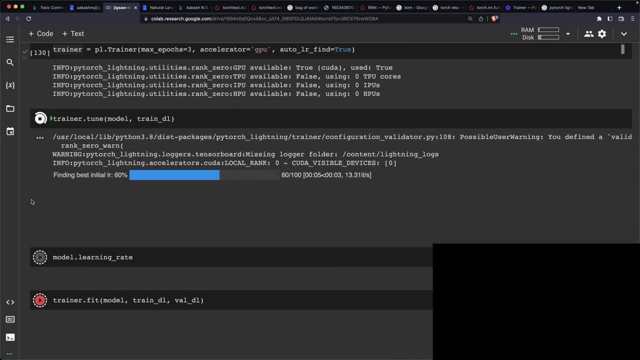 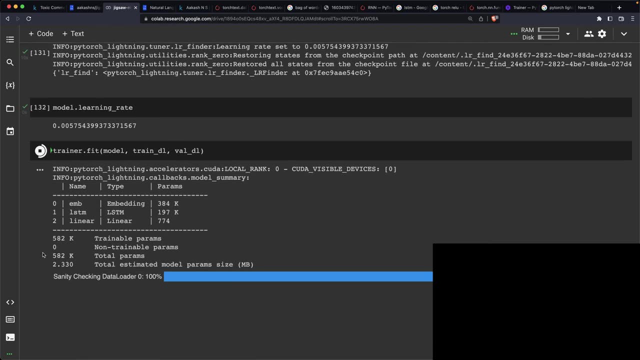 fit the model. So it has found the learning rate, the model, it has found the learning rate and now it is going to fit the model. The learning rate is 0.005 and it has started to fit the model. So what exactly is happening when it tries to fit the model? 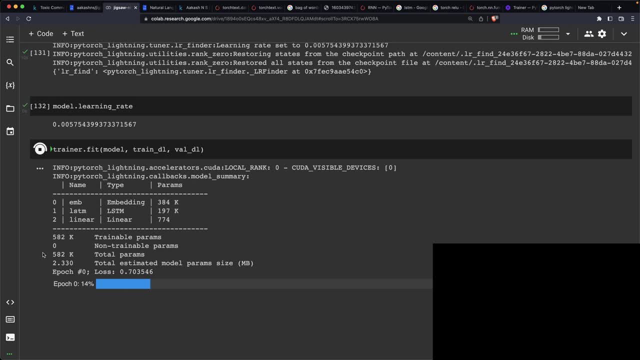 So the first thing that happens is the trainer picks up: Okay, The training data loader, So we've passed in a training data loader. It starts to get batches from the training data loader one by one. So it gets the first batch from the training data loader. 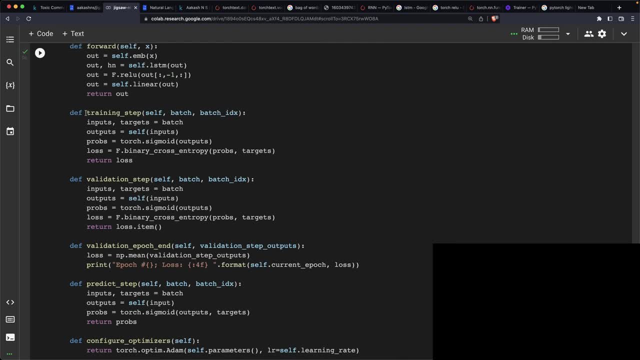 Then it calls the method training step on the batch. that calls the method training step that is going to get the inputs and targets on the batch. That's going to take those inputs and pass those inputs into the model and get some outputs. Then it is going to apply the sigmoid function to those outputs to get some probabilities. 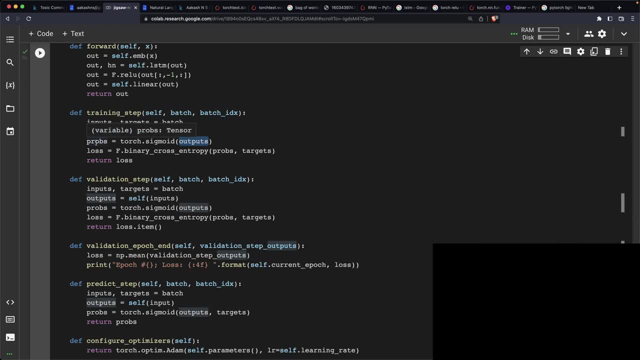 because the outputs We have a large range, but we want probabilities And remember we are getting six outputs for every row of data because we are predicting six classes. Then it is calculating a loss. So there are certain targets. Each row has a certain target: 0 1 0, 1 0, 1, something like that. 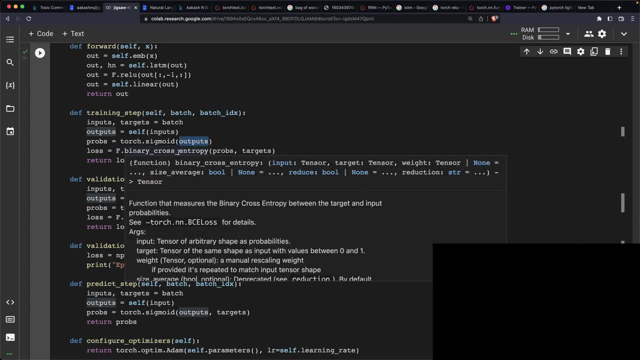 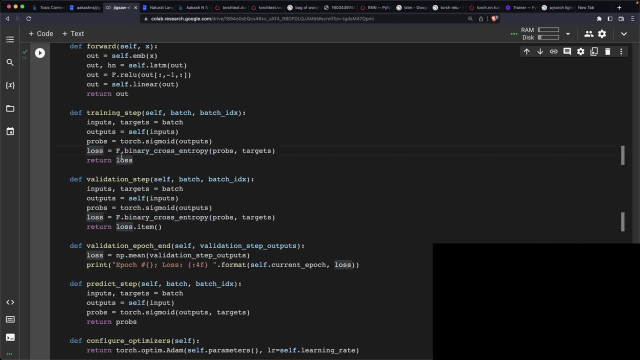 And each row, we have come up with certain probability, certain predictions, which could be values in the range of zero to one. after performing sigmoid, Then we compute the binary cross entropy loss and, using this loss, we then calculate gradients for all the parameters present inside the model and then, using the gradient, descent. 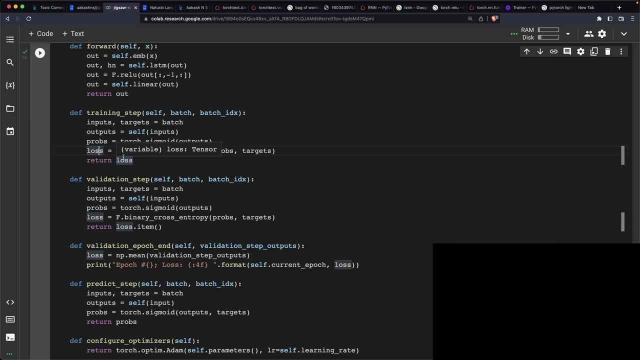 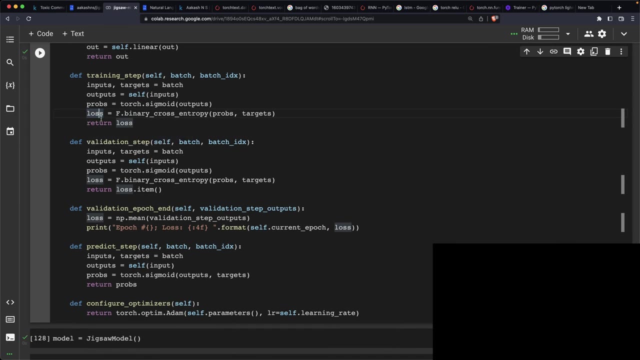 optimization technique, we slightly tweak all the parameters to make the model slightly better suited to make these predictions, to have a slightly lower loss the next time. And this is done batch after batch after batch after batch for the entire training set, And then, once all the training batches are complete, then it goes through batches of 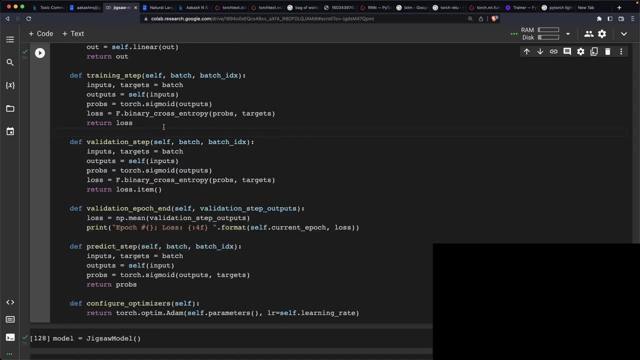 the validation set, And now it does not use this law, The validation set loss, To actually improve the model. it simply collects all the losses And then at the end of the validation epoch it is going to just compute the mean of the. 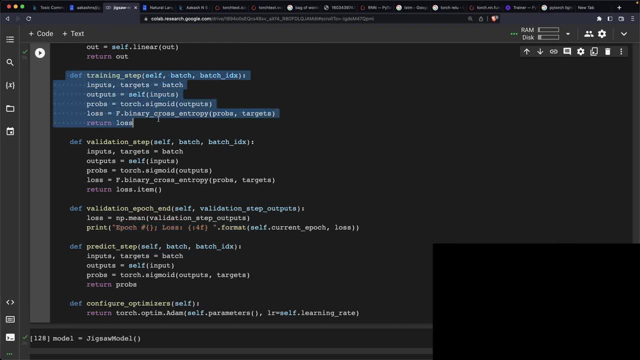 loss and it's going to just print it out. Okay, So that's what these three things are doing. Training step is used for training. validation step is used for simply evaluating on a batch and validation epoch and is used to combine the results of all the validation batches. 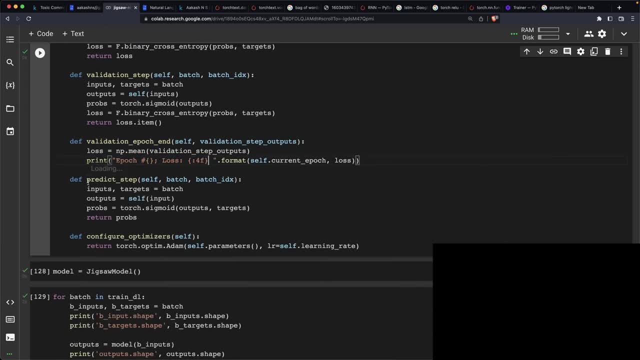 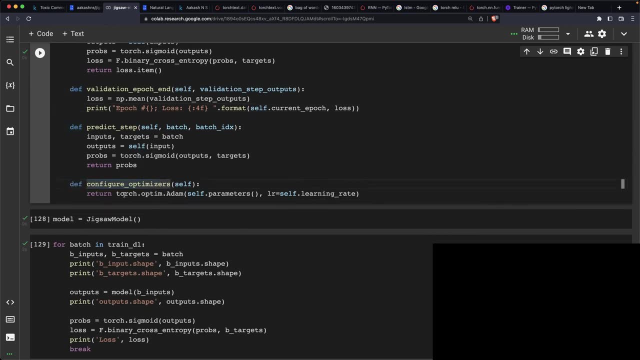 and print the overall loss And the predicts that will be used later when we are actually using it on the test data set. And in all of this the optimization algorithm, Loss reduced is determined by the optimizer that we have configured And in each batch the optimizer uses the learning rate that has been configured in. 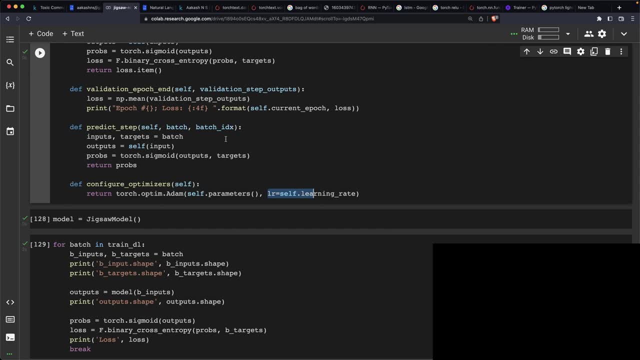 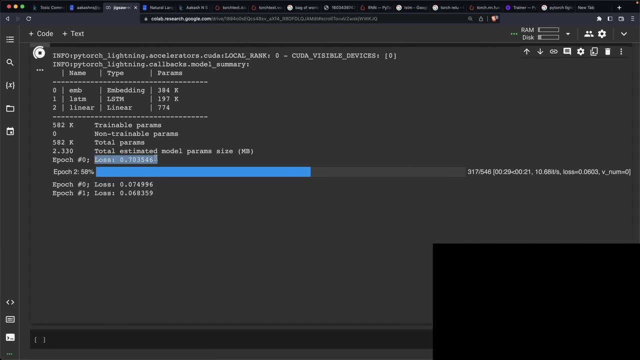 self dot learning rate, after tuning the model, after figuring out the right learning rate. Okay, So that's what is happening here. You can see that initially, before we even began, the loss was 0.70,, which would be matching the loss. 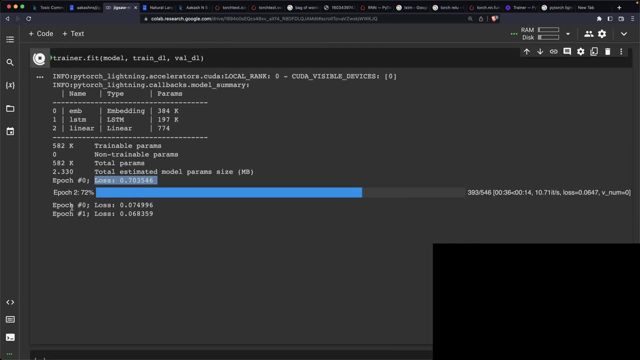 Yeah, which was, and this was a loss on the validation set. but then the model trained for one epoch And then the loss reduced to 0.07.. And then the model trained for one more epoch and the loss reduced to 0.06.. 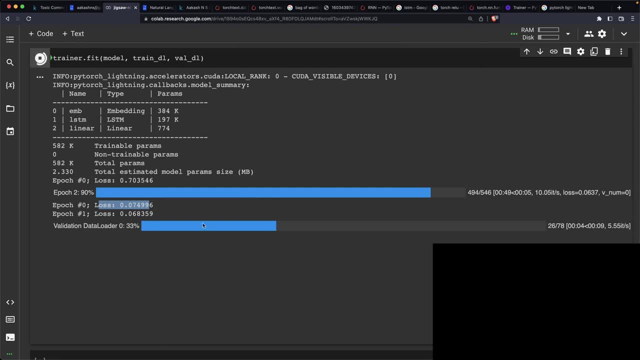 And now the model is training for the third epoch And hopefully the loss will go down even further. right, And this is what happens in machine learning or in deep learning. no matter what kind of model you're training, The loss is used to train the improve the model and slowly over time, the loss should. 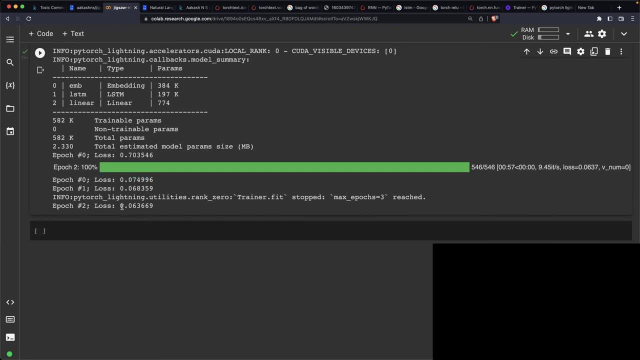 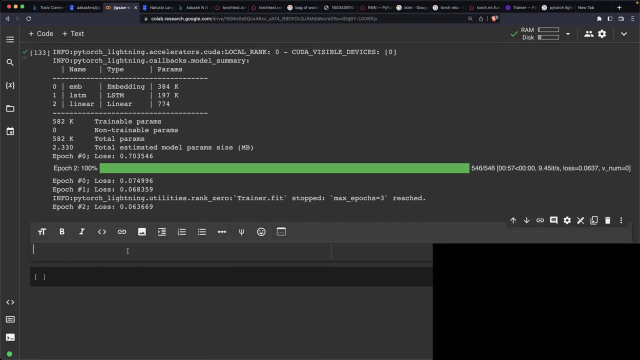 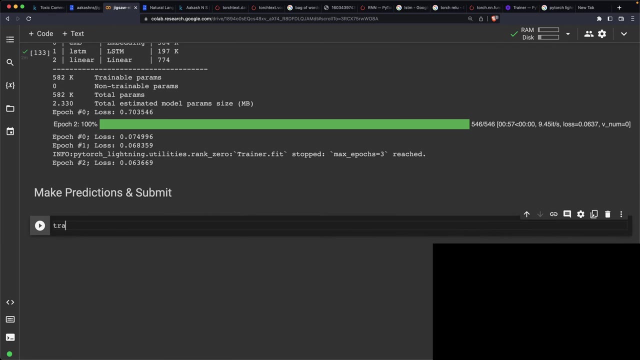 be going down All right. So it looks like we've reached a loss of 0.06, and let us now make predictions and submit. Submit them to Kaggle. So how do we make predictions? Here is how we make predictions. We can say: test Preds equals trainer dot predict. 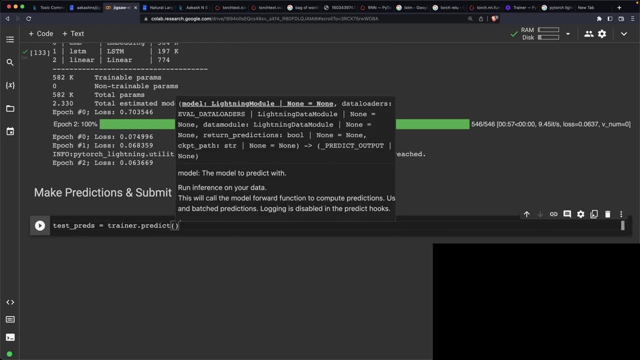 Now the trainer is also managing the whole GPU setup for for us. So it is going to put the training data on the GPU, It's going to put the model on the GPU, is going to get the outputs and bring them out of the GPU, and so on. 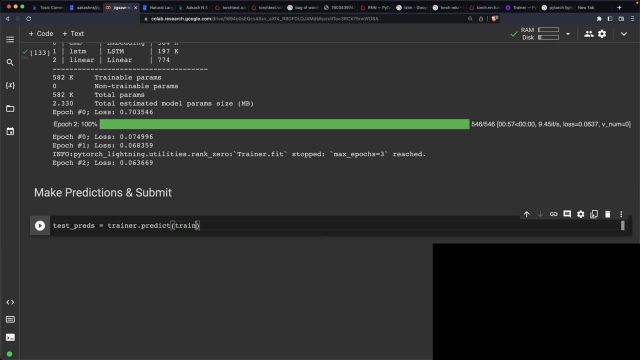 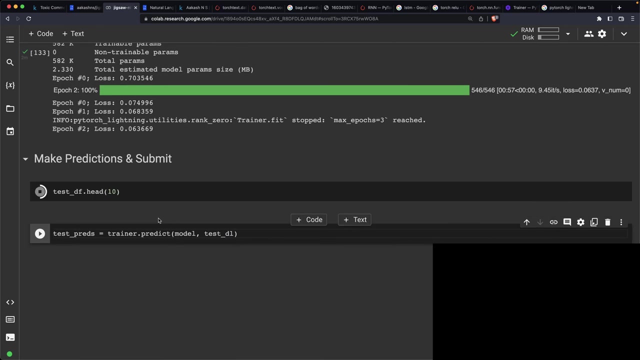 So test Preds equals trainer dot predict. Give it, let's give it the model and let's give it the test DL. And what does the test DL represent? The test DL simply represents the data from the test set. So see, this is the test set. or let's maybe just look at the first five. 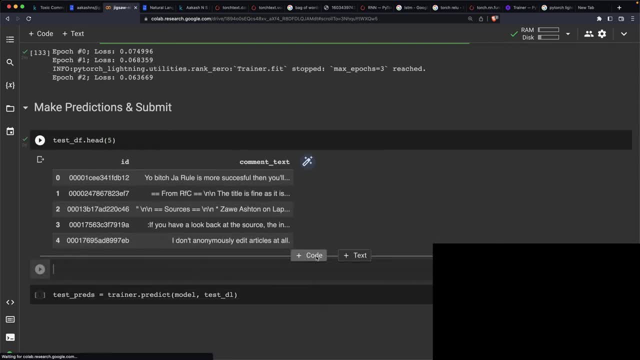 So this is what the test set contains. These are the first five rows of the test set and we can say for batch in test DL, we can just get like be in beat, Let's just call it B. inputs equals batch. Let's just print their shape. 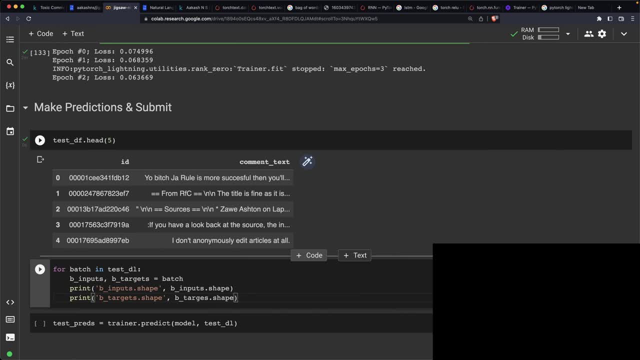 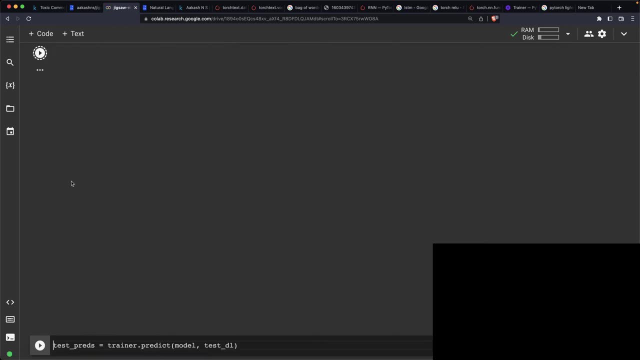 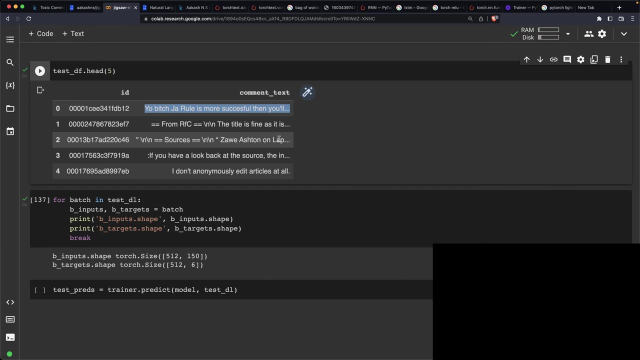 All right, So this is the test data loader, and- oops, I should probably. Okay, Let me break so that we just look at one batch of data. So the test data loader simply takes this and takes batches of 512 and converts each. 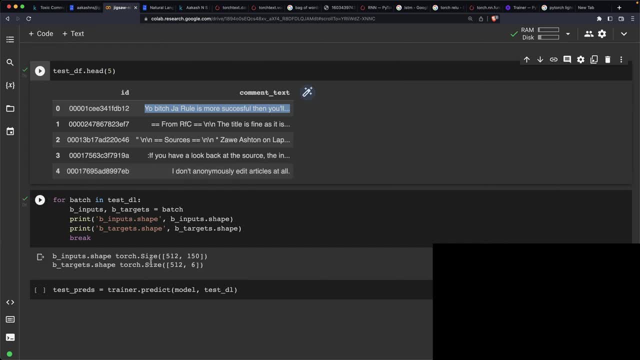 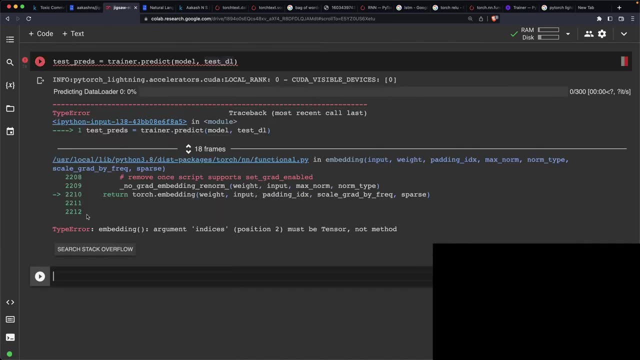 of these into tokens, then into indices and those indices. there are 150 indices And then those are going to get passed through the model when we call trainer dot predict, Okay, Once again, I think there is an error here that we need to fix. 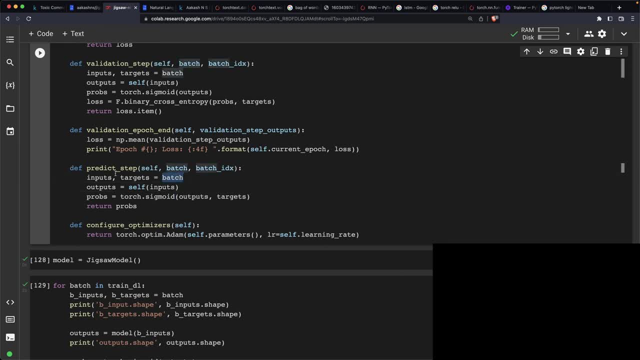 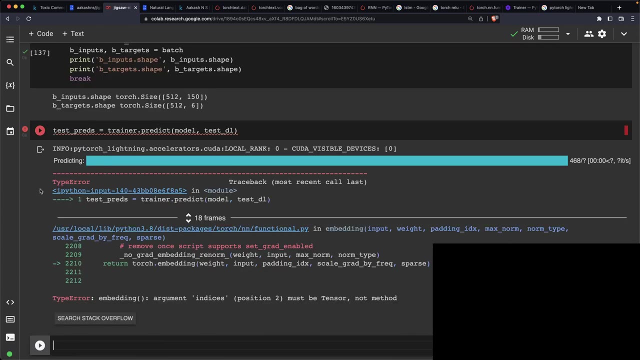 So this should say inputs. So we get the batch from the batch, We get these inputs, which is 256 cross 150, that gets passed through the model and we get six outputs or six results for each one, And then we are going to just get those results out batch by batch and put them together. 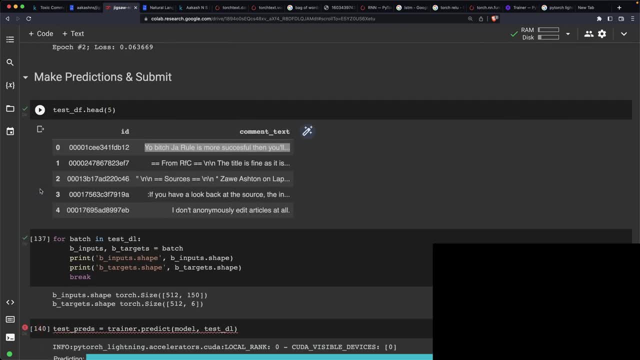 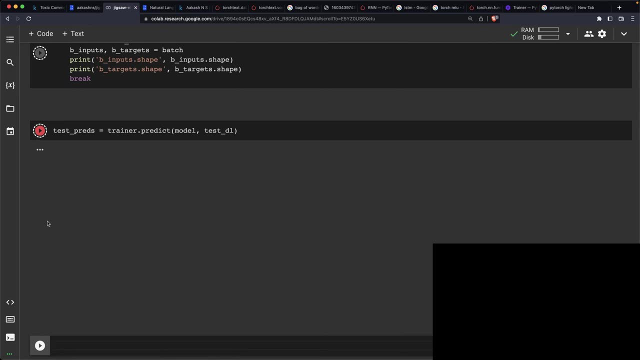 Okay, Argument indices. Oops, So the problem here is now: we'll have to retrain the model. So I'm just going to quickly retrain the model, because that error is present in the old model which we have already trained. Okay, 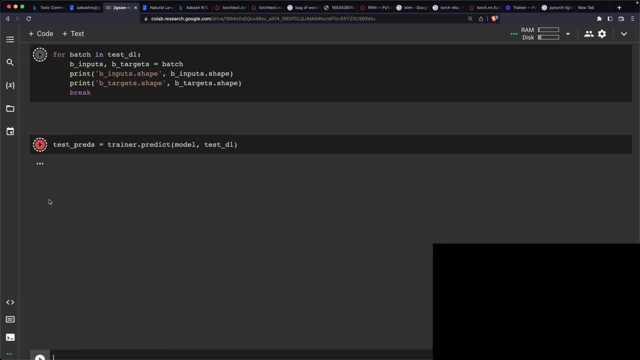 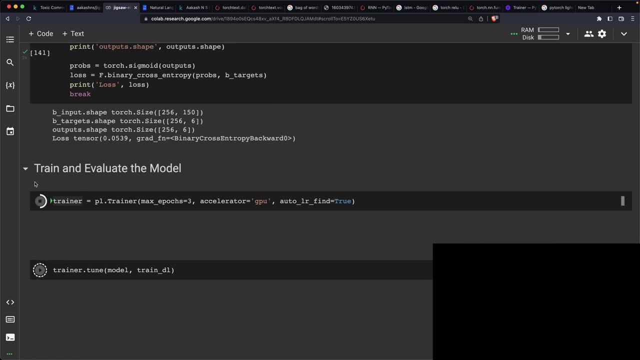 The model is. the new model that we class, that we defined, is not going to have the. there's not going to be without the error, So let's just retrain the model. That's going to take a few minutes, a few more minutes, but in the meantime we'll also. 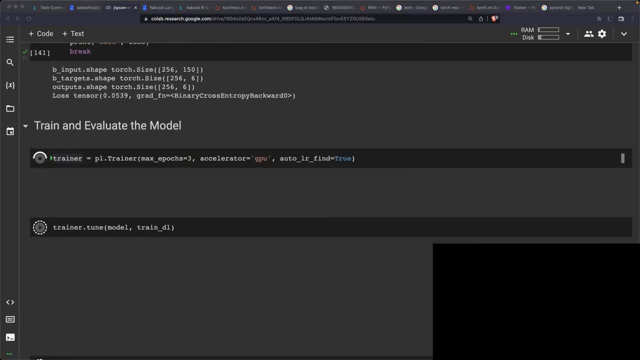 check if we have any questions. Okay, There is a question. Why are you using binary cross entropy If there are six classes? Well, the reason we're using binary cross entropy Is because this is a multi-label classification problem. So there are two kinds of classification problems. 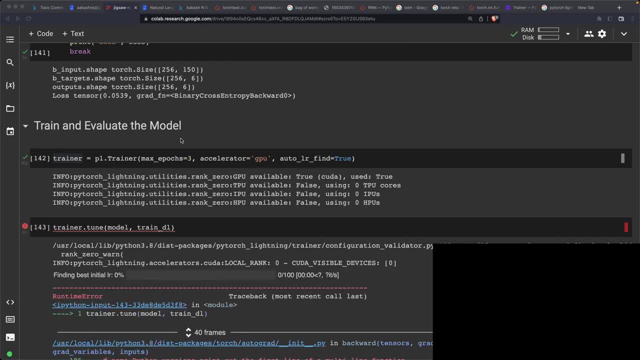 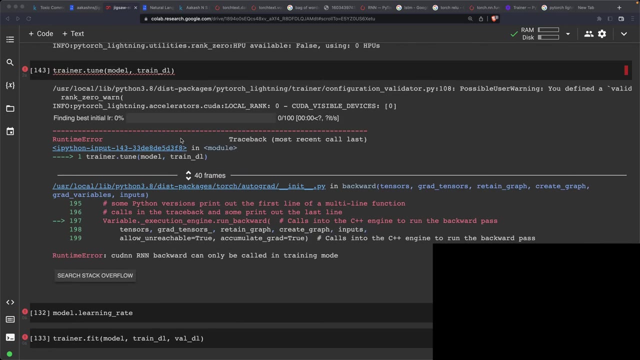 One is the multi-class classification problem, where one row can belong to one of many classes, For example the handwritten digit recognition. So one input image is only going to is only going to represent one digit, from zero to nine. on the other hand, 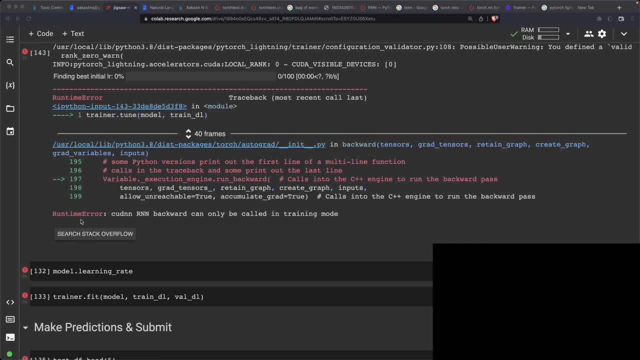 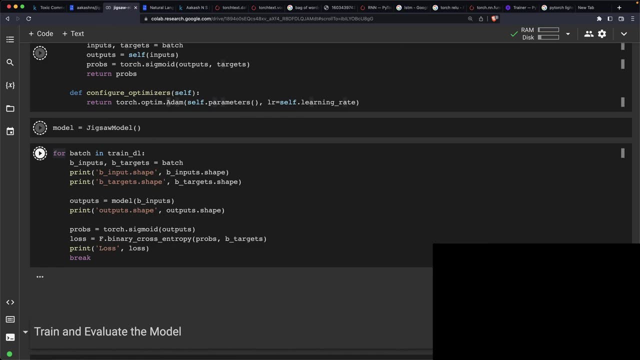 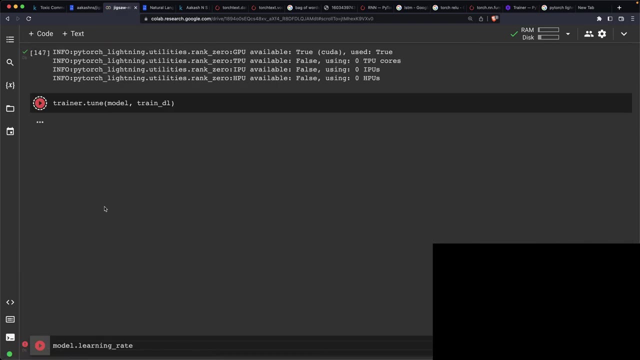 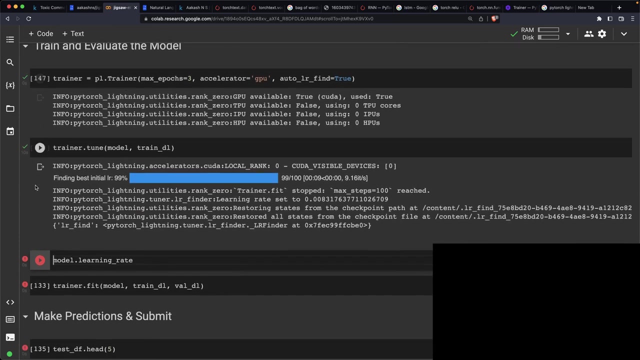 Okay, Well, it looks like. Okay, There is still something wrong here. Yep, So one row is yeah, So one row is only going to belong to one class in a single, in a multi-class classification problem, And that is when you use a normal cross entropy. 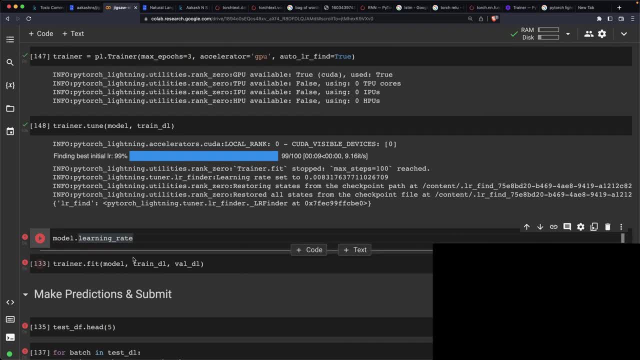 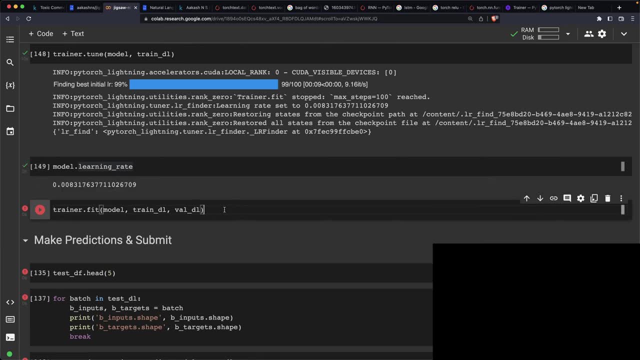 But in this case, one row can belong to many classes, And that is where we have to evaluate each class individually, And that's where we use binary cross entropy. Okay, So the model has now has a learning rate of 0.008, and now we are going to fit the model. 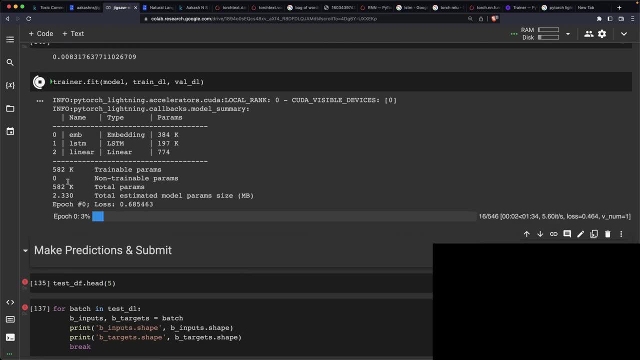 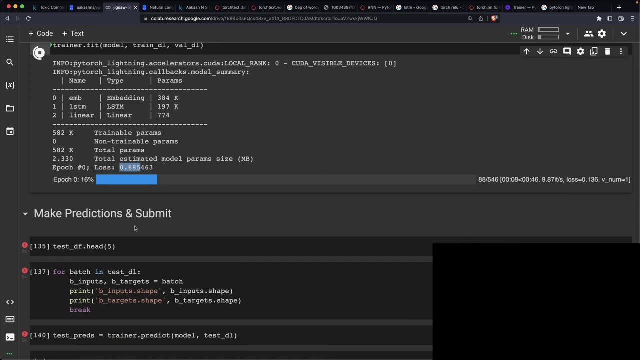 once again, and it's going to take a few minutes- two or three minutes- to fit the model. We start out with a loss of 0.68, but the loss is going to kind of keep going down slowly, And once we have fit the model, we can then make some predictions and then submit them. 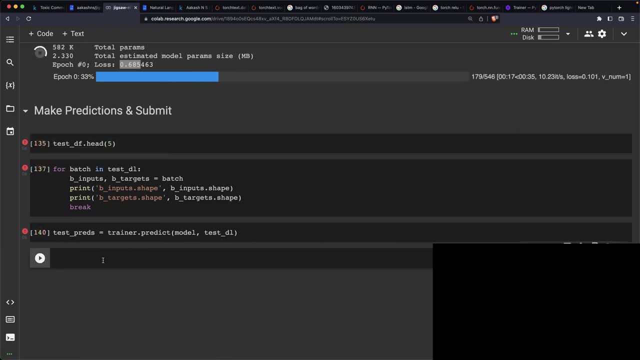 to cattle: Okay, predictions. i am also going to create a submission file, so we are also going to use the submission data frame and in the submission data frame we are going to take the predictions that we have obtained from the trainerpredict and then we are going to generate a csv. 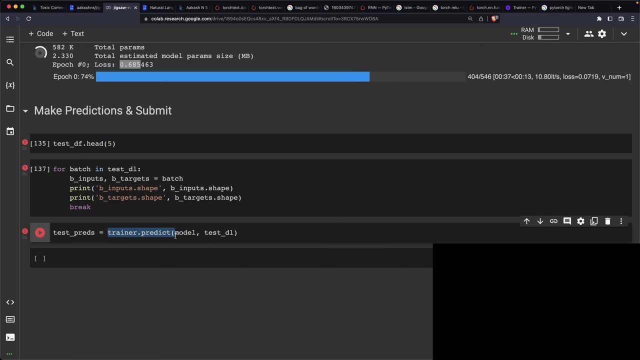 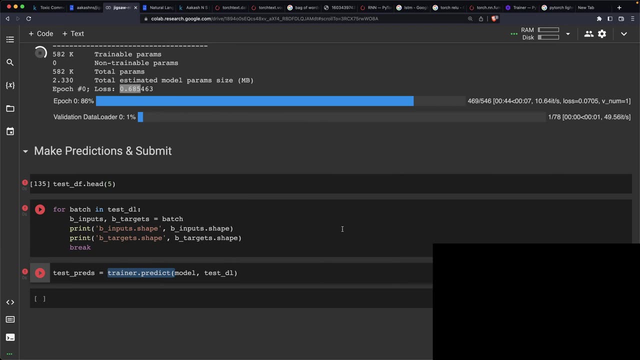 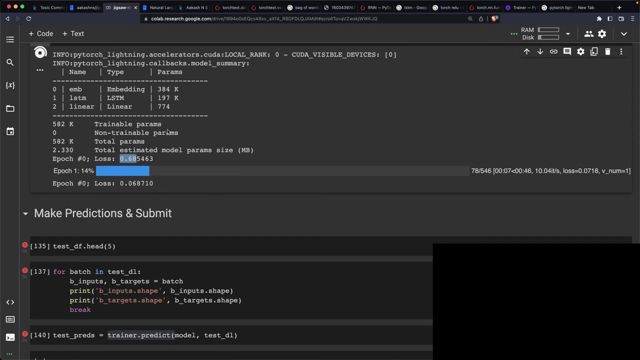 file and then we are going to put it on kaggle and see what result we get. so all right, so that was epoch number one. so we've already gone on from a loss of 0.68 to 0.06. now one thing you can experiment with here is try. 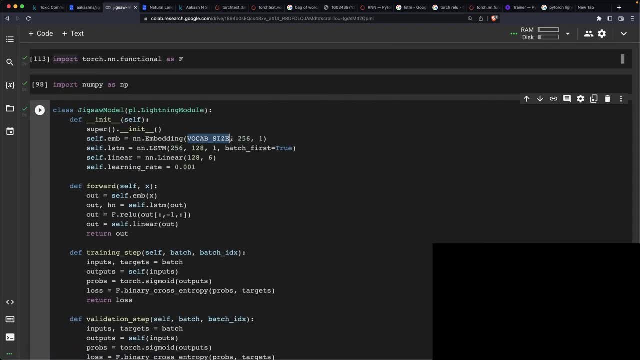 experiment with the parameters. try changing the vocab size by changing the batch size. try to experiment with the parameters. try changing the vocab size by changing the batch size, changing the embedding size, the word embedding size. try changing the number of layers in LSTM So you can actually stack LSTMs on top of each other. try changing. 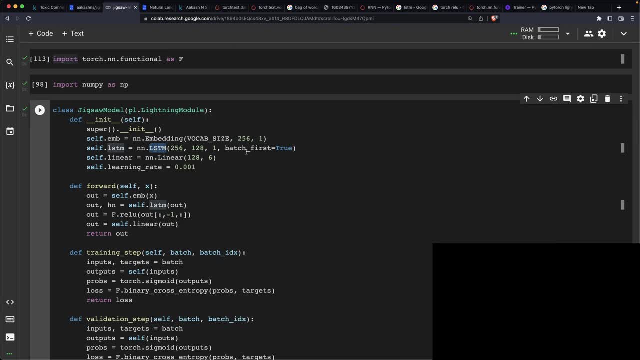 this to nnrnn. try changing this to nngru. then try changing. try maybe having multiple linear layers. try adding things like dropout Um, and try. you can also experiment with different activations other than the ReLU activation. Those are all the things that you can try and change. 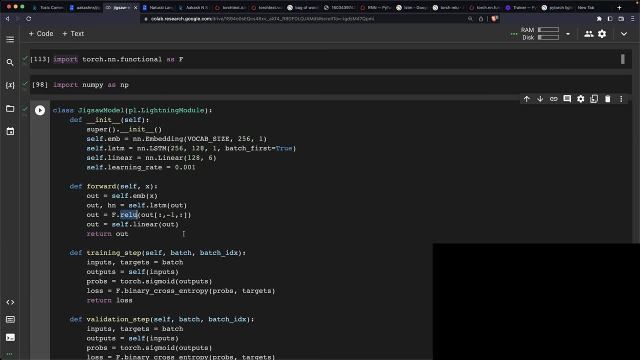 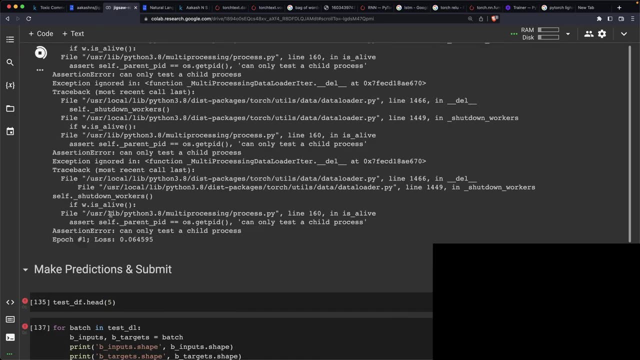 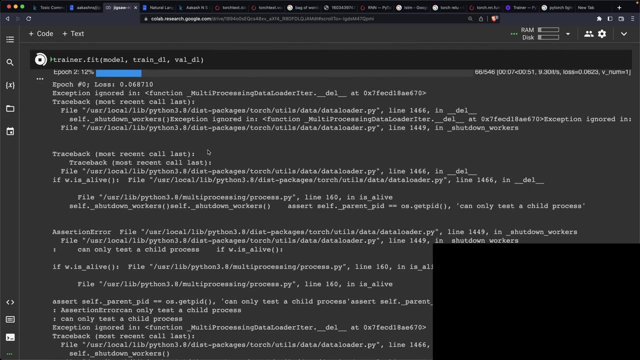 Of course, you can also change the number of steps. So right now we've picked max length of 150, pick a smaller max length or pick a larger max length and see what that gives you. Okay, So looks like there are some errors in terms of shutting down. 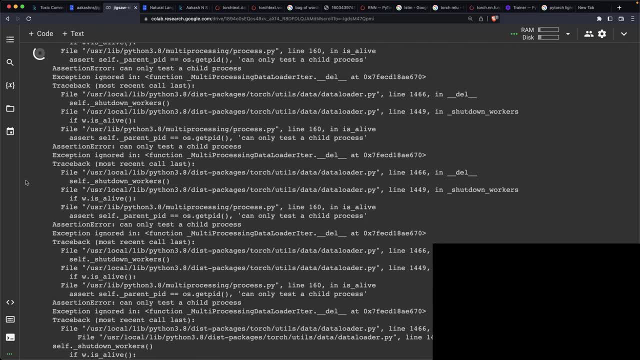 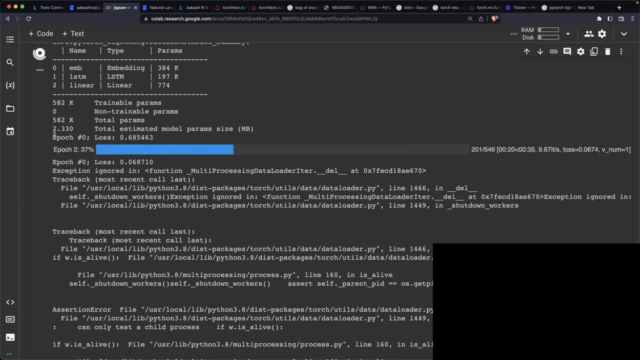 workers and things like that, but it seems like our training is still going on. fine. There is, I don't see, any issue with the training itself. In a few seconds, our second epoch should be done, our third epoch should be done, and then we will be able to make predictions. 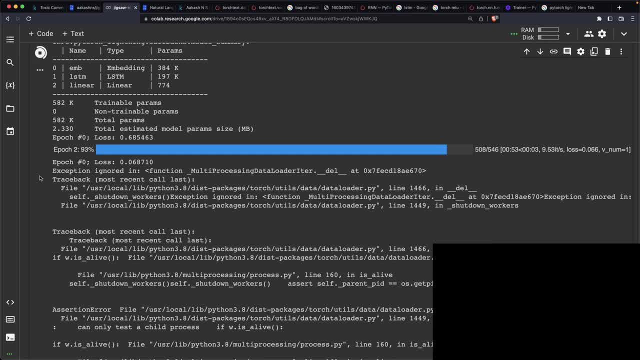 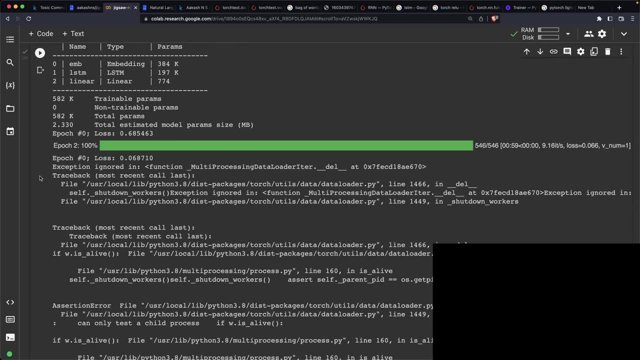 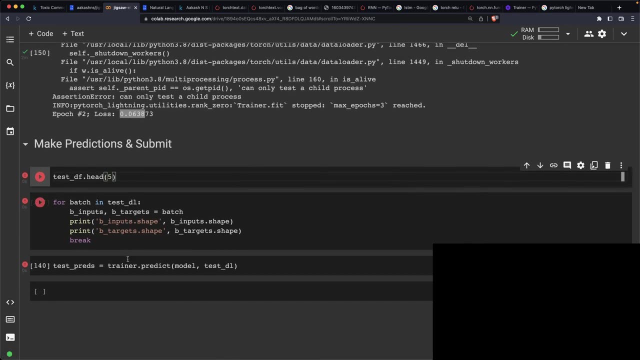 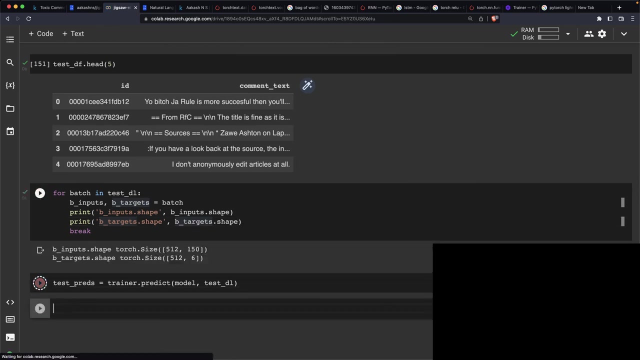 All right, So it looks like our model has finished training. Yeah, And we have reached a loss of 0.638.. That's great. That's less than one 10th of the loss that we had initially. Okay, So now we have this training and now we are passing the test data into. 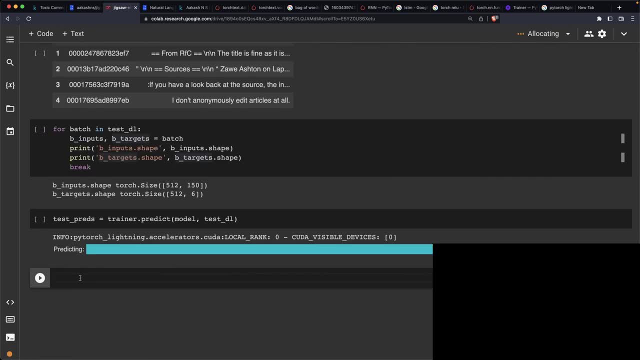 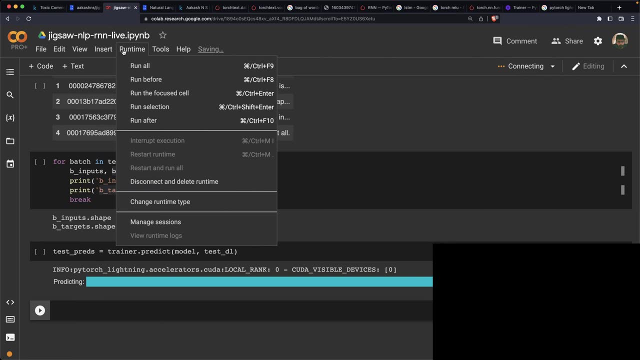 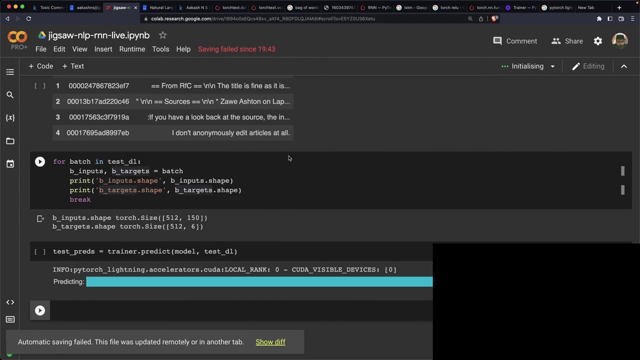 trainer dot predict and that is going to make all these predictions for Us. Okay, It looks like something crashed. I think I'm going to have to restart this. So, yeah, I'm going to have to restart this runtime and let's. 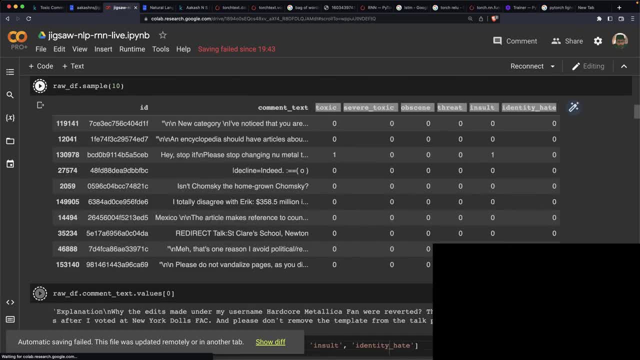 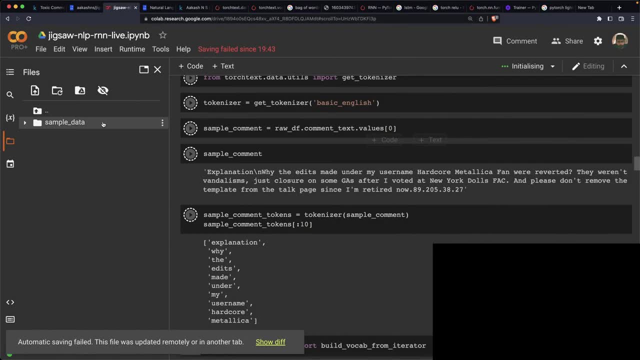 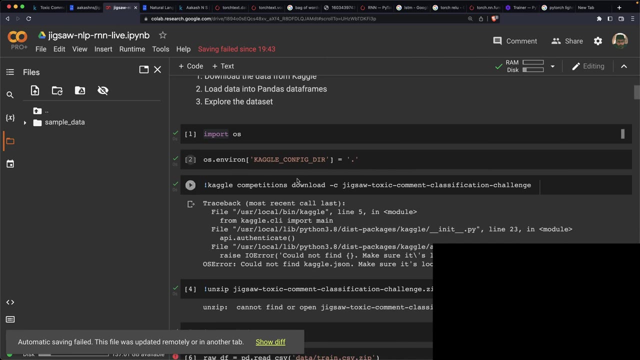 just run this from the start. Of course I'm also going to have to upload the Kaggle JSON file. Let me do that as well. Let's upload the Kaggle or JSON file again. Okay, Now we have the Kaggle or JSON file. 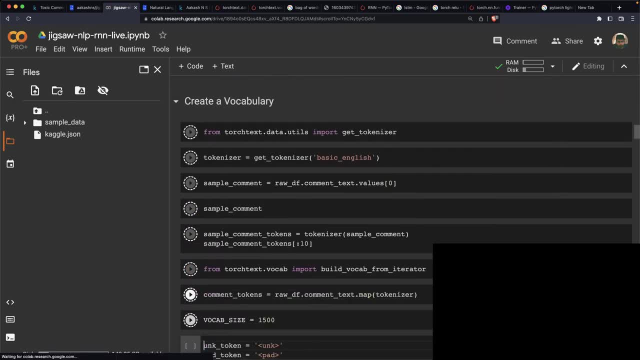 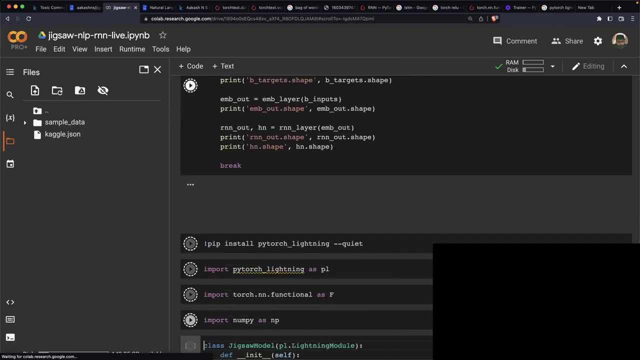 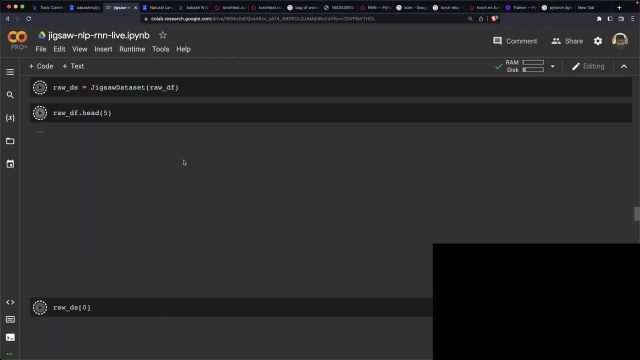 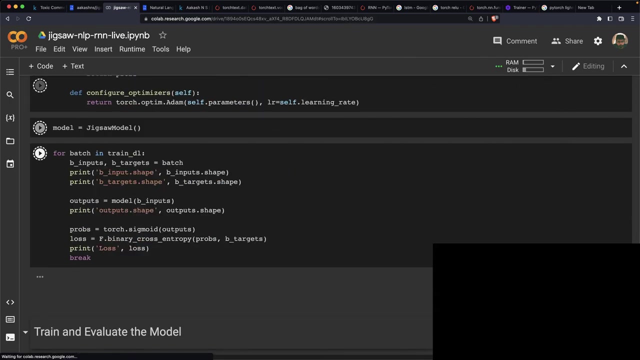 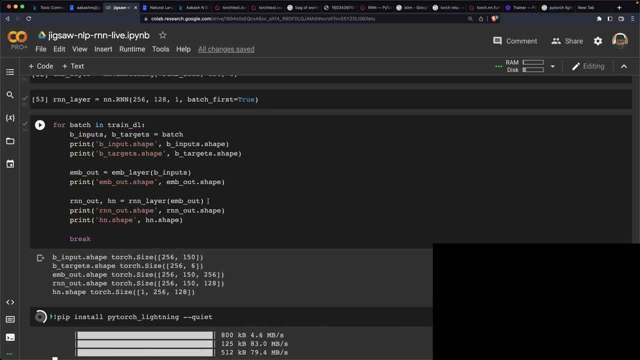 Now we can read on all of this, Probably also a good time for us to just recap exactly what we have done. while all of this reruns, Let's just run it all the way to the bottom And then, Okay, Pytosh lightning is installed. 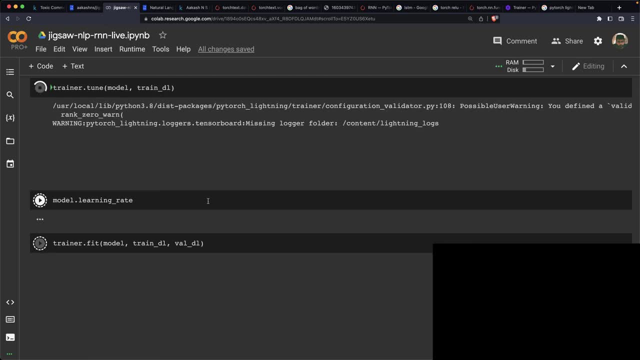 The model is created. The model is getting tuned. Great, The it is finding the best learning rate for us- Once again, Awesome, Okay, So let's see if we can get my learning rate. Good, We have the learning rate right now. 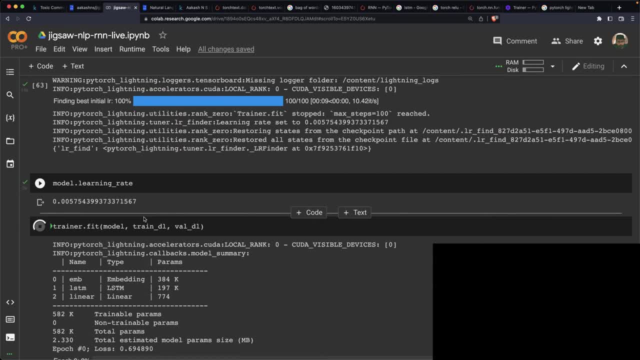 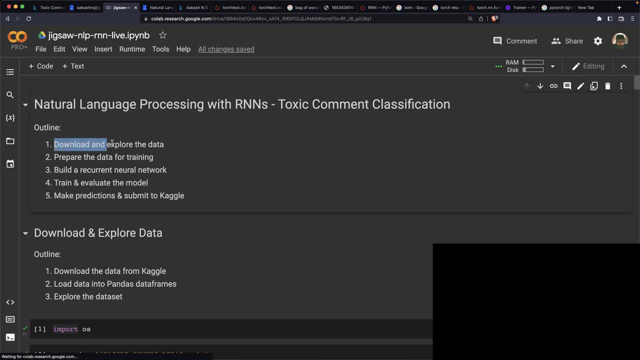 You can see it's learning. It is now training the actual model, so the best learning rate is 0.005 and the model is getting trained. Okay, So right from the top. today we looked at how to download and explore a dataset from 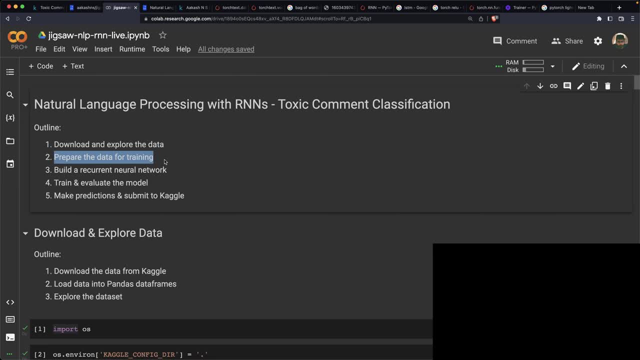 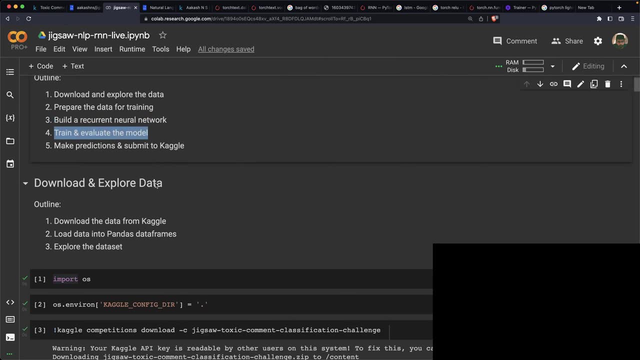 Kaggle. Then we looked at how to prepare an NLP dataset for training using PyTorch, using RNNs, We saw how to build a recurrent neural network and then we are currently training and evaluating the model. And finally, we are also going to make predictions and submit to Kaggle. 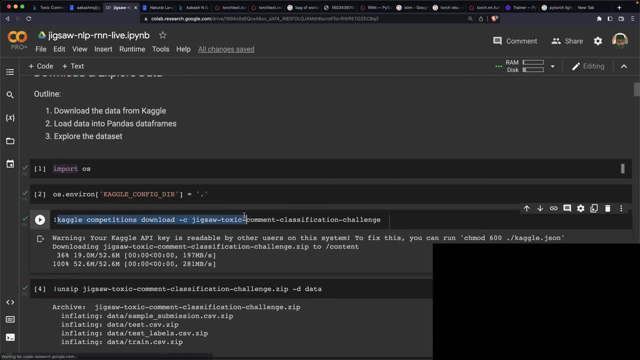 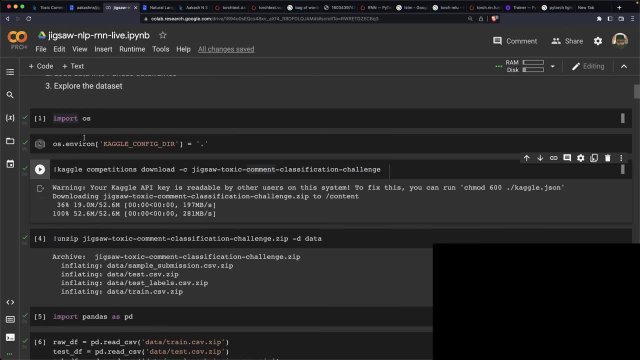 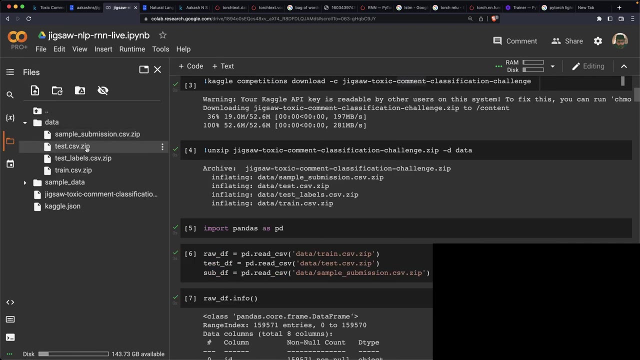 So to download the data we are using the Kaggle command line tool And to do that we have to upload our Kagglejson file, which comes from our Kaggle account settings, and set the config directory to the current directory, And then we also unzip the data into the data folder which had a strain test and submission. 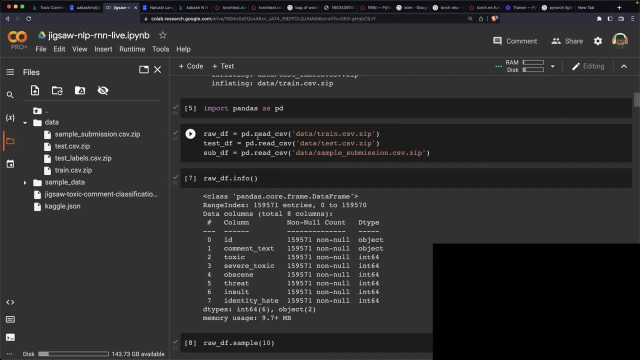 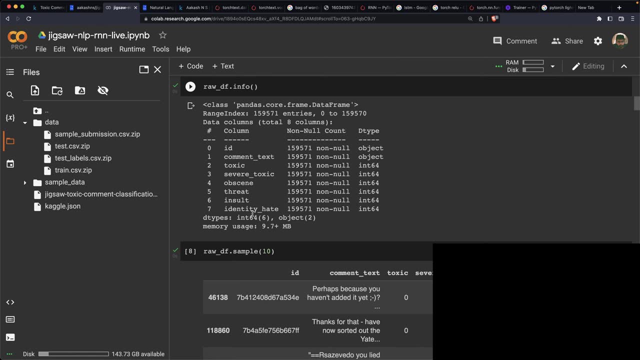 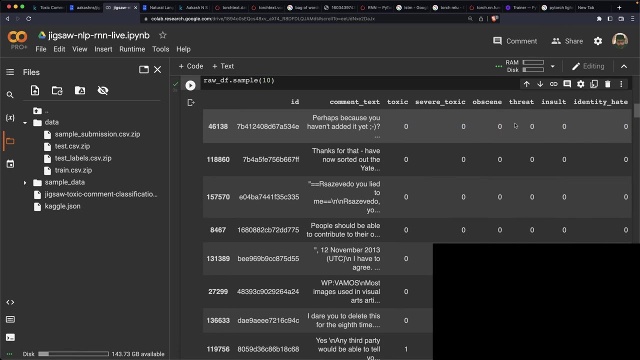 CSV zip files. Then we use Pandas to read these CSV files And we saw that the test, the training data, had about 159,000 rows And it contained a common text and then it contained six labels. Now this is a multi-label classification problem, which means one row can have many labels. that 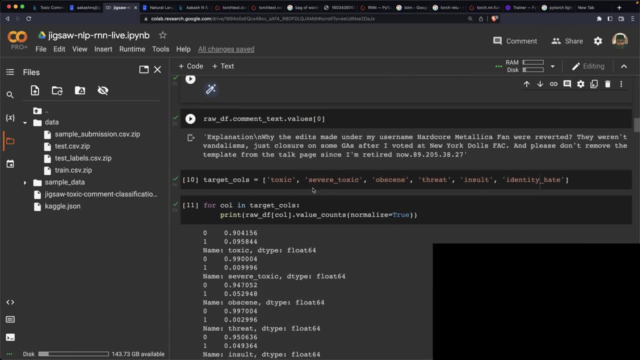 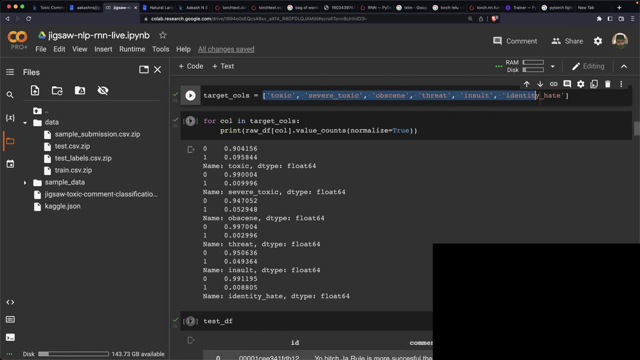 can contain multiple ones. Then we looked at individual common texts as well And we saw that the target columns had different distributions, but mostly- over 90%- of them did not fall in the category zero. So there's something we might have to do about the class imbalance at some point as well. 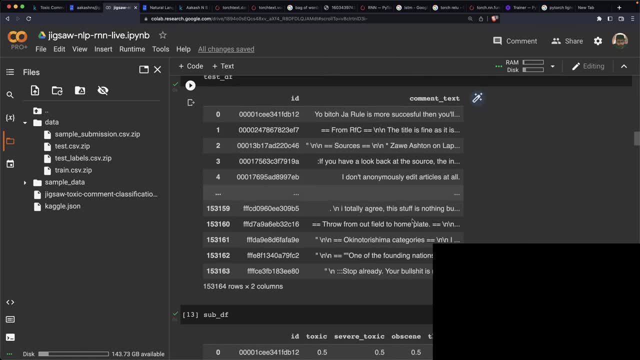 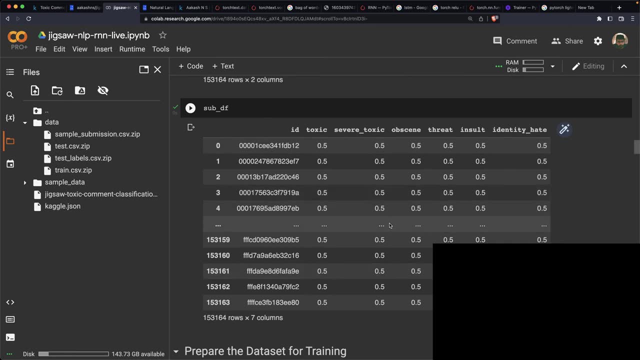 Then we looked at the test data frame. So in the test data frame we simply have the common text and we have to make predictions for each of these comments And we have to put them into the submission data frame and generate a submission file. 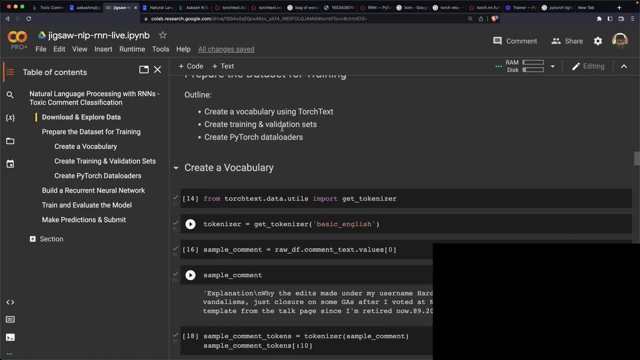 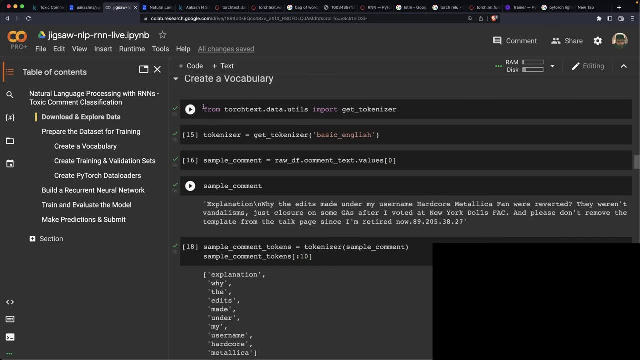 To prepare the data set for training, we decided to create a vocabulary using Torch text And then we created training and validation sets and then we created PyTorch data loaders. So we created a vocabulary from Torch text. First we created a tokenizer, a basic English tokenizer, which can take some text. 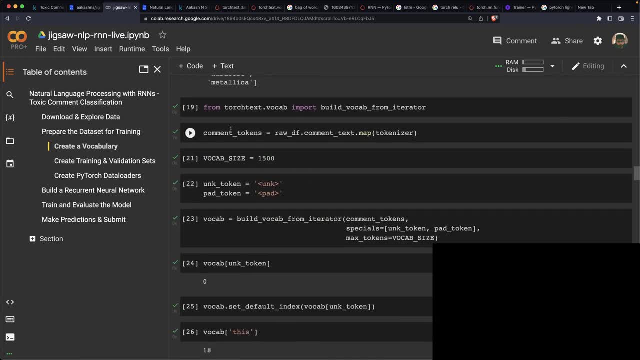 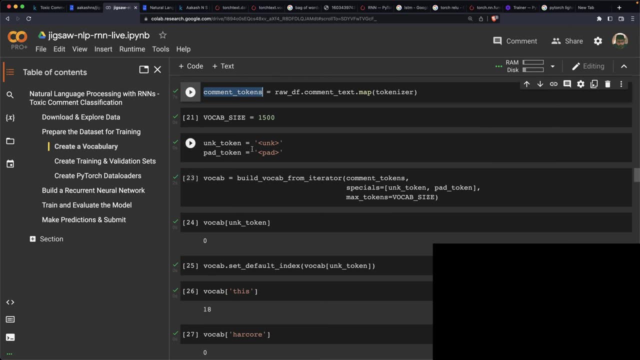 And convert it into tokens. Then we took all the common texts and map them or map the tokenizer onto them to get common tokens. And then we created the vocab using build vocab from iterator. We gave it the common tokens, we gave it the vocab size of 1500. 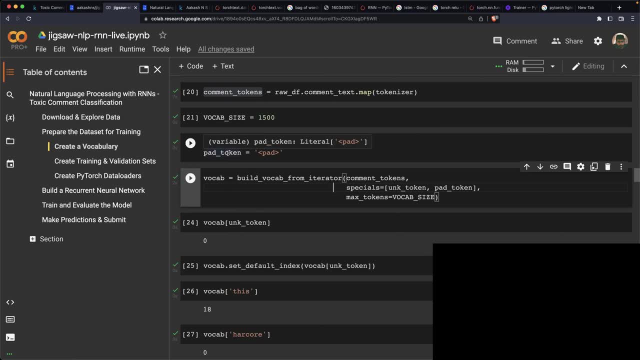 And we gave it the unknown token and the pad token, two special tokens: Unknown would be used to represent words which do not occur in the vocabulary, and pad would be used to increase the length of shorter sentences. Okay, And we looked at how we can use vocab. 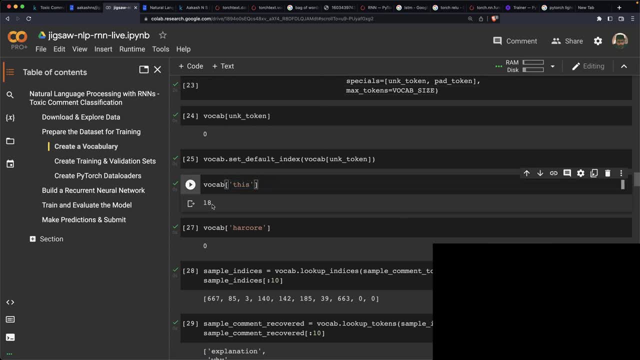 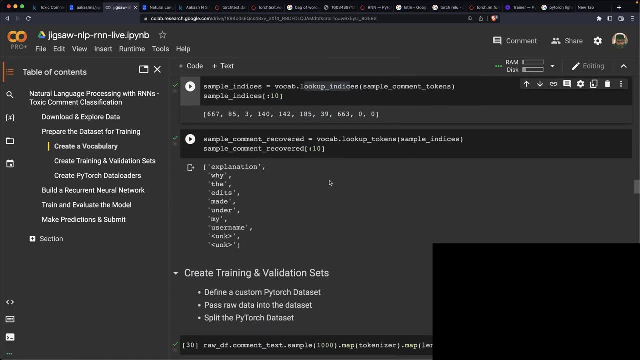 So we can give it directly. We can give it a word, a token, and it can give us the index of the token. or we can call lookup indices- give it a list of tokens And it's going to give us a list of indices. or we can call lookup tokens: give it a list. 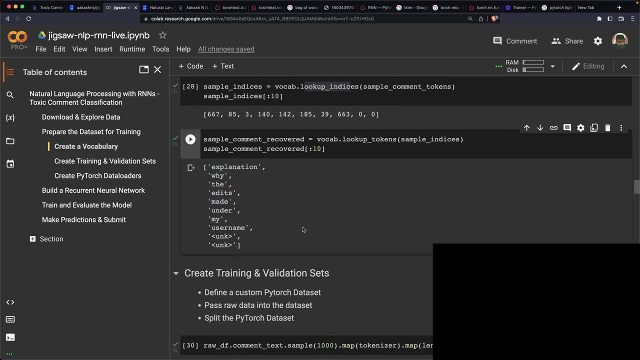 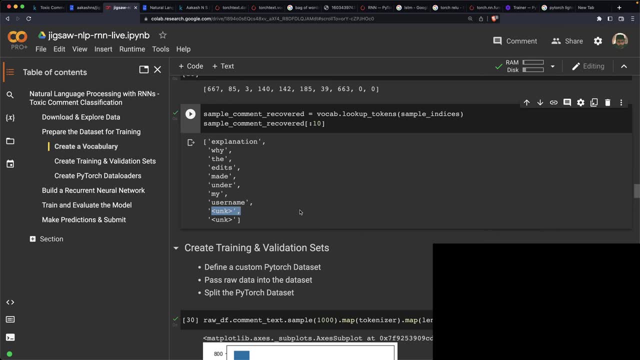 of indices And it's going to give us the tokens. Now, of course, when we are looking up indices, if a token is not found in the vocabulary, then the index used is the index of the unknown token, Because we've set the default index. 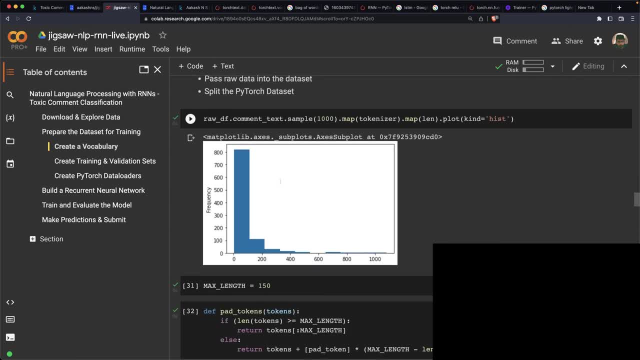 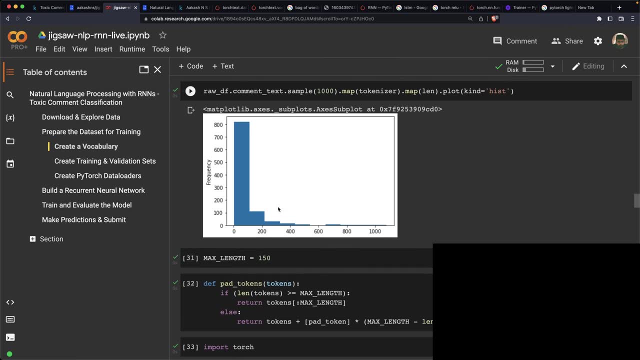 Then to create a training and validation set. the first thing we had to decide was what is the max length we are going to set for each vector? So we looked at the distribution of lengths of the comments and we picked the max length of 150, 150. 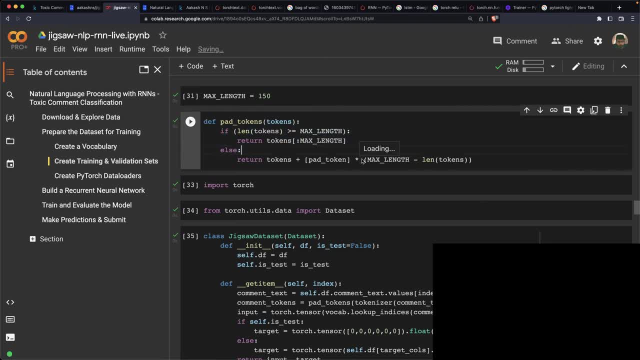 And then we created a pad tokens function which is going to trim any common text which contains more than 150 tokens to exactly 150 tokens, And if something contains less than 150 tokens, it's just going to add the pad token to make. 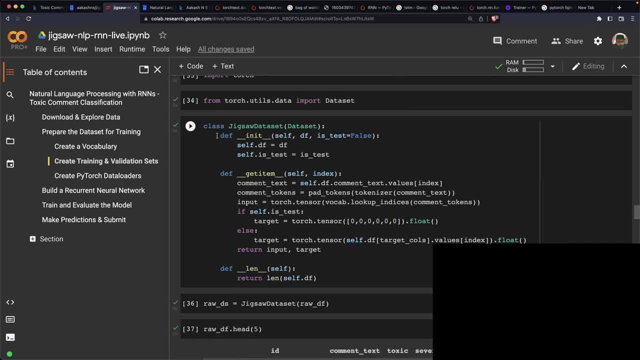 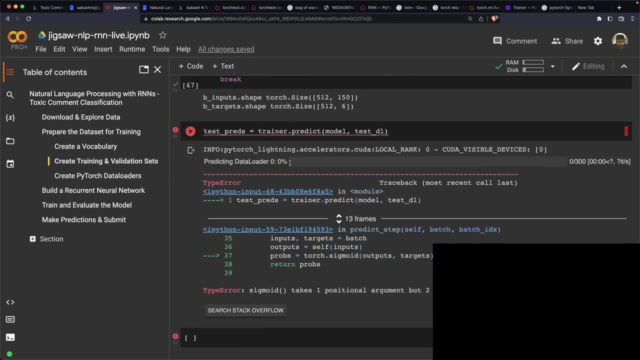 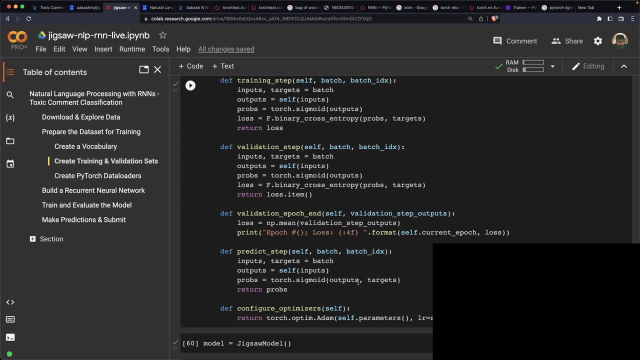 their loan length 150.. Then we created a pytorch data set which requires- I'm just going to check quickly if things have run okay. still one last issue that needs to be fixed, which is we do not need to pass targets here. 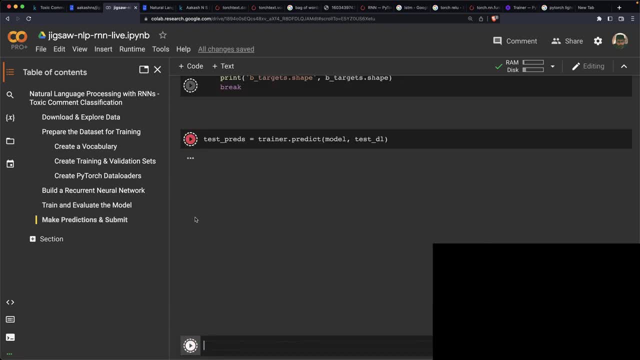 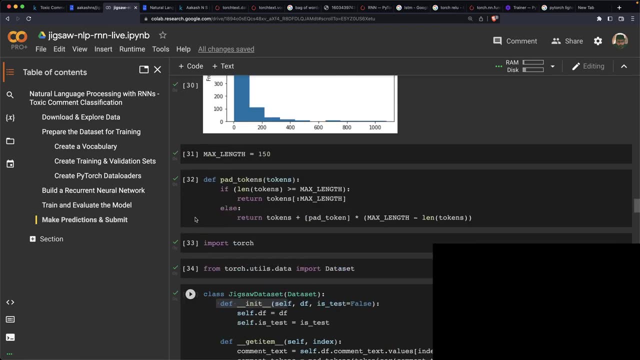 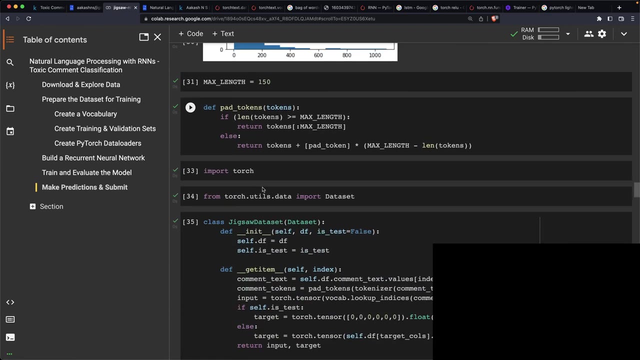 I'm just going to run this one last time. All right, So then, coming to how we decided to create pytorch data sets. So first we decided that we are going to pad the tokens to a length of 150, or trim longer sentences to a length of 150 tokens. 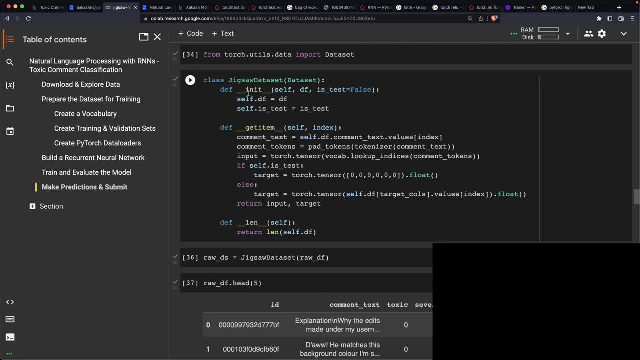 Then we created a pytorch data set, the jigsaw data set, and the jigsaw data set is going to be initialized with a data frame and with is test equals true or false. Now we have to define a get item function in any pytorch data set. 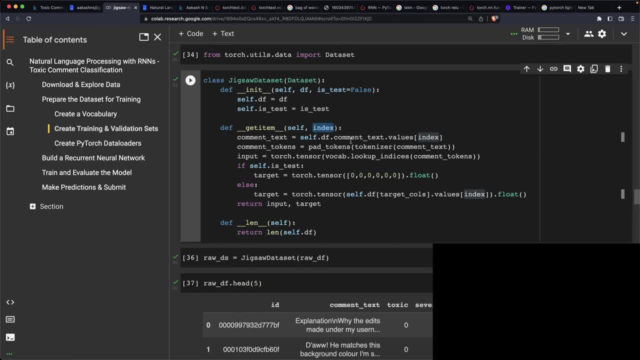 Given an index. we are going to first get the common text from the data frame that has been stored inside the data set, And then we are going to convert those, the common text, into tokens And then we're going to pad the tokens to get the tokens for that comment. 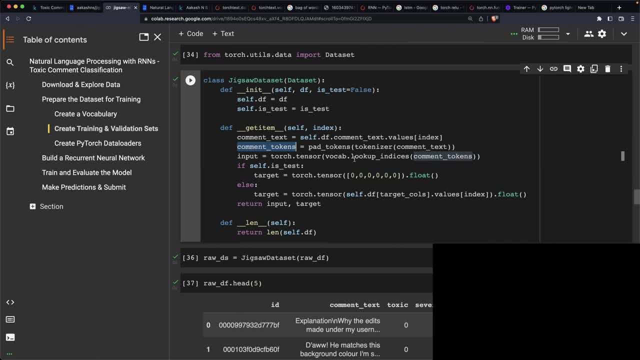 Then we are going to look up the indices for those tokens, to convert the tokens into numbers and convert that into a pytorch tensor. That is going to be the input. Now, in case, this is a test data frame, we are simply going to return the target of all. 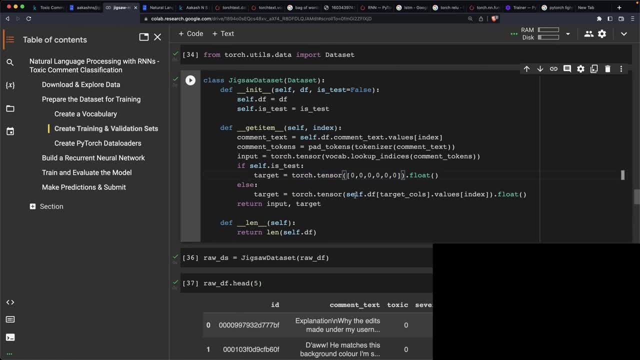 zeros, Because it's not going to be used Anyway. but in in case this is a training or validation data, then we are going to get the target columns. from the target columns, We're going to get the values and we're going to get the get the values at the given index. 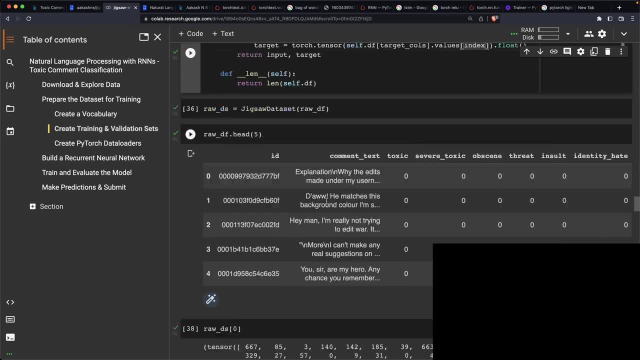 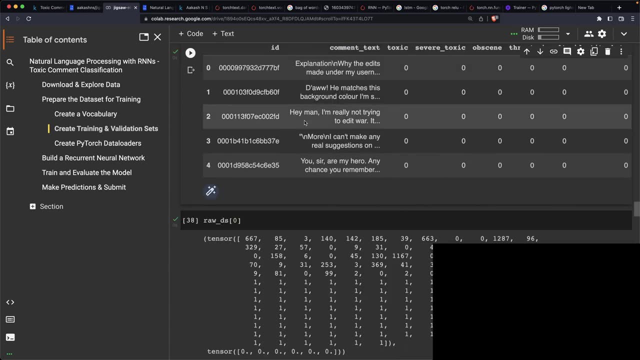 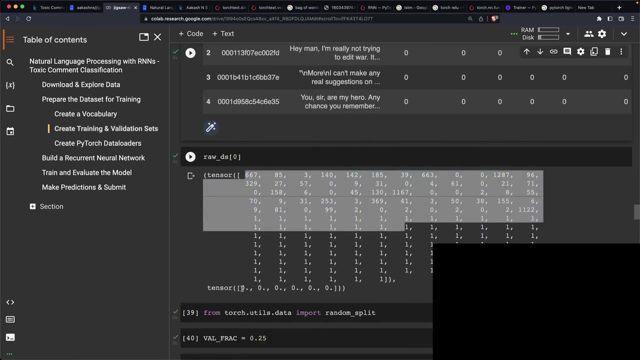 and convert them into pytorch tensors and return it. And that is how we create the data set, the jigsaw data set, And then we can check that, since we can check that the first element here corresponds to the first comment here in the raw data frame and has the proper targets as well. 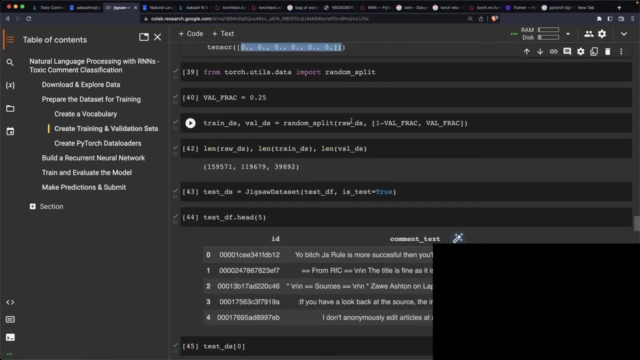 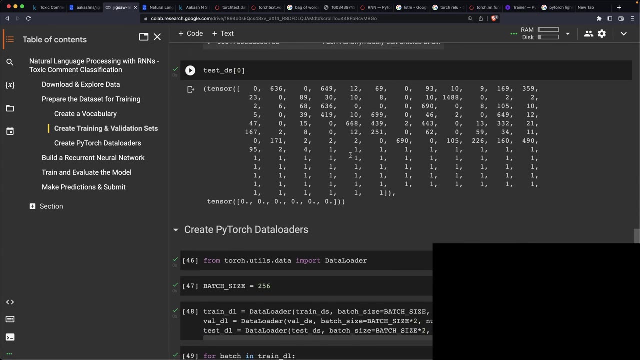 Then, to create training and validation data sets, we use random split, So we pass raw data set and we give it one minus valfrac, which is 0.25 as the size of the training data, and the rest is the validation data. And then we also create a test data set and here we pass: is test equals true. 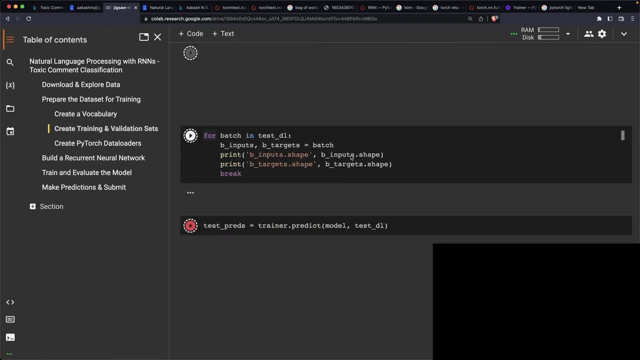 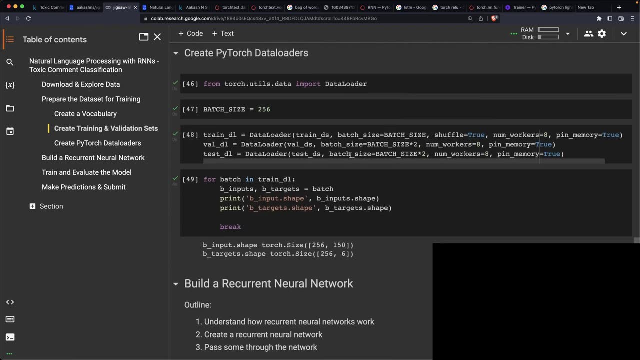 Then we create pytorch data loaders. Let's see if this is completed. Okay, This is currently in progress. So then we create pytorch data loaders Because we have to process the data in batches. we use a batch size of 256.. 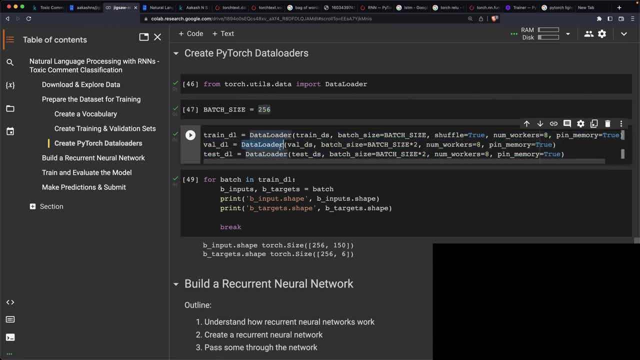 We create a training data loader, a validation data loader and a test data loader, And in the training data loader we use shuffle equals true, because we want to shuffle the data before we create batches from it in each epoch And we can check that we get back. we get back batches of data. 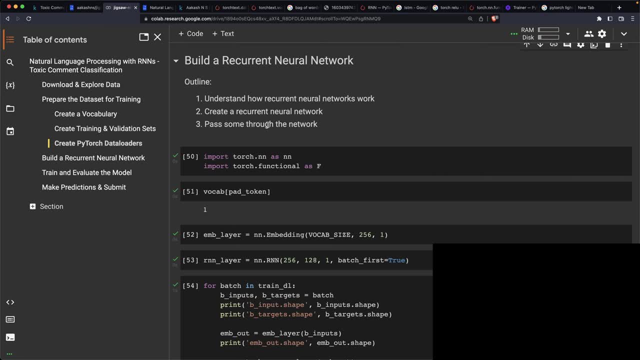 Then to build recurrent neural networks. We first understood how recurrent neural networks work, which is by essentially like a for loop: taking the first Data, taking the first word, converting that into a vector using an embedding layer, passing it through a recurrent layer and which takes a also default hidden state, returns an output. 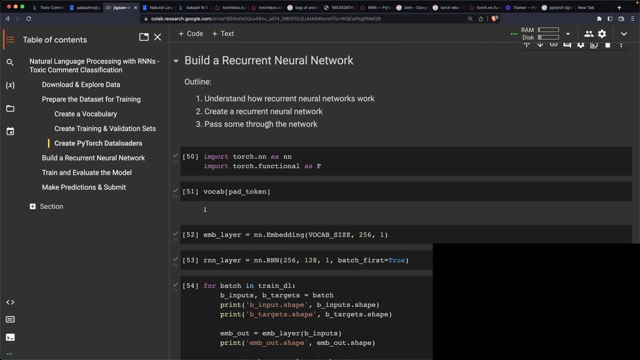 returns a new hidden state. The new hidden state is then passed once again into the recurrent layer along with the word vector for the second vector, And that process is repeated 150 times And we get an output for each of those 150 times. 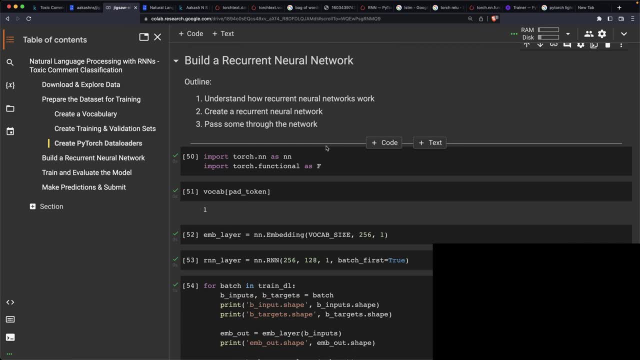 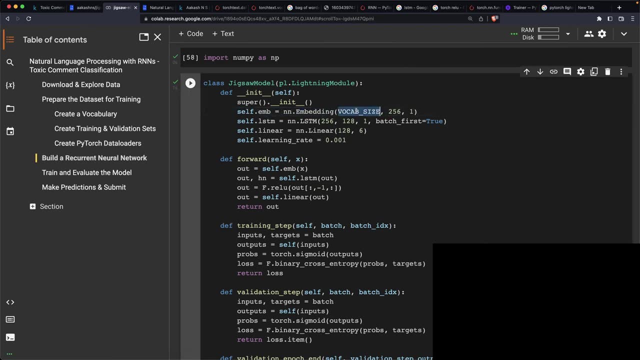 And we take all those outputs And from those output we just pick the last one and pass that into a linear layer. So that's what we created. So here we create an embedding layer which starts with the vocab size. So, given an index, it returns a vector of size 256. 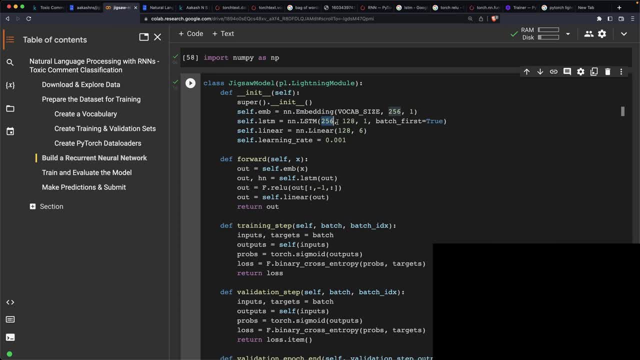 Then we can use an LSTM which takes that vector size 256. And it takes a hidden state of size 128, it returns a new hidden state and it returns an output, both of size 128. And that it does over each of the 150 tokens within each input within the batch. 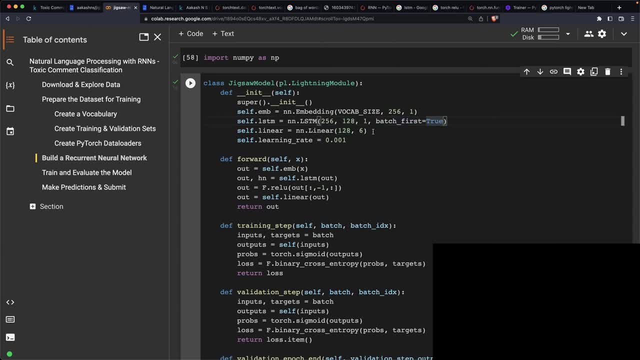 And of course you have to specify batch first equals true here as well because of how the data is structured. Then we take the output of the last batch and we are going to pass it through a linear layer And all that logic is captured here under the forward method. 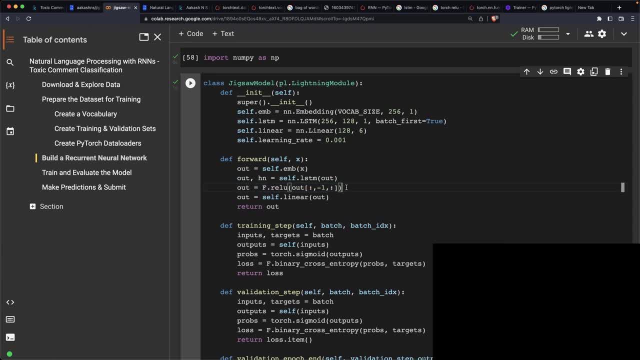 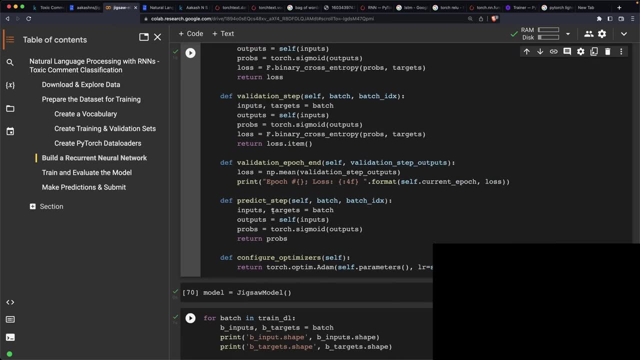 And in between, after the LSTM layer, we also have a relu activation. then we define the training step, which is what to do with a batch of training data. we defined a validation step and we defined the predict step And right now we have trained the model and the model reached a loss of 0.64.. 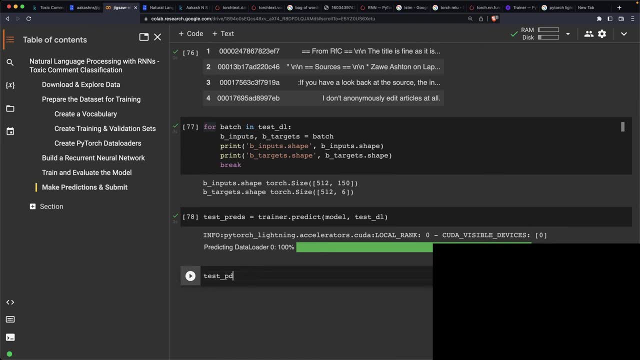 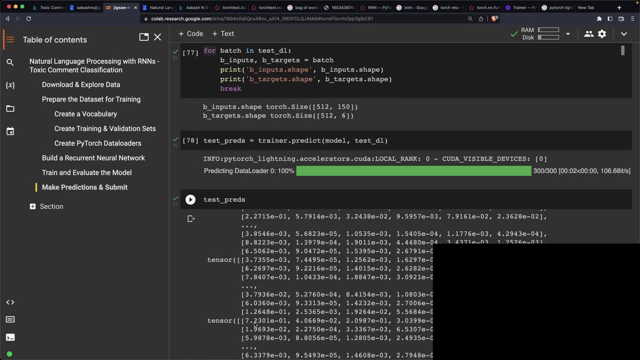 And then, finally, we have finally have some test predictions as well. So let's look at test prets. So the test spread contains a list And in the list, each item is basically the information, basically the result of the output of the model on one batch of test data. 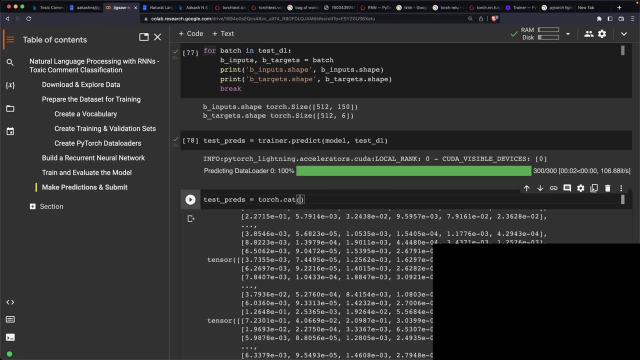 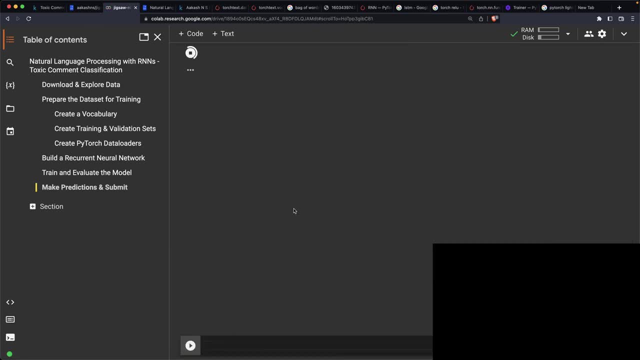 So here's what we can do. we can say: test prets equals torch dot cat test prets, And it's going to take each the data from each of the batches and it's going to combine them all together into a single tensor. 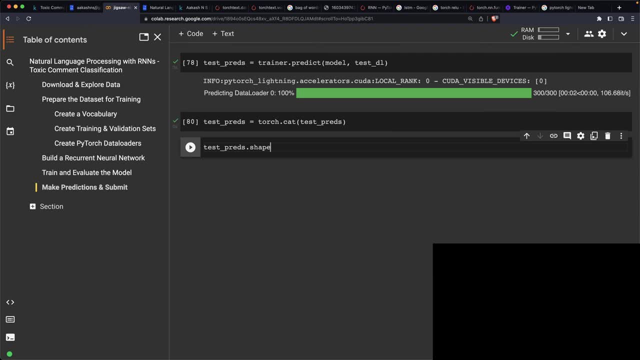 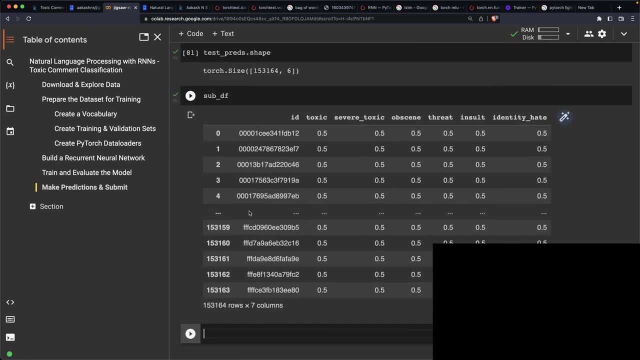 So now we can check test breads dot shape. You can see that now we have 153, 164 values in. we have six values for each And we can now go back into a submission data frame and put these. put this information back into the submission data frame. 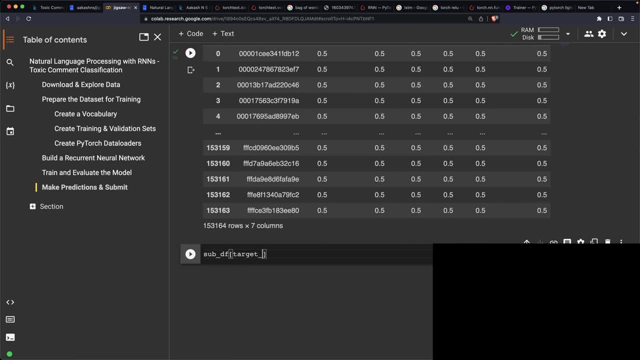 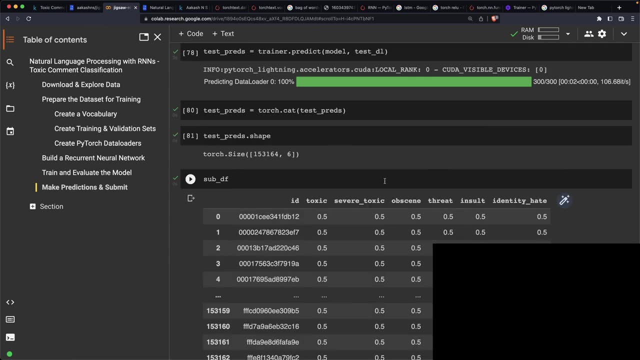 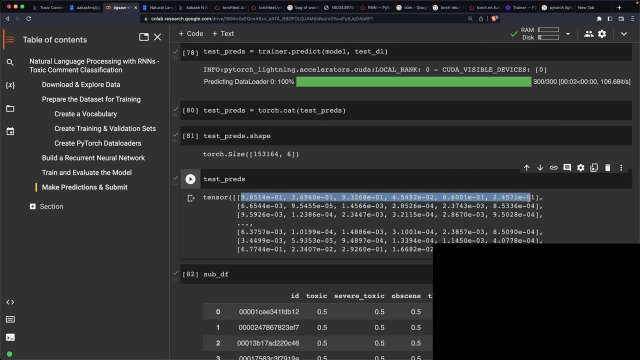 So let's say sub df equals or sub df target calls equals. test breads. Let's look at test breads also, what it contains. Now, one thing to keep in mind is that these values- so we have six values for each row in the test data- 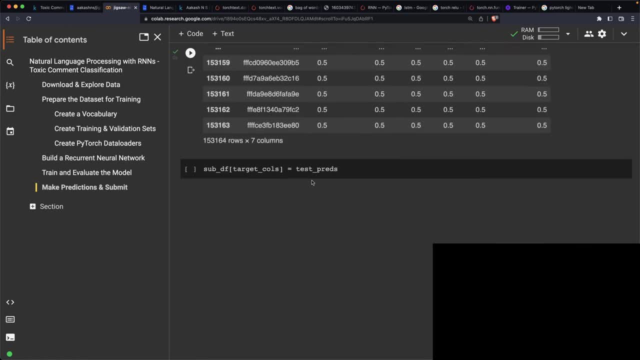 One thing to keep in mind is that these values are pytorch tensor, So you may want to just convert them into NumPy arrays. So I'm just going to say dot detach first, dot CPU, dot NumPy. That's just going to convert these into NumPy arrays. 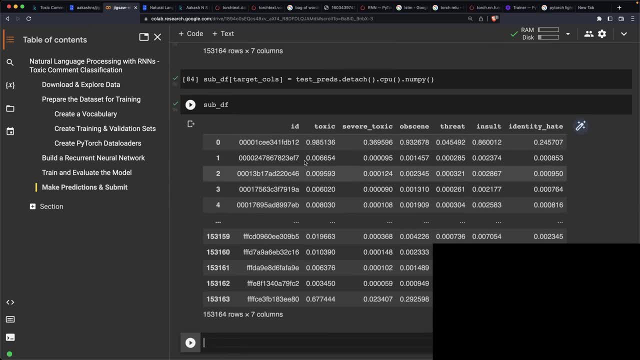 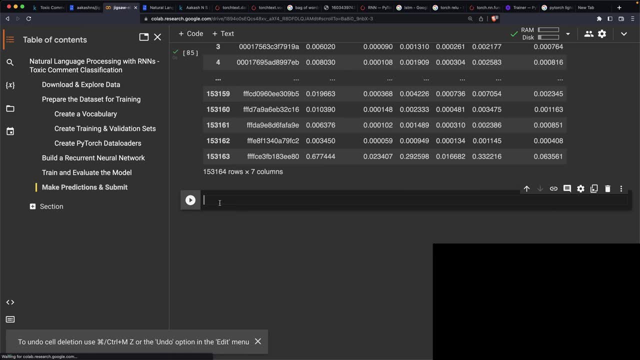 And now Our submission data frame contains a bunch of useful predictions from our model. So we don't need this And now we can just save it as CSV. So now we can say: sub df, dot, two CSV, submission dot. CSV index equals none. 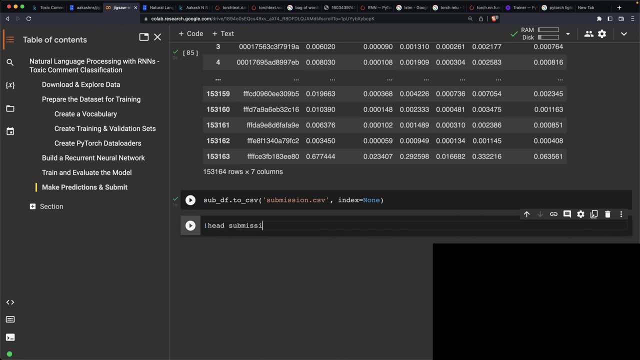 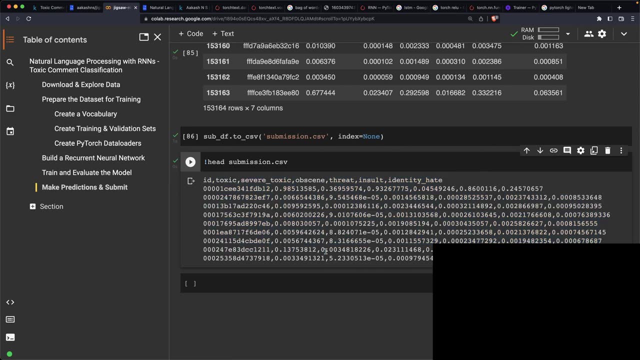 And that is going to generate a submission or CSV file. You can see here a submission or CSV file has been generated And it contains, for each ID, the predictions of our model. we can now go in and we can download the submission or CSV file. 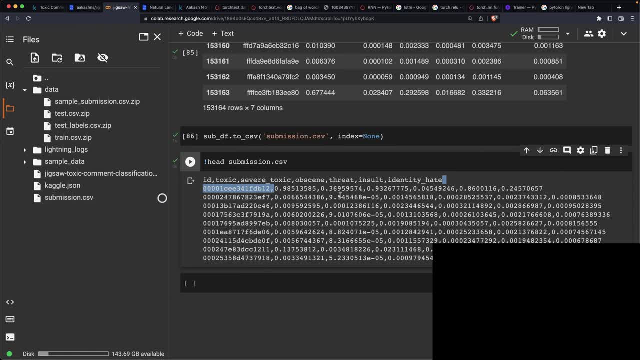 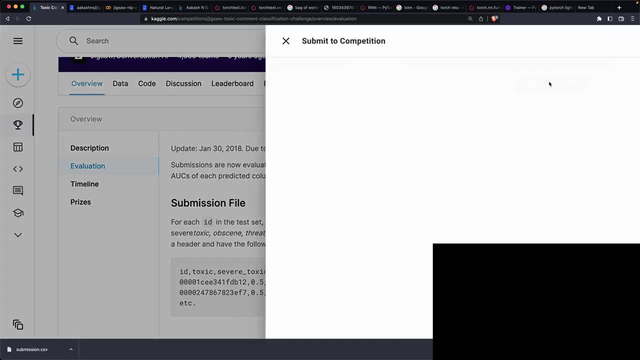 Let's go in here, Let's download the submission or CSV file to our computer And then let us upload the submission or CSV file here under late submission And let's put in a description here: So this is an LSTM single layer, And let us click Submit. 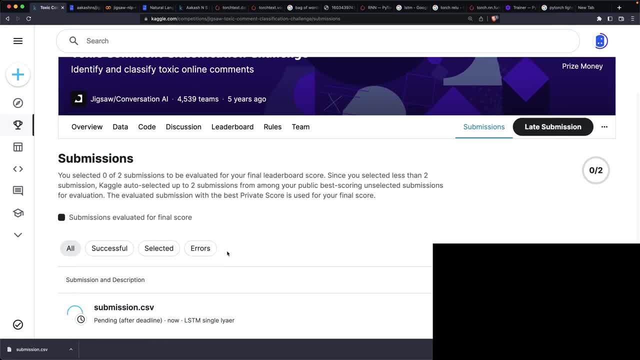 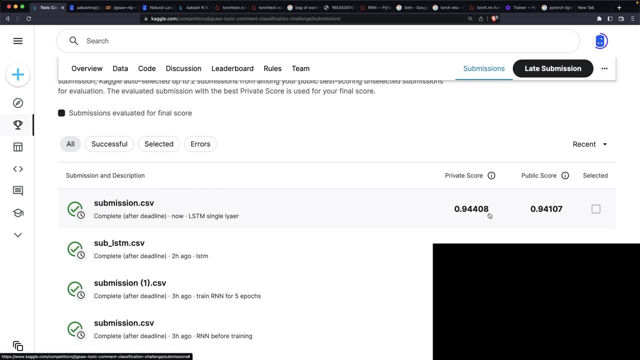 And let's see what happens to this. Now we've just made the submission, And the submission is going to get evaluated, and the submission gives us a score of 0.944.. All right, that's pretty good, So let's go to the leaderboard. on the leaderboard, 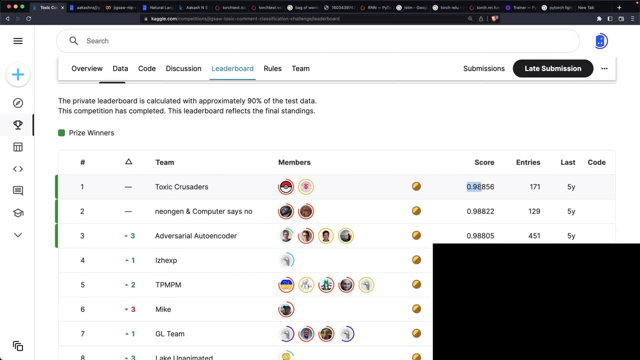 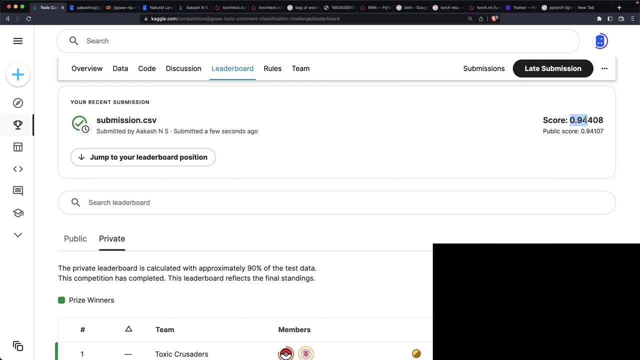 And this is the ROC AUC On the leaderboard, the best score is 0.98.. And we have obtained a score of 0.94.. And we have done it in under two hours after making so many mistakes, Right? So that's pretty good. 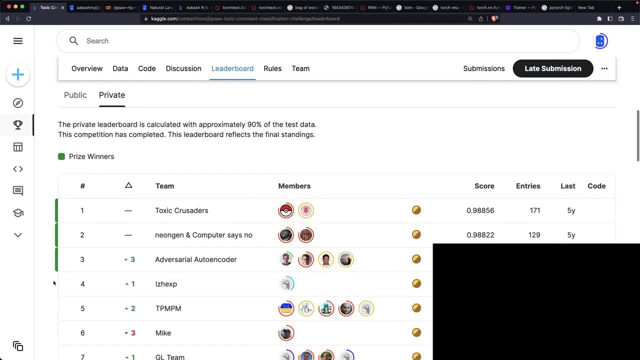 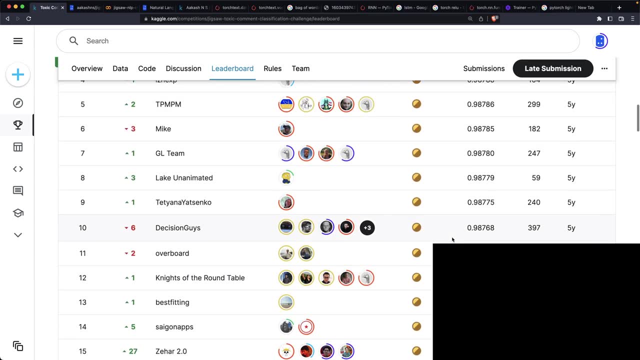 And considering, we've just have a single layer LSTM. we've not done anything fancy here. We've not modified any hyper parameters. we're just using the most basic version. we're just using a very simple learning rate that's already present. Of course, if you actually look at where 0.94 lies, it might be very low. 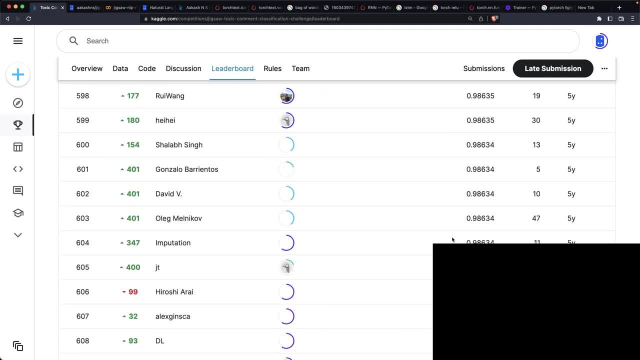 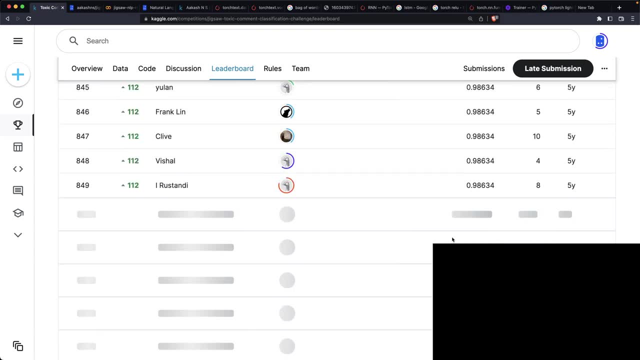 And that's because this is an old competition and a lot of people have participated at the time and they've probably created some public notebooks which others were able to use. But just as an overall number, if 0.98 is the best score and you have gotten to 0.94,, 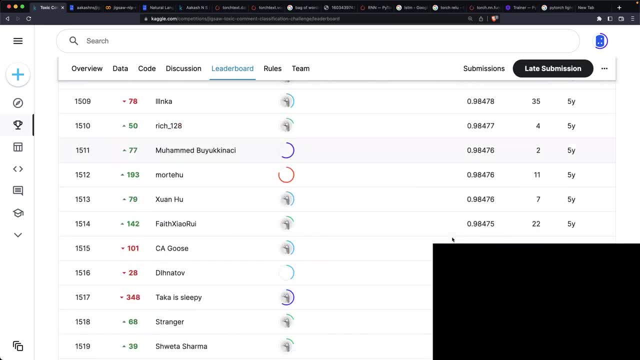 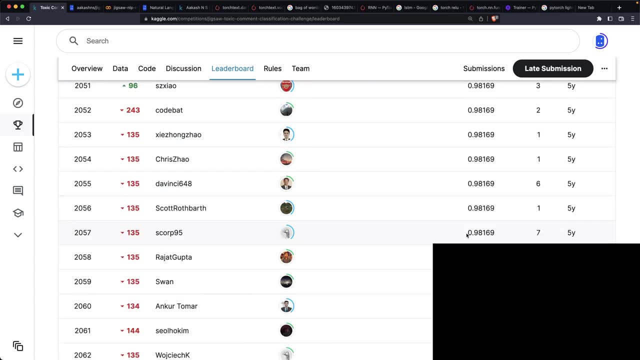 that is pretty good to begin with, And of course I encourage you to now experiment with it and get to a better score. Yeah, you can see that you have to kind of really scroll down a lot. there are a lot of people at 0.98.. 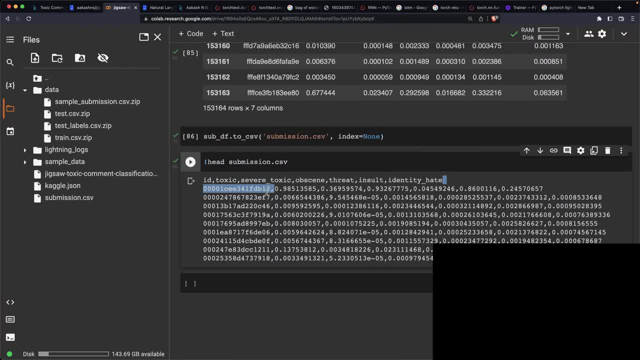 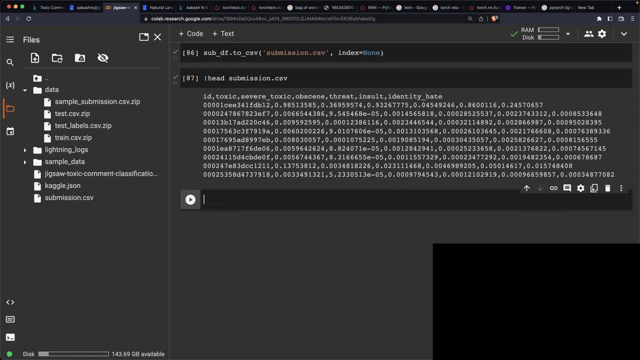 So that could be the best score. That could be the next challenge for you: to get to the score of 0.98.. So let's maybe also look at some predictions on some actual data. So let's get a sample. the sample df equals raw df. dot sample n. 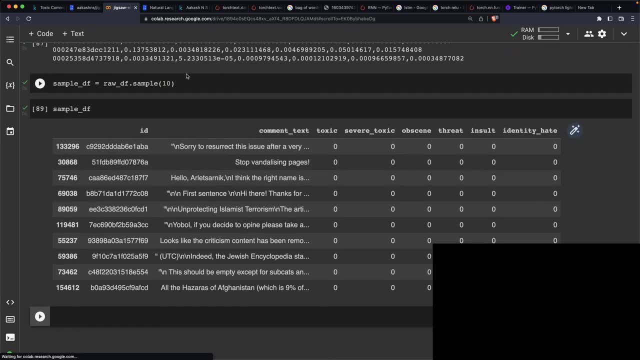 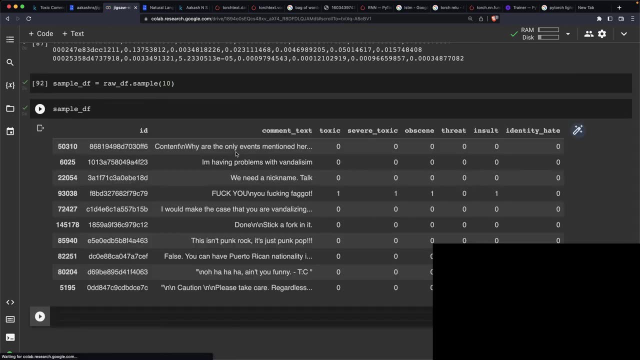 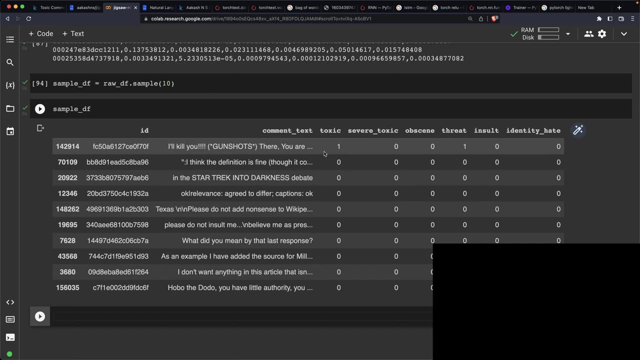 Let's look at sample df. let's try to get a data frame which contains a good mix of: okay, Let's try again. Yeah, so let's see something where we have: Yeah, so here there is this comment. I'll kill you. 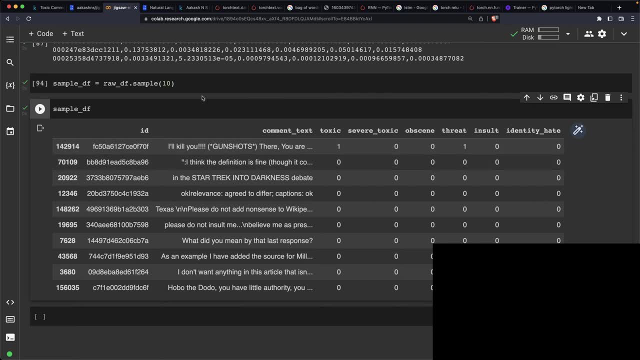 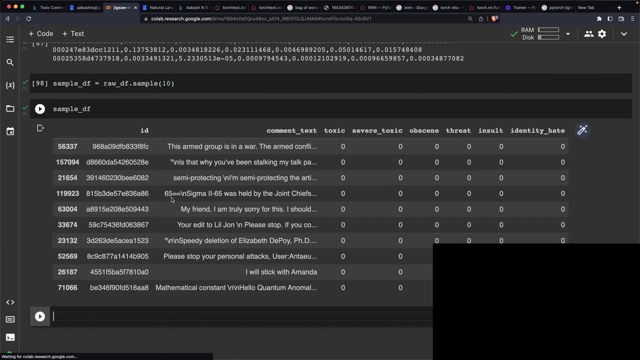 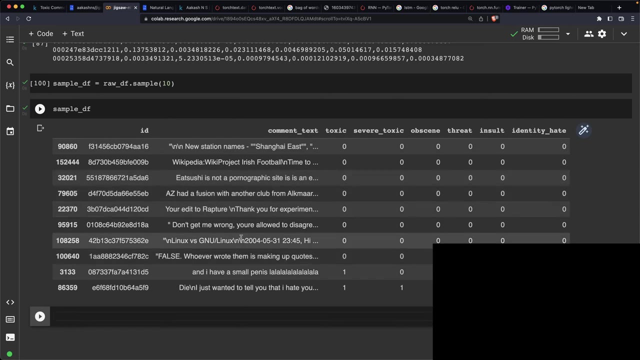 That's definitely definitely somewhat toxic. Let's try a couple more times. Let's see if we can get 10 where we have some variation, some good variation between the data. Okay, so here definitely you can see here that this is a toxic comment. there is something. 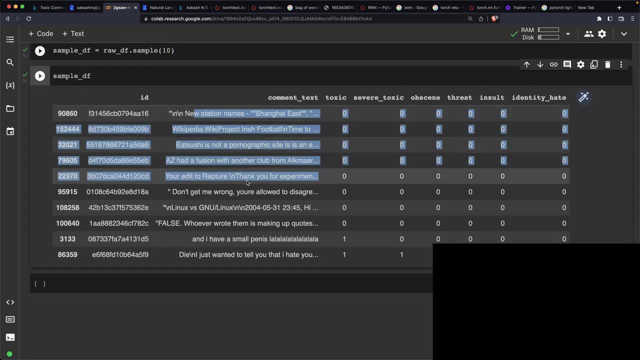 derogatory being said here. none of these are toxic comments. that's fine. And then here again there's like a threat here. So this is a fairly toxic and threatful comment as well, or identity hatred related comment. Okay, so now we have a sample df. I'm going to first create a sample data set a sample. 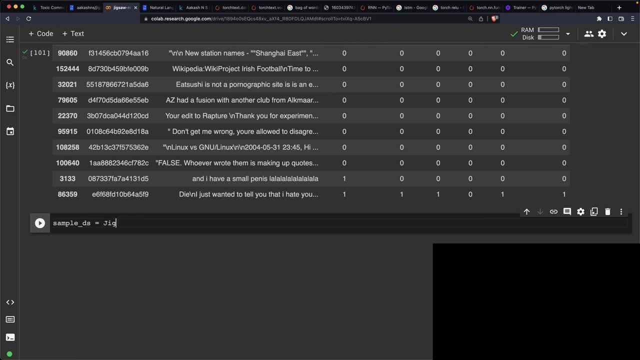 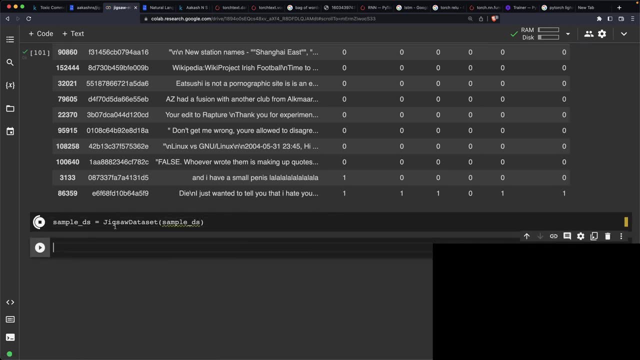 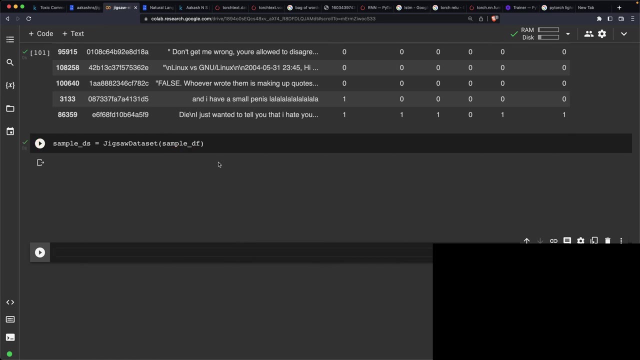 DS, which is going to be a jigsaw data set. Okay, sample df. sorry, And this is not a test data set, So I'm going to just keep this information here. Then let me create a sample data loader. So this is going to be data loader. 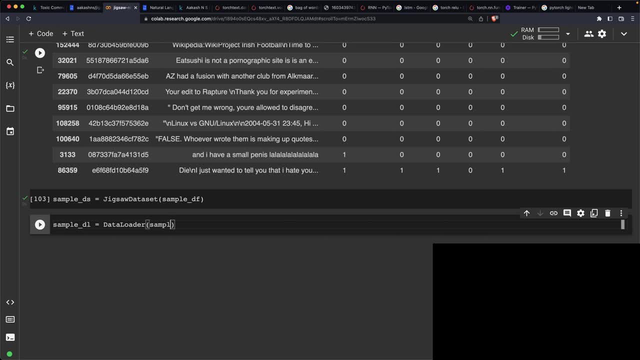 And I'm just going to give it sample DS and nothing else. You don't need to configure anything. actually, I will pass a batch size, So let me pass a batch size of 10.. So that, so there's just one, One batch in the data. 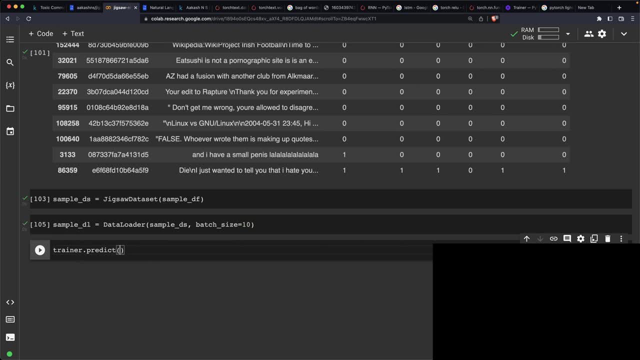 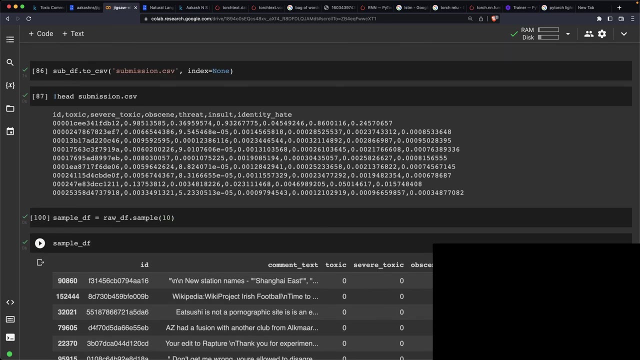 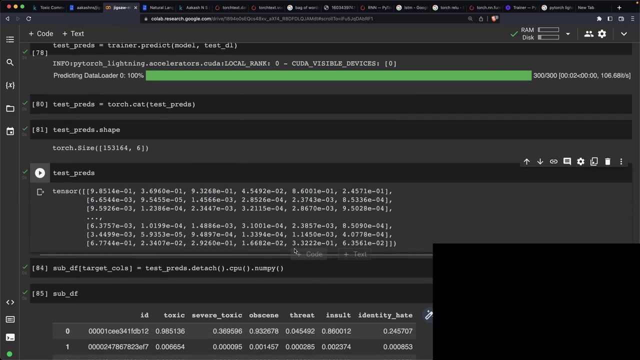 And now let us say: trainer dot, predict model and sample DL, The sample threads. well, actually, one thing we should also do is we should convert these into probabilities, which we haven't done. maybe that might give us an even better score. 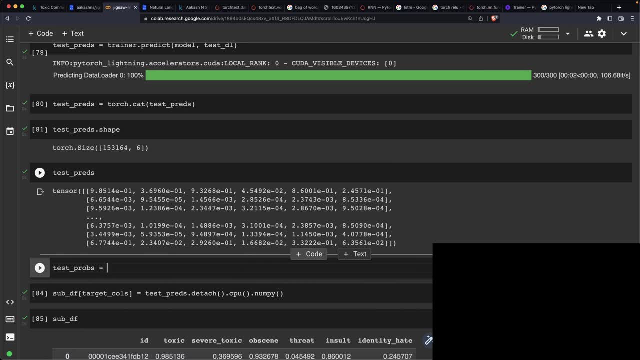 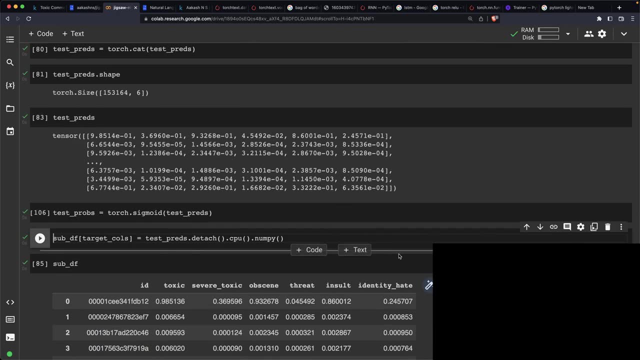 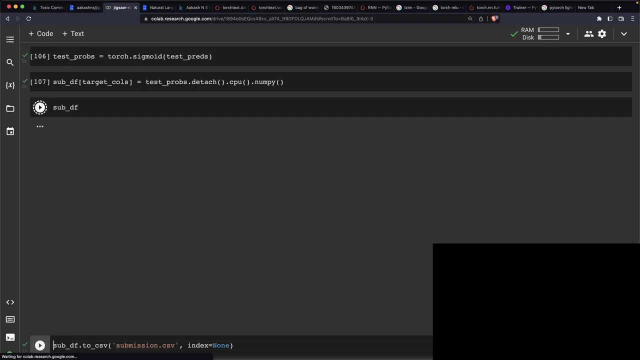 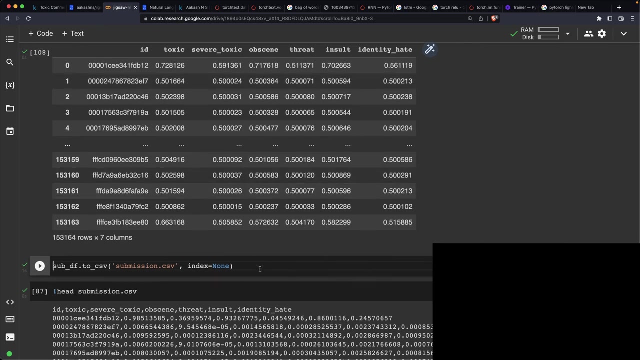 So test props equals torch dot sigmoid test rates. And then let us just make it test prompts, Yeah, and I'll let you submit that and check it out if that actually gives a better result. Because the predictions of the model are not. we have not applied sigmoid onto them. 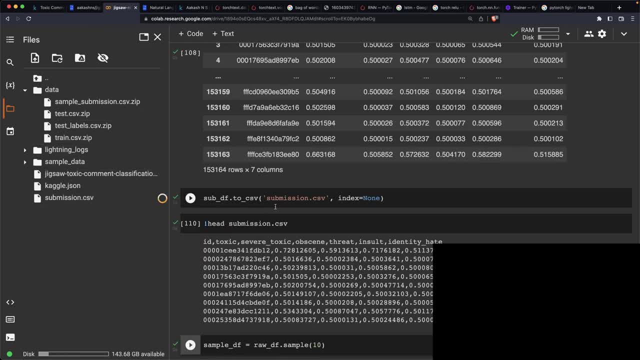 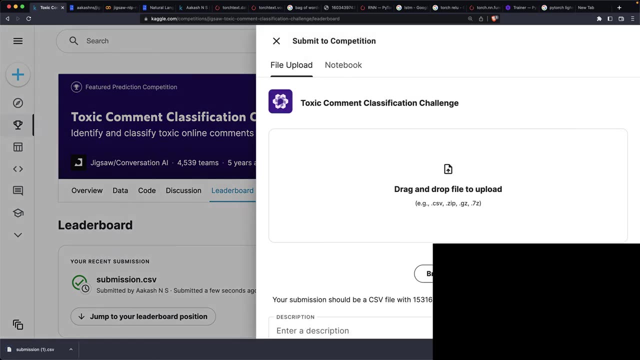 Let's see. let's just download this and see Submission one. let's go back here. Let's click late submission. Let us browse submission one- dot CSP And we'll make actually converting it into probabilities, And let's click Submit. 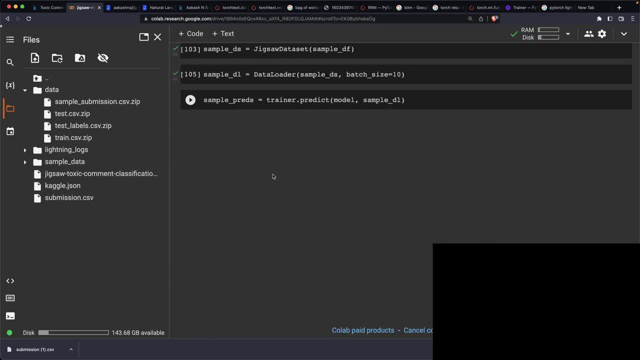 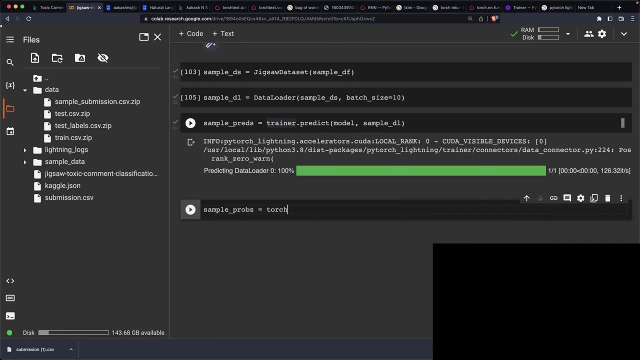 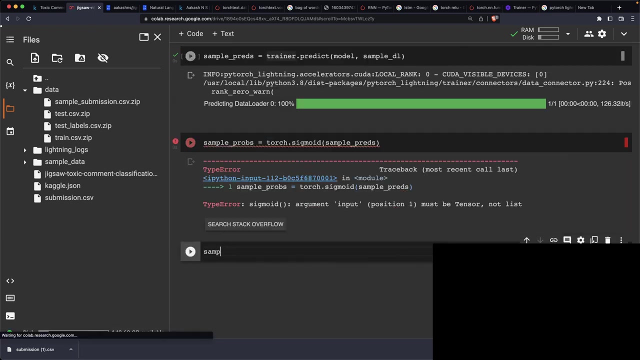 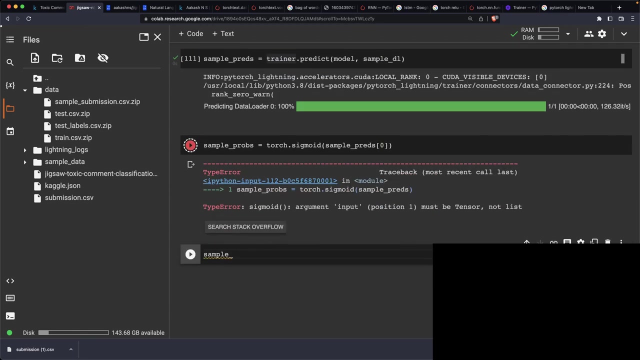 So we'll check out the score in a moment, But right now we are just looking at the predictions for a sample data, And sample problems are simply torch, dot, sigmoid sample rates. And let's look at sample zero, because this is going to get information for from a batch. 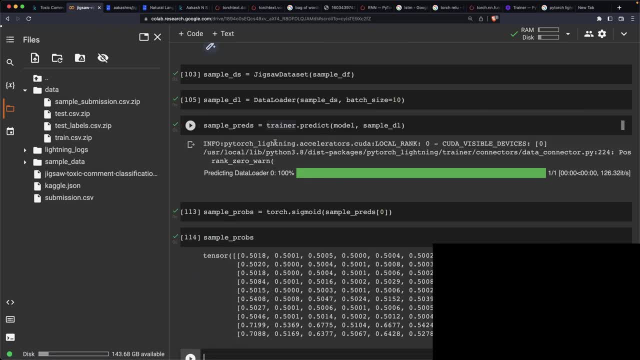 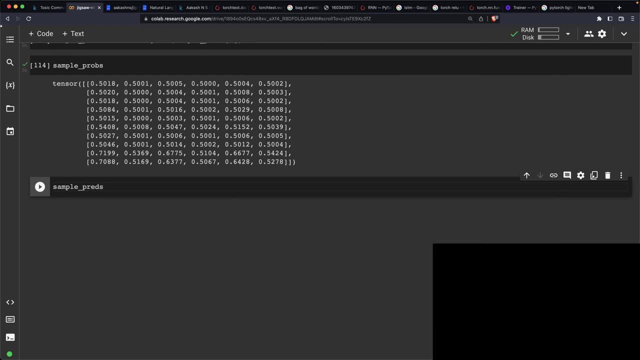 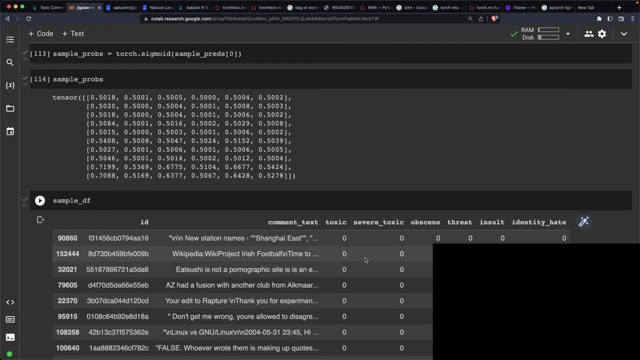 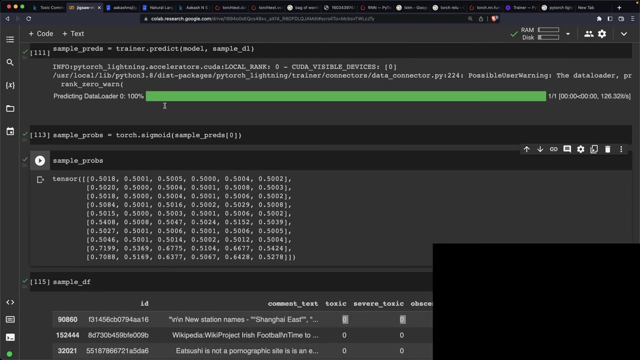 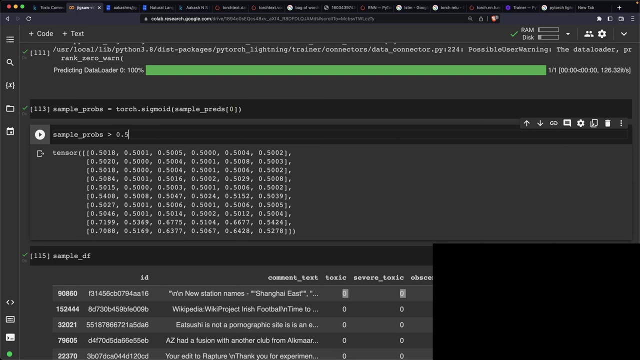 Let's look at sample problems And let's compare the sample probabilities with the sample DF Yep. So here you can see it is predicting something just slightly higher than 0.5, which not doing a great job On this data set. you can actually just check sample problems greater than 0.5. 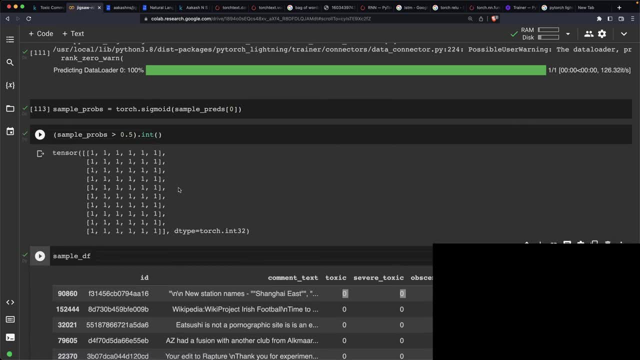 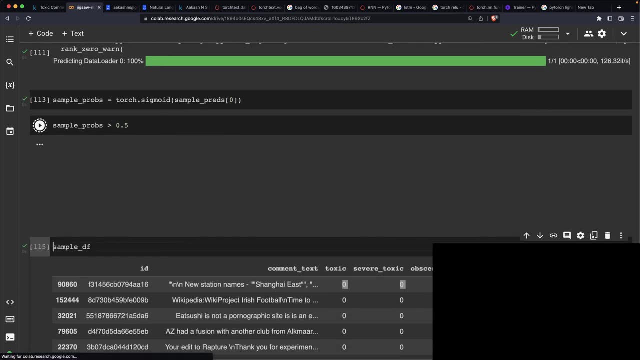 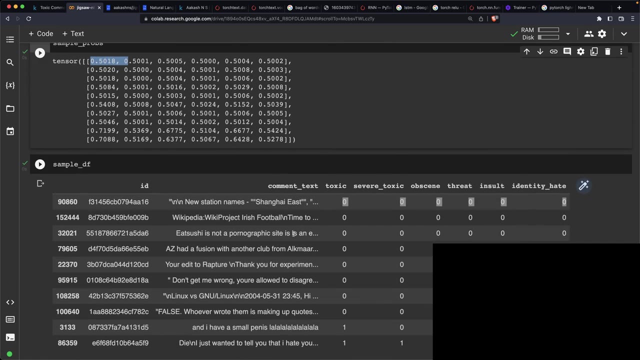 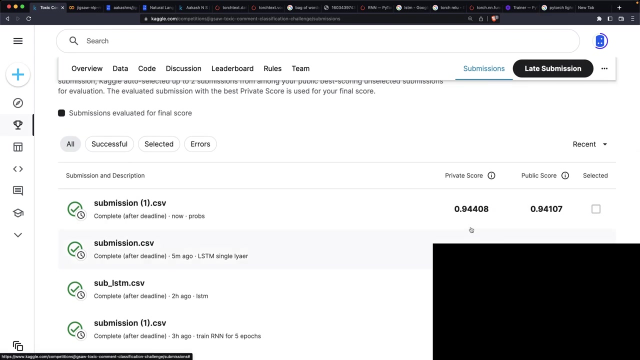 Not in. Yeah, maybe that's why we have the ROC here. But one thing that you can do here is you can actually look at these probabilities and compare whether these probabilities make sense. on this data as well, Let's see it returns about the same score: 0.944. exactly the same, actually in private. 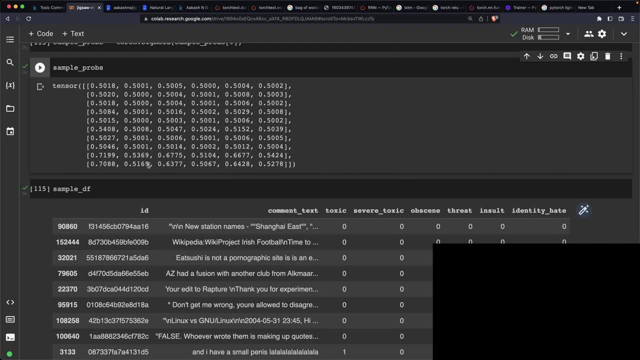 but, as we can see here, We might have to maybe play around with the threshold a bit right. So, because almost all of these predictions are a slightly higher than 0.5.. So leaning a little bit towards one. So actually we might want to set the threshold at maybe point 60.6 or something like that. 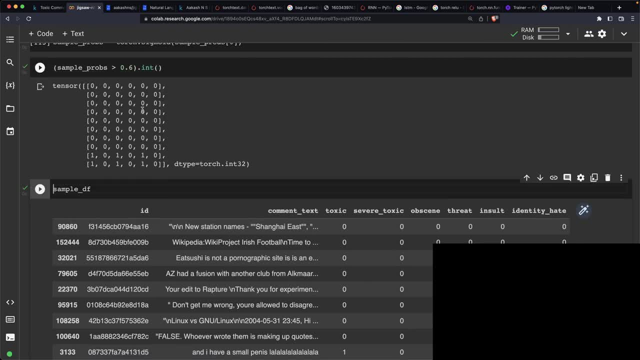 And if we set the threshold at point six and we check, this is the prediction that our model gives us. okay, so this is the thing with ROC AUC, that it actually checks across a bunch of thresholds. Okay, By converting the probabilities into actual predictions, you might have to just check. 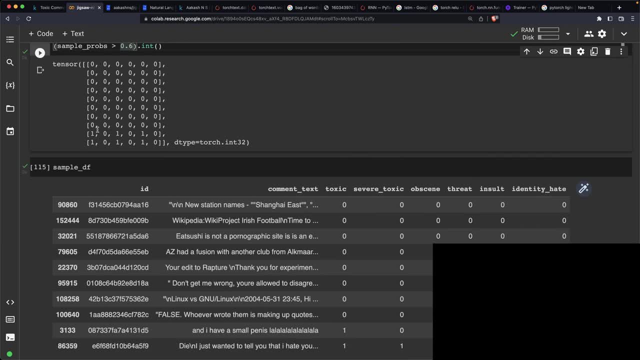 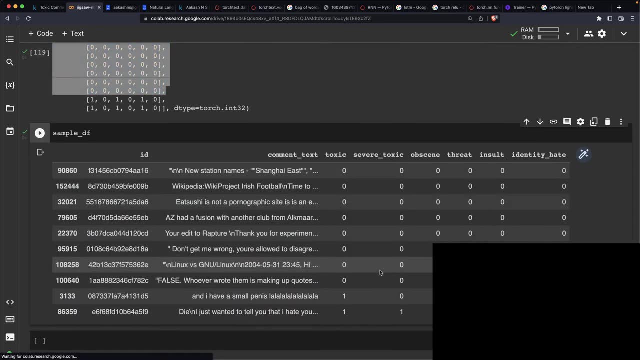 you might have to play around with the thresholds a little bit. Okay, so clearly this here. all of these are zero, And our model is also detecting all of these as non toxic, But the last two are definitely toxic. So this one is just toxic, but it is also detecting it as obscene and as an insult.